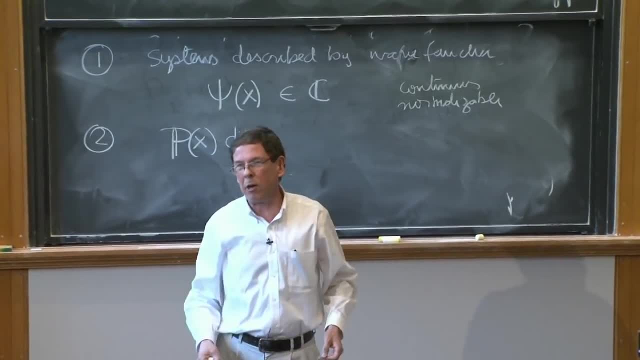 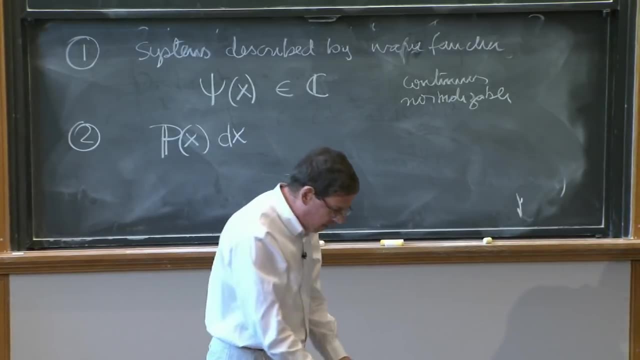 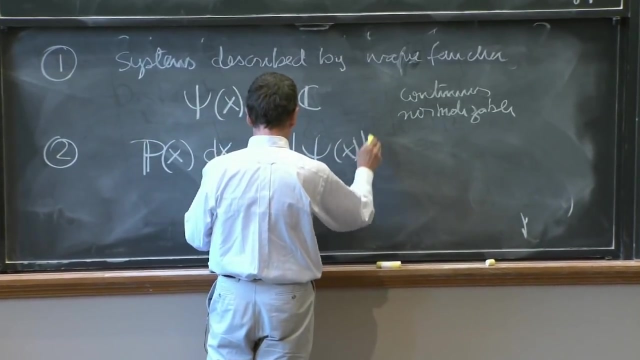 what is the probability that the particle is just at this point? It would be 0. in general, You have to ask typically, what's the probability that I find it in a range? Is any continuous variable That's postulated to be given by the square of the wave function. 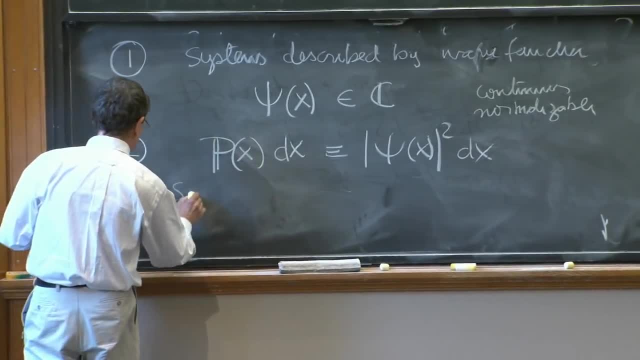 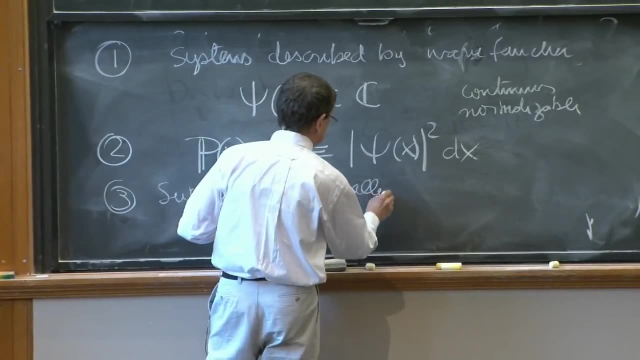 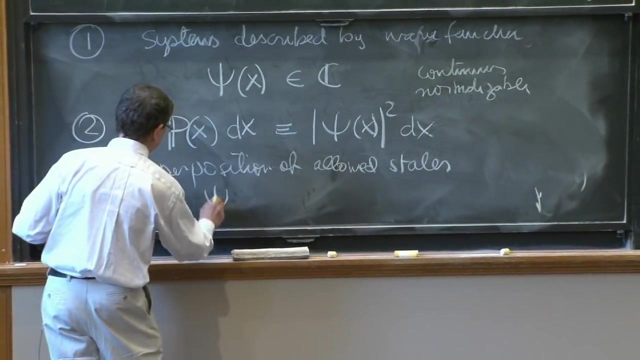 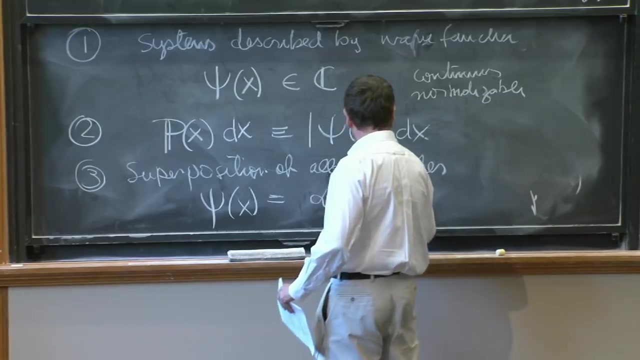 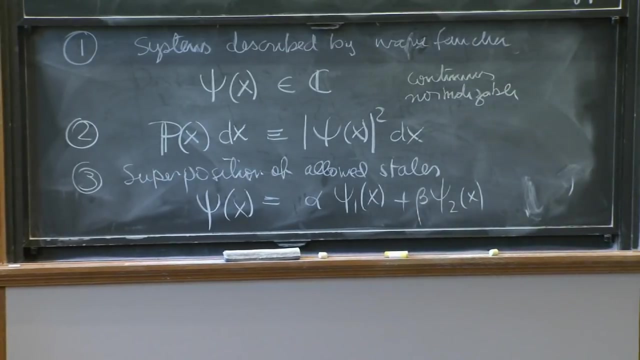 and the x. Third, there's superposition of allowed states, So particles can be in superposition. So a wave function that depends of x may quickly or generally be given as a superposition of two wave functions, And this is seen in many ways. 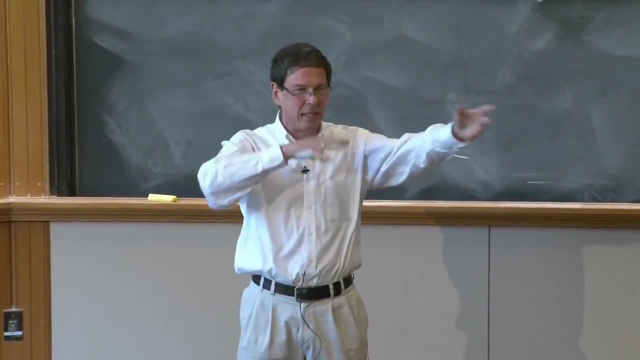 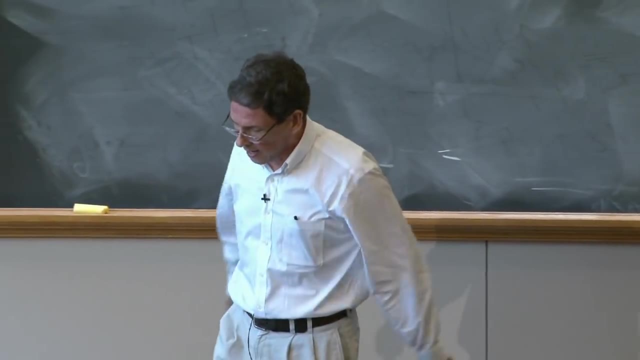 You had this box as a particle was a superposition, a top and side and hard and soft, and photon superposition of linearly polarized heat And you can see that it's either polarized here or that way. That's always possible to explain. 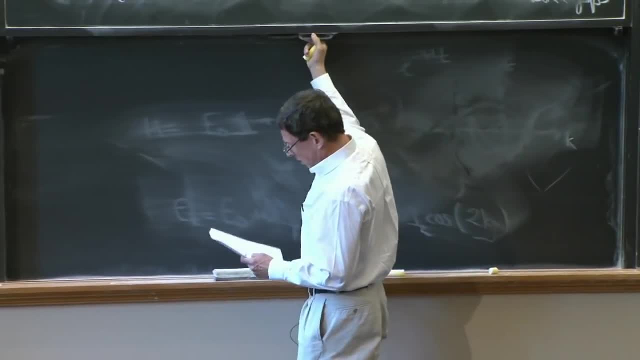 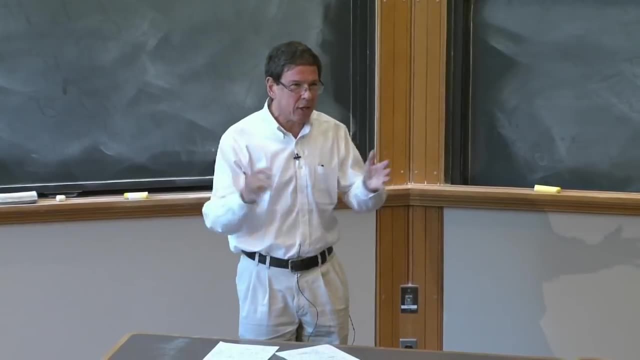 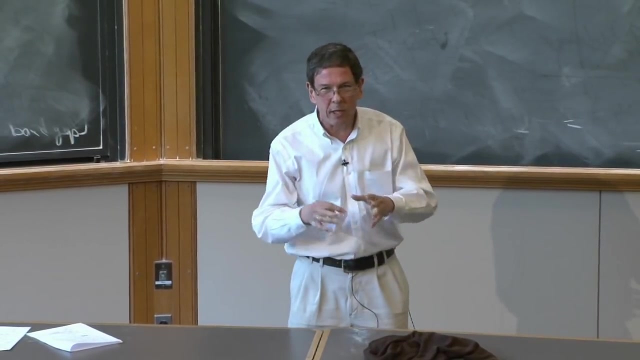 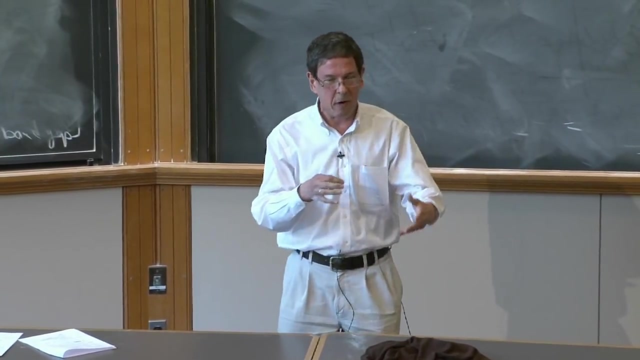 Now, in addition to this, to motivate the next one, we talk about relations between operators. There was an obstruction going on in this lecture, in this course, in the previous lectures, in which the idea of the momentum of a particle is associated with that of an operator on the wave function. 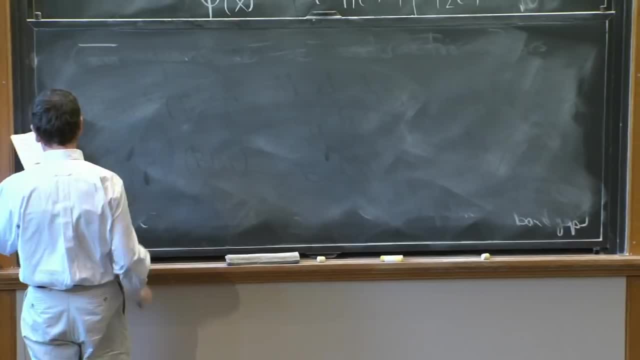 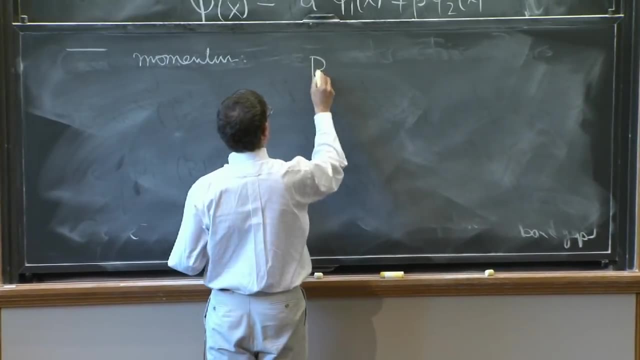 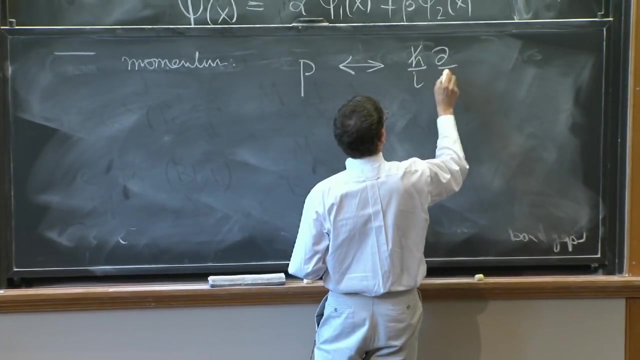 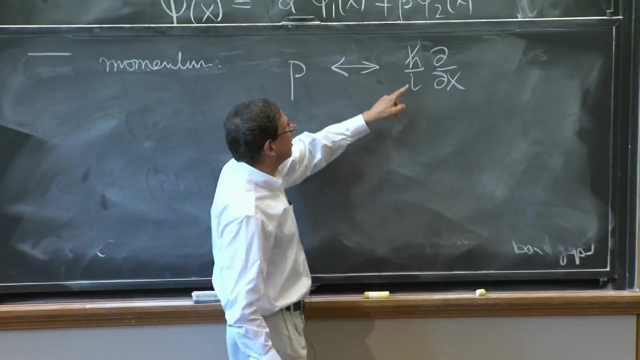 So we've been. so as an aside. operators, momentum, momentum. we have that the momentum of a particle has been associated with an operator. h bar over i, d, dx. Now two things here. I my taste: h bar over i. 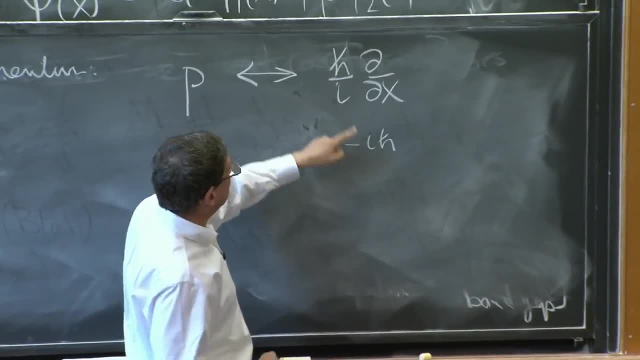 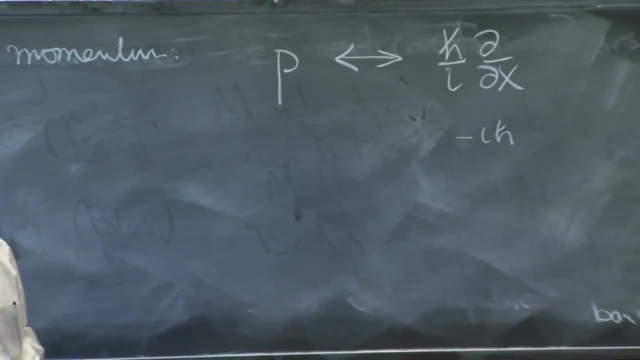 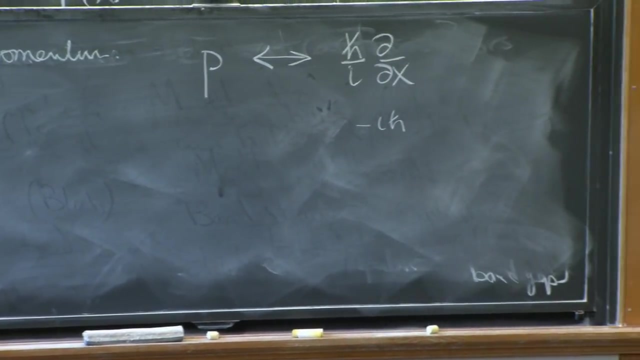 Alan likes to put ih bar. That's exactly the same thing. But no minus signs is a good thing in my opinion, So I avoid them when possible. Now there's d dx here. It's a partial derivative And there seems to be no need for partial derivatives here. 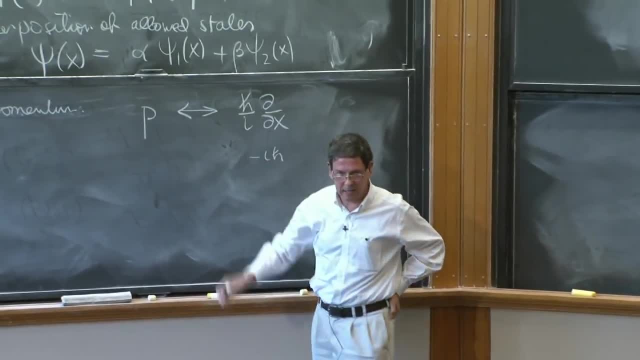 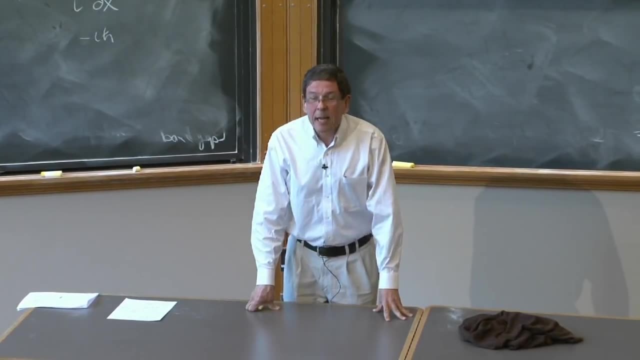 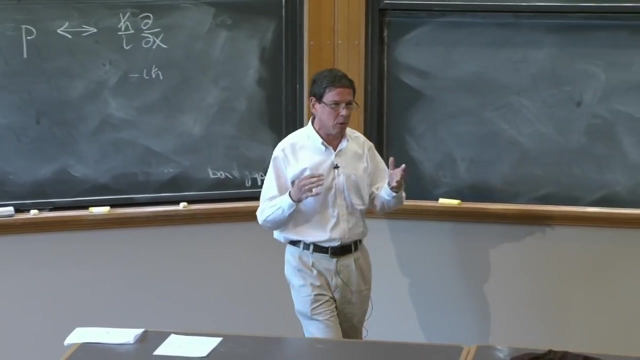 Why partial derivative? I only see functions of x Anybody Why? Yes, The complete wave function also depends on time. Complete wave function depends on time as well. Yes, exactly That's where we're going to get to today. 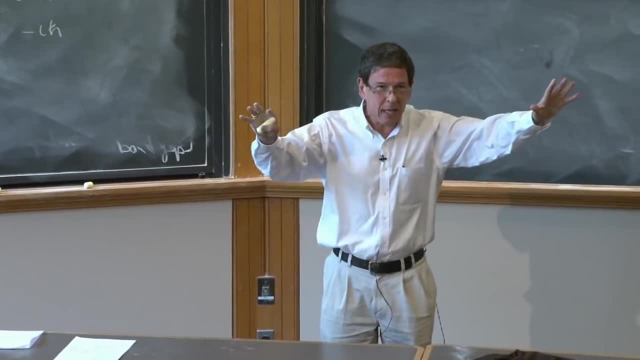 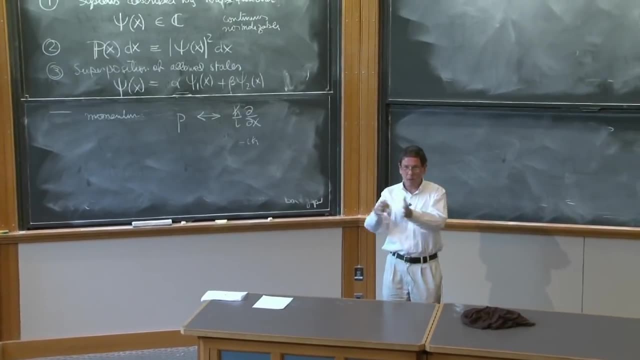 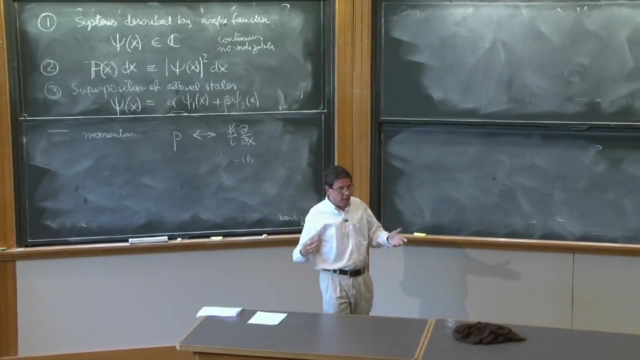 This is the description of this particle at some instant. So we didn't put a time. The time here is implicit. It could be at some time now, later some time, But that's all we know. So in physics you're allowed to ask the question. well, 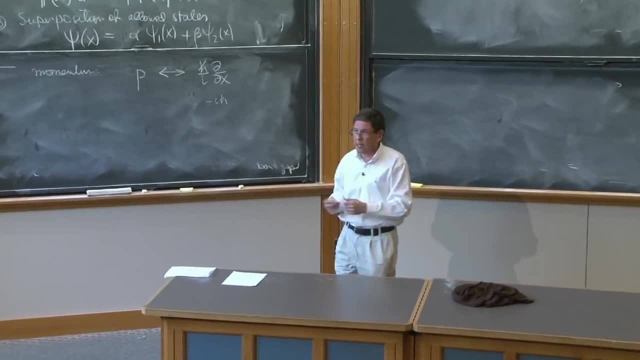 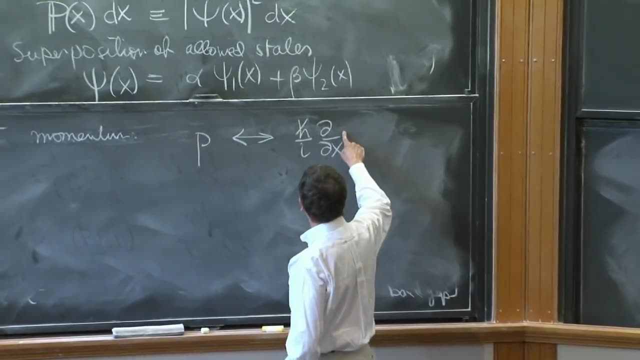 if I know the wave function at this time- and that seems to be what I need to describe the physics- what will it be later And later time will come in. So therefore we'll stick to this partial d dx in here, All right. 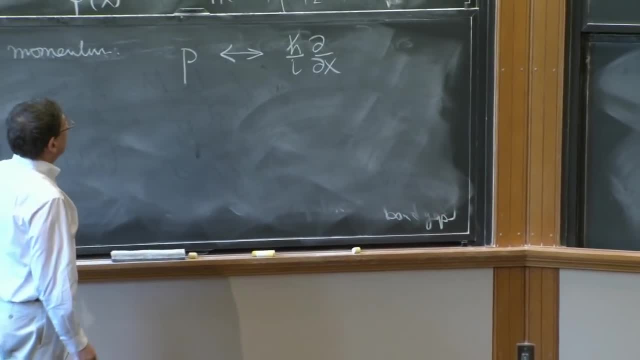 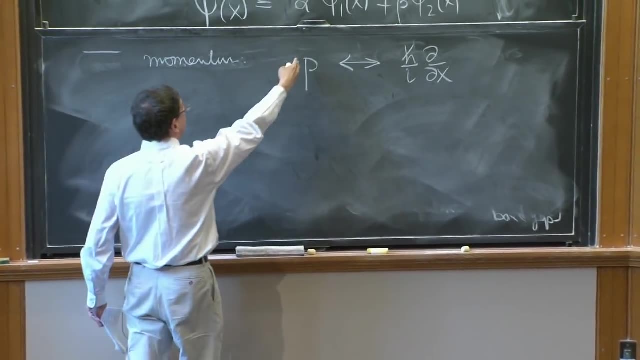 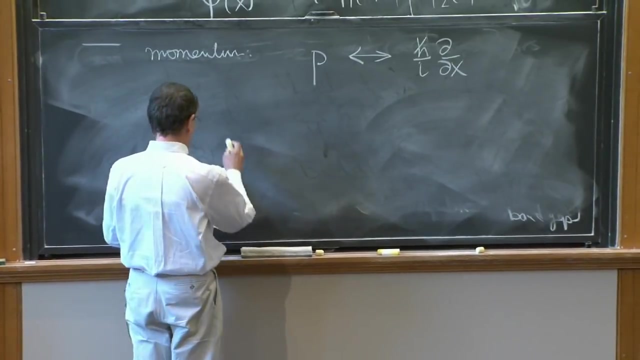 So how do we use that? We think of this operator as acting on the wave functions, to give you roughly, the momentum of the particle, And we've made it In such a way that when we talk about the expectation value of the momentum, the expected value, 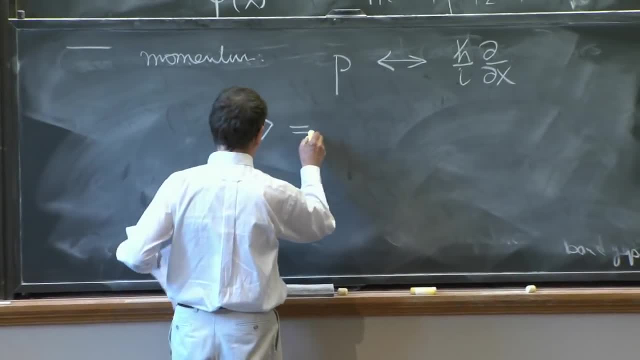 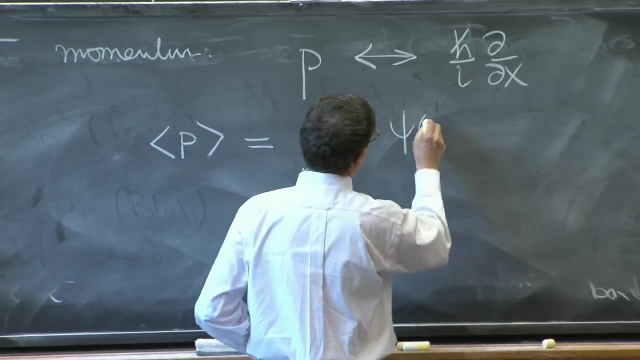 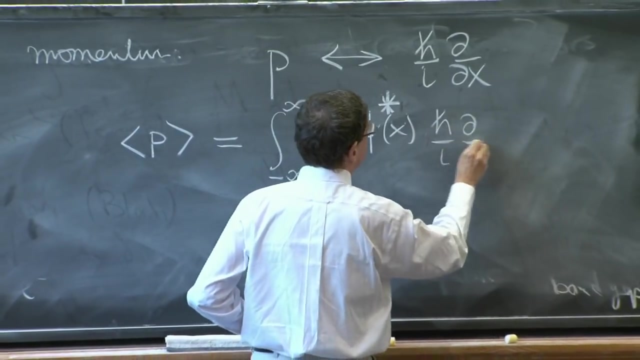 of the momentum of a particle. we compute the following quantity: We compute the integral from minus infinity to infinity dx. We put the conjugate of the wave function here And we put the operator h bar over i d dx. acting on the wave function here. 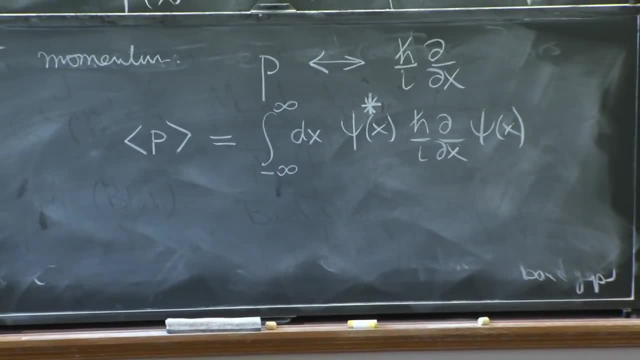 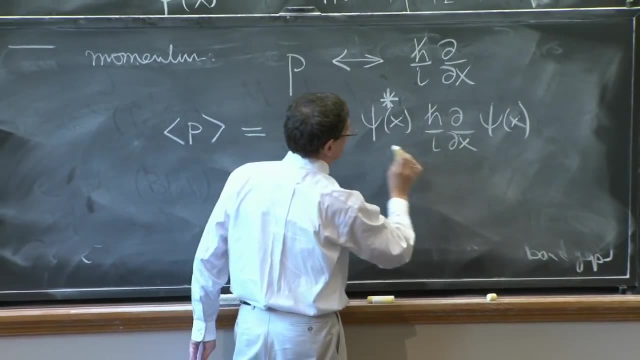 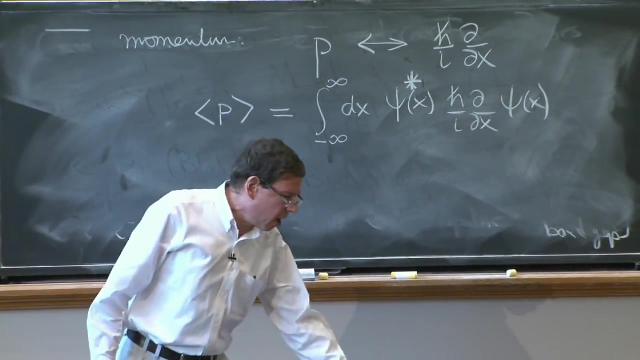 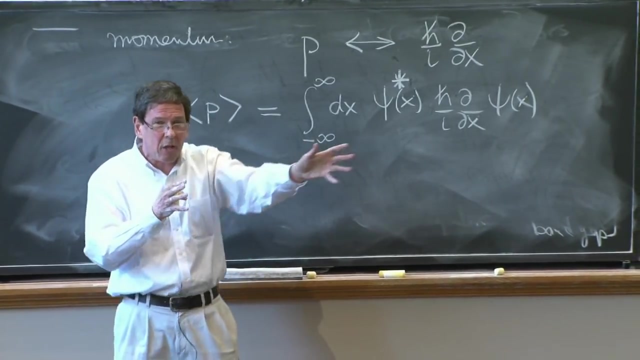 OK, OK, OK. And that's supposed to be sort of like saying that this evaluates the momentum of the wave function. Why is that so? It is because if you try to say, oh, any wave function, a general wave function need not. 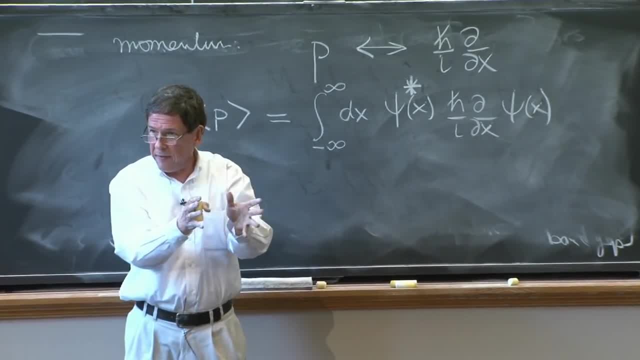 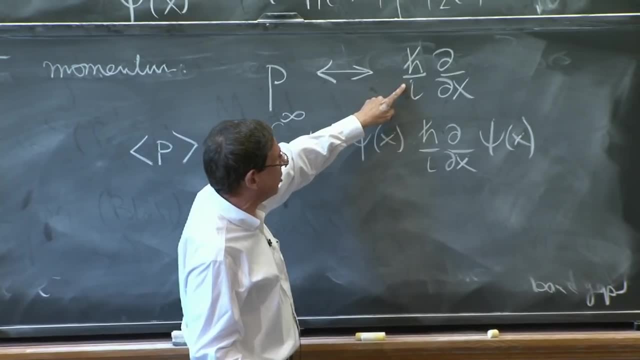 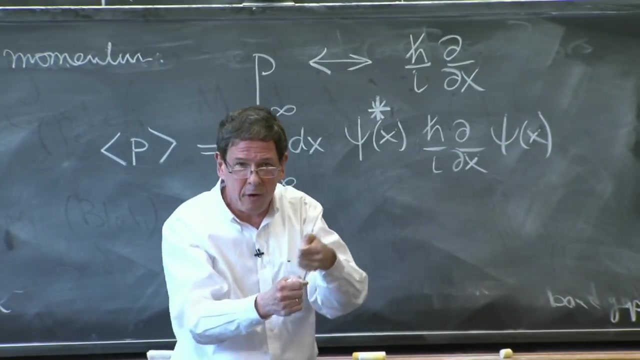 be a state in which the particle has definite momentum. So I can't, I cannot just say the momentum of a particle is the value of this operator on the function, Because if I act with this operator on the function on the wave function, it might not return me the wave function. 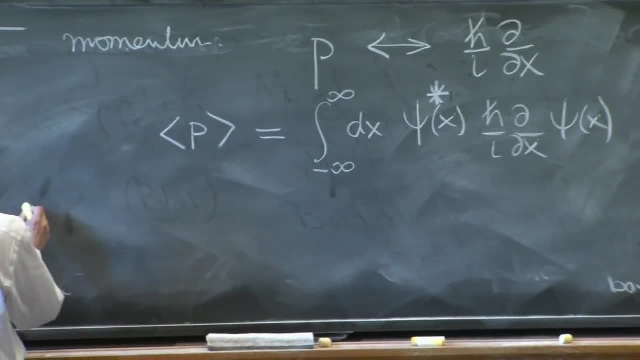 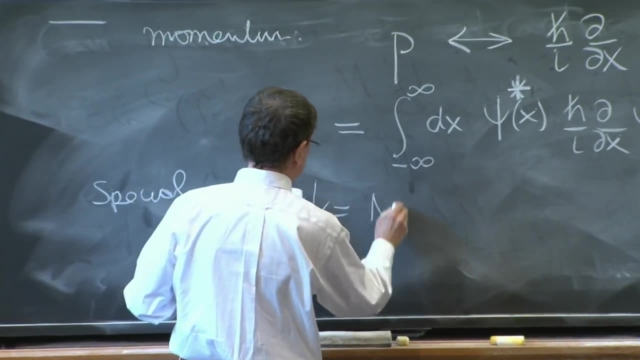 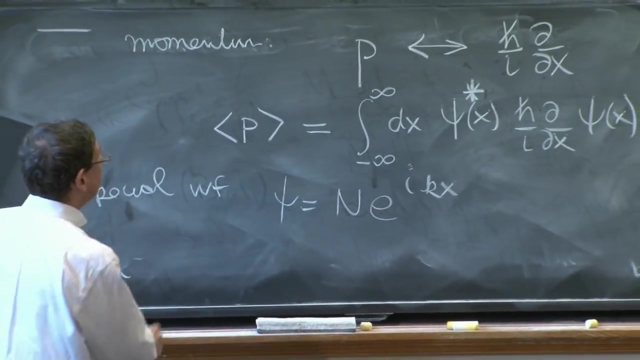 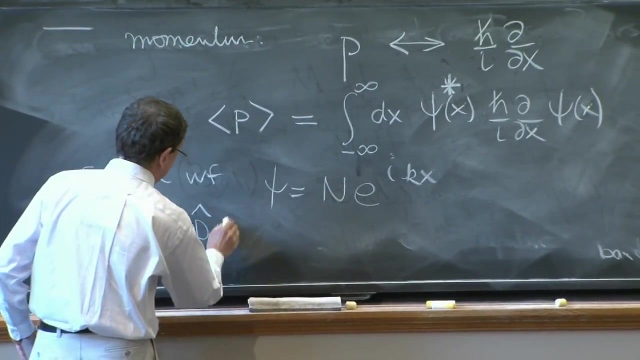 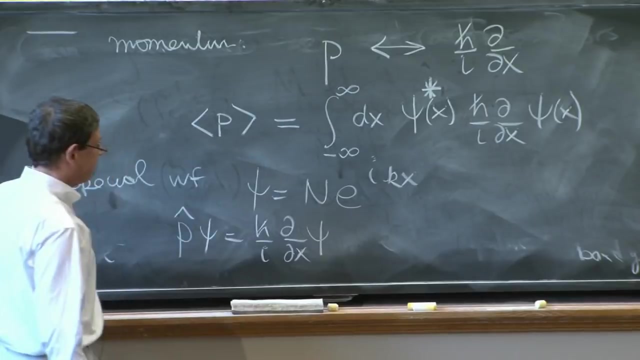 In fact, in general, we've seen that for special wave functions, wave functions of the form psi, a number e to the ikx, Then p, let's think p hat, as the operator on psi would be h, bar over i d dx on psi gives you what. 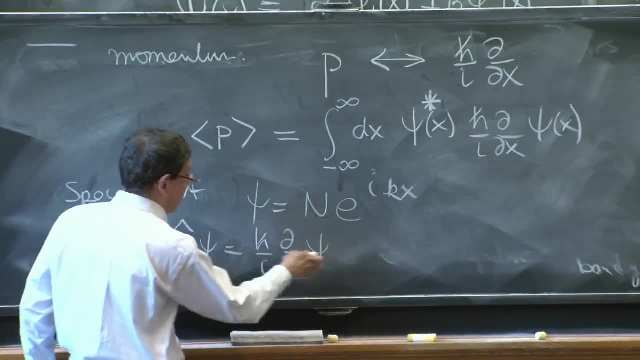 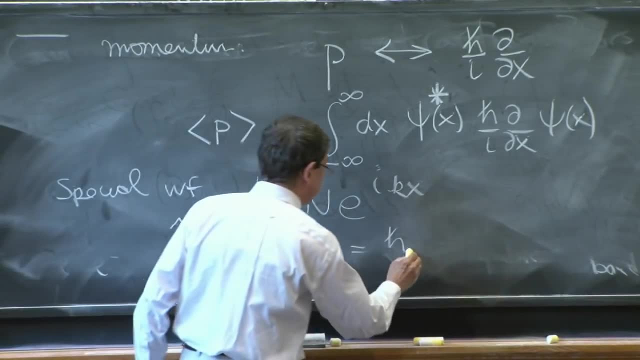 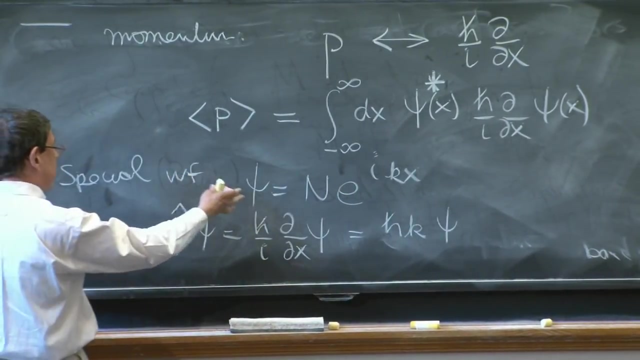 Well, this h over i. the h remains there. When you differentiate with respect to x, the ik goes down and the i cancels, So you get hk times the same wave function, And for this we think that this wave function is a wave. 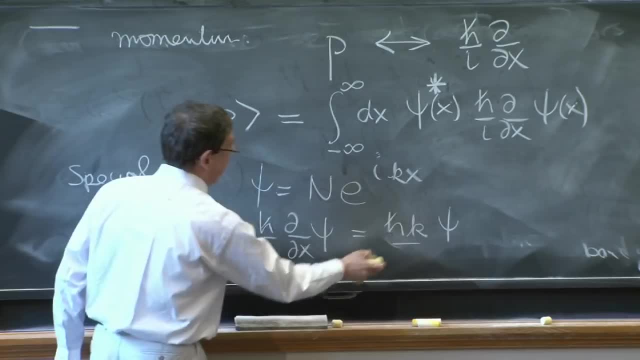 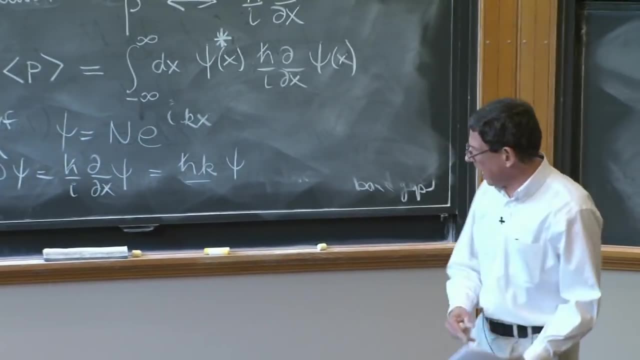 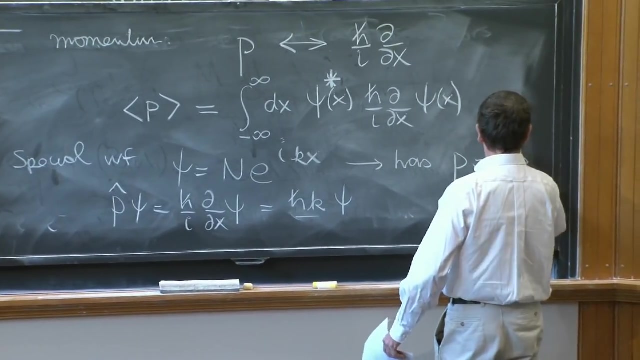 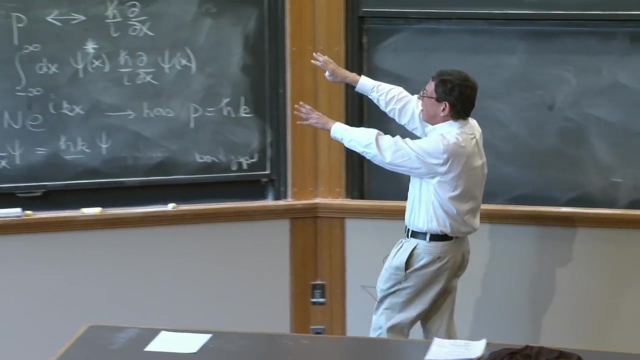 function with momentum hk, Because if you act with the operator p on that wave function, it returns for you hk. So we think of this as has p equal hk, h bar k. So the thing that we want to do now is make this a little more general. 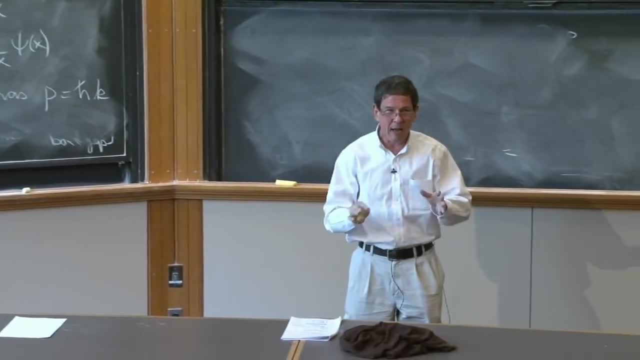 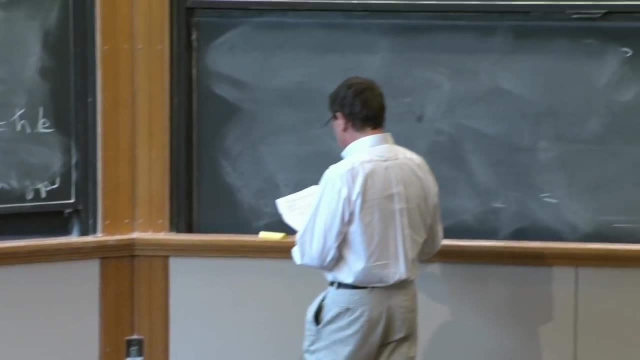 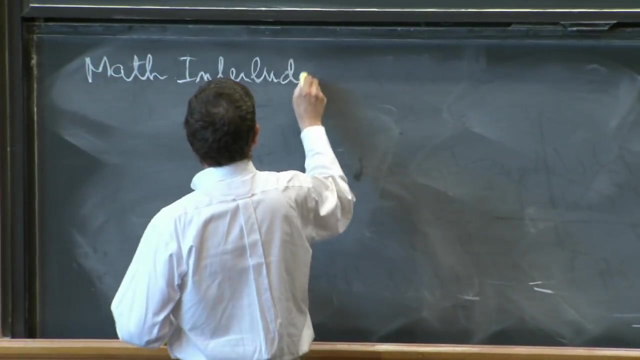 This is just talking about momentum, But in quantum mechanics we're going to have all kinds of operators, So we need to be more general. So this is going to be, as Alan calls it, a math interlude based on the following question: 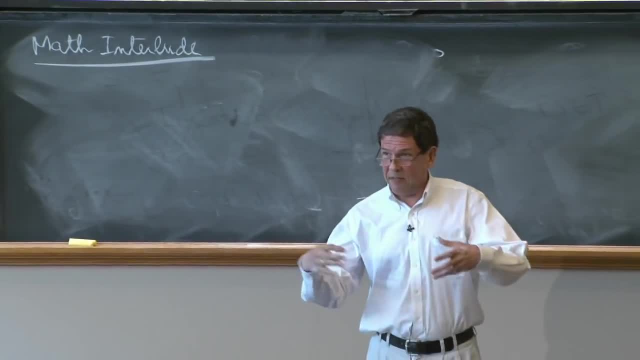 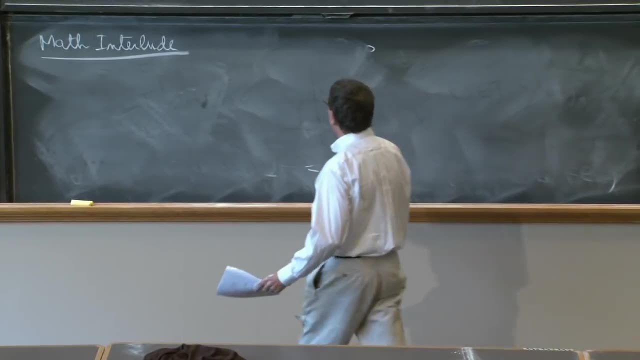 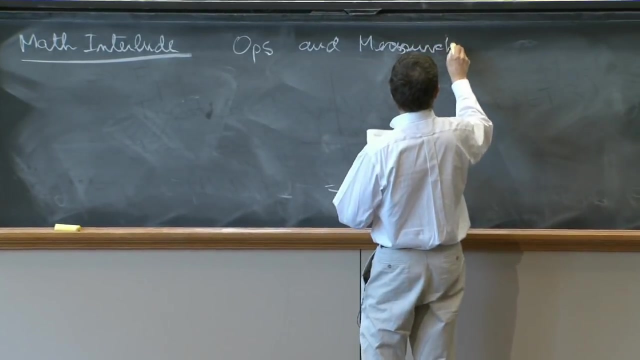 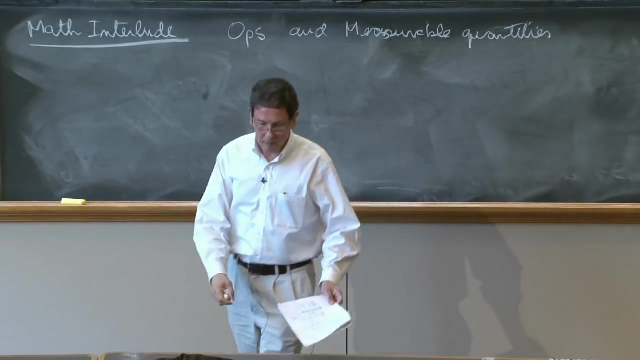 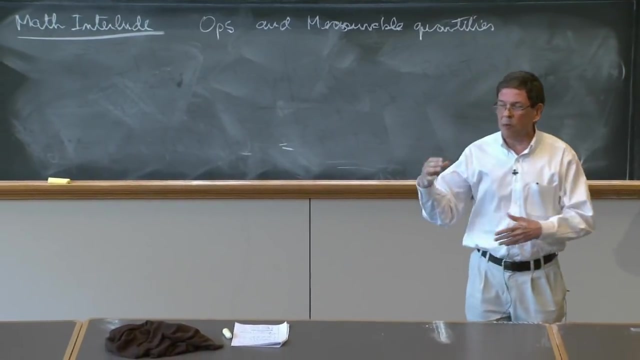 What is an operator? And then the physics question: What do measurable things have to do with operators? So about operators and measurable things, quantities. Now, your view of operators is going to evolve. It's going to evolve, Of course, it's going to evolve in 8.05.. 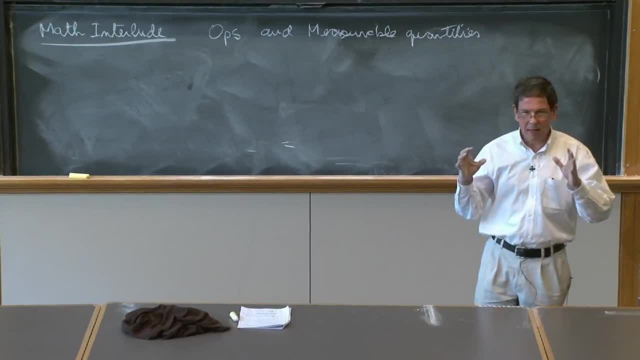 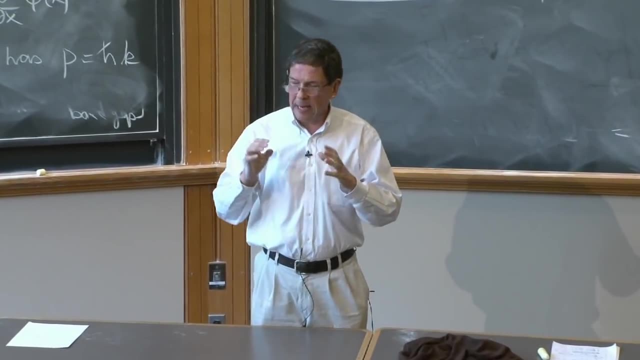 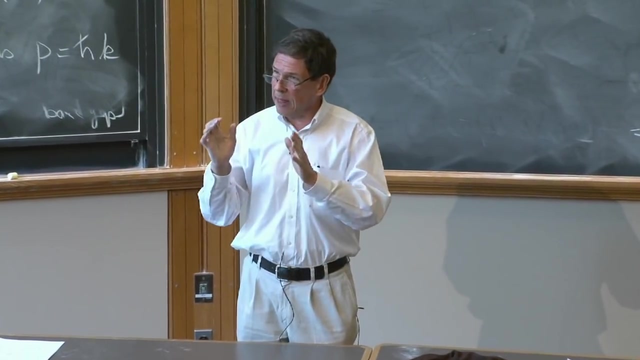 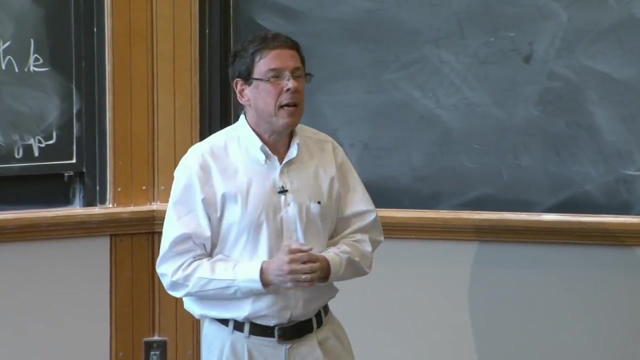 It probably will continue to evolve. So we need to think of what operators are, And there is a simple way of thinking of operators that is going to be the basis of much of the intuition. It's a mathematical way of thinking of operators And we will sometimes use it as a crutch. 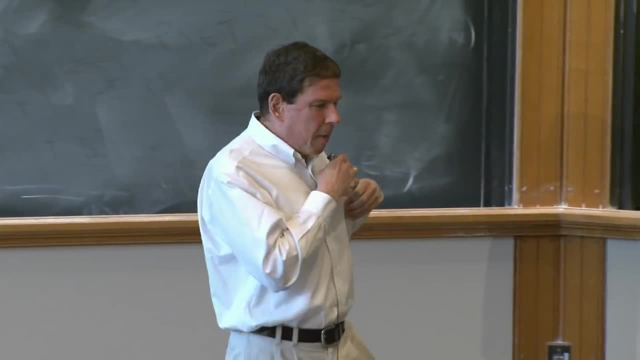 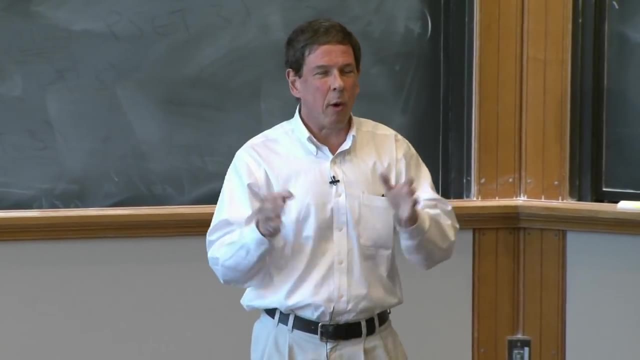 And the idea is that, basically, we're going to be able to do a lot of things, but we're not going to be able to do much of it. So operators are things that act on objects and scramble them. So whenever you have an operator, 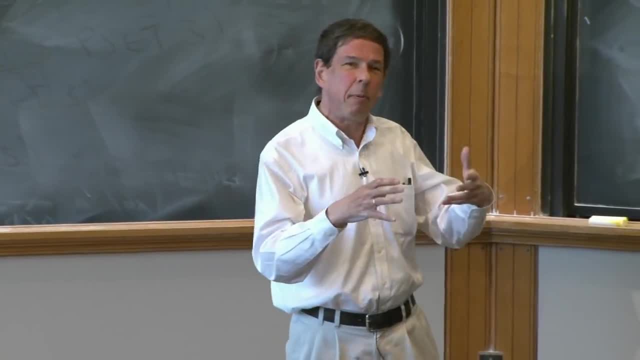 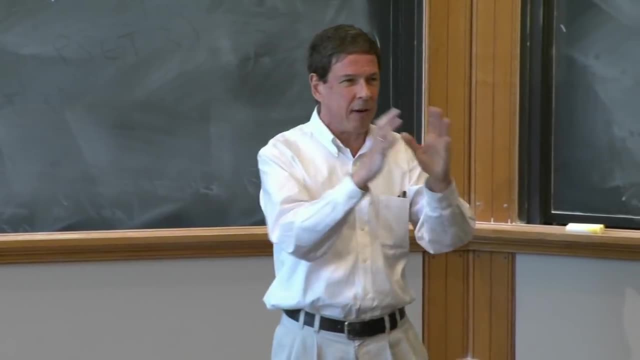 you really have to figure out what are the objects you're talking about. And then the operator is some instruction on how to scramble it, scramble this object. So, for example, you have an operator, You must say what it does to any object here. 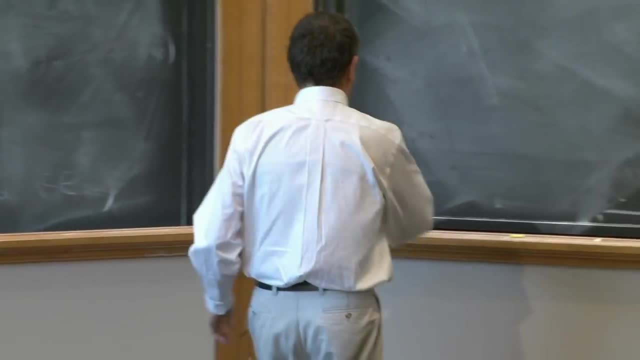 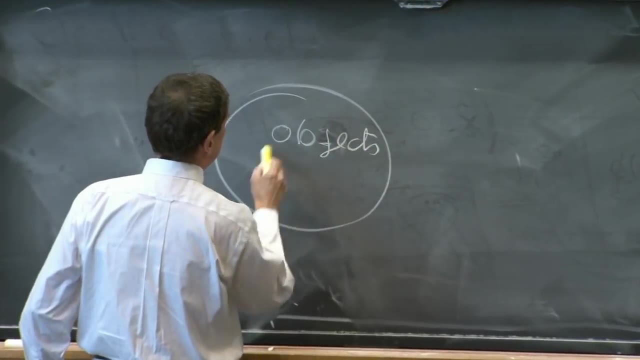 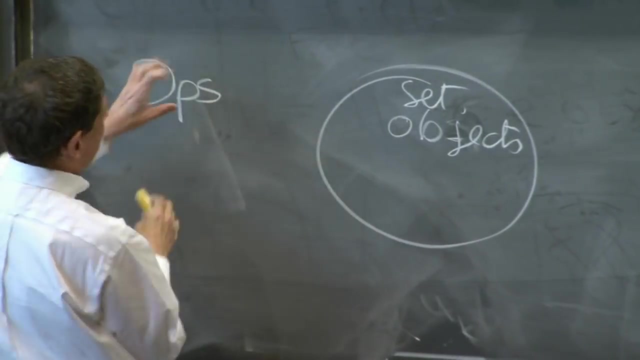 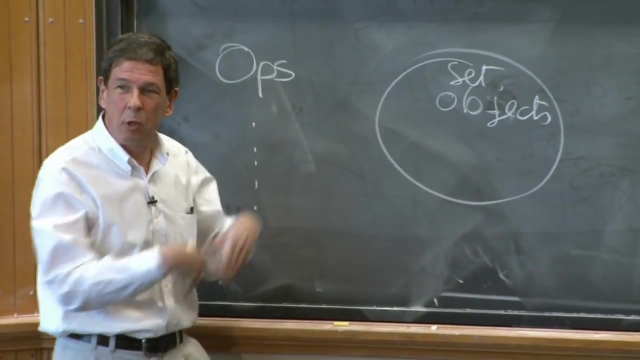 And it gives you another object. So in a picture you have all kinds of objects, sets, a set of objects And the operators are things. You can have a list of operators And they come here and move those objects, scramble them. 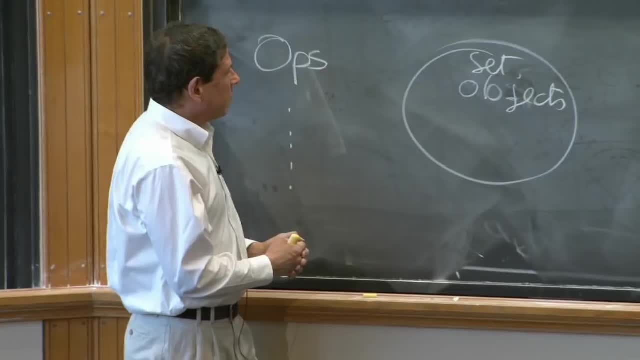 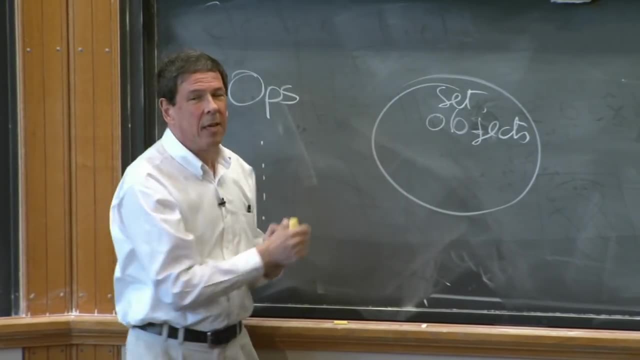 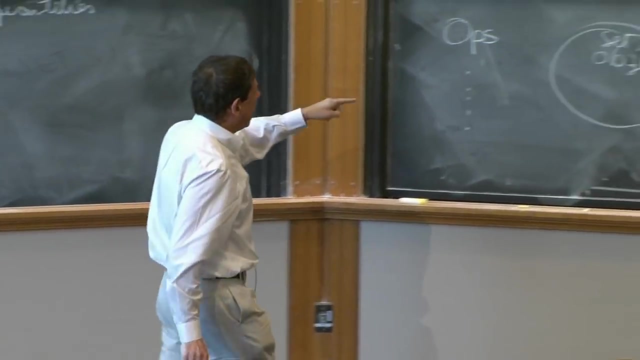 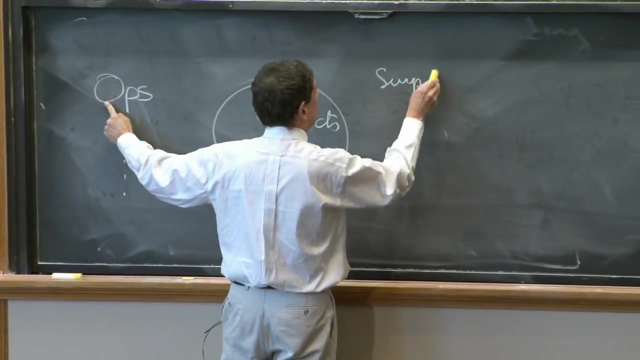 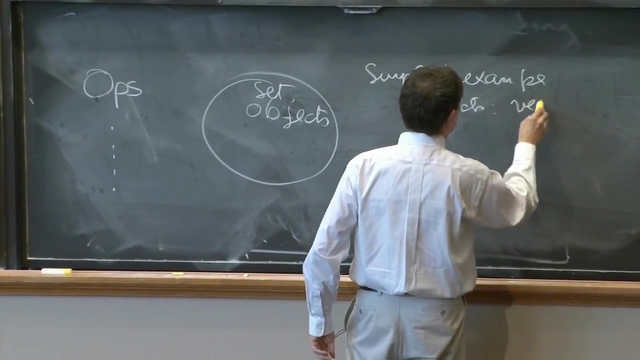 do something to them And we should distinguish them, Because the objects are not operators And the operators are not objects. So what is the simplest example in mathematics of this thing? It's vectors and matrices. Simplest example: objects are vectors. 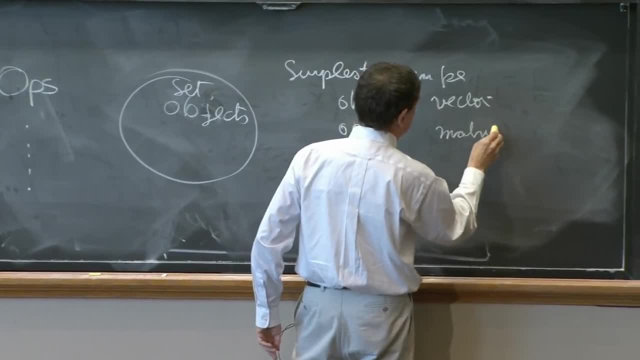 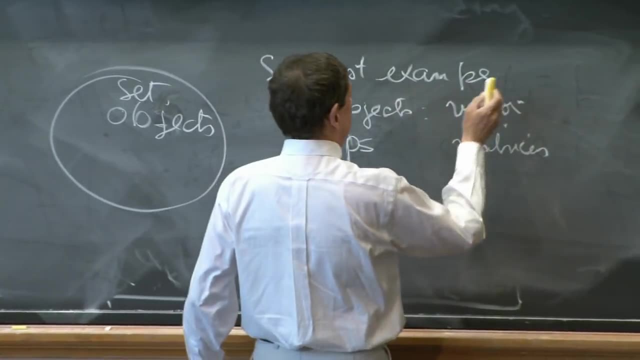 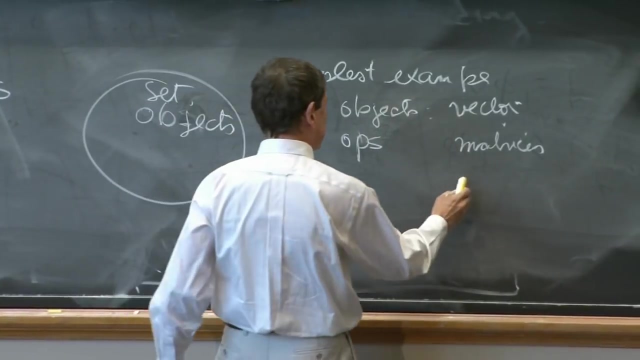 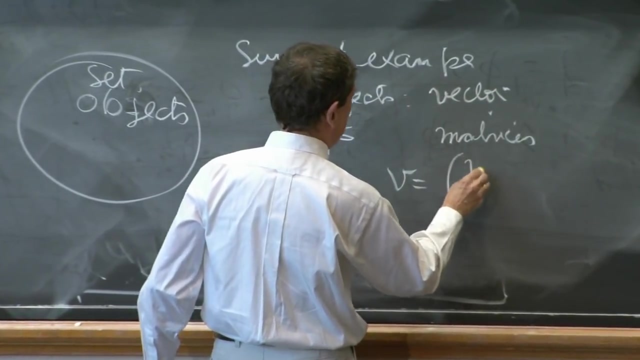 Operators are matrices. And how does that work? Well, you have a 2 by 2, the case where you have a set in which you have vectors with two components. So example: a vector that has two components, v1 and v2.. 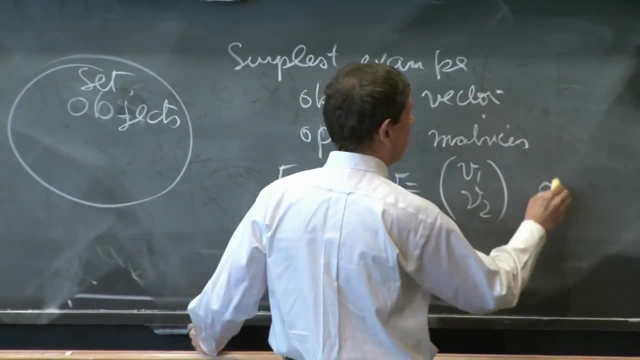 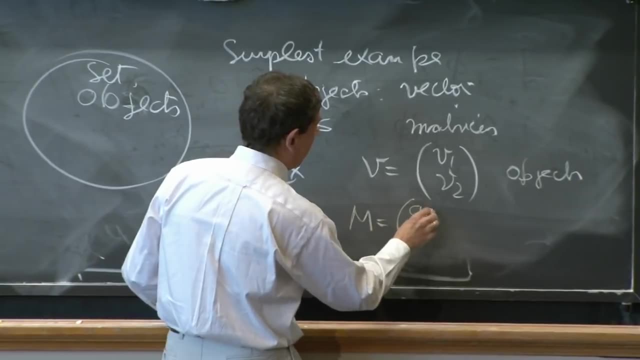 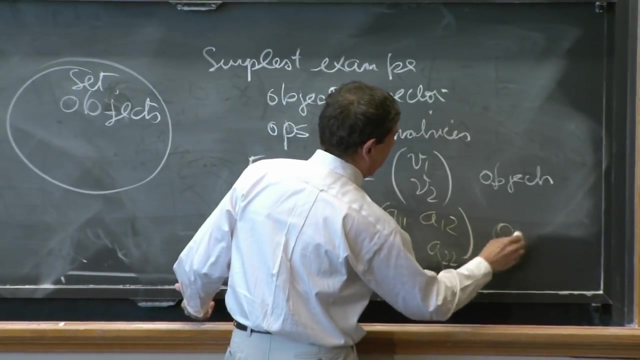 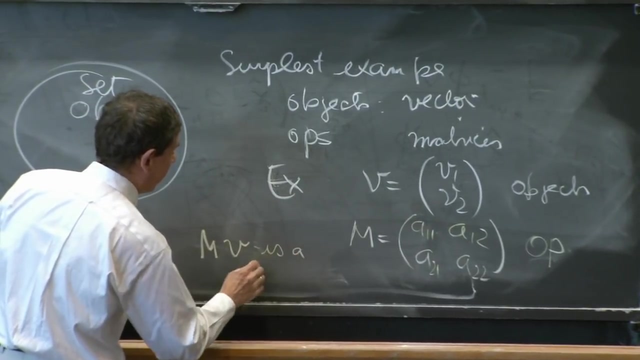 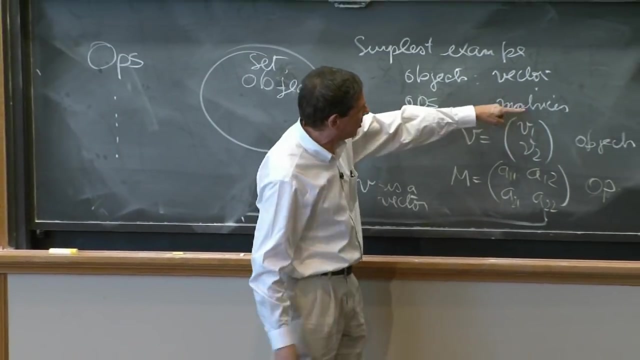 And the matrices. this is the object and the operators. a matrix a11, a12,, a21, a22, as an operator, And m on a vector is a vector. If you add with a matrix on a vector, this 2 by 2 matrix. 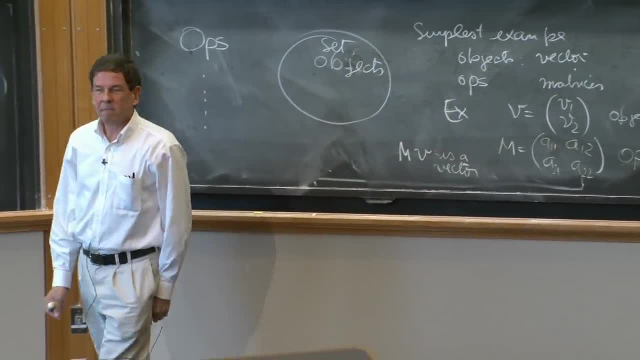 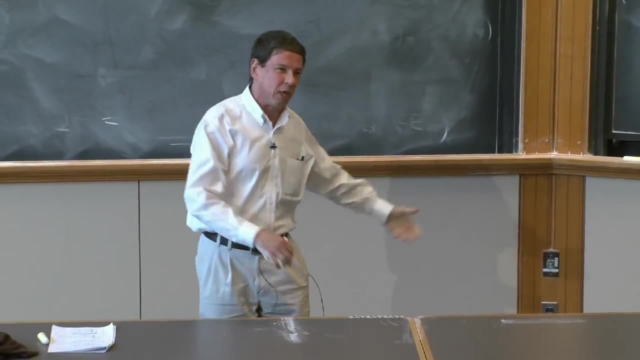 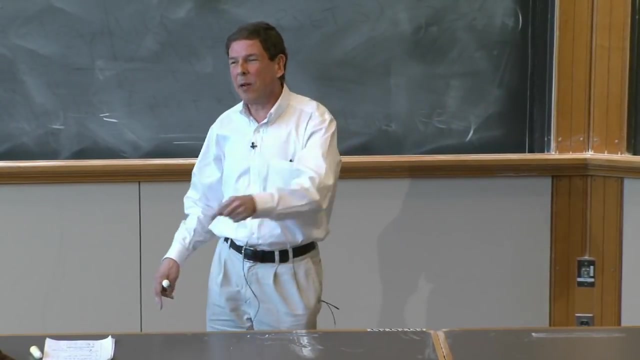 on this column vector, you get another vector. OK, OK, OK. So that's the simplest example of operators acting on objects. In our case, we're going to talk about a more. we're going to have to begin in quantum mechanics. 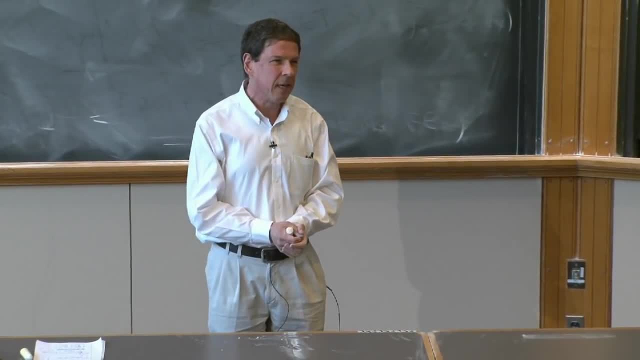 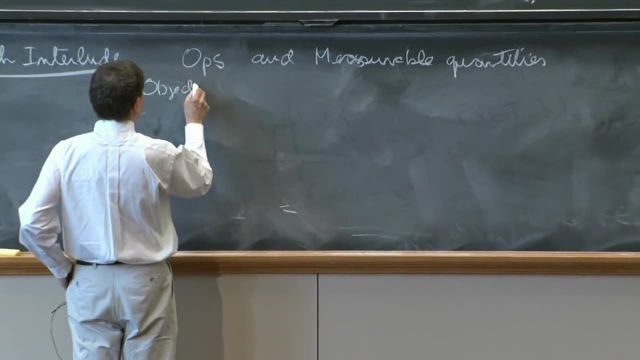 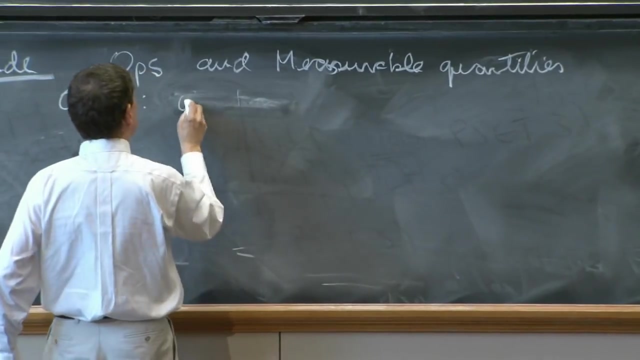 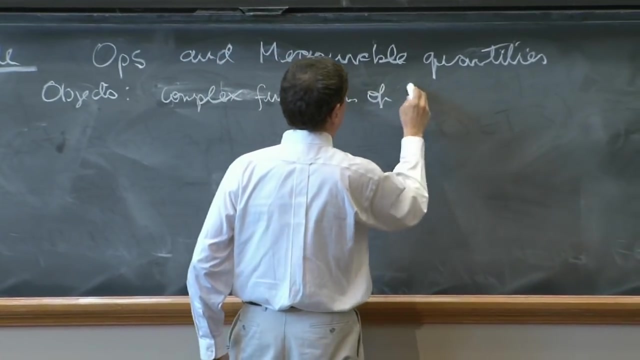 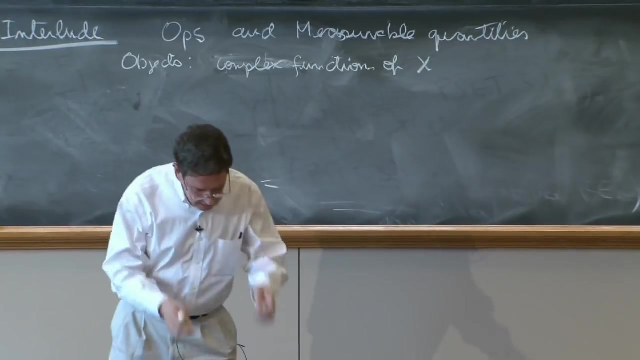 we're required to begin with a more sophisticated one, in which the objects are going to be objects are going to be functions. In fact, I will write complex functions of x. So let's see at the list of operators. And what do the operators do? 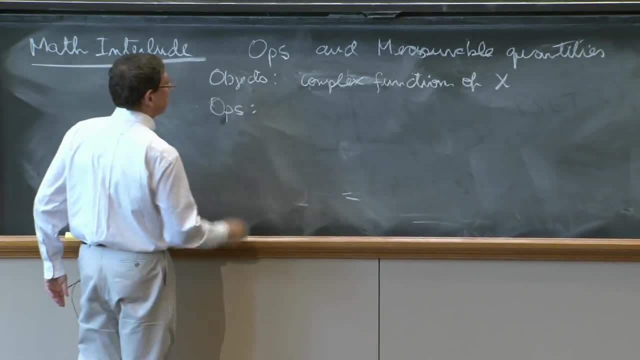 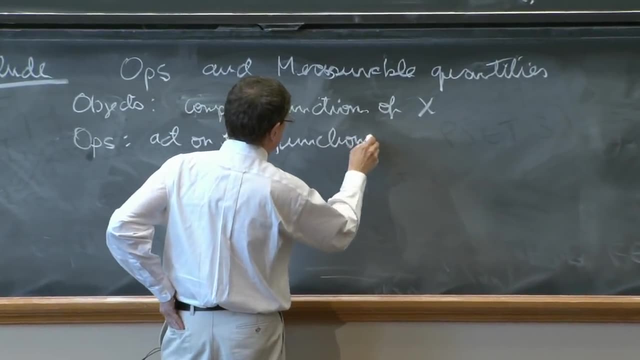 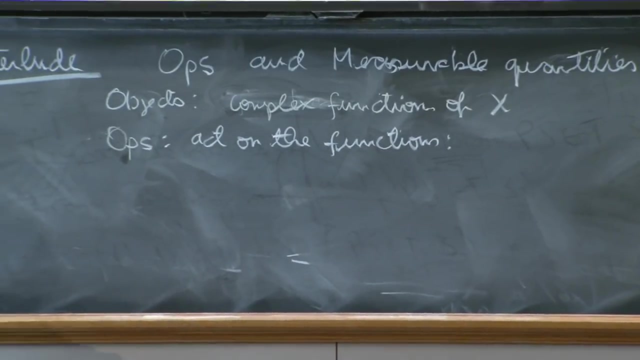 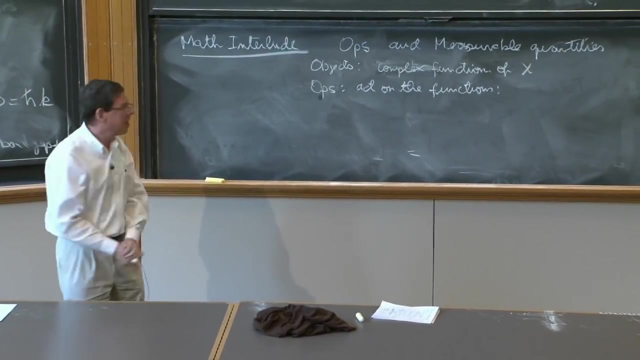 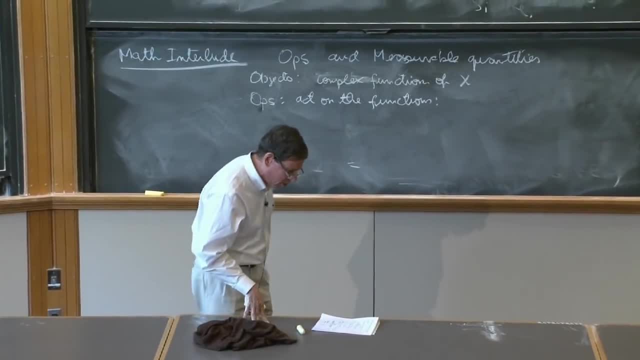 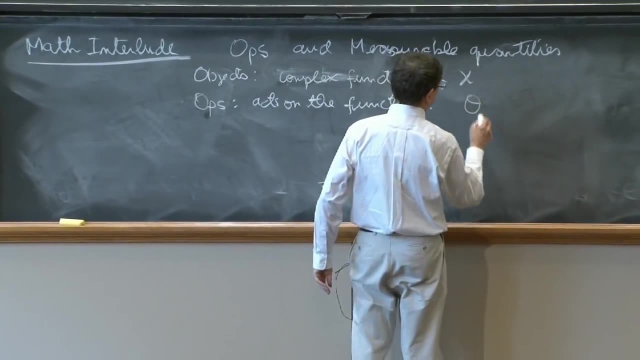 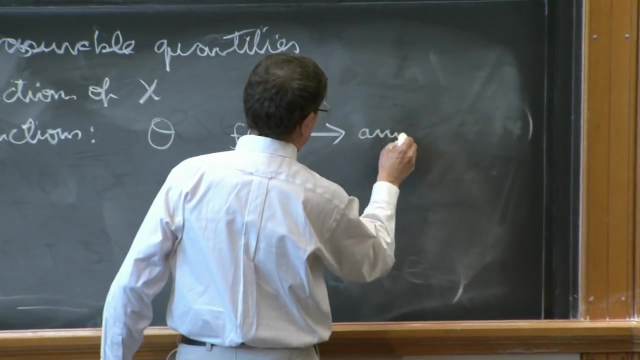 It's a rule on how to take any function, and you must give a rule on how to obtain from that function another function. So let's start with examples. It's probably the easiest thing to do. We'll give you another function of x. 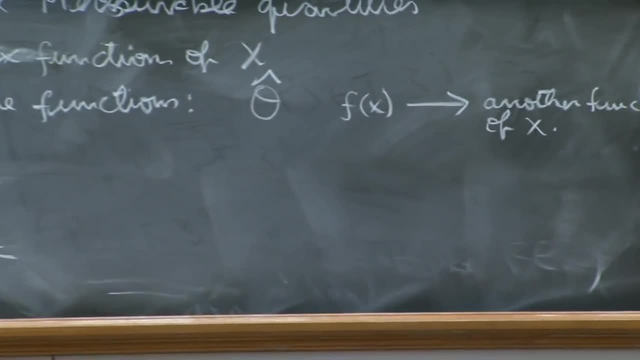 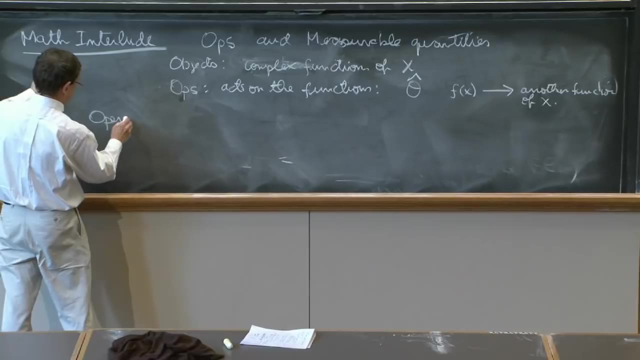 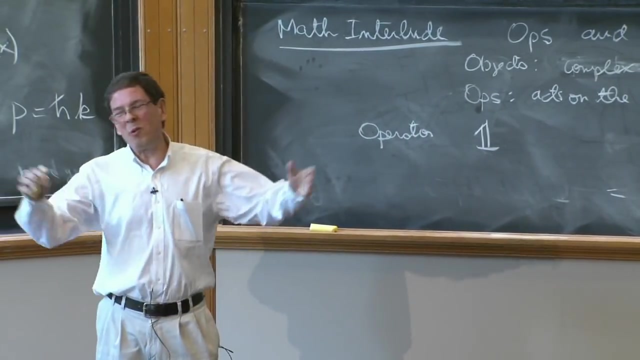 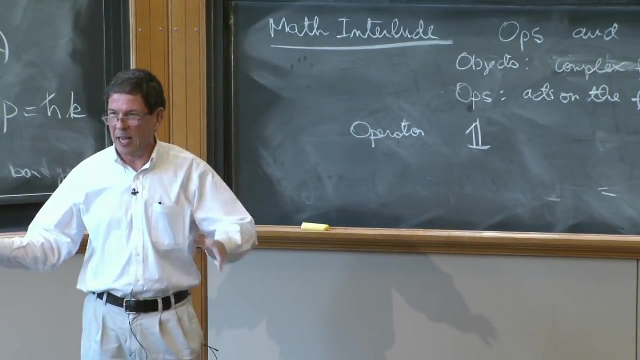 And here's operator O. We put the hat sometimes for operators, So the simplest operator, operator 1.. We, always mathematicians, love to begin with trivial examples. Some examples don't illustrate anything almost and just can confuse you many times. 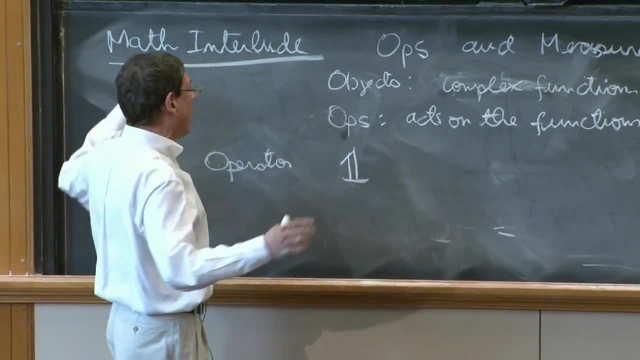 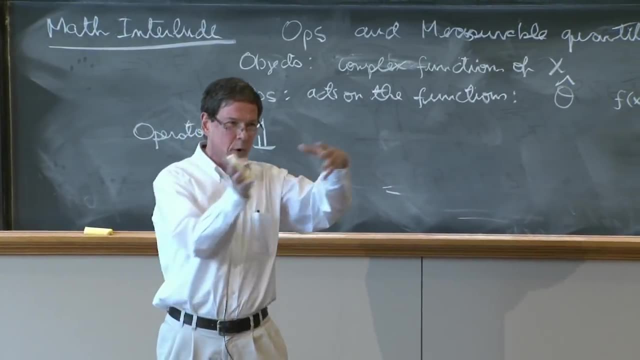 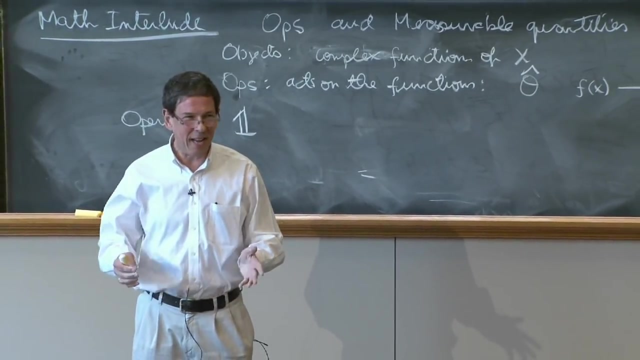 But actually it's good to get them out of the way. So what is the operator 1?? One possibility: It takes any function and gives you the number 1.. Do you think that's it? Who thinks that's it? Nobody. 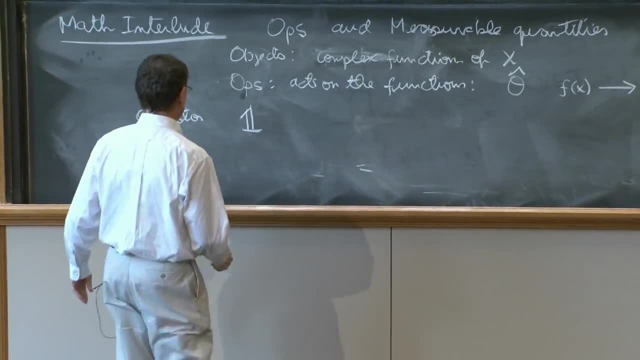 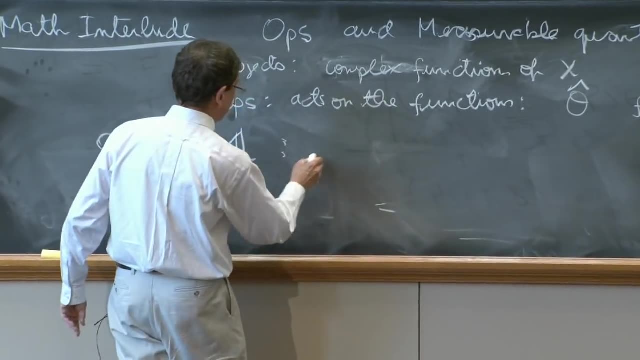 Very good. That definitely said It's not a good thing to do to give you the number 1.. So this operator does the following. I will write it like that: The operator 1 takes f of x and gives you what? 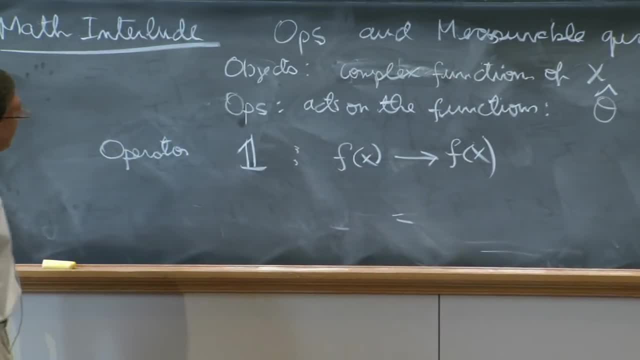 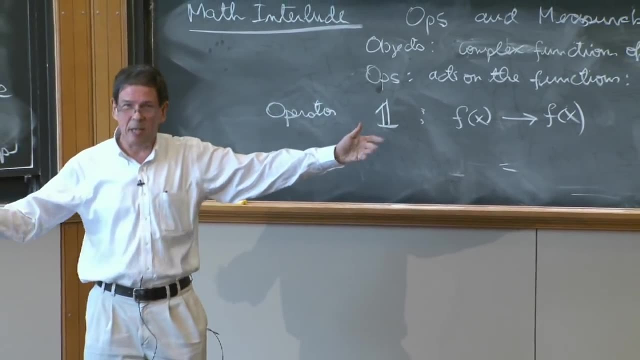 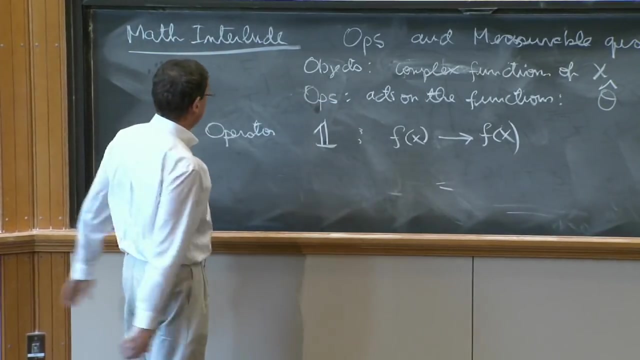 f of x, Correct, Good. So it's a very simple operator, but it's an operator. It's like: what matrix? The identity matrix? Very good, There could be a 0 operator, That gives you nothing and it would be the 0 matrix. 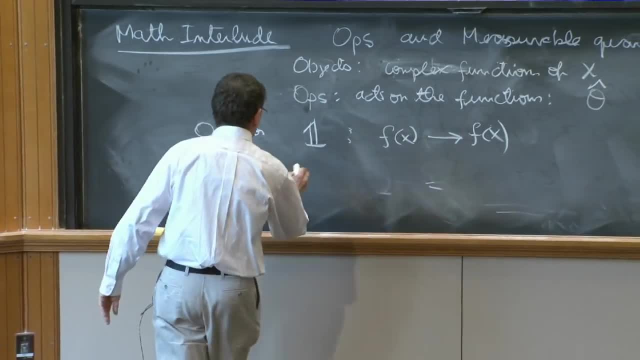 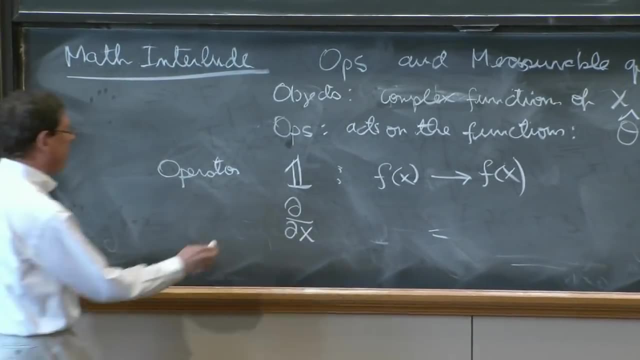 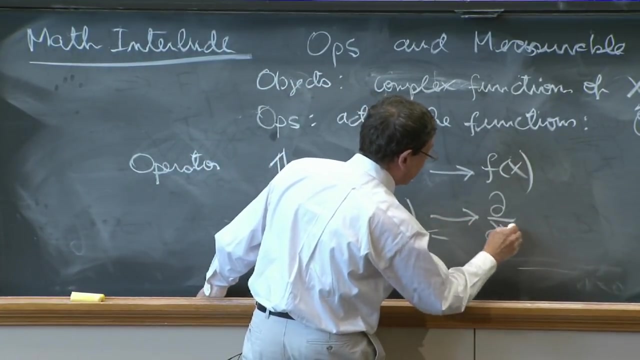 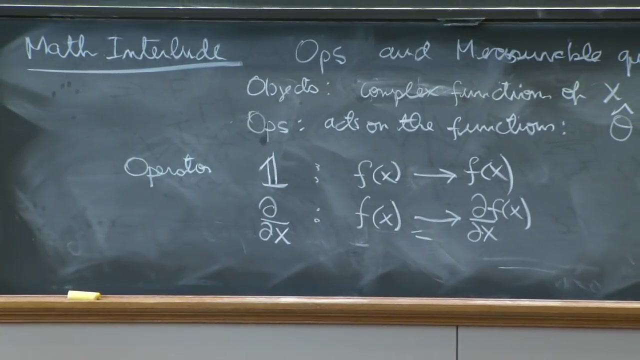 So let's write the more interesting operator, The operator ddx. That's interesting. The derivative can be thought of as an operator, because if you start with f of x, it gives you another function, ddx of f of x, And that's a rule to get from one function to another. 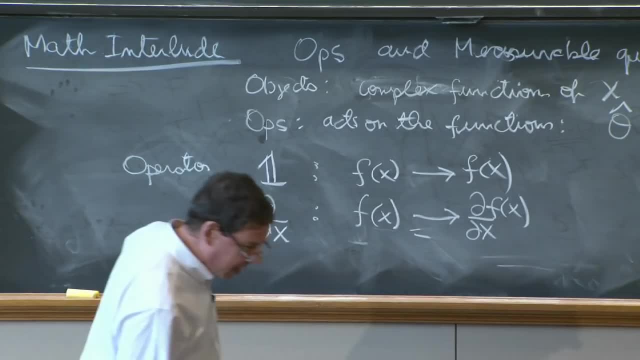 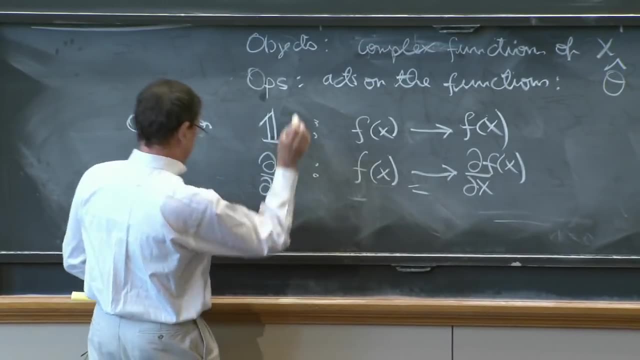 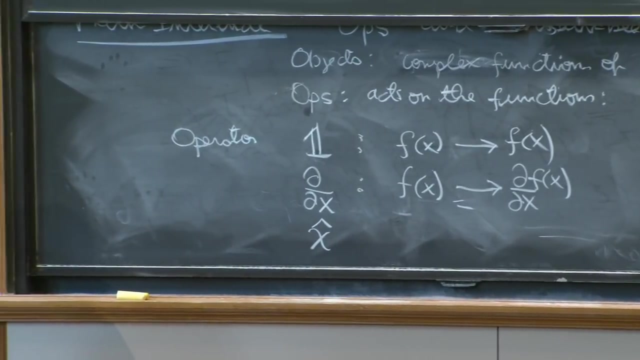 Therefore, that's an operator. It qualifies as an operator. Another operator that typically can confuse you is the operator x x an operator. What does that mean? Well, you just have to define it. At this moment, it could mean many things. 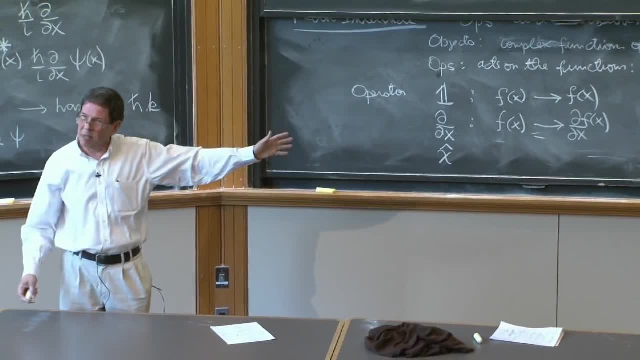 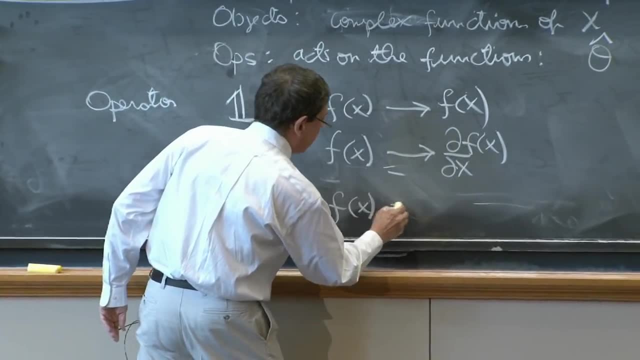 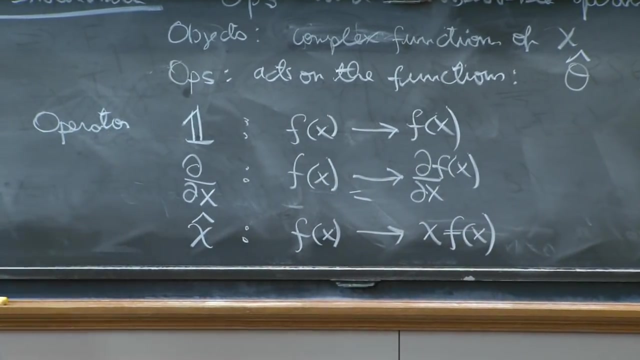 But you will see that what I'll write is the only thing that probably makes some sense. So what is the operator x? Well, it's the operator that, given f of x, gives you the function x times f of x. That's a reasonable thing to do. 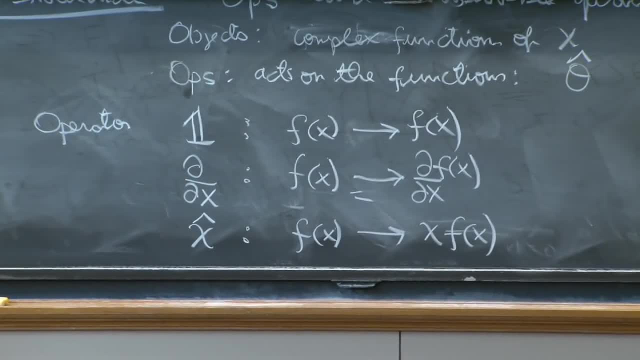 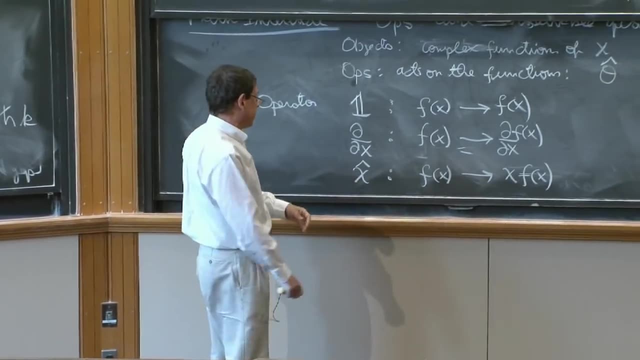 It's multiplying by x. It changes the function. You could define the operator x squared that multiplies by x squared, And the only reasonable thing is to multiply it by. You could divide by it and you may need to divide by it as. 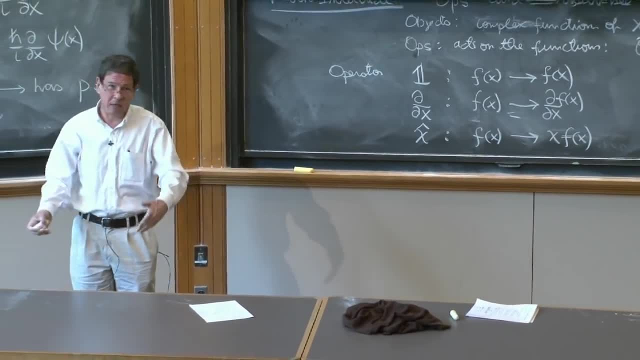 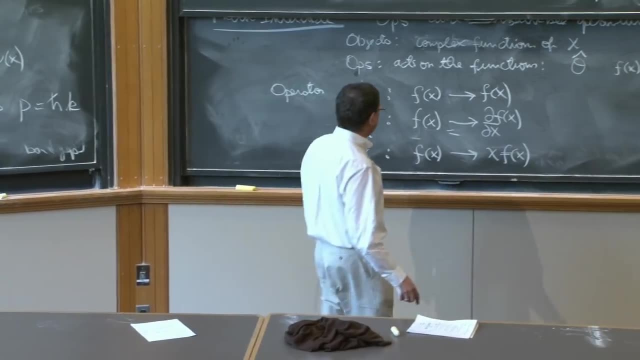 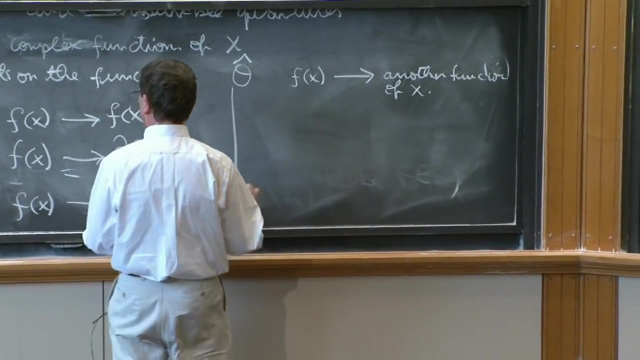 well, And you could define the operator 1 over x. That gives you the function times 1 over x And we will need that sometime, but not now. Let's see another set of operators where we give a name. It doesn't have a name because it's not all that useful. 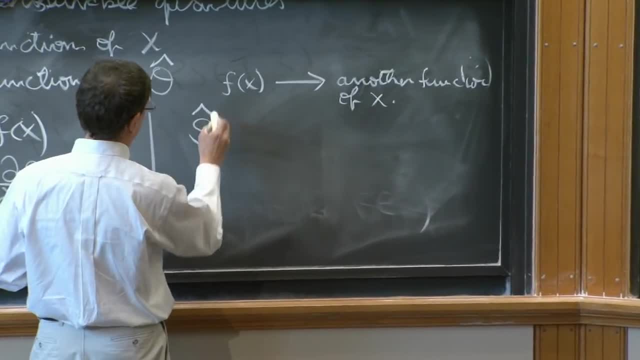 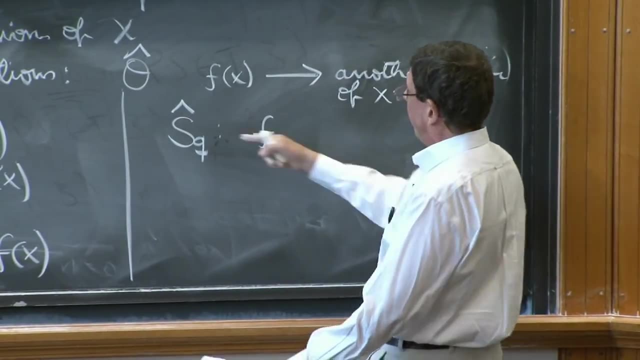 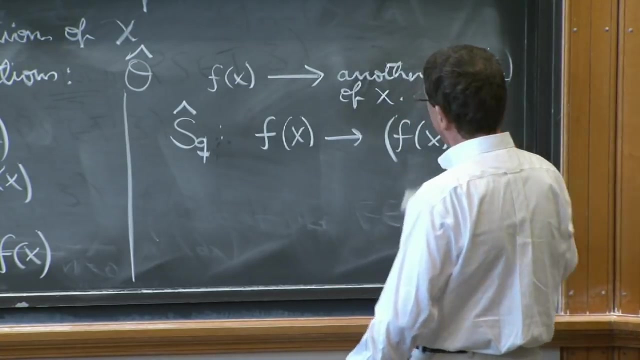 in fact, But it's good to illustrate things, The operator s sub q for square, sq for the first two letters of the word square. that takes f of x into f of x squared. That's another function. You could define more functions like that. 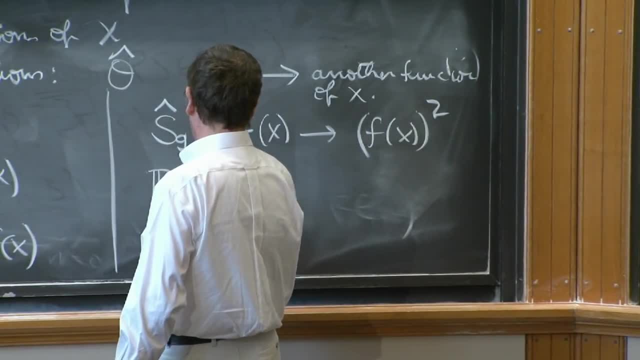 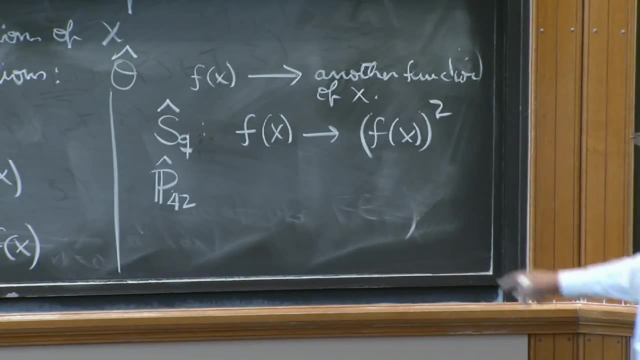 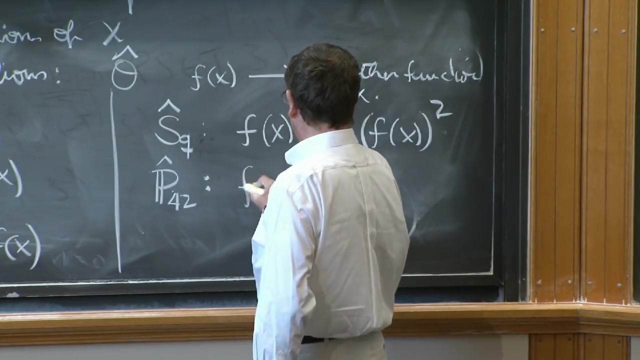 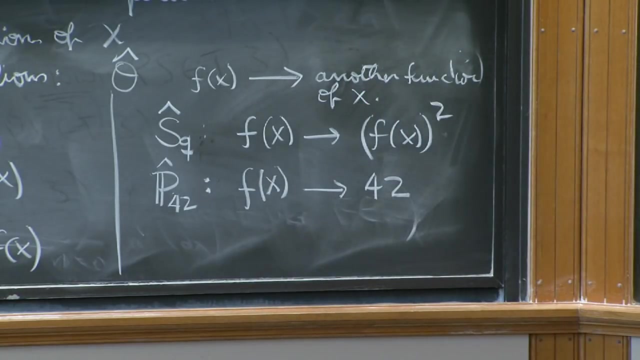 The operator p 42, that's another silly operator. Well, certainly a lot more silly than this one. That's not too bad. But the p 42 takes f of x and gives you the number 42 times the constant function. So that's a function of x. 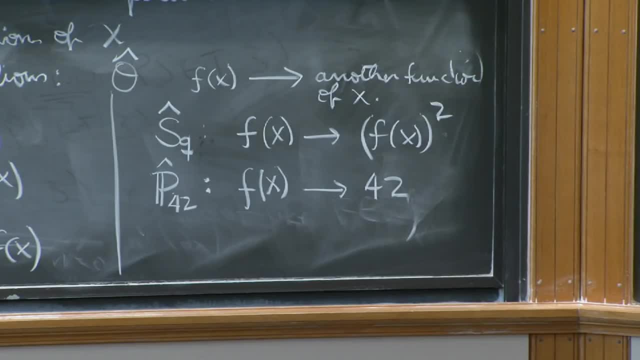 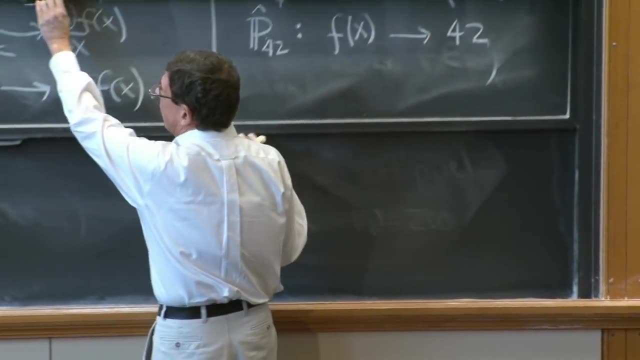 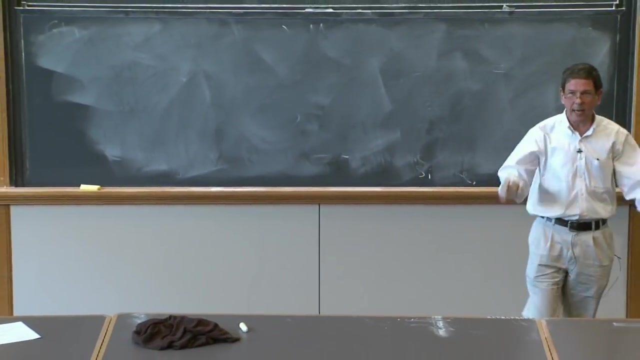 It's a trivial function of x. Enough examples. So you get the idea. Operators act on functions and give you functions And we just need to define them, and then we know what we're talking about. Yes, Is the Dirac delta an operator? 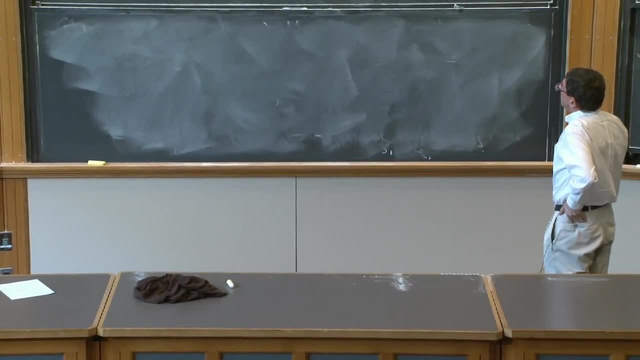 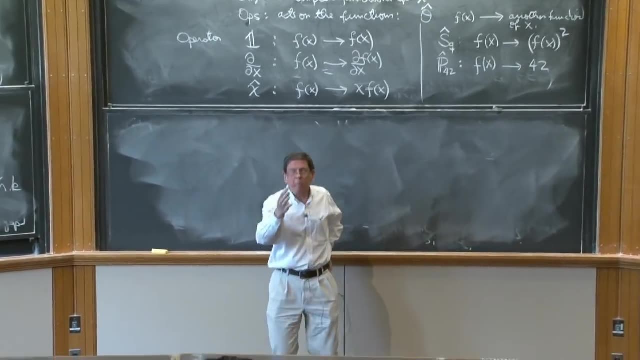 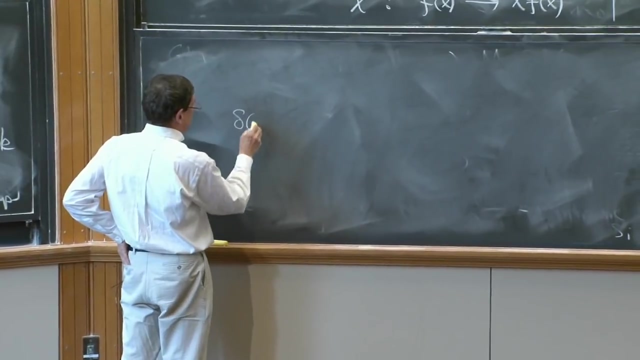 The Dirac delta. well, you can think of it as an operator. So it all depends how you define things. So how could I define the Dirac delta function to be an operator? So delta of x minus a. can I call it the operator delta? 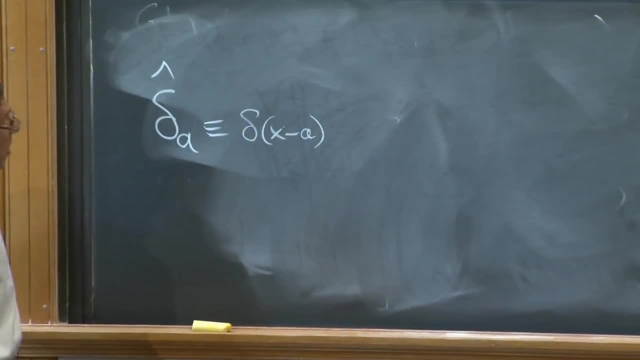 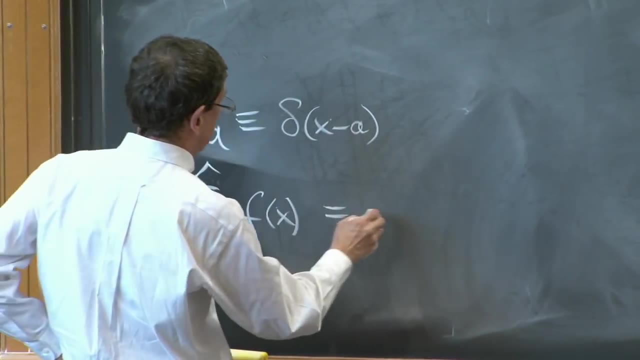 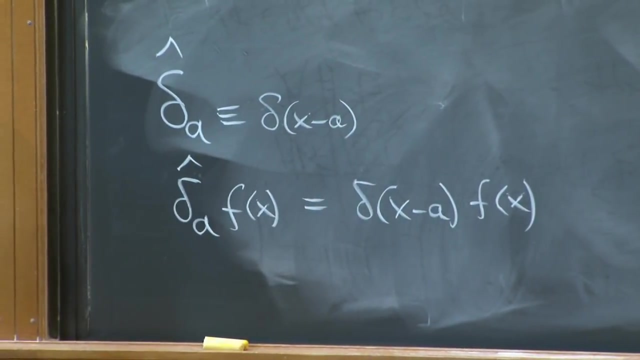 hat of a. Well, I would have to tell you what it does on functions, And probably I would say: delta hat on a on a function of x is equal to delta of x minus a. So delta of x minus a times the function of x. 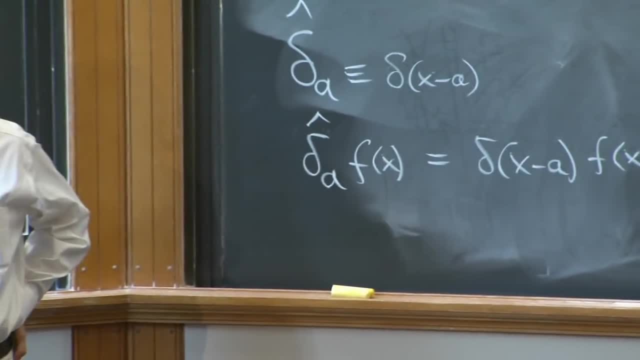 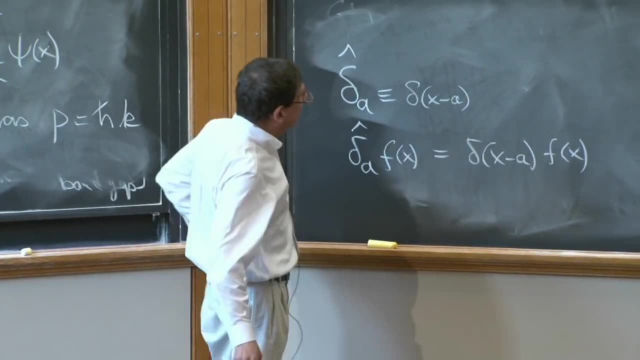 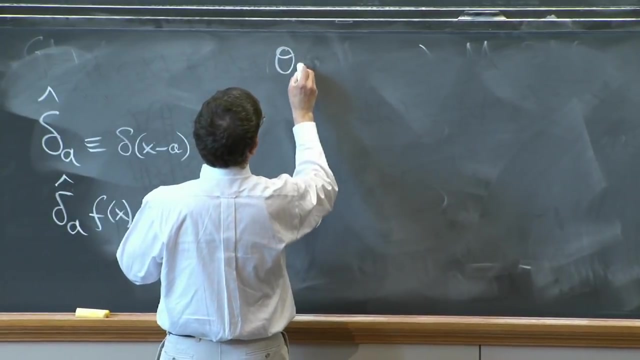 And that's it. It's an operator. Now the question is really: is it a useful operator? And sometimes it will be useful. in fact, This is a more general case of another operator, And maybe I could define O sub f the O sub h of x. 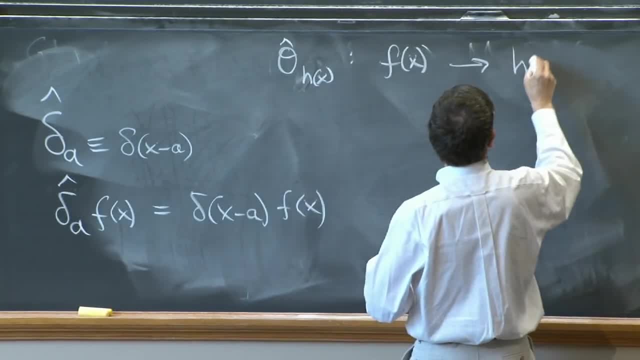 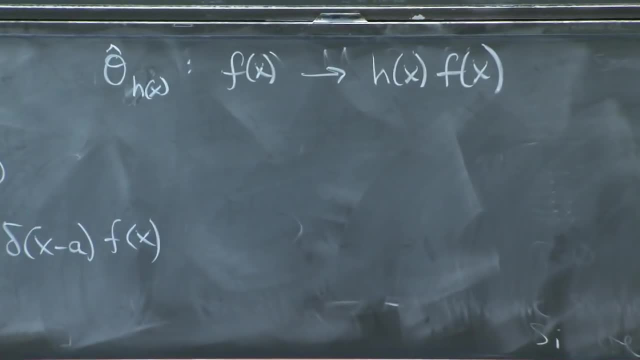 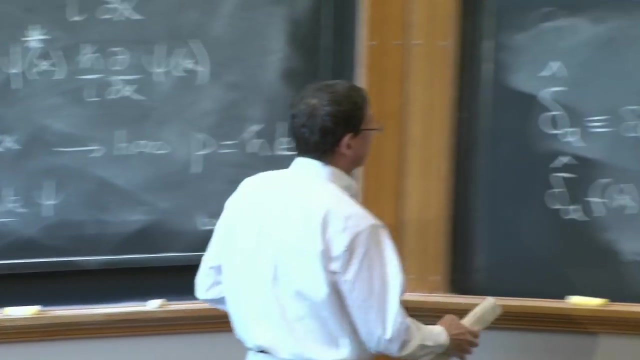 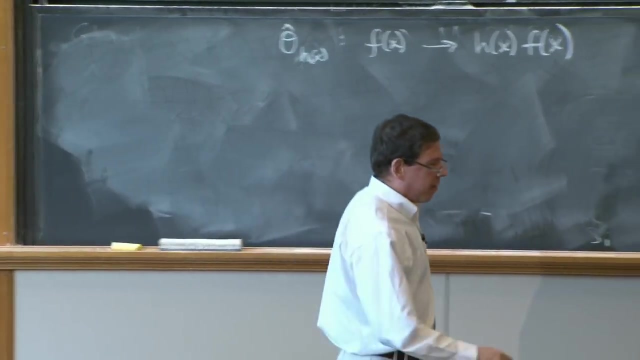 is the operator? It's the operator of x into h of x times f of x, So that would be another operator. Now, there are operators that are particularly nice And there are the so-called linear operators. So what is a linear operator? 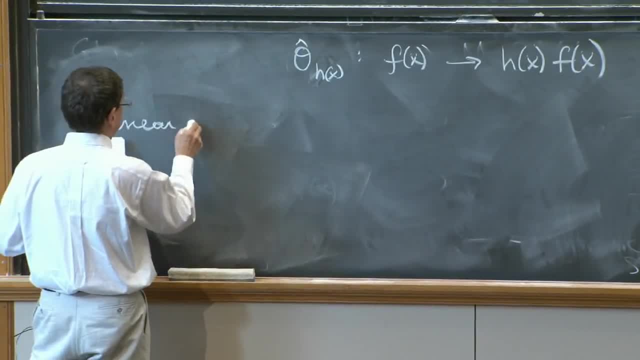 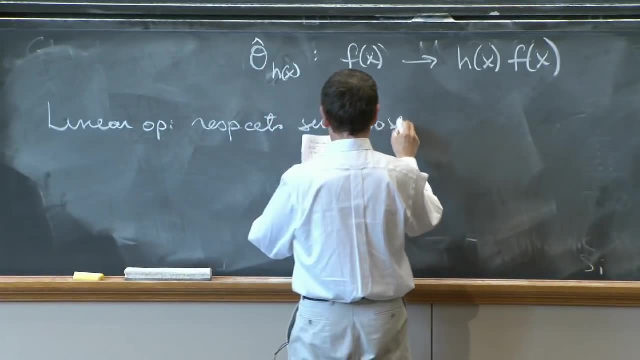 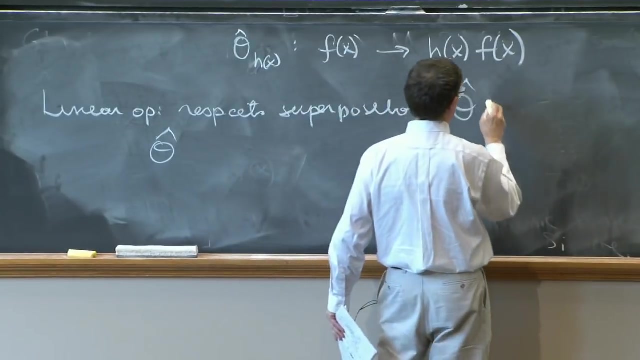 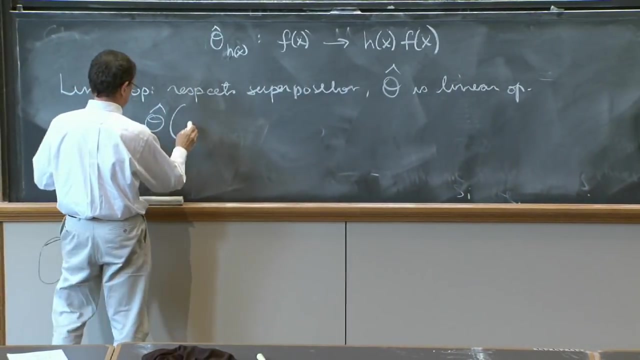 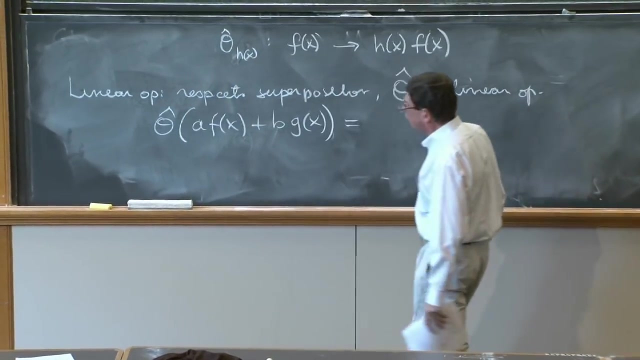 It's one that respects superposition. A linear operator respects superposition. So O hat is linear. O hat is linear. It's a linear operator. If O hat on a times f of x plus b times g of x, it can be an operator. because what? 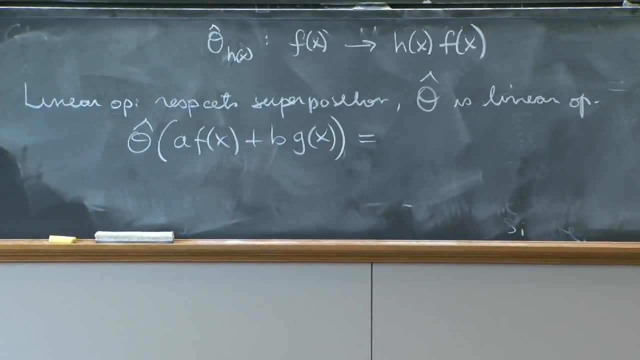 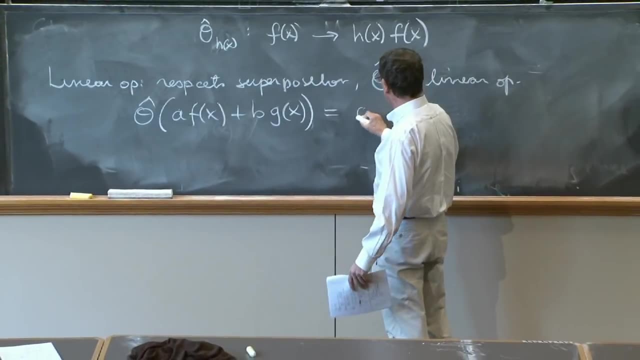 you would imagine it should do. it acts on the first and it acts on the second. Acting on the first, a number goes out and it doesn't do anything say on the number. It's linear. It's part of that idea. 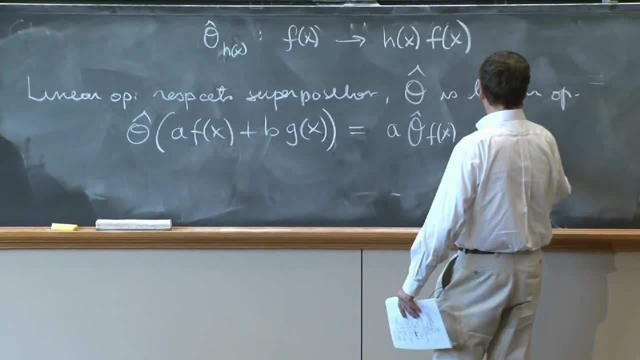 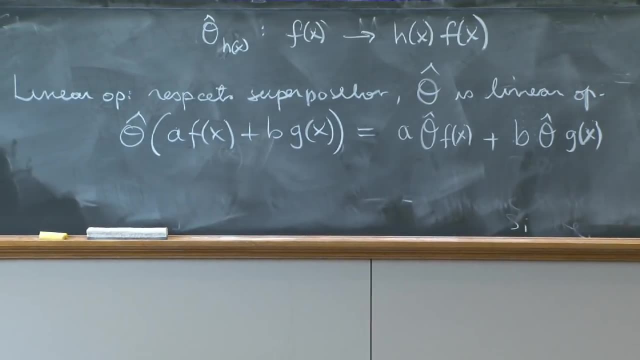 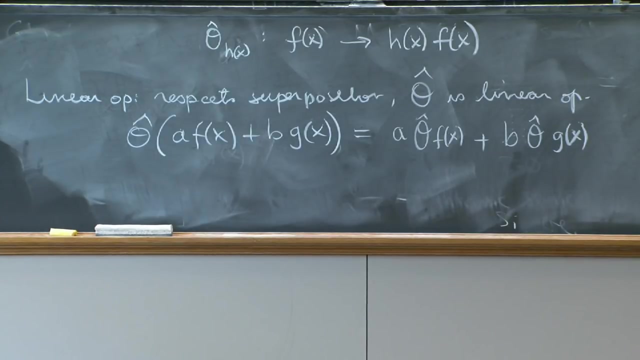 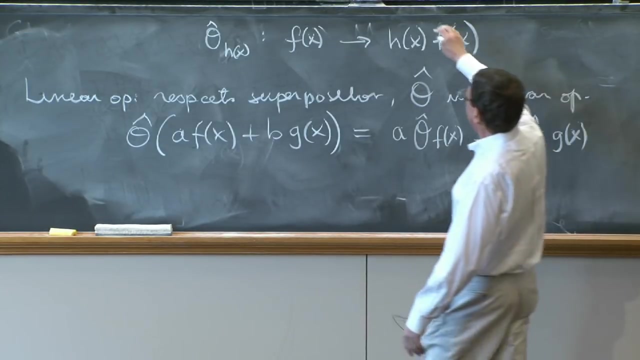 And it gives you O on f of x plus B times O on g of x. it's linear, It's part of that idea- linear or it may not be linear, And we have to just test them And you would imagine that we can decide that. 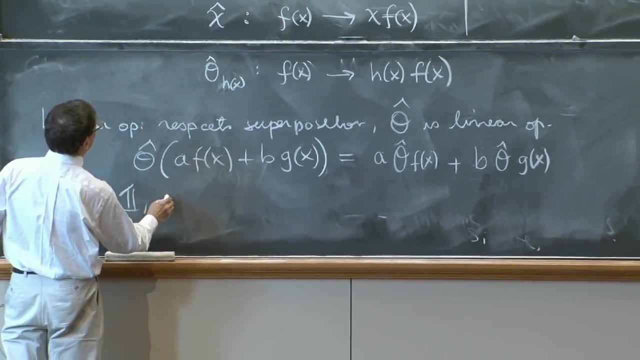 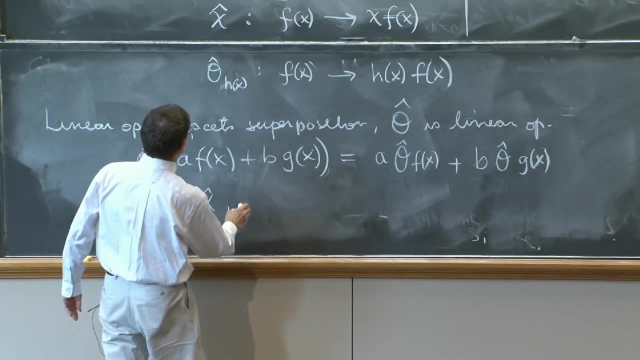 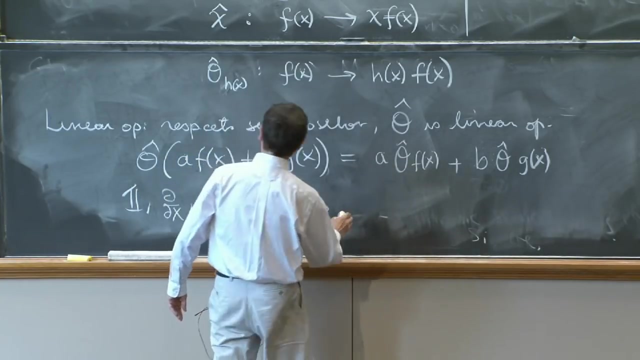 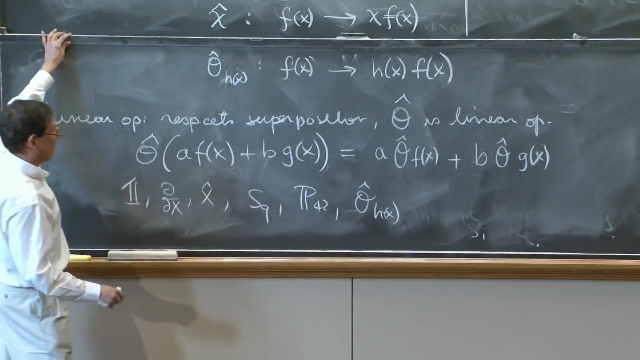 of the list of operators that we have, let's see: 1, ddx. x. how much? which one? sq p42, and O sub h of x. Let's see. Let's vote on each one, whether it's linear or not. 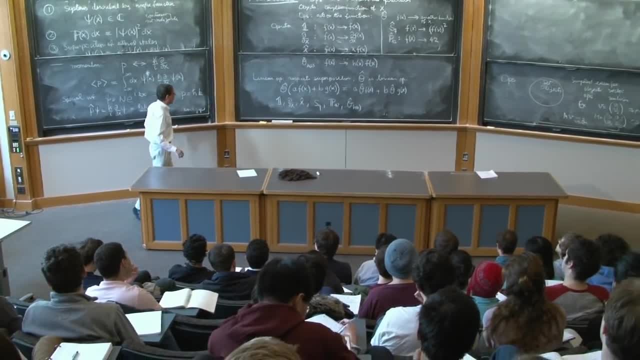 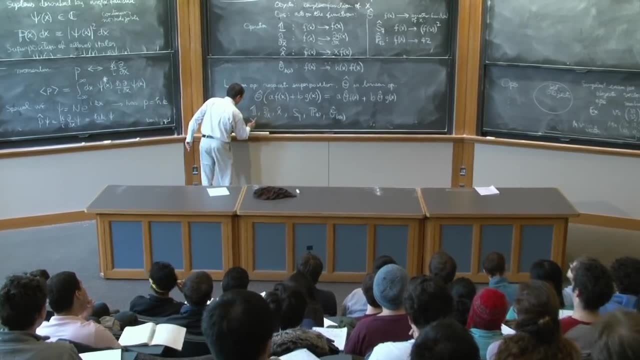 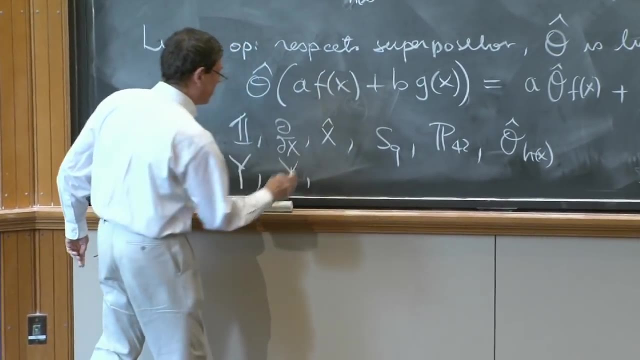 A shouting match. whether I hear a strong or yes or no. OK, 1 is a linear operator. yes, Yes, No, Yes, All right, ddx linear. yes, Yes, Good, that's strong enough. Don't need to hear the other one. 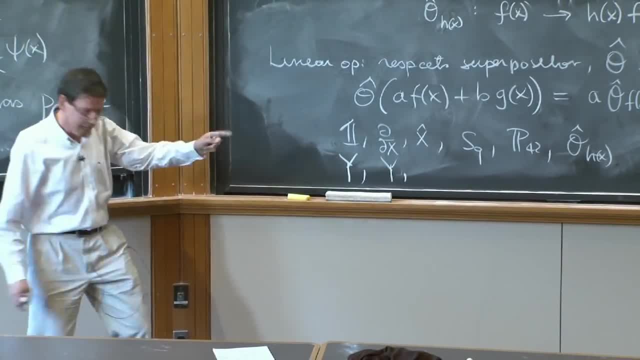 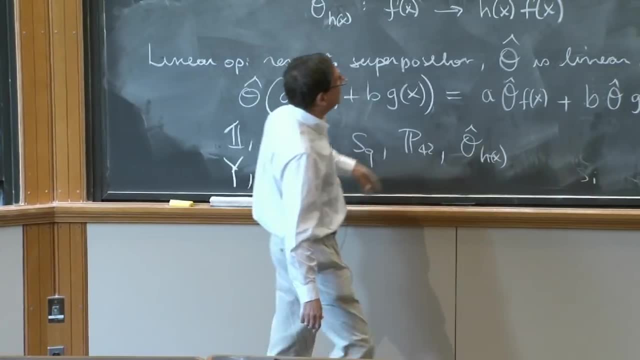 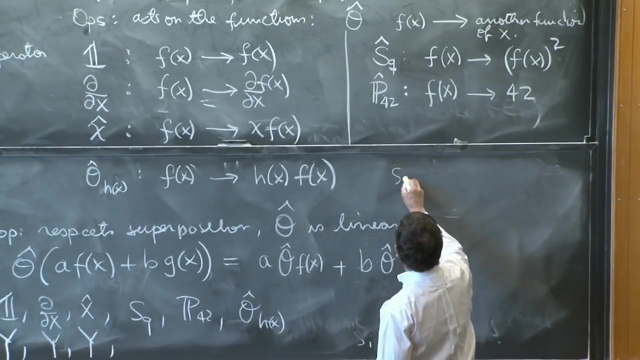 x hat linear operator. yes or no? Yes, Yes, good, Squaring linear operator. No, no, no way it could be a linear operator. It just doesn't, It just doesn't happen. If you have sq on f plus g, it would be f plus g squared. 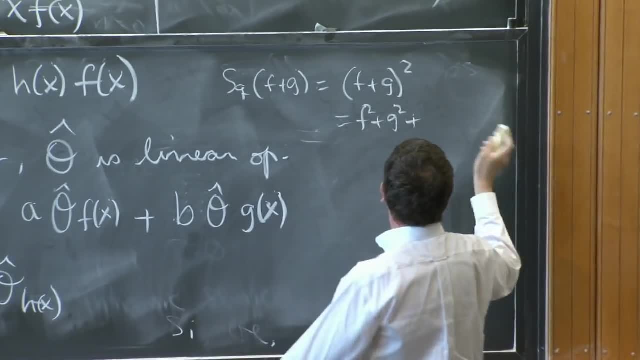 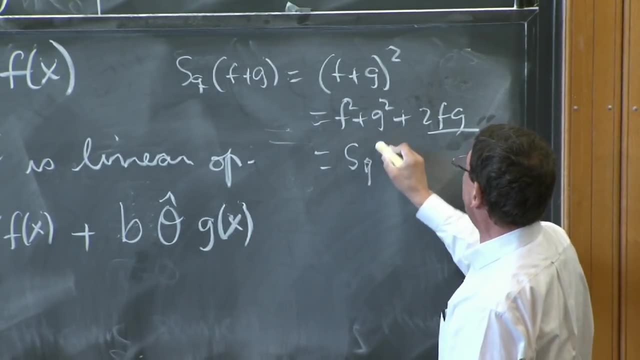 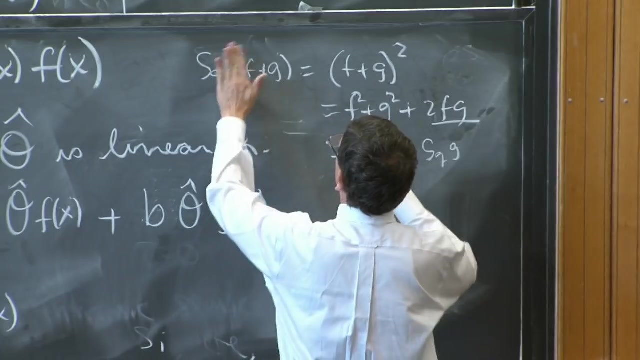 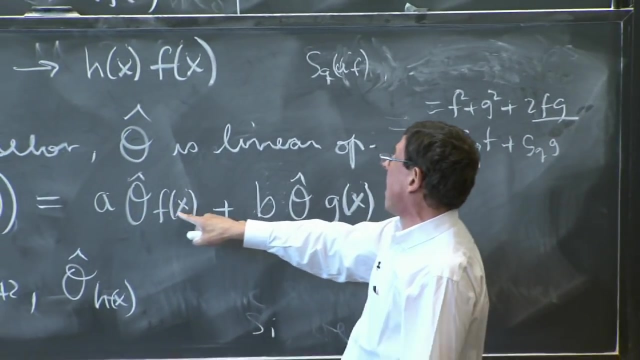 which is f squared plus g squared plus, unfortunately, to fg, And this thing ruins it because this is sq of f plus sq of g. It's even worse than that. You put sq on af By linearity. it should be a times the operator. 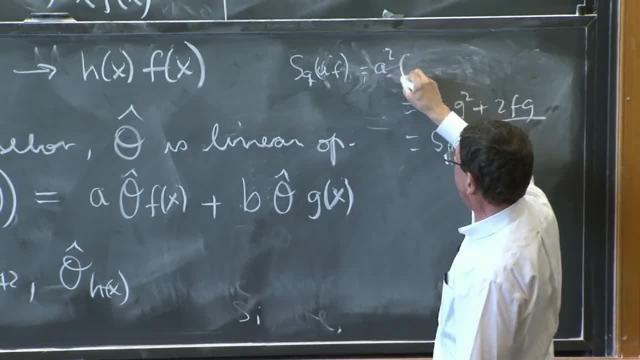 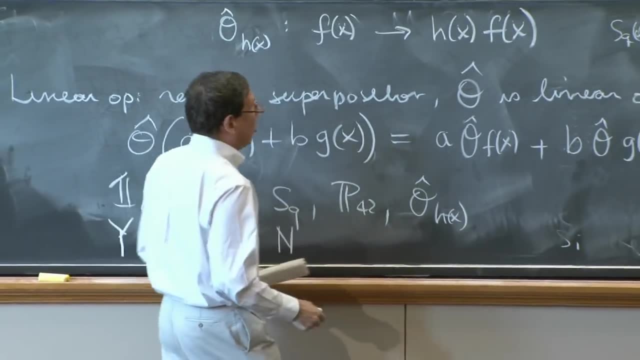 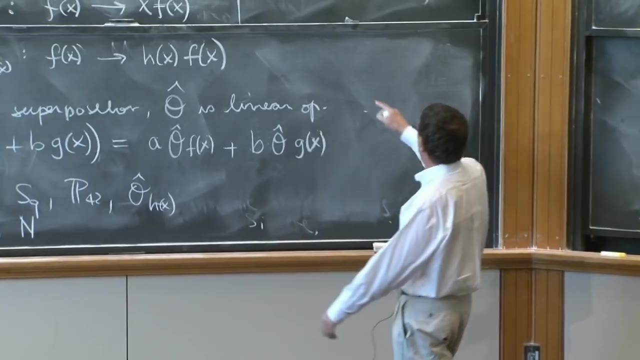 But when you square a times f, you get a squared f squared, So you don't even need two functions to see that it's not real. So definitely no. How about p42?? No, of course not, because if you add two functions, 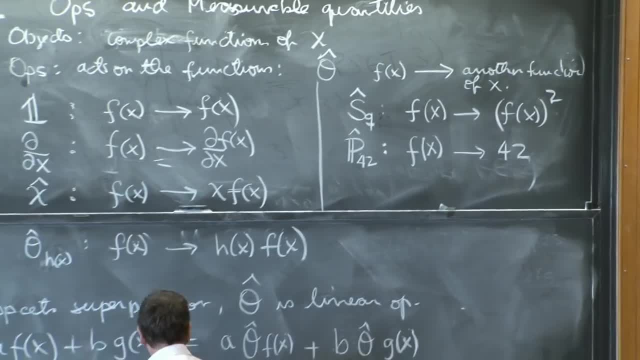 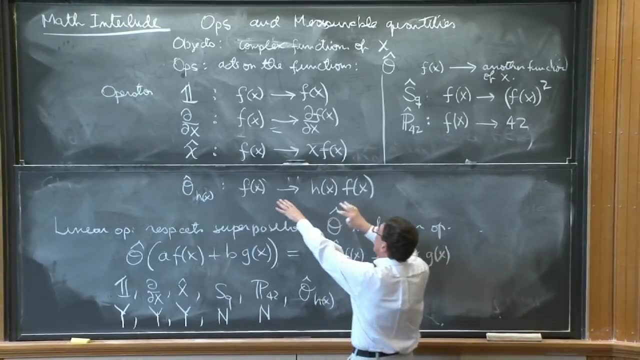 it still gives you 42. It doesn't give you 84. So, no, How about oh of x? Yes, Yes, it does that If you act with this operator on a sum of functions, distributive law- it works. 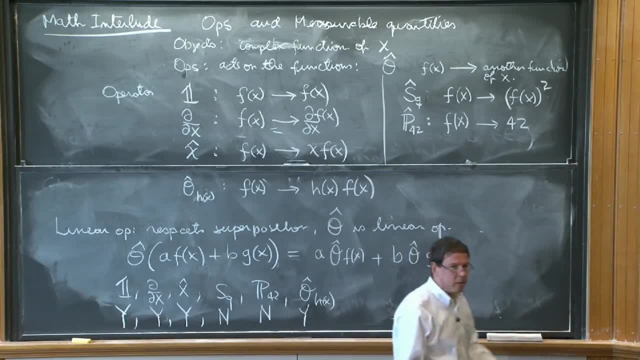 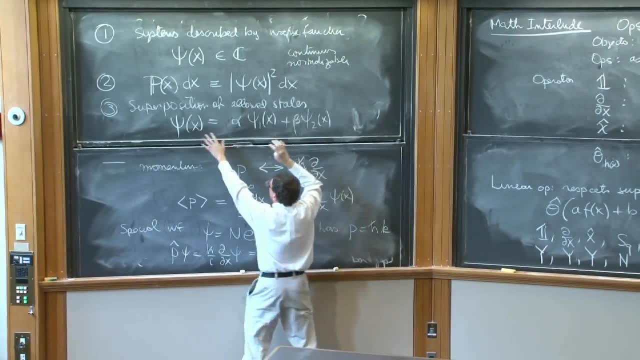 So this is linear. Good Linear operators are important to us because we have superposition of allowed states. So if this is a state and this is a state, this is also a good state. So if we want superposition to work, we can't. 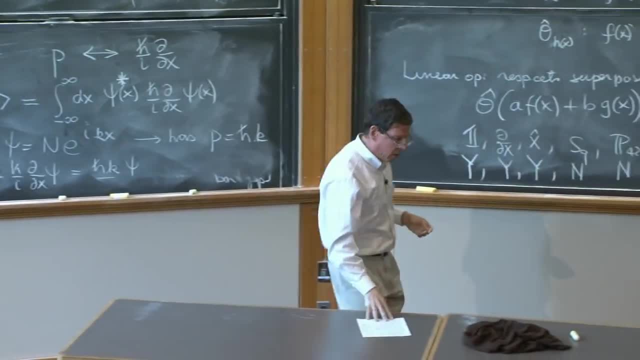 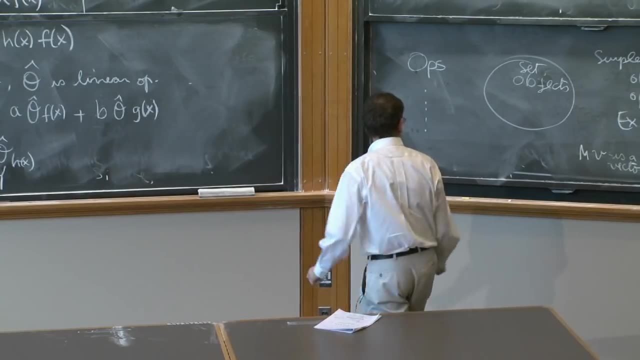 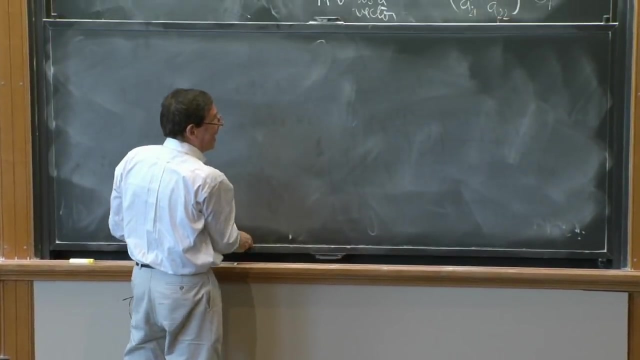 To work well with our theory. we want linear operators, So that's good. So we have those linear operators. And now operators have another thing that makes them sometimes special. It is the idea that they act. They're simpler objects They can act on. 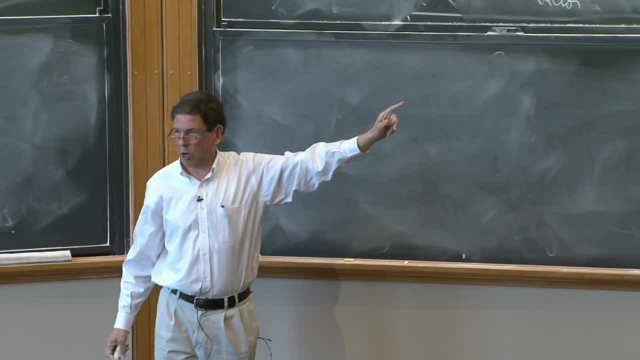 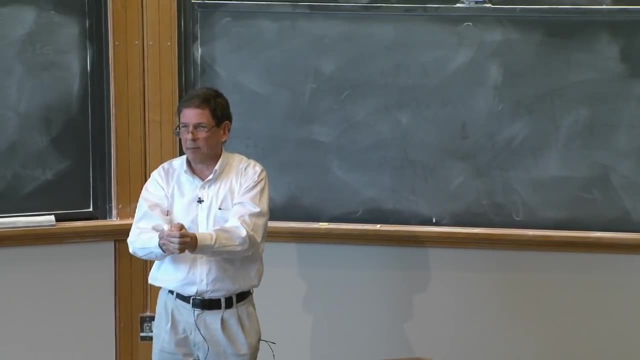 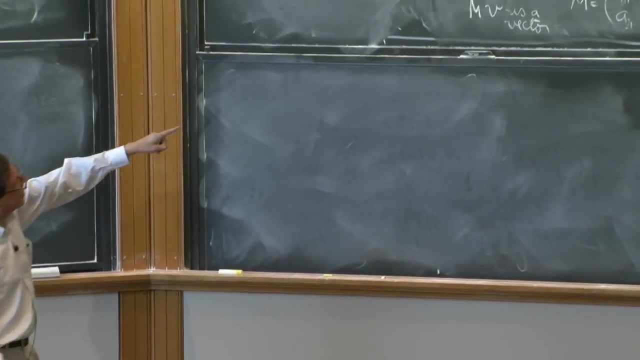 We don't assume you've studied linear algebra in this course. So whatever I'm going to say, take it as motivation to learn some of linear algebra. at some stage You will need a little more linear algebra in 8.05.. But at this moment just basic ideas. 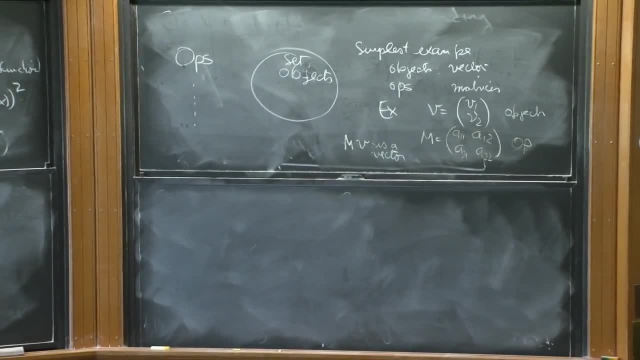 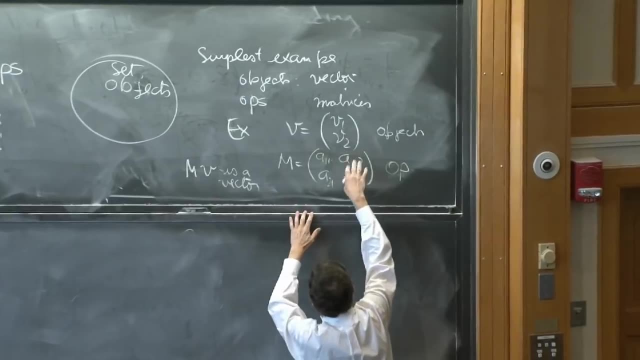 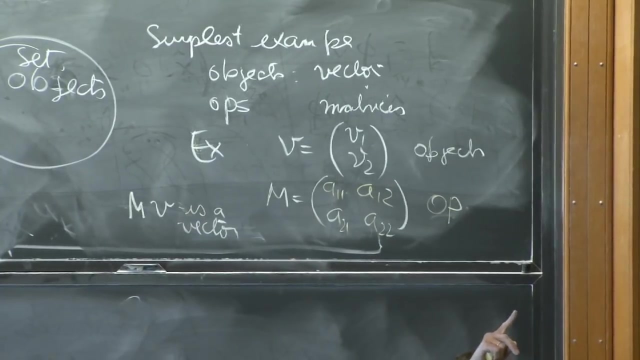 So whenever you have matrices, one thing that people do is to see if there are special vectors. Any arbitrary vector when you act it with a matrix is going to just jump and go somewhere else, point in another direction. But there's some special. 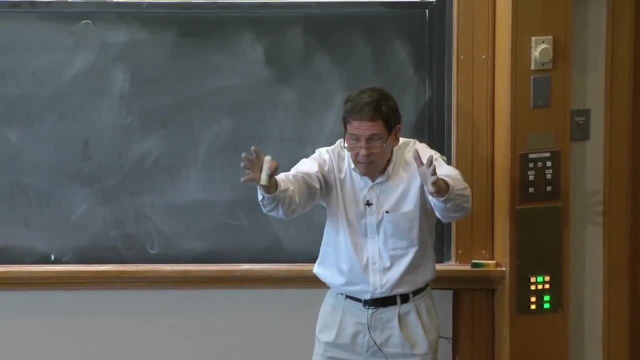 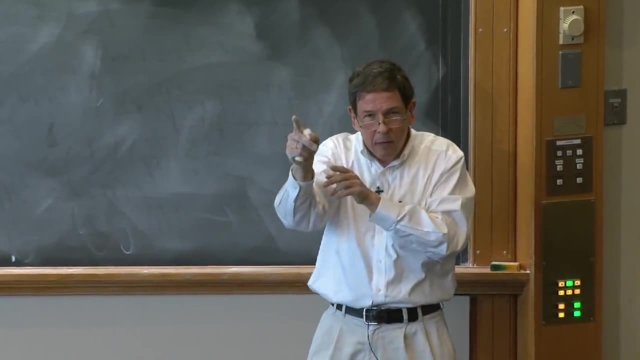 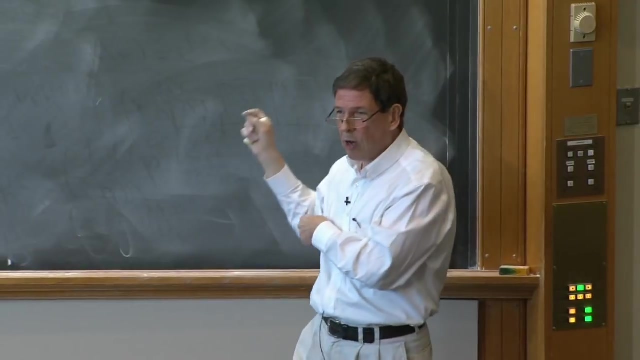 There's some special vectors that you act If you have a given matrix M. there are some funny vectors sometimes that, acted by M, remain in the same direction. They might grow a little or become smaller, but they remain in the same direction. These are called eigenvectors. 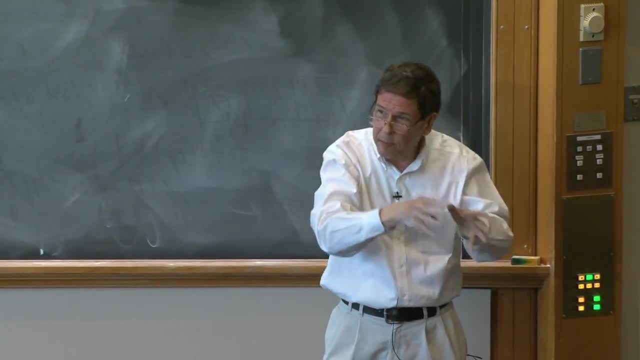 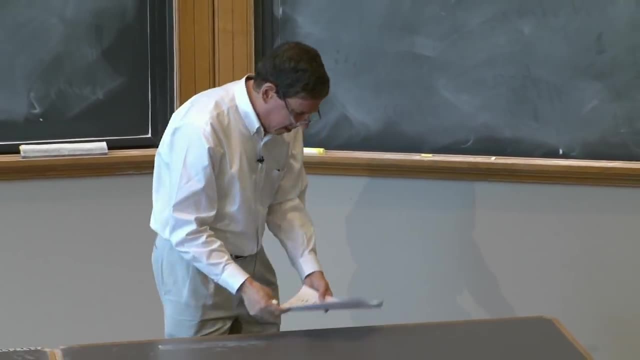 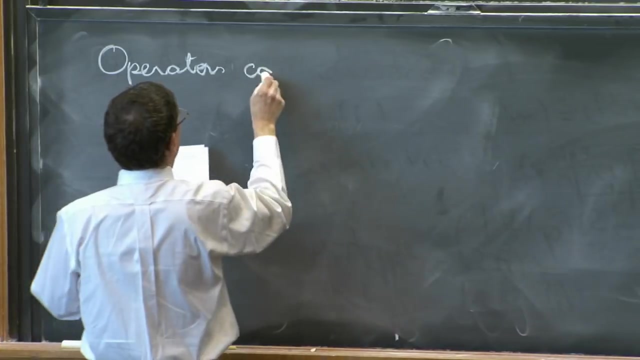 And that constant of proportionality- proportional to the action of the operator on the vector- is called the eigenvalue. So these things have generalization And we're going to talk about eigenvectors and eigenfunctions for our operators. So operators can have special functions, eigenfunctions. 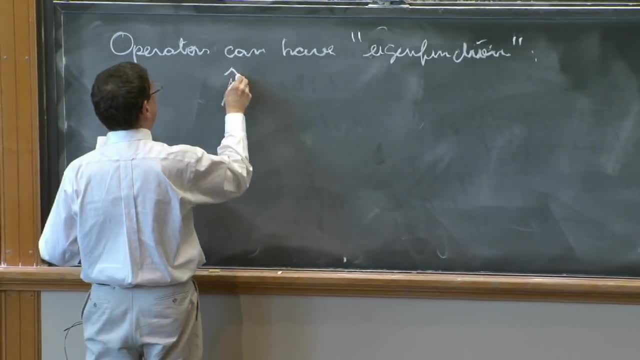 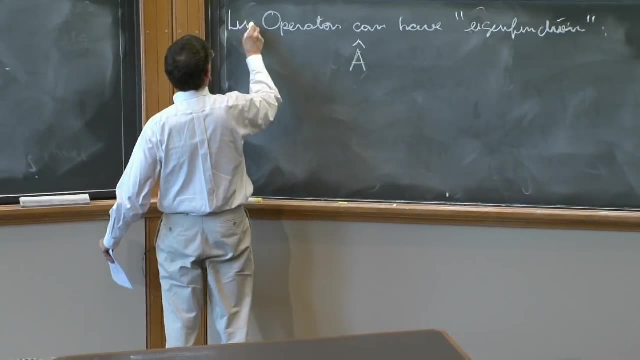 What are these eigenfunctions? So let's consider the operator A hat. It's some operator, I don't know which one of these, but we're going to talk about linear operators or linear operators. It's going to have eigenfunctions. 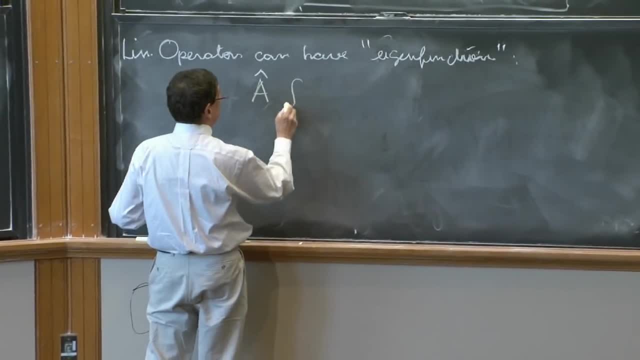 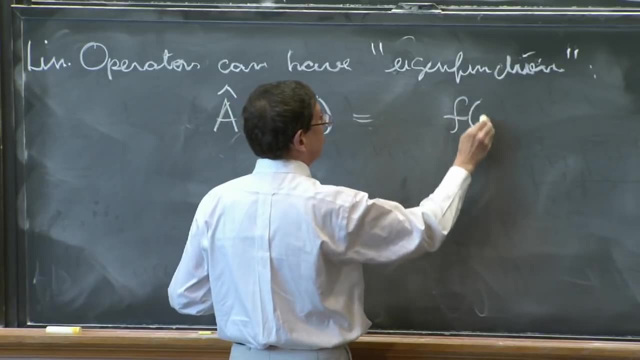 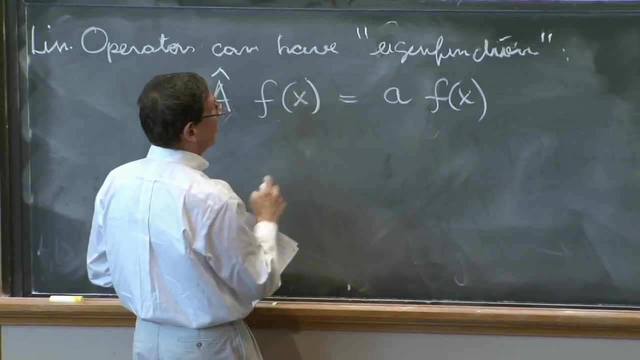 A hat, So A hat. there may be functions that when you act with the operator you sort of get the same function up to possibly a constant A, So you may get A times the function And that's a pretty unusual function. 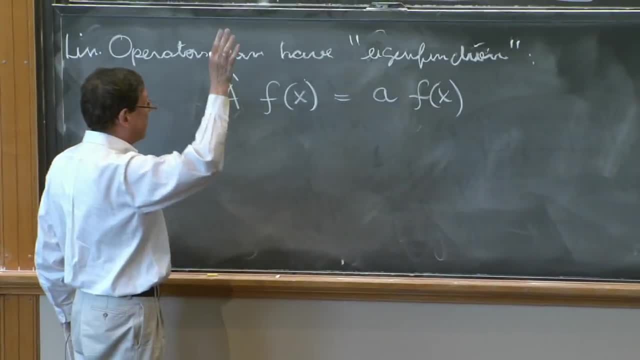 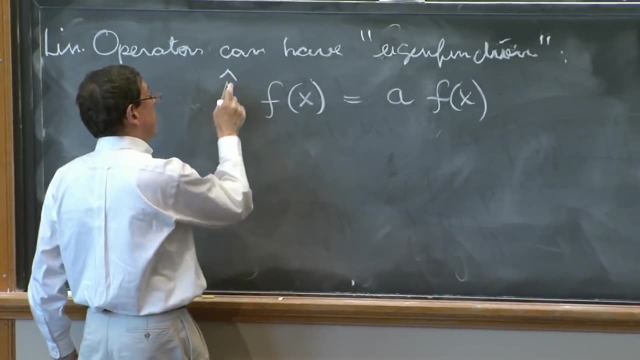 because on most functions any given operator is just going to make a mess. It's going to make a mess out of the function, But sometimes it does that. So to label them better, with respect to operator A, we put the subscript A, which means 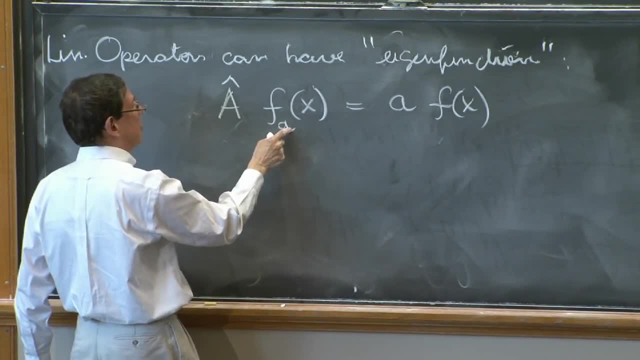 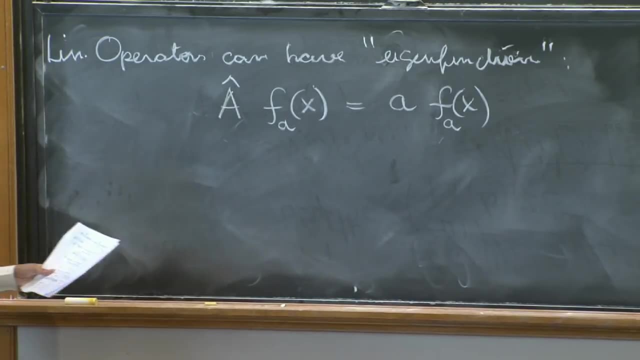 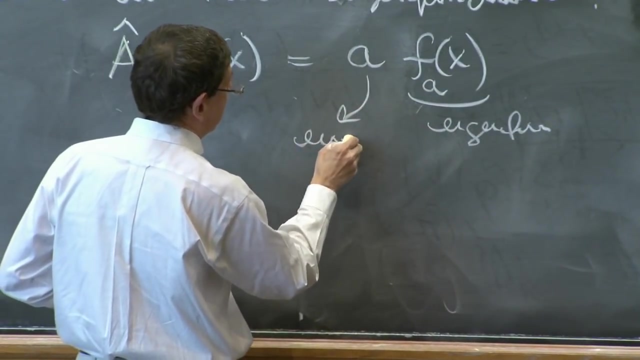 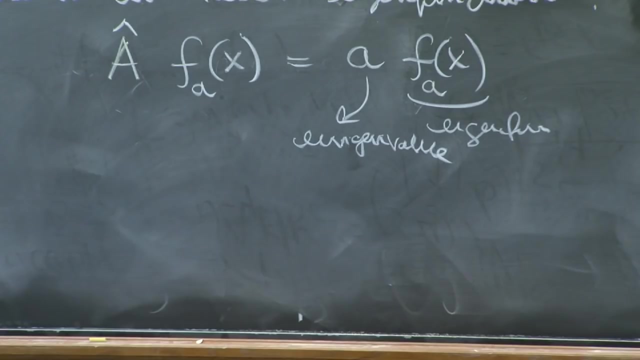 that there's some special function that has a parameter A, for which this operator gives you A times that special function, And that special function is called: this is the eigenfunction and this is the eigenvalue, And that eigenvalue is a number. 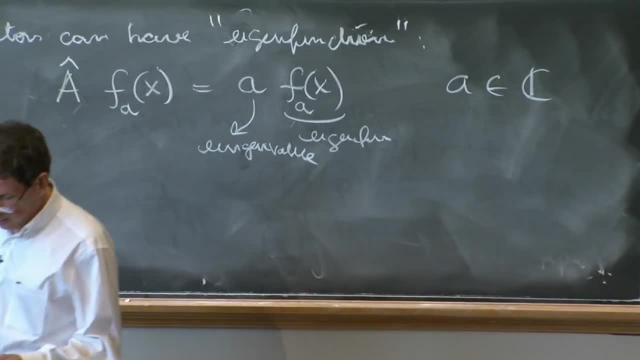 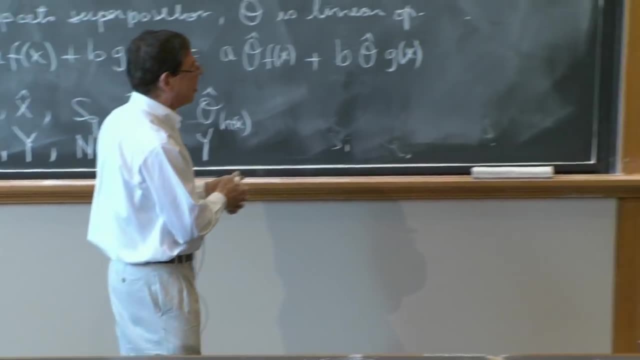 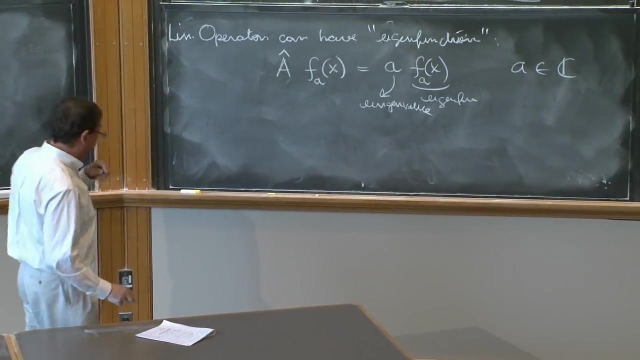 It's a complex number, that C letter over there. So these are special things. They don't necessarily happen all the time to exist, but sometimes they do and then they're pretty useful And we have one example of them that is quite nice for the operator A. 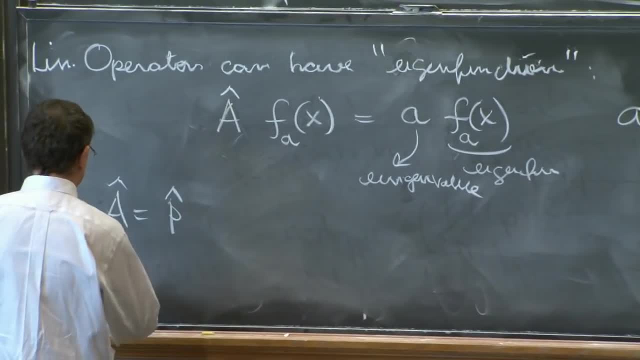 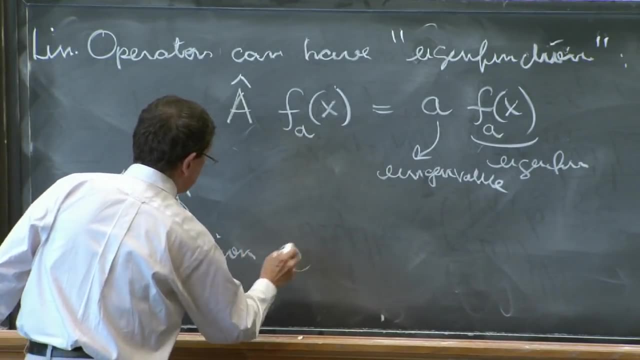 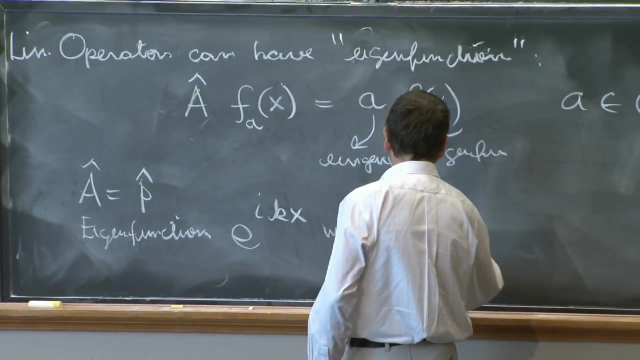 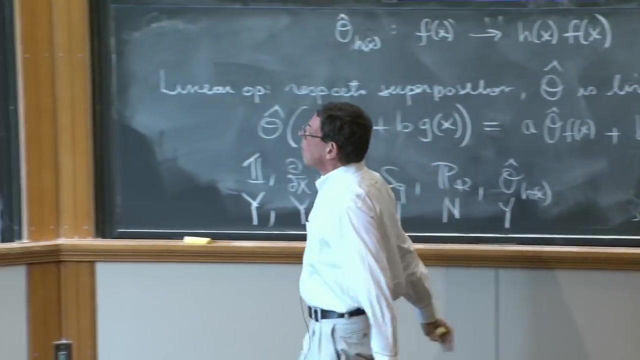 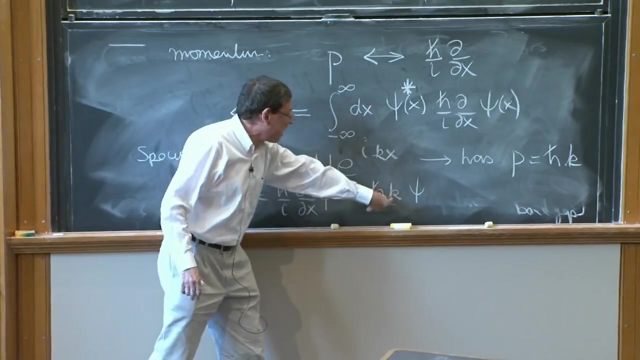 So if we put A equals P, we have eigenfunctions e to the ikx with eigenvalue hk. So this is the connection to this whole thing. We wanted to make clear for you that what you saw here, interacting on this function, gives you something. 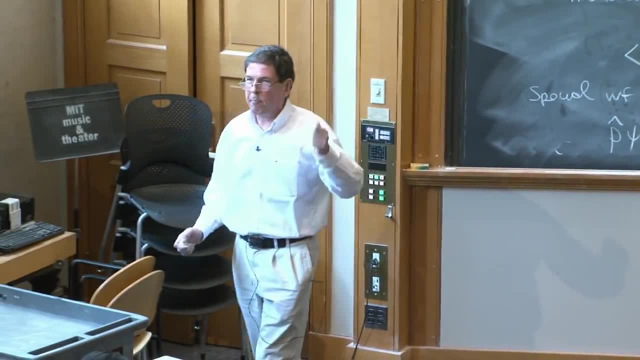 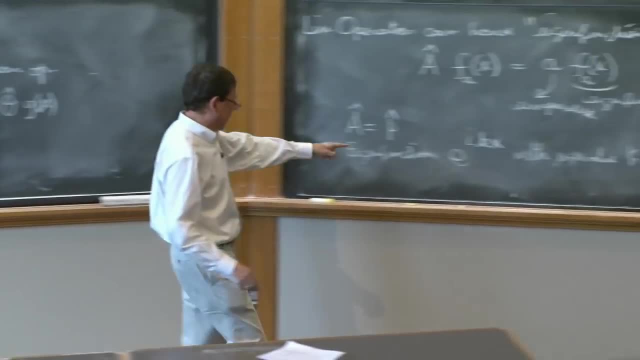 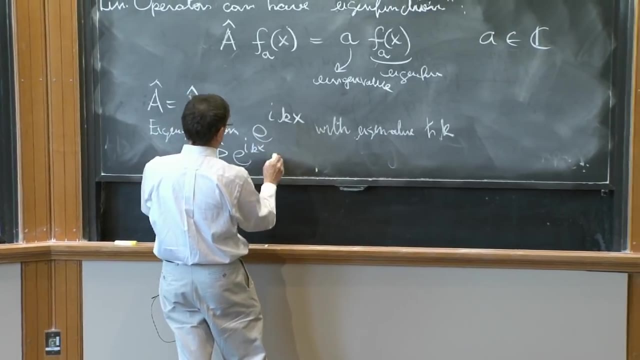 times this function is a general fact about operators. Operators have eigenfunctions. So the eigenfunction e of x with eigenvalue hk, because indeed P hat on this e to the ikx. as you've seen, is h bar k times e to the ikx. 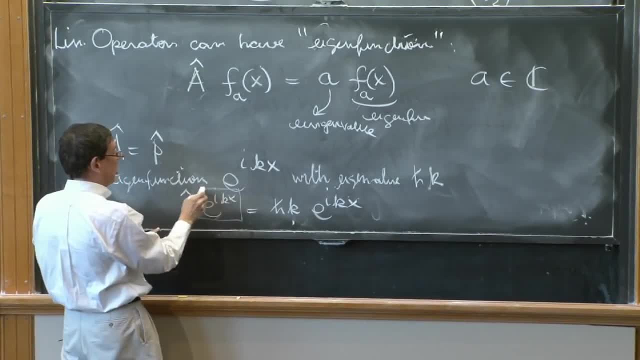 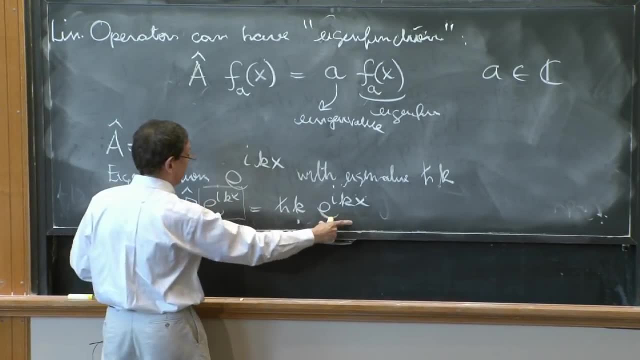 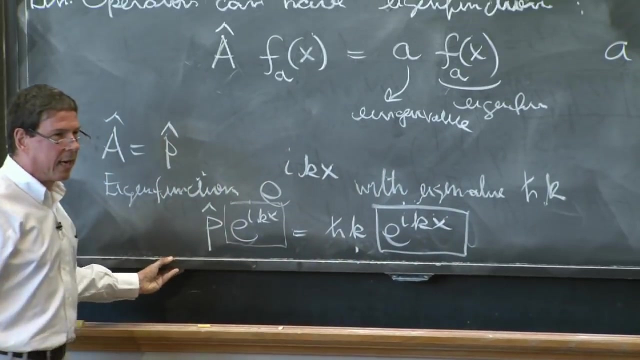 So here you have P. hat is the A. This is the function Labeled A would be like k. Here is something like k again and here is this thing, But the main thing. operator on the function: number times. the function is an eigenfunction. 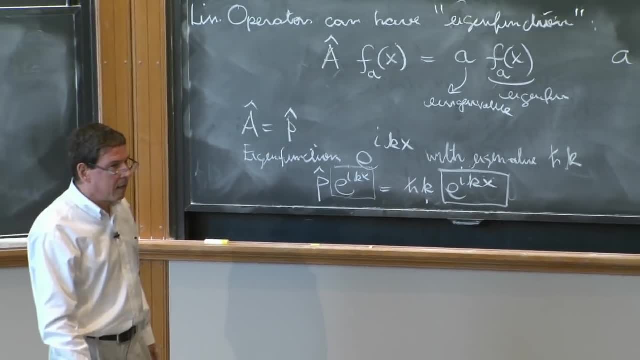 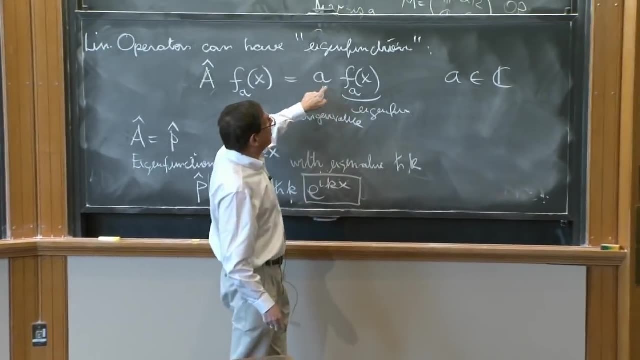 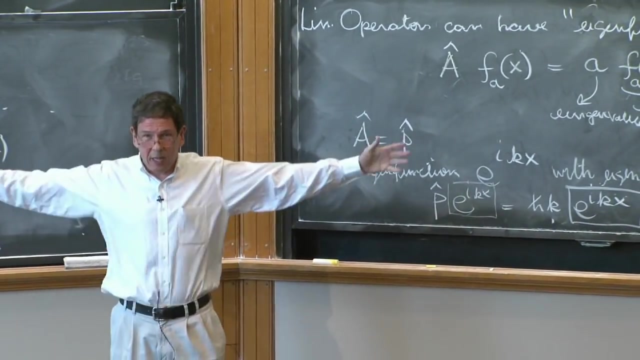 Yes, For a given operator, is the eigenvalue constant by an e here. Well, for a given operator, good question, A is a list of values, So there may be many, many, many eigenfunctions. Yes, Many cases, infinitely many eigenfunctions. 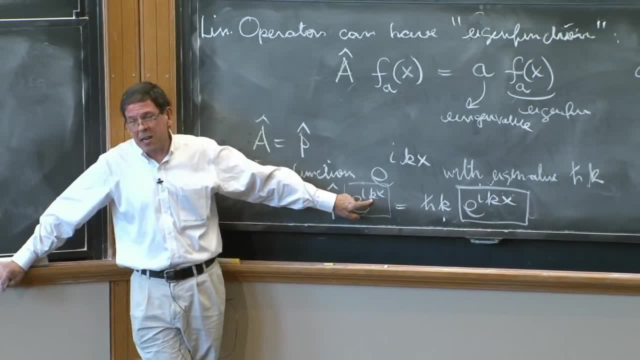 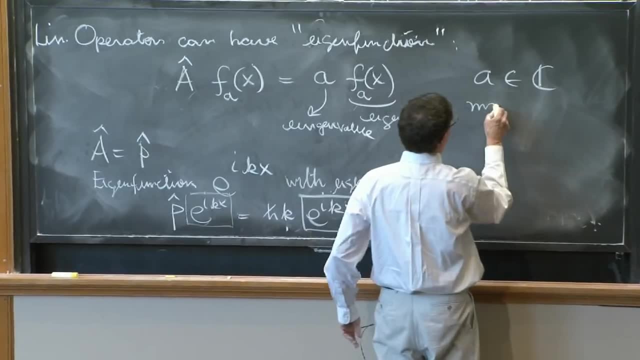 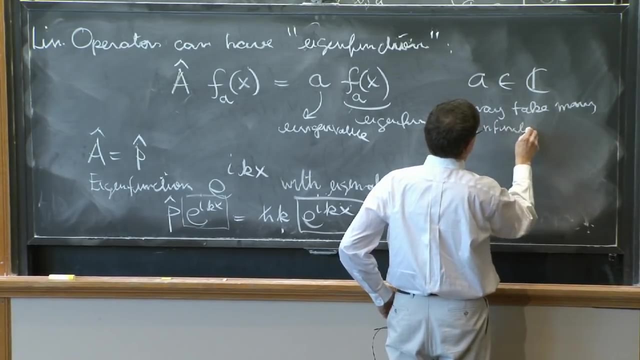 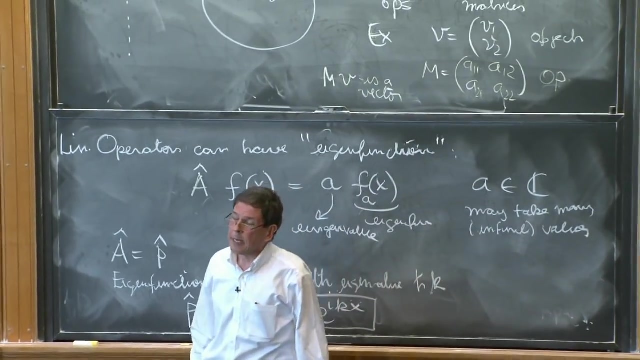 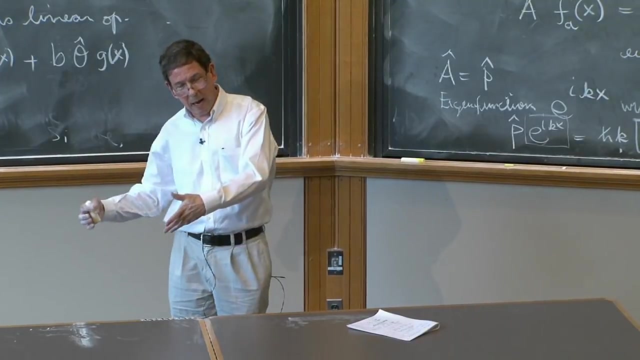 In fact here I can put for k any number I want and I get a different function. So A belongs to C and may take many or even infinite values. If you remember, for nice matrices n by n matrix may mean a nice n by n matrix has n eigenvectors and eigenvalues. 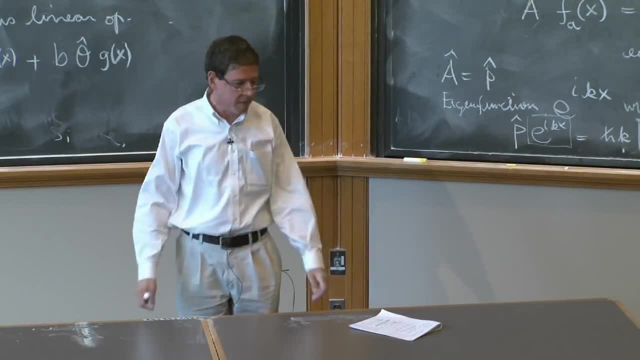 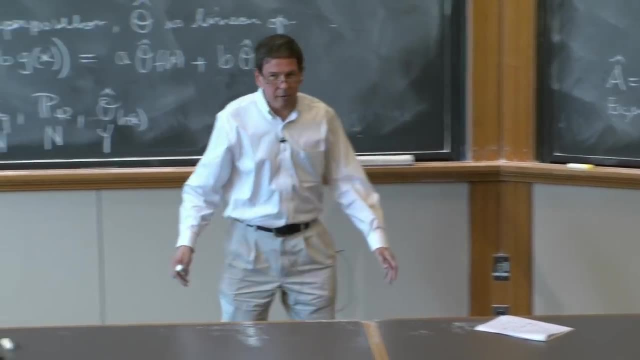 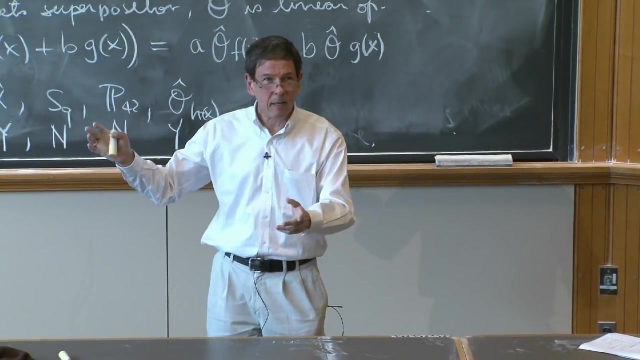 that sometimes are degenerate. Sometimes the eigenvalues have the same numbers and things like that. So, OK, linearity Is the sum of two eigenvectors: an eigenvector Yes, No, No, No, Correct That's. 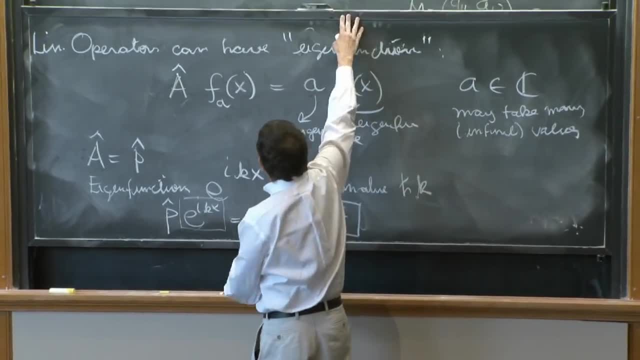 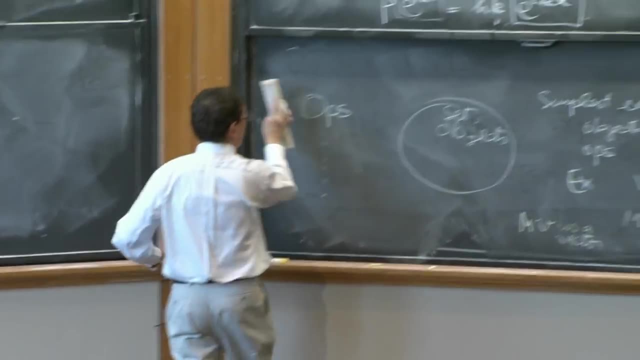 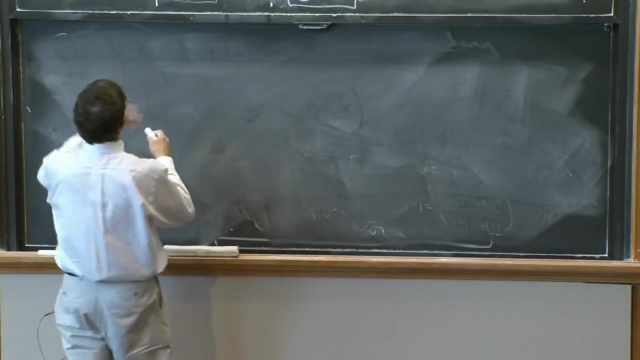 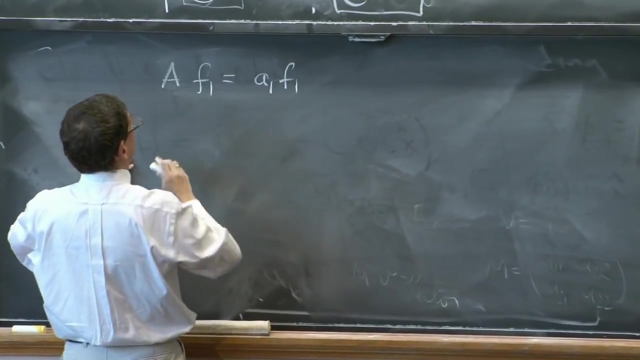 Not necessarily true. If you have two eigenvectors, they have different eigenvalues, so things don't work out well necessarily. So an eigenvector plus another eigenvector is not an eigenvector. So you have here, for example, A F1 equal, A1 F1 and A F2 equal. 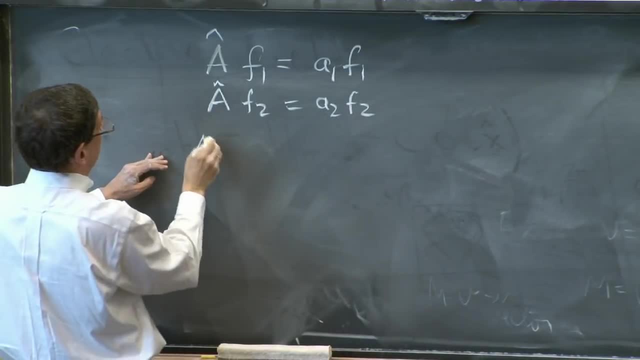 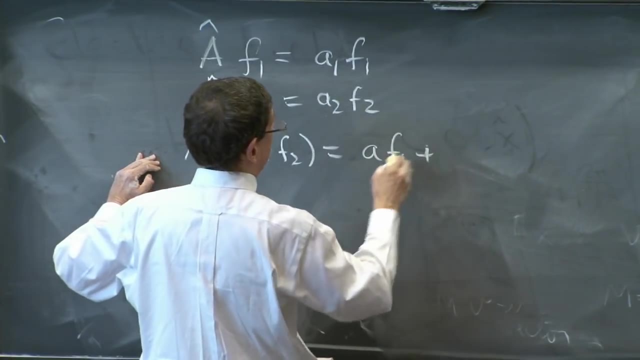 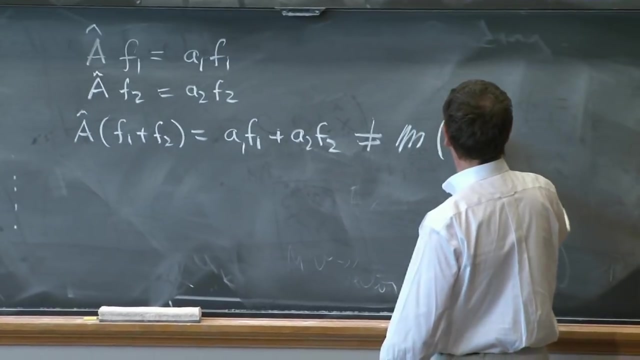 A2, F1.. OK, So if you have A F1 equal A2, F2, then A on F1 plus F2 would be A F1 plus A1, F1 plus A2, F2. And that's not equal to something times F1 plus F2.. 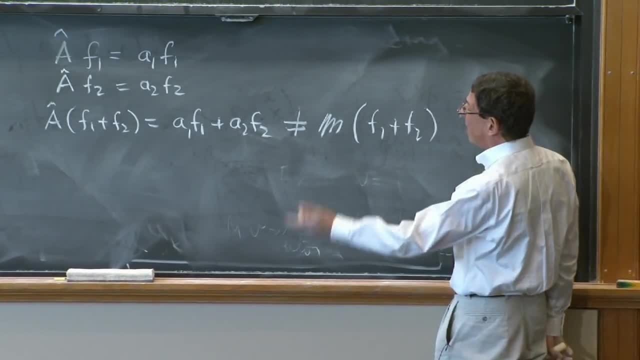 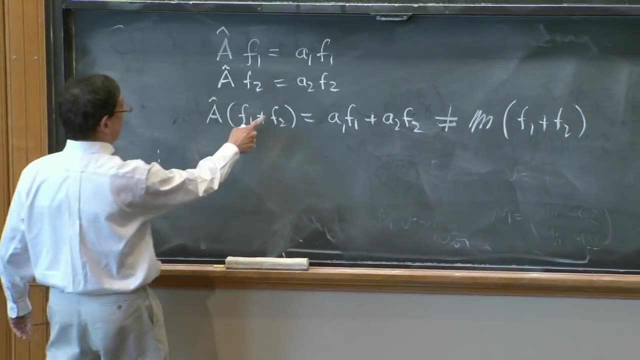 It would have to be something times F1 plus F2 to be an eigenvector. So this is not necessarily an eigenvector And it doesn't help. OK, It doesn't help to put a constant in front of here. Nothing helps. 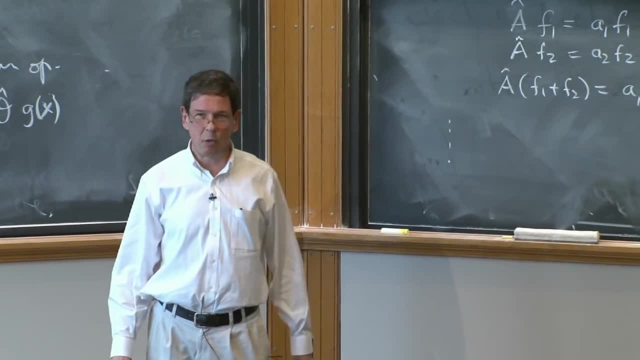 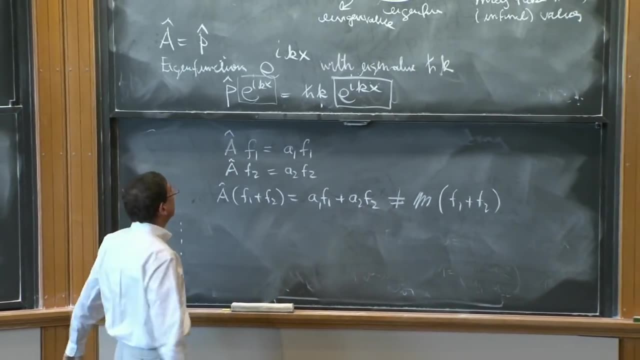 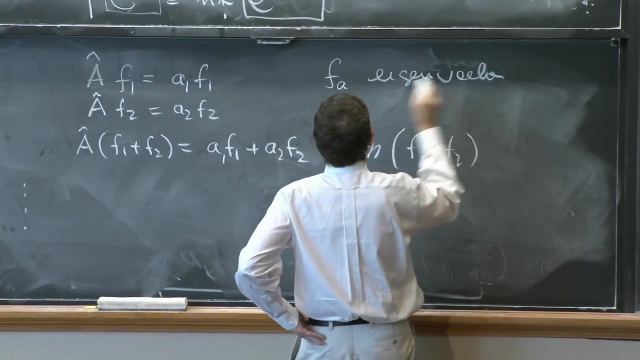 There's no way to construct an eigenvector from two eigenvectors by adding or subtracting. The size of the eigenvector is not fixed either. If F is an eigenvector, then 3 times F is also an eigenvector. 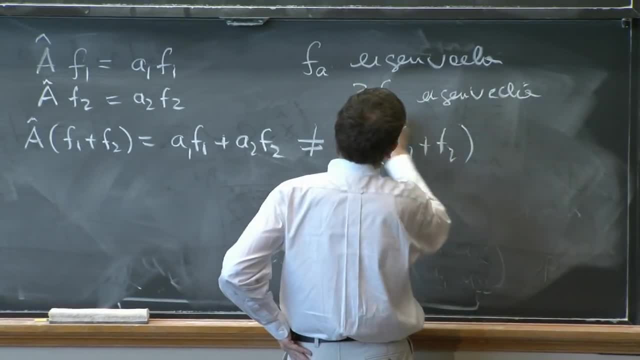 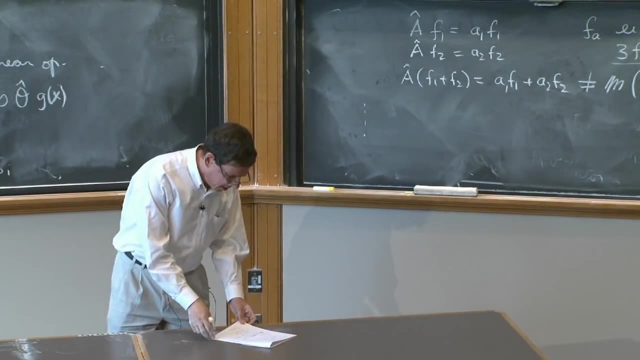 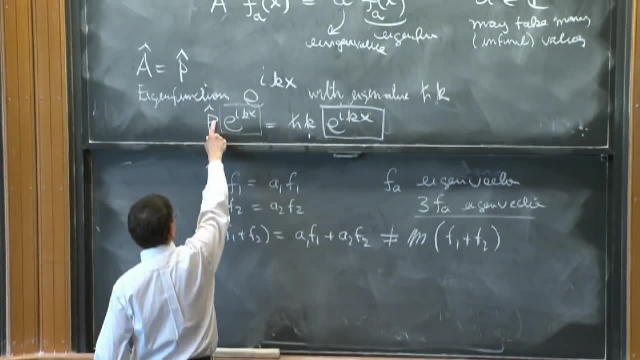 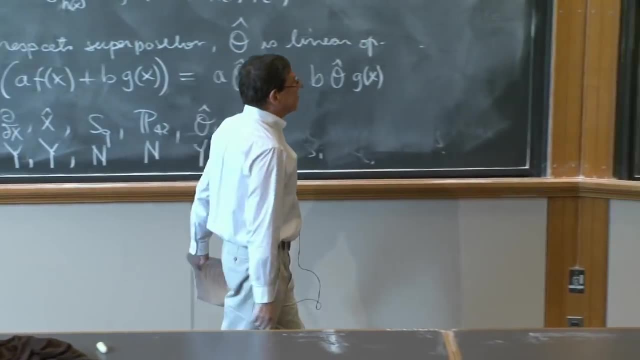 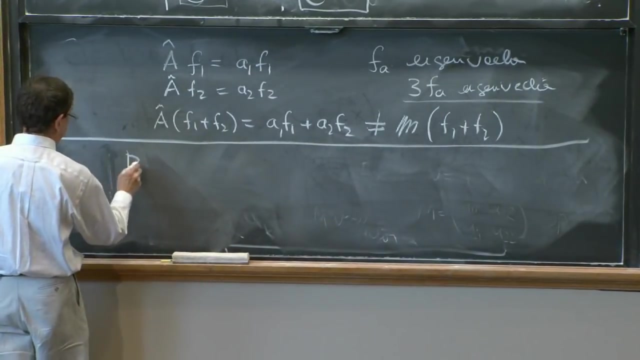 Well, we've seen it here already that one operator that we've learned to work with is the momentum operator. It has those eigenfunctions. So back to physics. we have other operators. Therefore, we have the p operator. That's good. 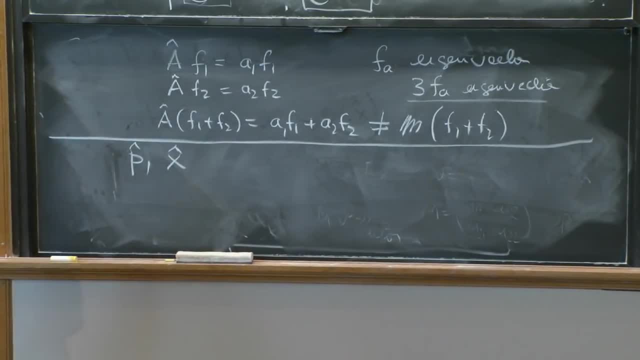 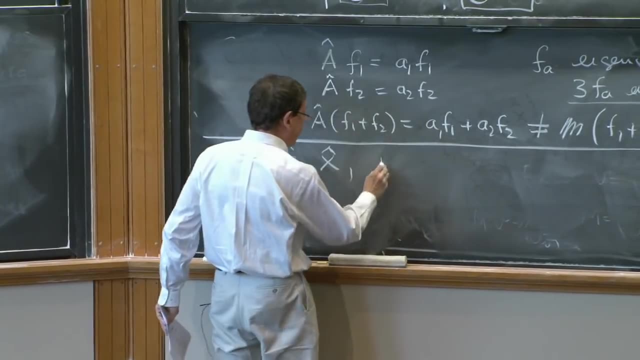 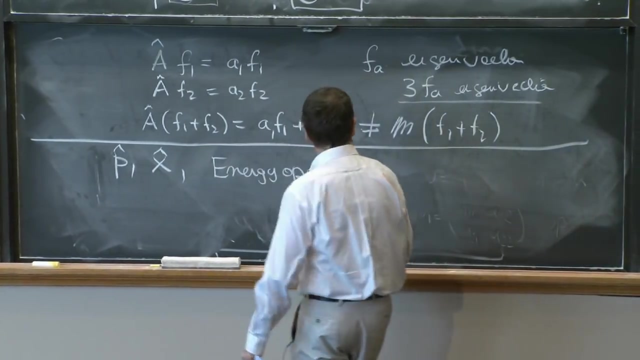 out. we have the x operator. That's nice, It's multiplication by x. And why do we use it? Because sometimes we have the energy operator. And what is the energy operator? The energy operator is just the energy that you've always known. 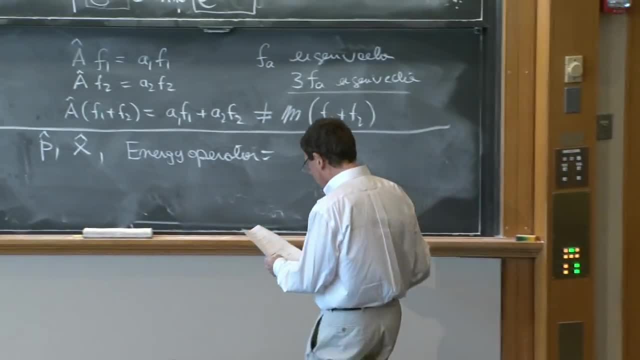 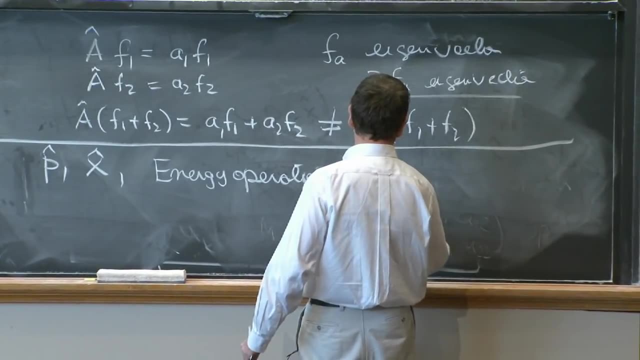 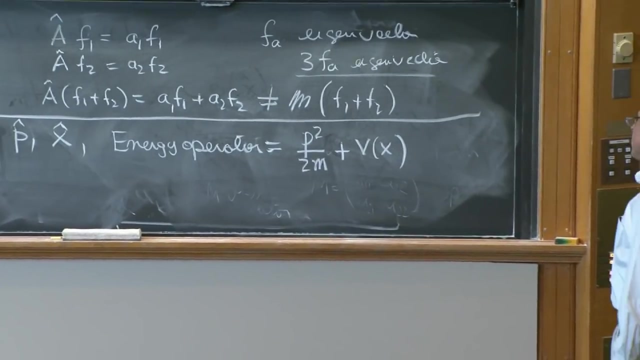 but think of it as an operator. So how do we do that? Well, what is the energy of a particle? We've written p squared over 2m plus v of x. Well, that was the energy of a particle: the momentum. 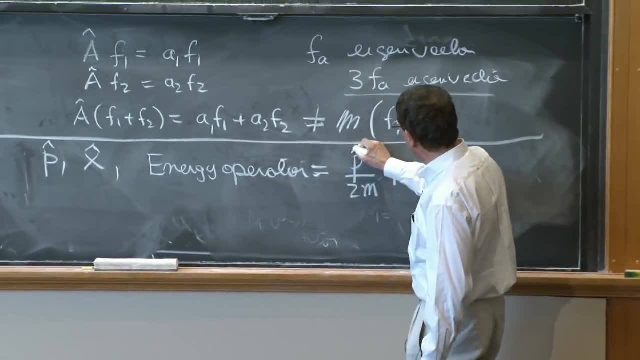 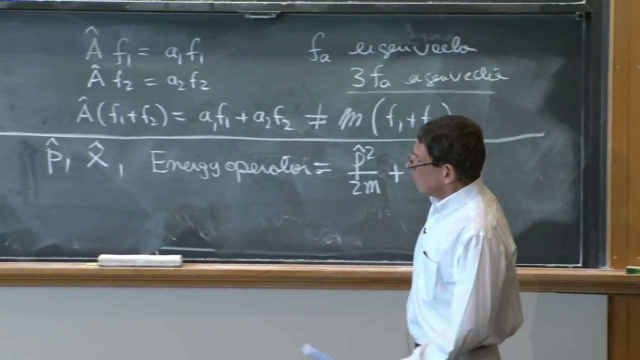 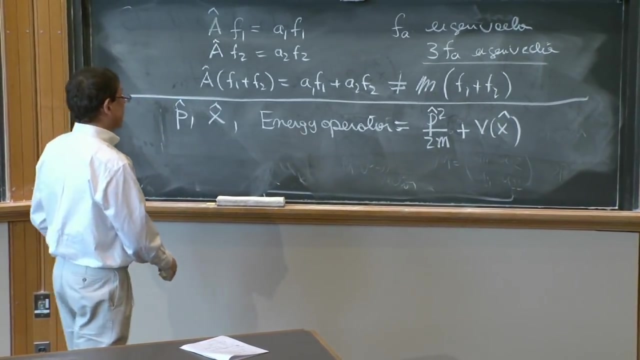 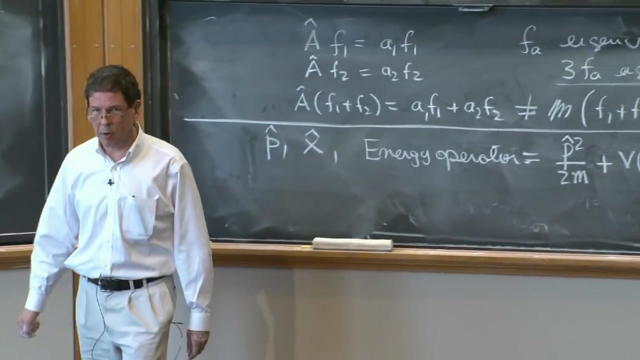 squared over 2m plus v of x. So the energy operator is hat here, hat there, And now it becomes an interesting object. Now this energy operator will be called e hat. It acts on functions, It is not a number. 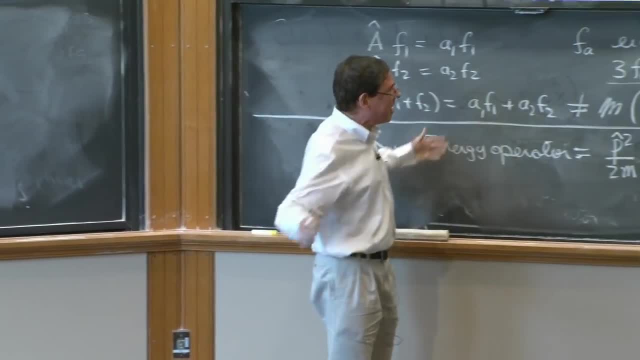 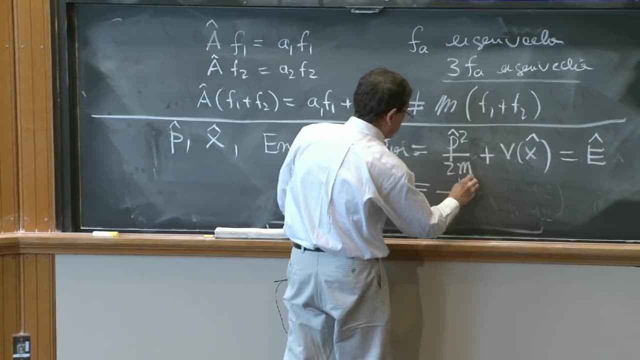 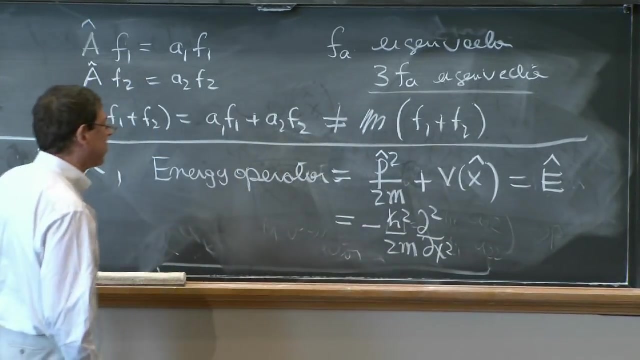 The energy is a number, but the energy operator is not a number. far from a number, In fact. the energy operator is minus h, squared over 2m d, second dx squared. Why that? Well, because p was h bar over i d dx. 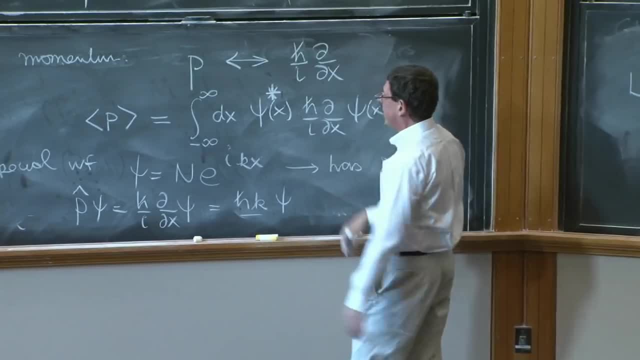 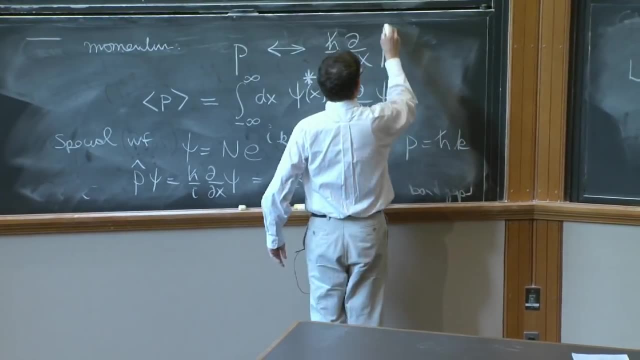 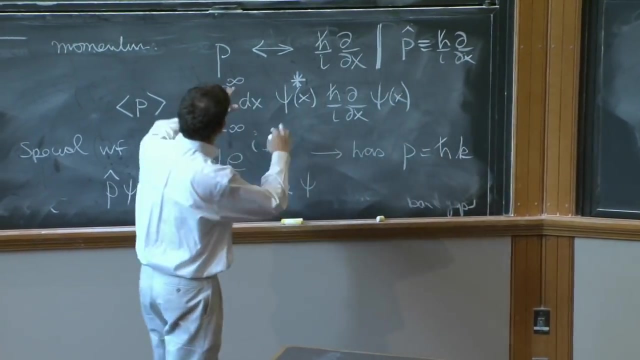 As an operator. So this sort of arrow here. it's sort of the introduction, But after a while you just say p hat is h bar over, i d dx. End of story. It's not like double arrow, It's just what it is. 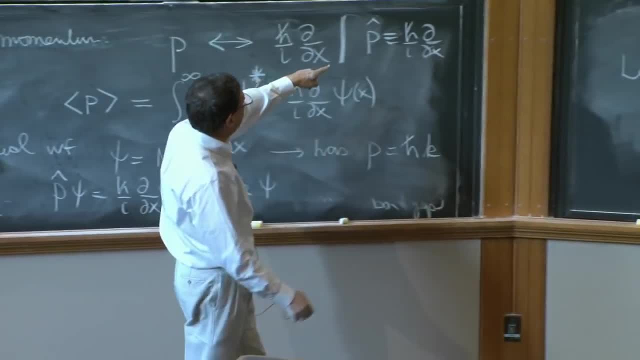 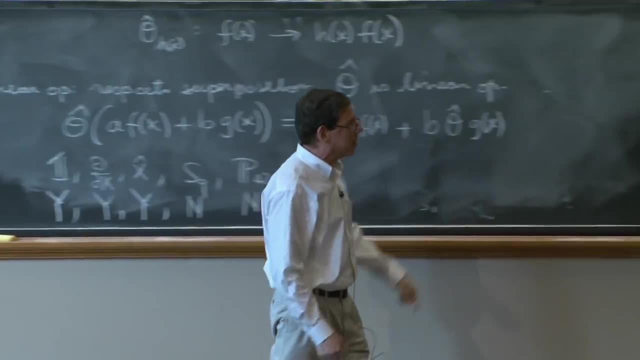 That operator, That's what we call it. So when we square it, the i squared is a minus h squared and d dx and d dx, x applied twice is the second derivative. And here we get v of x hat, which is your good potential. 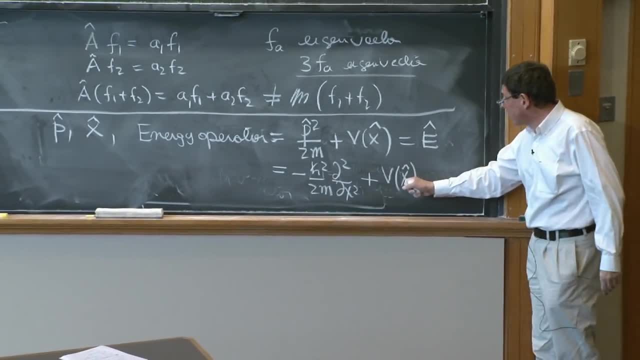 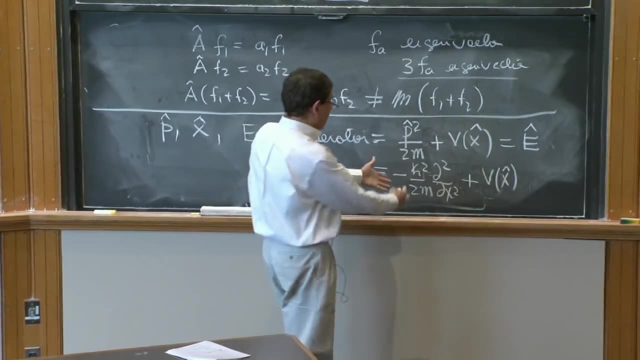 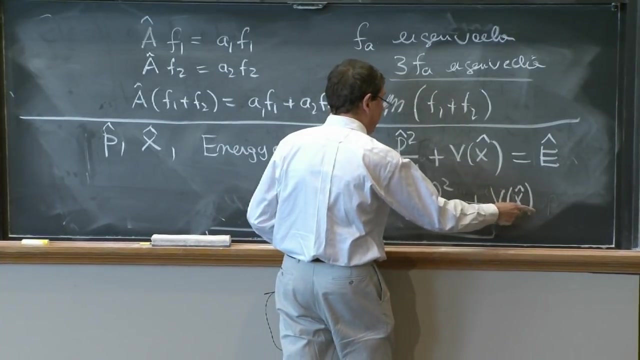 whatever potential you're interested in, in which, whenever you see an x, you put an x hat And now this is an operator. So you see, this is not a number, not a function, It's just an operator. The operator has this sort of operator: v of x. 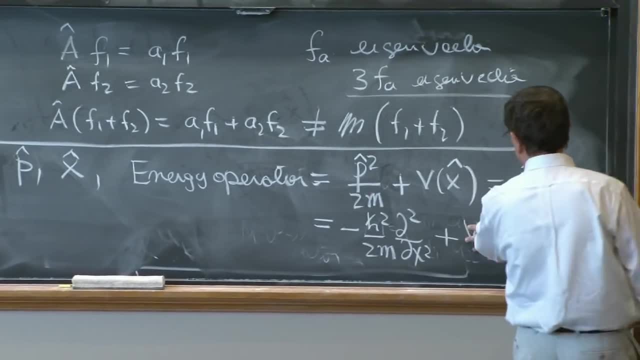 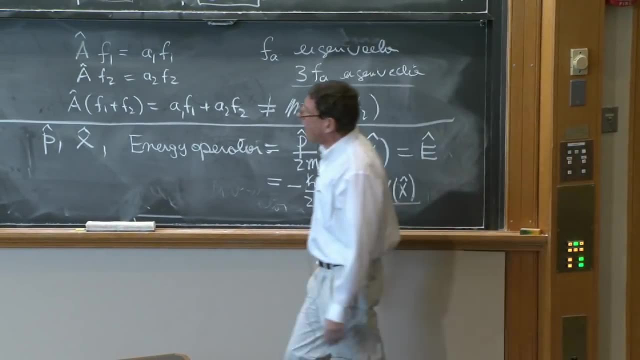 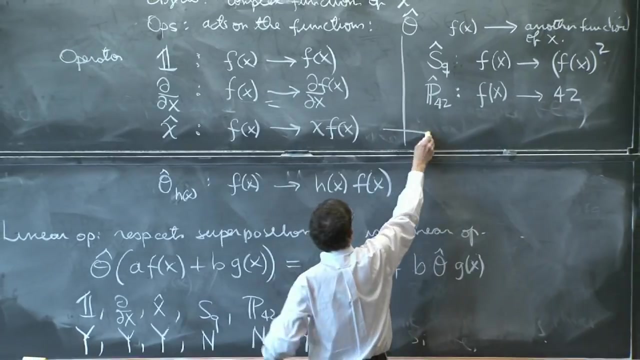 Now, what is this v of x here as an operator? This v of x as an operator is just multiplication by the function v of x. You see, you have here that the operator x is f of x. like that I could have written the operator x hat to the n. 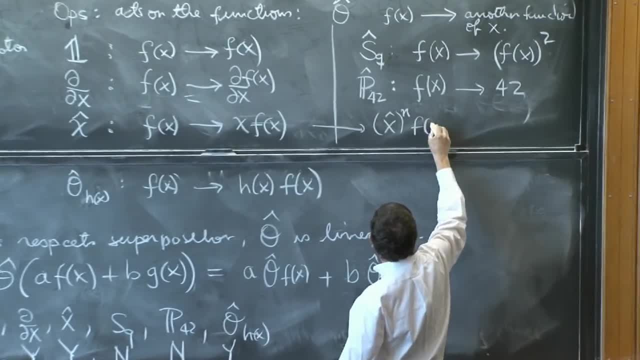 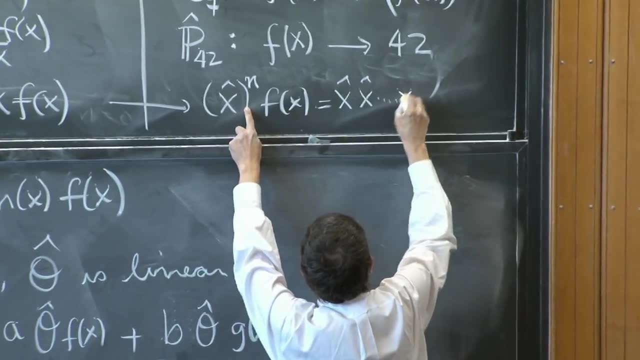 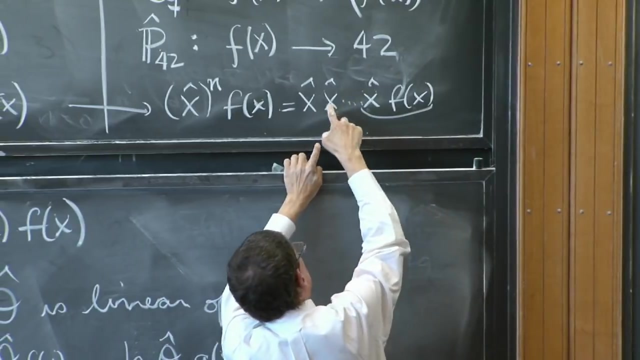 What would it be Well, if I act on a function, this is a lot of x hats. This is a lot of x hats acting on the function. Well, let the first one act. You get x times f of x. The second adds another x, another x. 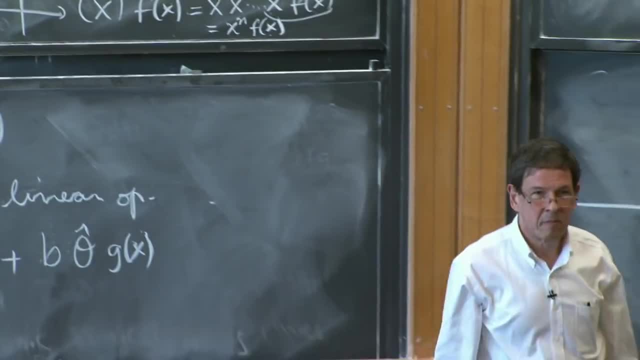 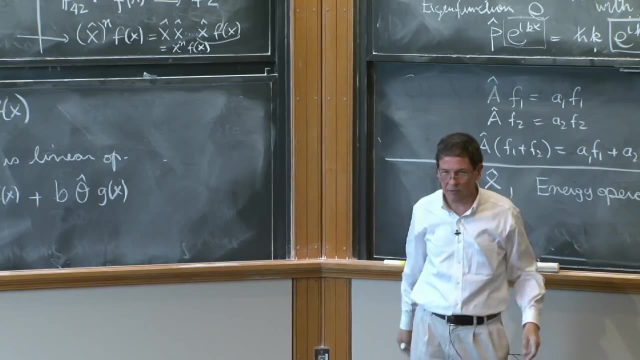 So this is just x to the n times f of x. So lots of x hats x hat to the 100 on a function is just x to the 100 times a function. So v of x on a function is just v of the number x. 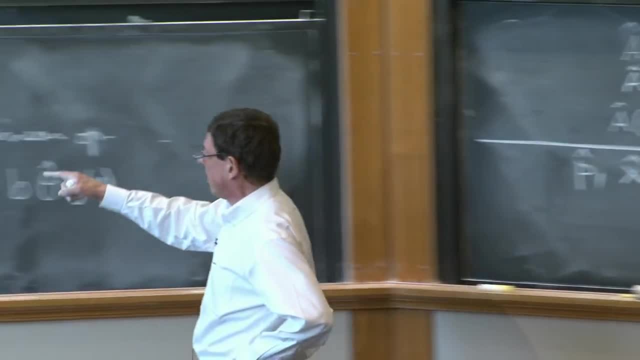 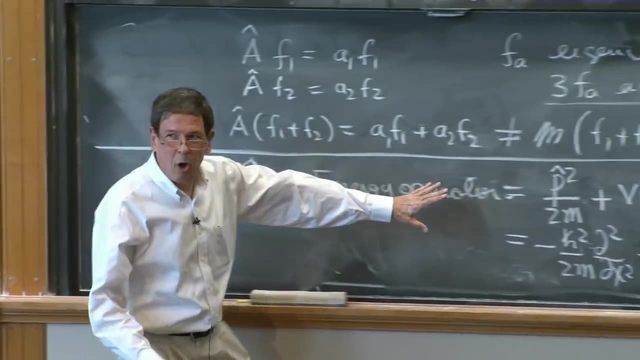 and of the number x. So that's a lot, That's a lot. So v of x on a function is just like this operator, the o in which you multiply by a function. So please, I hope this is completely clear what this means as an operator. 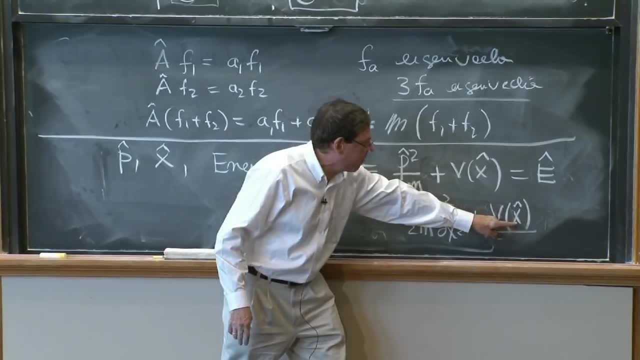 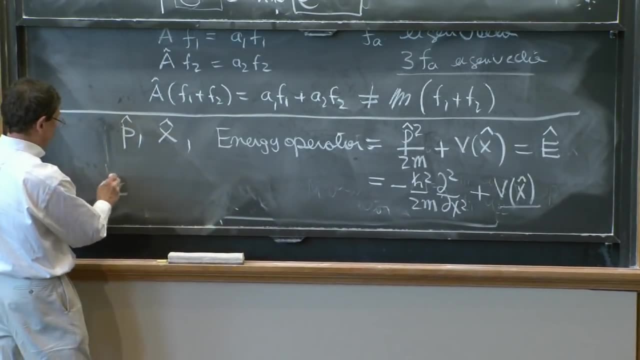 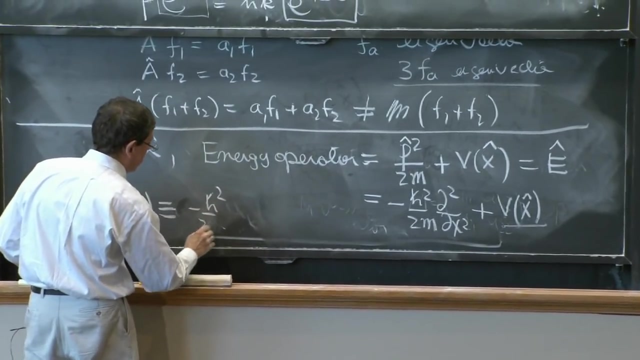 You take the wave function, take two derivatives and add the product of the wave function times v of plane x. So I'll write it here, maybe So important: e hat on psi of x is minus h squared over 2m d, second dx squared of psi of x. 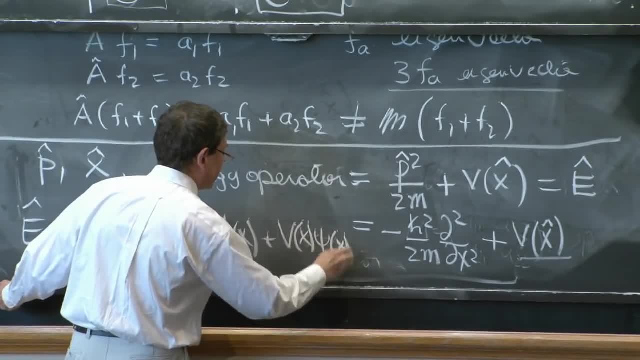 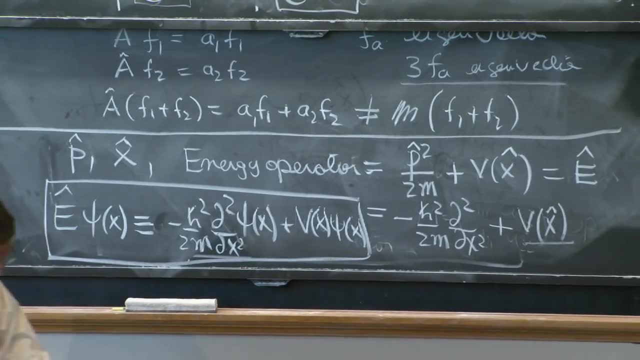 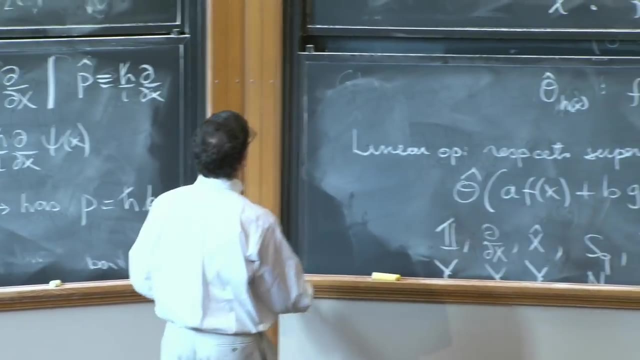 plus just plane v of x times psi of x. That's what it does. That's an operator, And for these operators in general. so we're how, math interlude: Is it over? Not quite, Wow, No, yes. 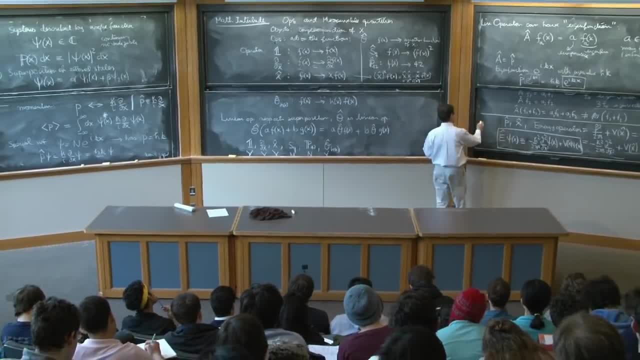 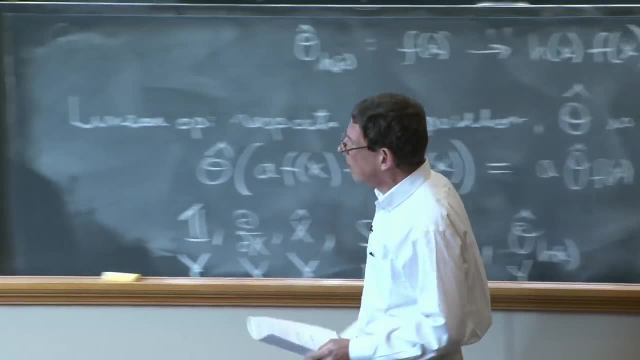 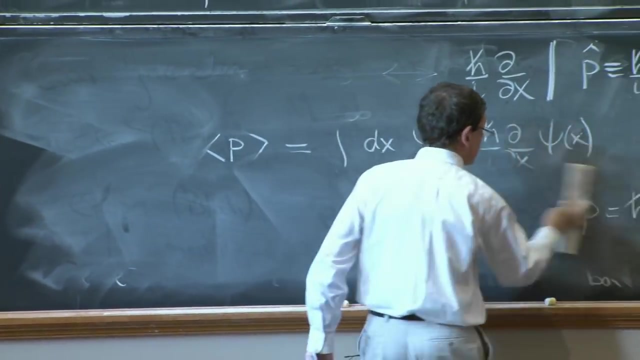 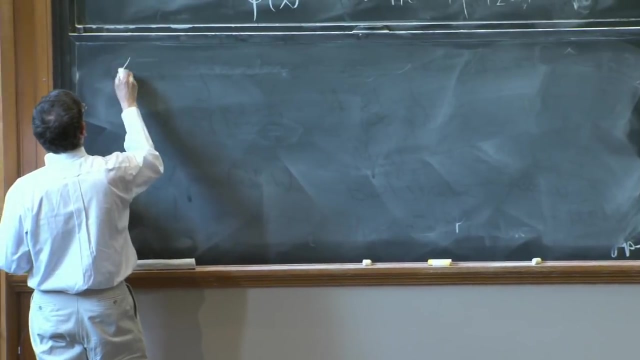 Alan said at this moment it's over when you introduce it here. So here is. I'll say something more here, but it's going to be over now. Our 3 continues here, then with 4.. 4 to each observable: Observable. 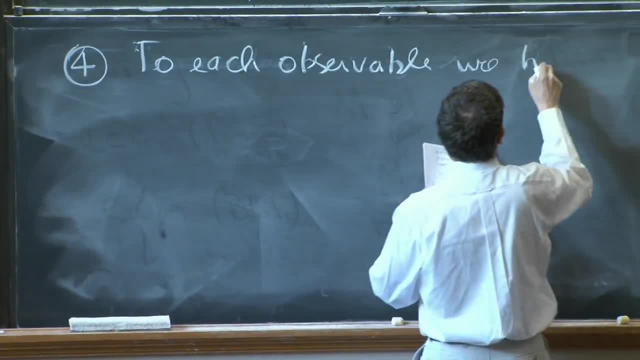 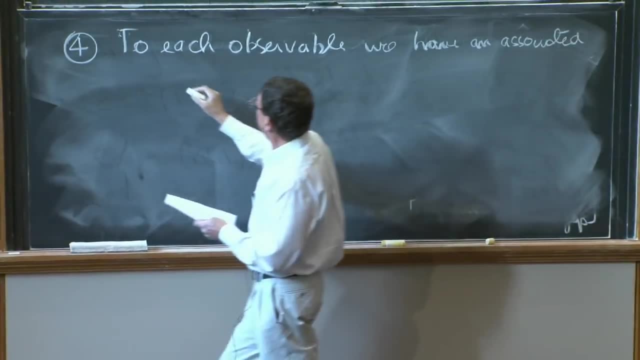 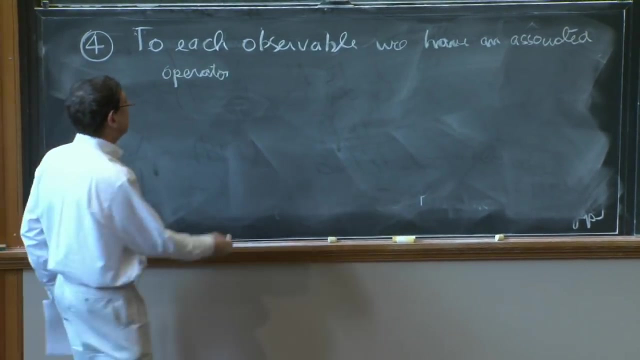 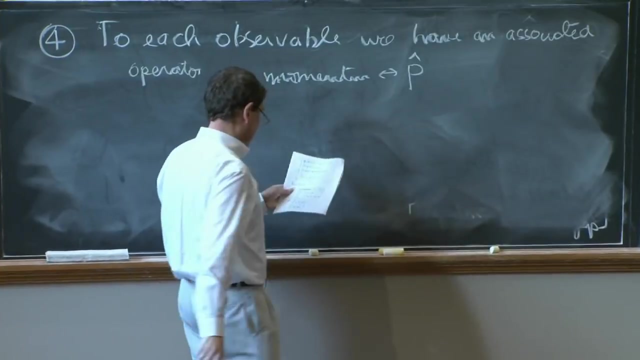 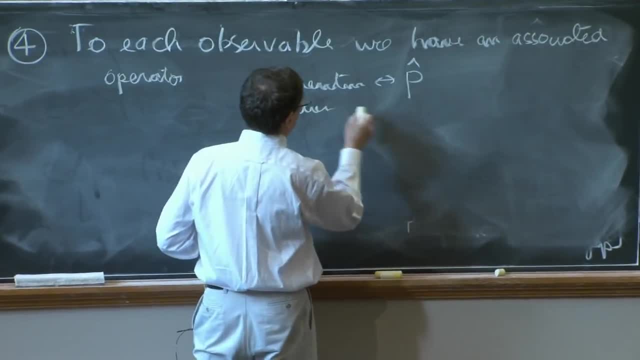 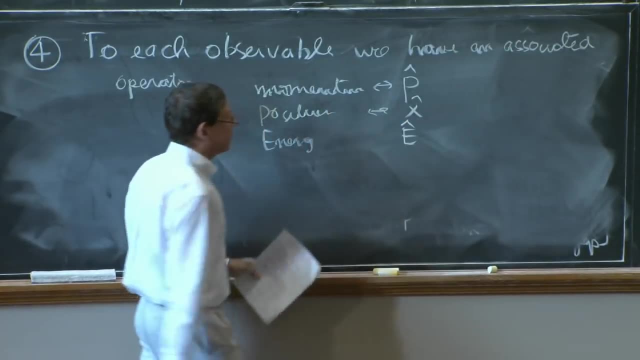 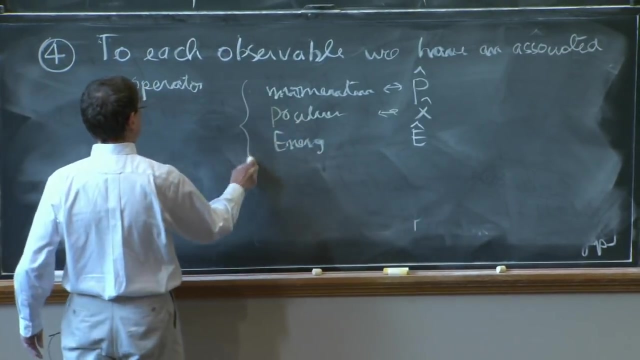 We have the disk. We have the disk And for energy we have the operator x hat And for energy we have the operator e hat. And these are examples of operators. Operators- Example: operator a hat. It can be any of those. 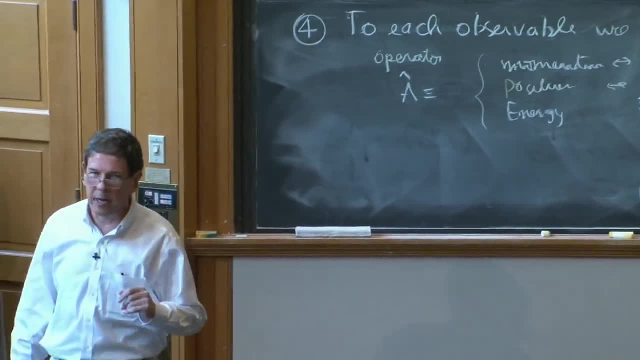 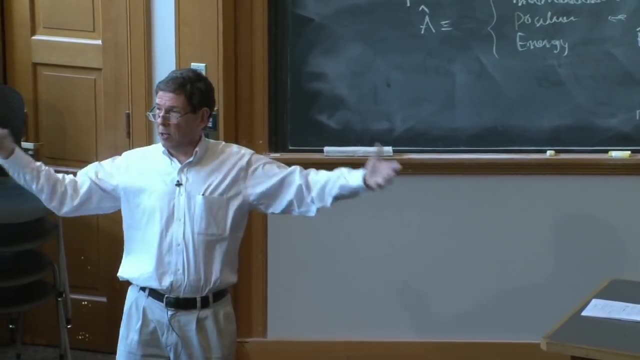 And there may be more observables depending on the system you're working in. On a line, there's not too many more observables at this moment. If you have a particle, in general you can have angular momentum. That's an interesting observable. 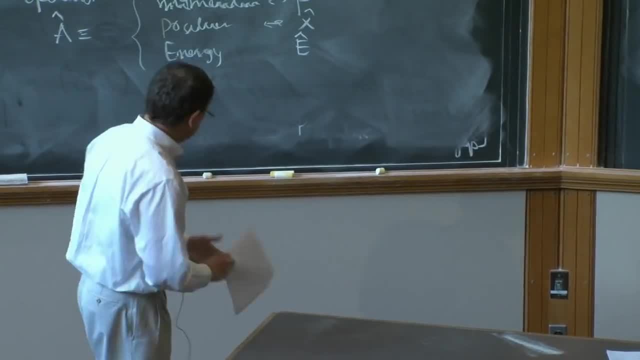 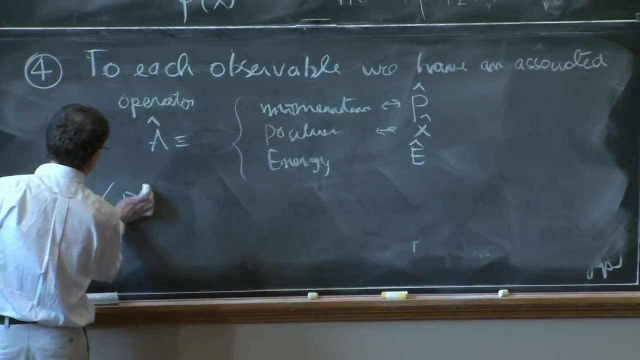 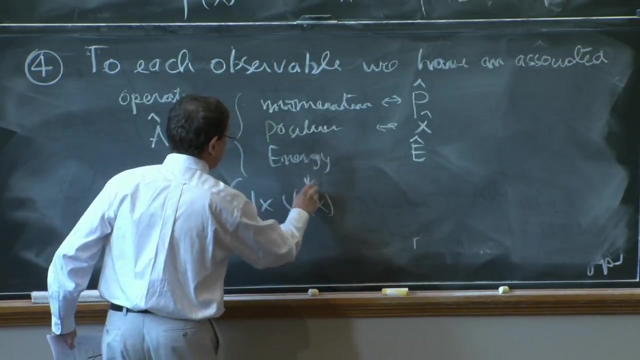 It can be others. So for any of those our definitions, just like we did for momentum, the expectation value of the operator is computed by doing what you did for momentum: You act with the operator, You act with the operator on the wave function here. 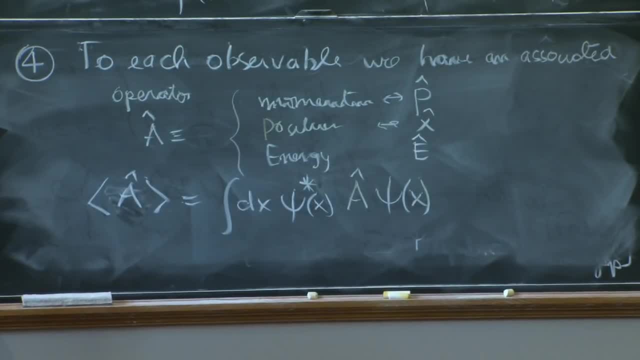 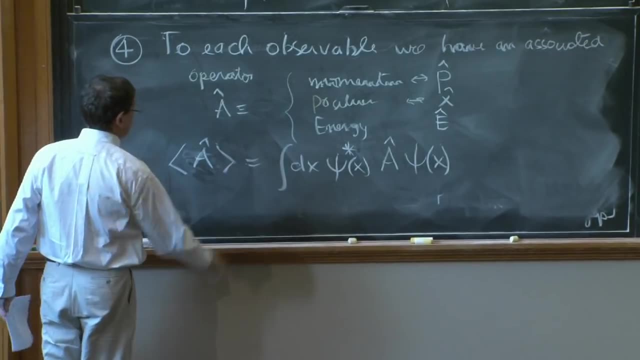 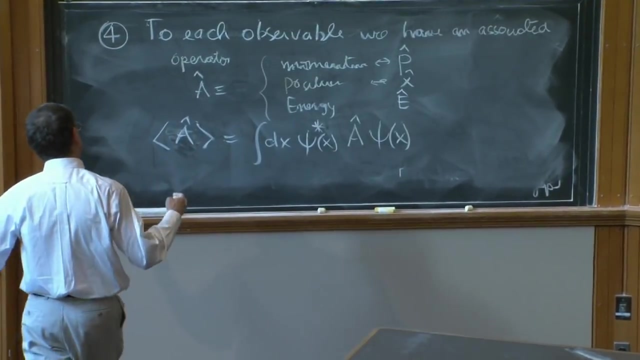 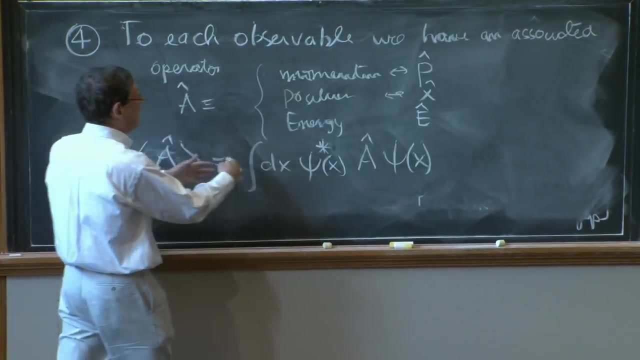 And multiply by the complex conjugate function And integrate, Just like you did for momentum. This is going to be the value that you expect After many trials on this wave function. you would expect that the measured value of this would exhibit the distribution which is expectation value. 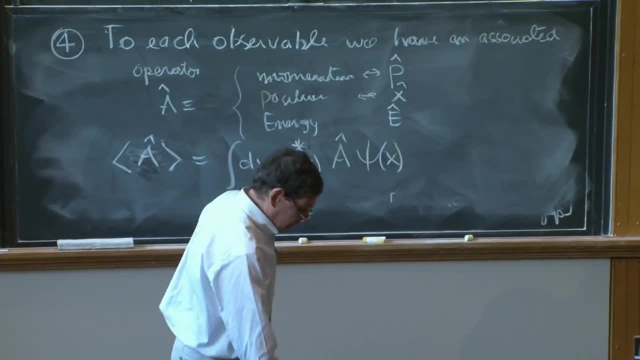 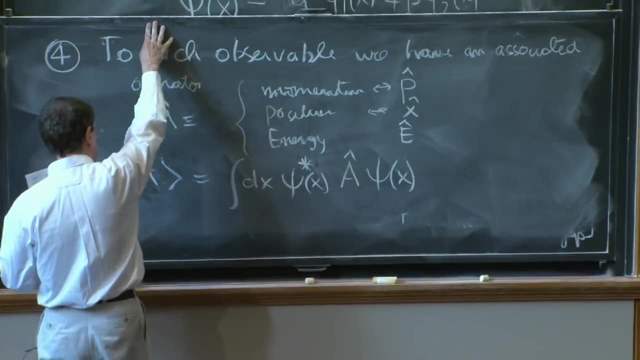 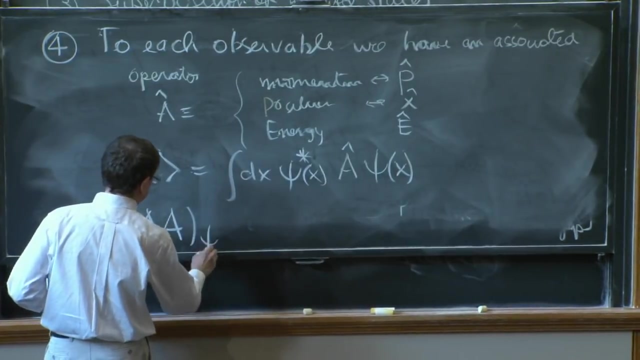 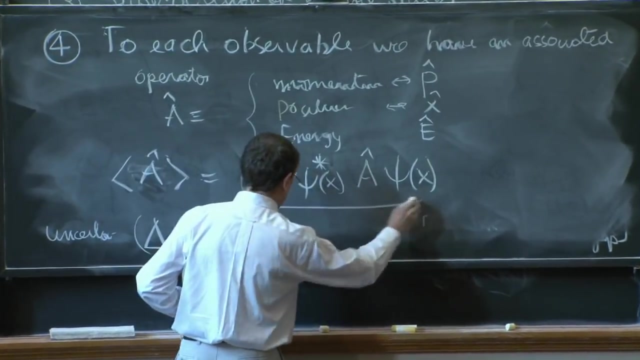 The mean is given by this. Now there are other definitions. One definition that already has been mentioned is that the uncertainty of the operator on the state psi. the uncertainty is computed by taking the square root of the expectation value of a squared. 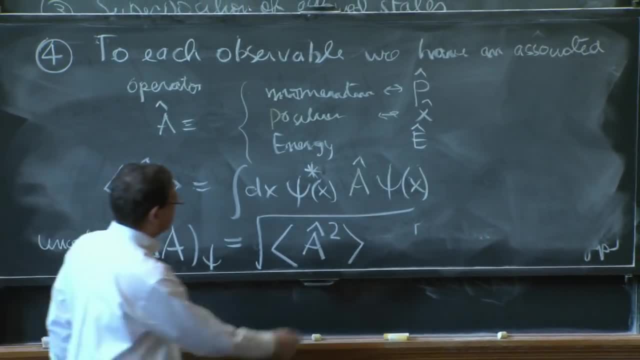 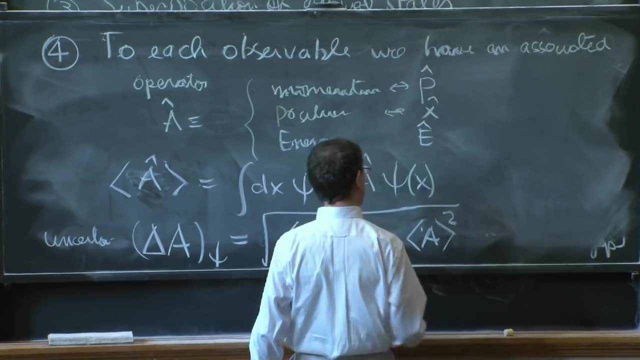 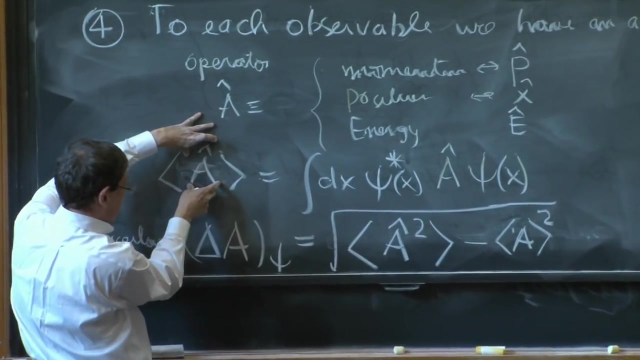 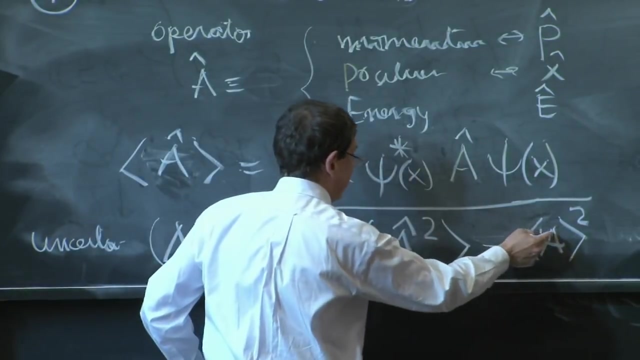 So that's minus the expectation value of a as a number squared, Now the expectation value of a squared. just simply, here instead of a you put a squared, So you put a squared here That, unless the function is very special, 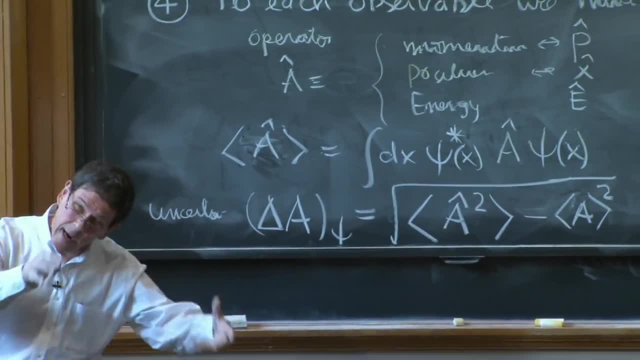 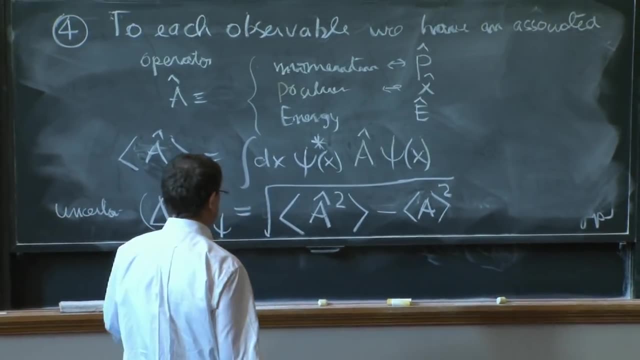 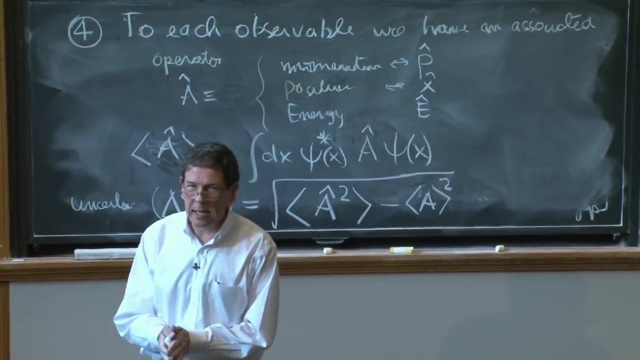 that's very different and always bigger than the expectation value of a squared. So this is a number and it's called the uncertainty And that's the uncertainty of the uncertainty principle. So for operators we need to have another observation that comes from matrices that is going to be crucial for us. 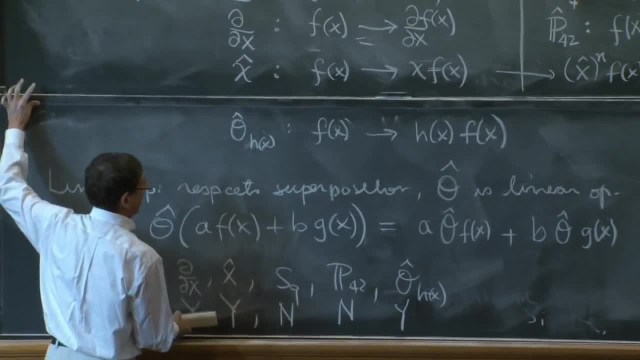 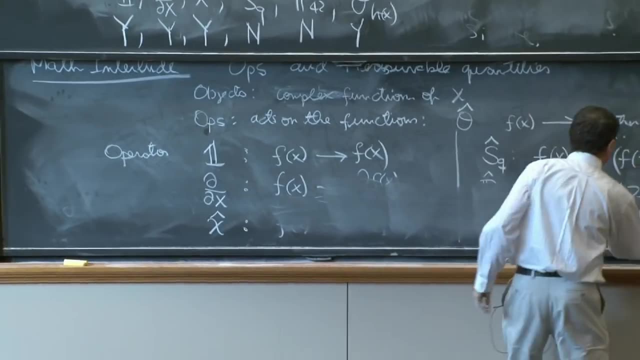 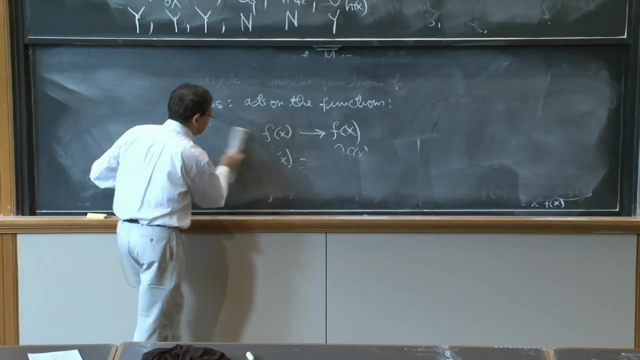 It's the observation that operators don't necessarily commute, And we'll do the most important example of that. So we'll try to see If the operators associated with momentum and position commute. And what do we mean by commute or don't commute. 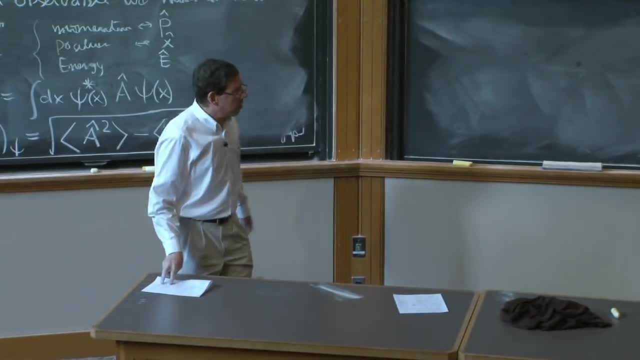 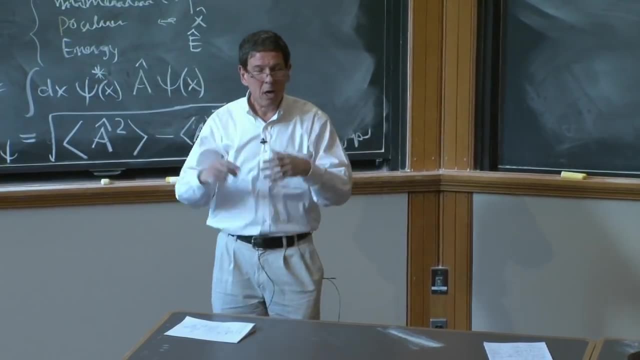 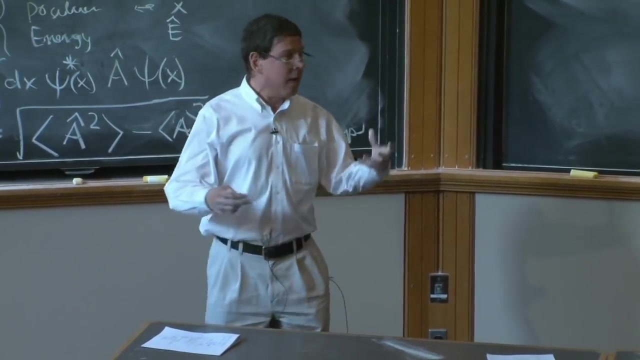 Whether the order of multiplication matters. Now we talked about matrices at the beginning And we said: matrices act on vectors to give you vectors. So do they commute? Well, matrices don't commute. The order matters for matrix multiplication. So these operators were in vectors. 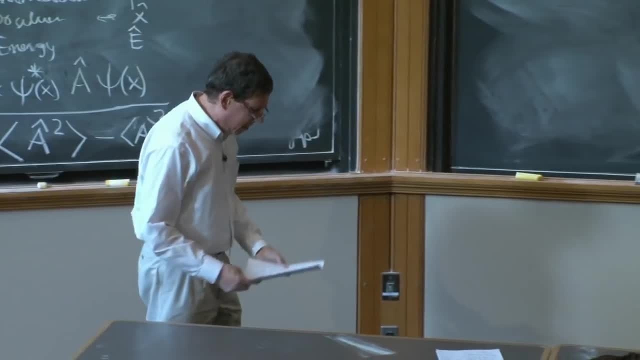 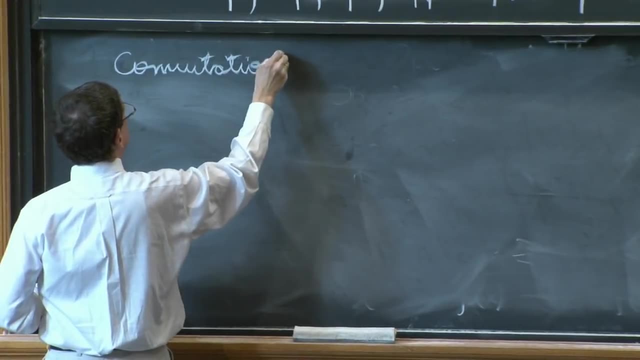 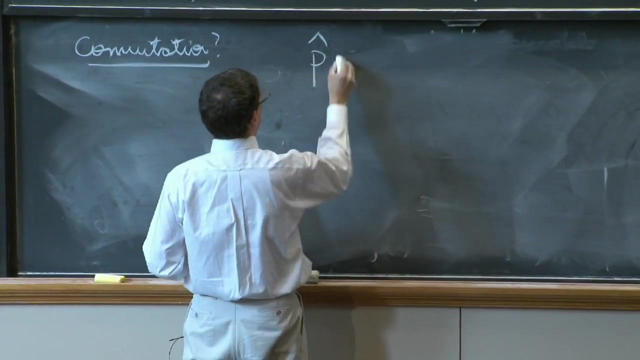 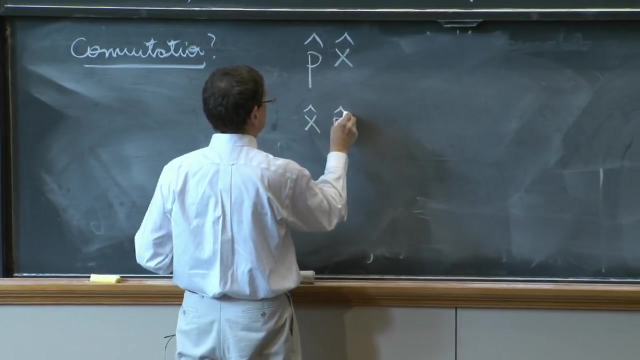 And what we're presenting here. for physics, the order does matter as well, So commutation. So let's try to see: if we compute the operator p and x hat, is it equal to the operator x hat times p? This is a very good question. 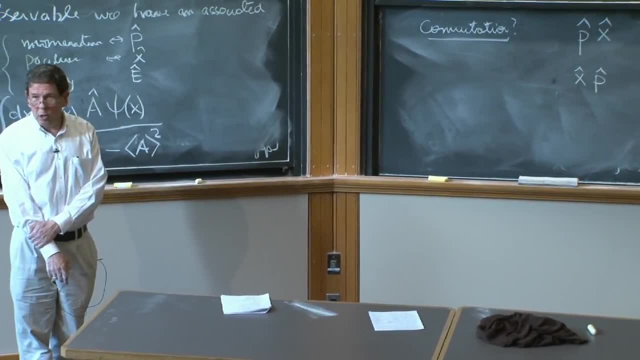 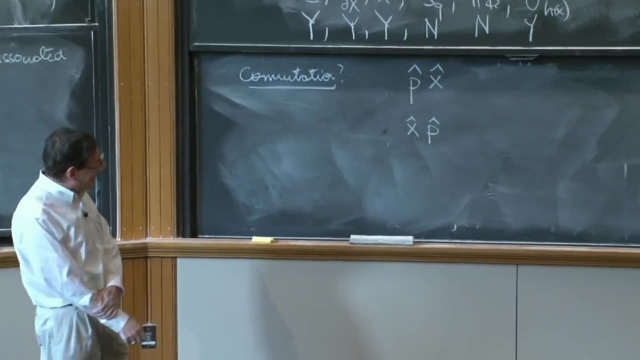 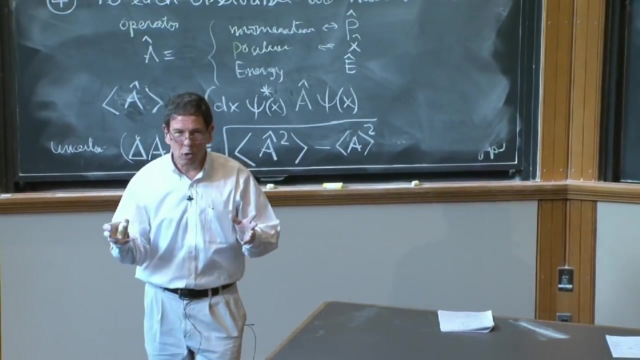 These are two operators, They're in the same line And we just want to know if the order matters or it doesn't matter. So how can I check it? I cannot just check it like this, Because operators are only clear what they do. 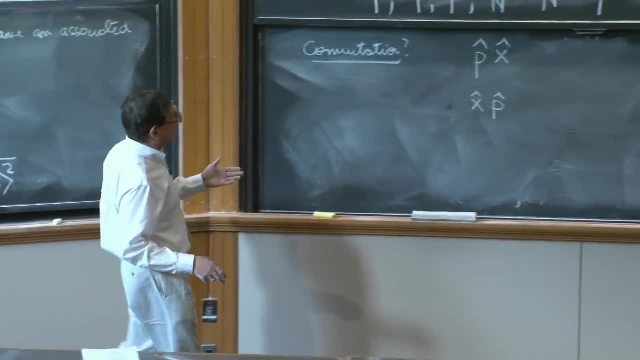 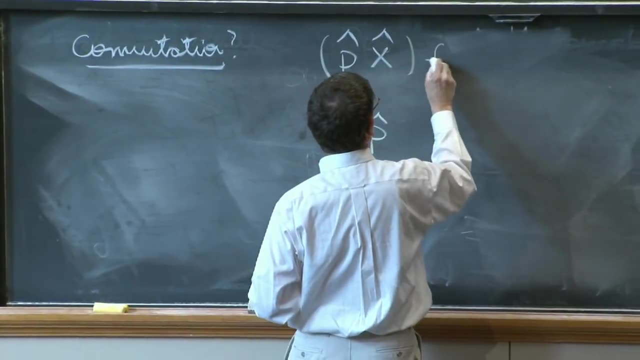 is when they act on functions. So the only thing that I can do is test if this thing acting on functions give the same. So I'm going to act with this on the function f of x And I'm going to act with this on the function f of x. 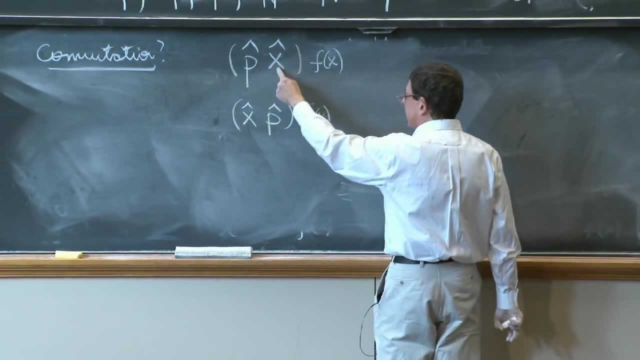 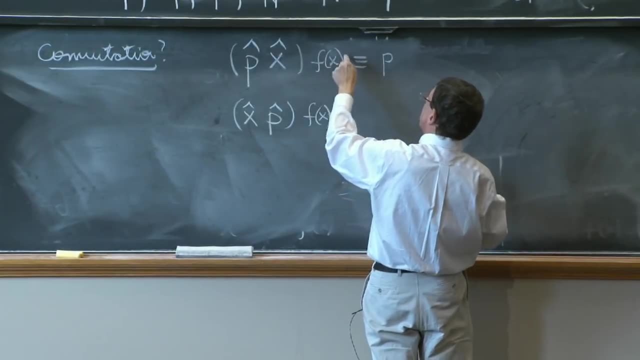 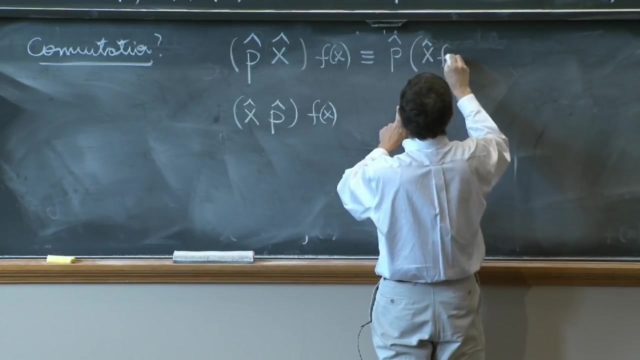 Now, what do I mean by acting with p times x? hat on the function f of x? This is, by definition: You act first with the operator that is next to the f and then with the other. So this is p hat on the function x hat times f of x. 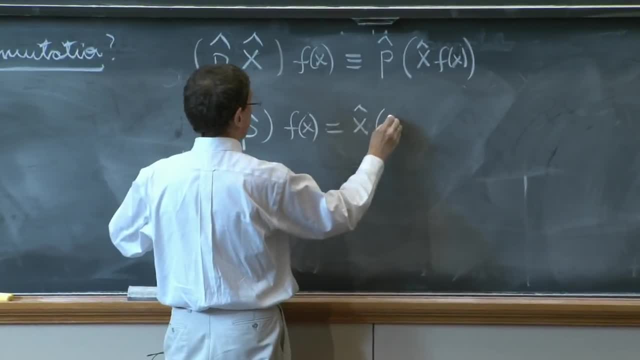 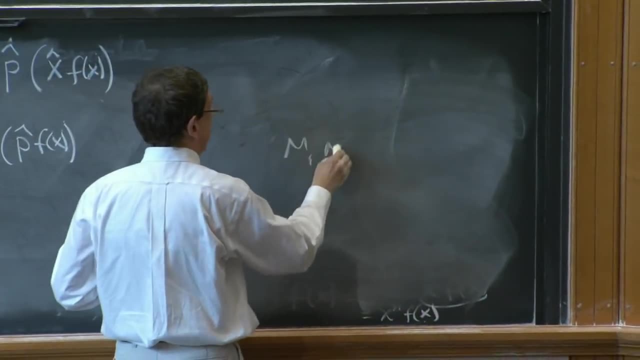 So here I would have. This is x hat on the function p hat f of x. See, if you have a series of matrices- m1, m2, m3, acting on a vector, what do you mean? 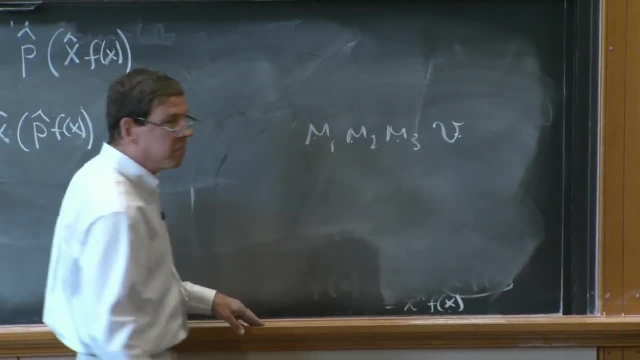 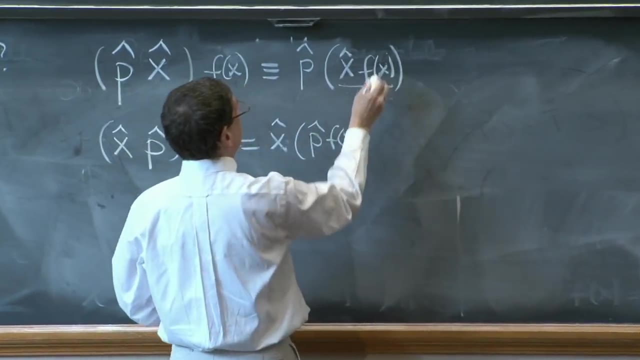 Act with this on the vector, then with this on the vector, then with this. That's multiplication. So we're doing that. So let's evaluate What is x operator on f of x. This is p hat on x times f of x. 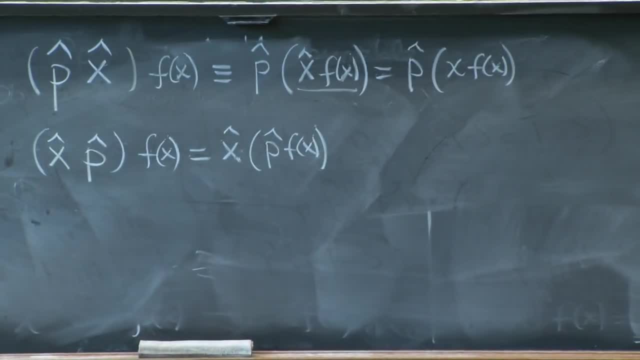 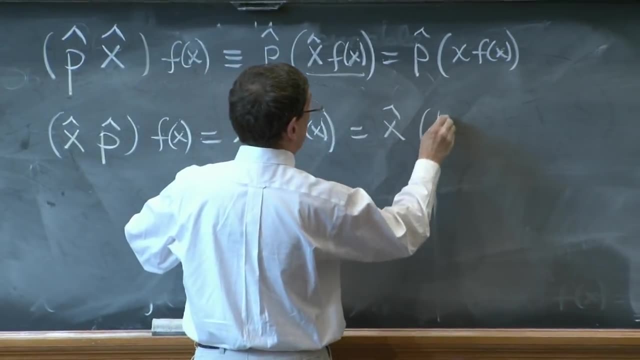 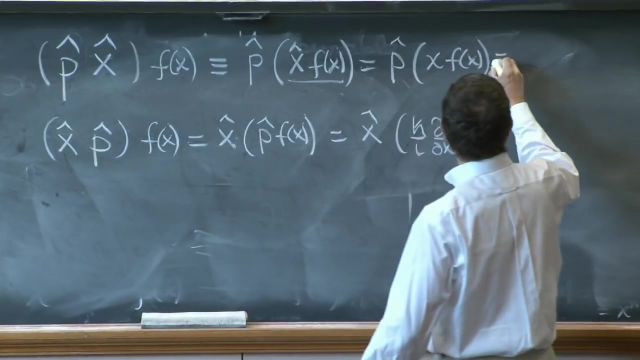 That's what the x operator on the function is Here. what is x hat? And now I have this. So I have here h over i d dx of f. Let's go one more step here. This is h over i d dx now of this function: x, f of x. 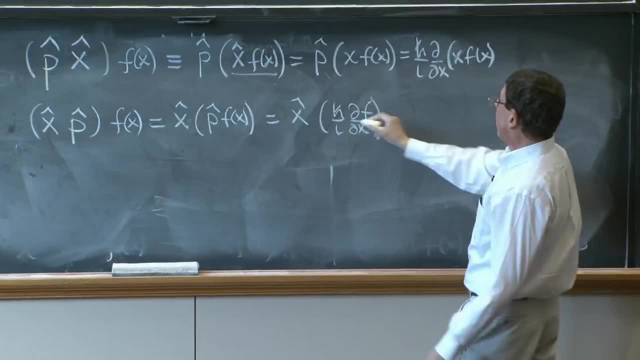 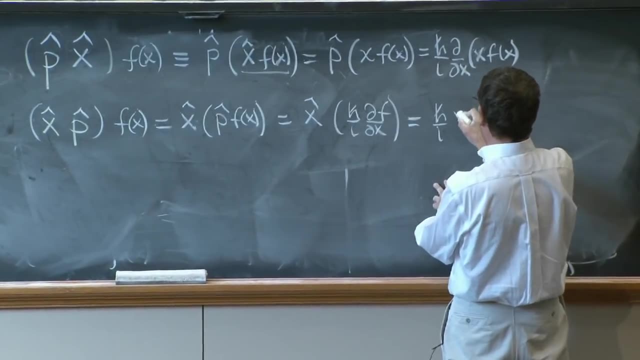 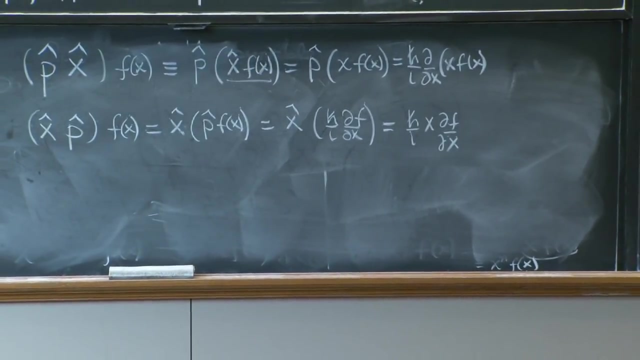 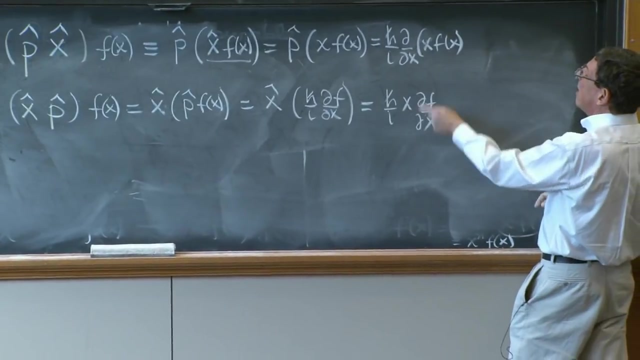 And here I have just h d of x. There, There, There, There, There, There. the x function times this function. So h over i x, df, dx. Well, are these the same? No, because this ddx here is not only acting on f, like here. 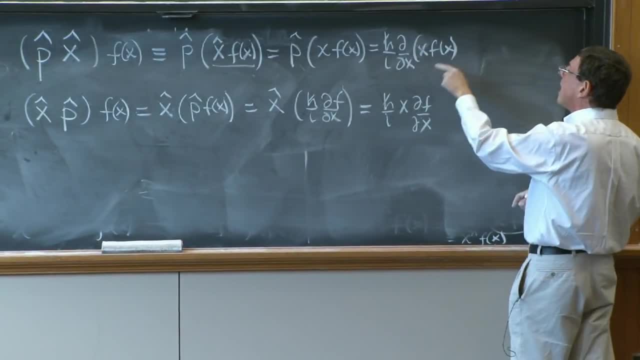 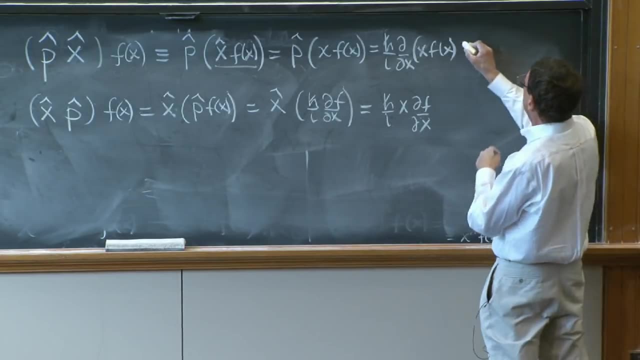 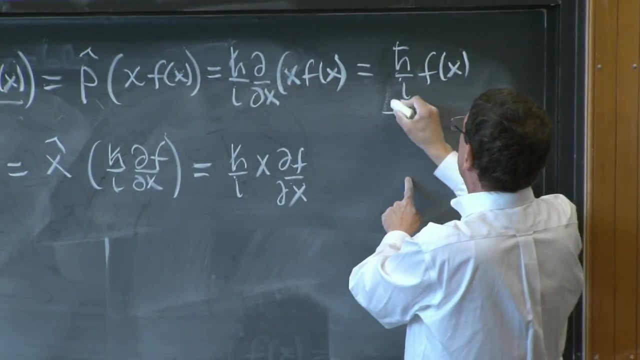 It's acting on the x. So this gives you two terms: one extra term when the ddx acts on the x, and then one term that is equal to this. So you don't get the same. So you get from here h over i, f of x when you act on the x. 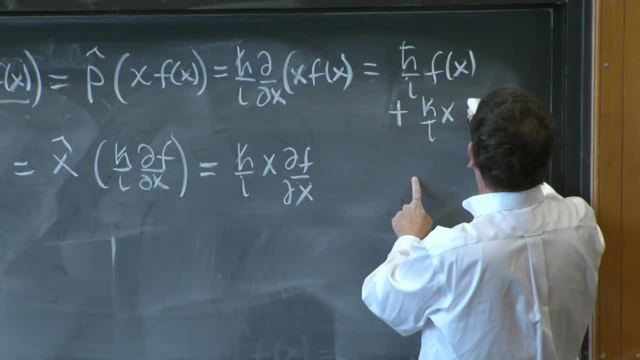 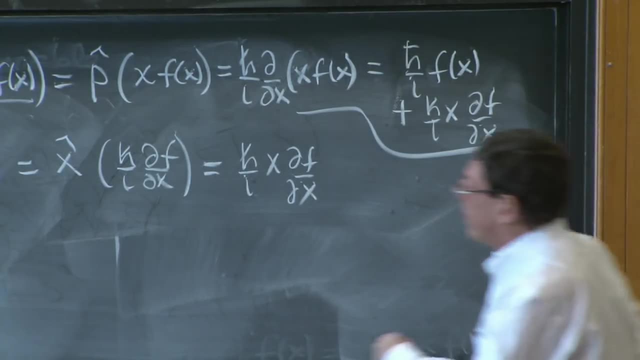 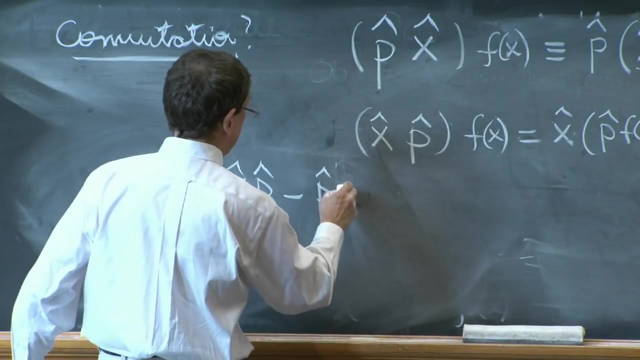 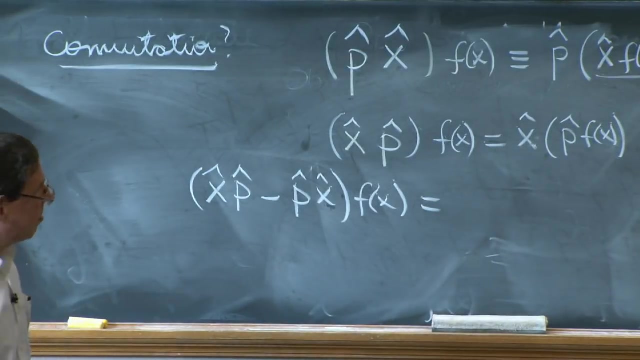 plus h over i, x, df, dx, So you don't get the same. So when I subtract them, so when I do xp minus px, acting on the function f of x, What do I get? Well, I put them in this order: x before the p. 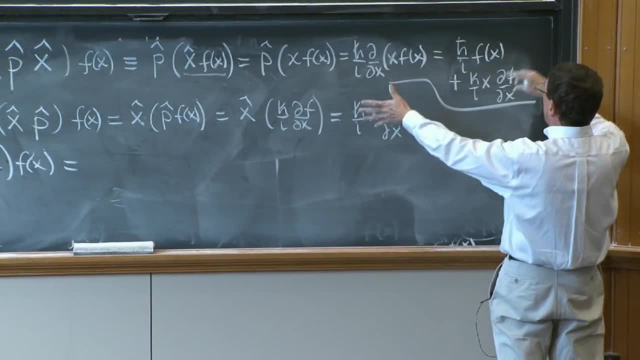 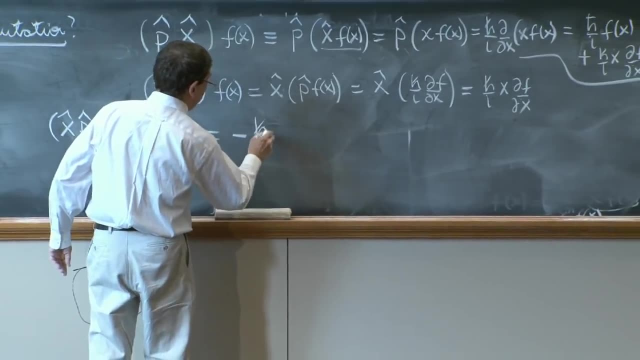 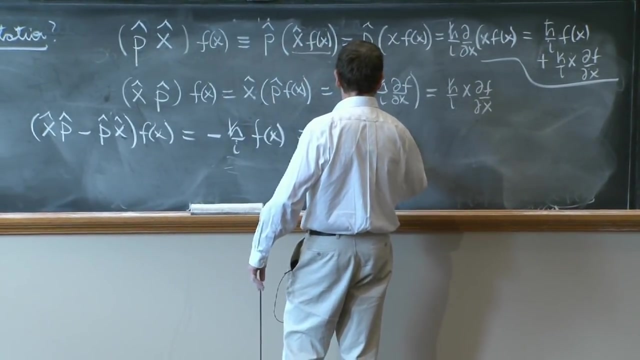 Doesn't matter which one you take, but many people like this: Well, this term's constant: I get minus this thing, So I get minus h over i f of x or ih bar f of x. Wow, You got something very strange. 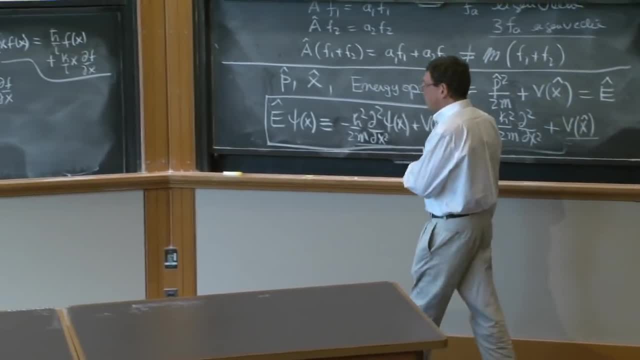 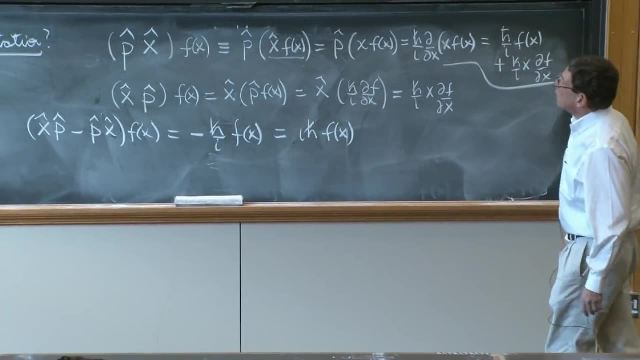 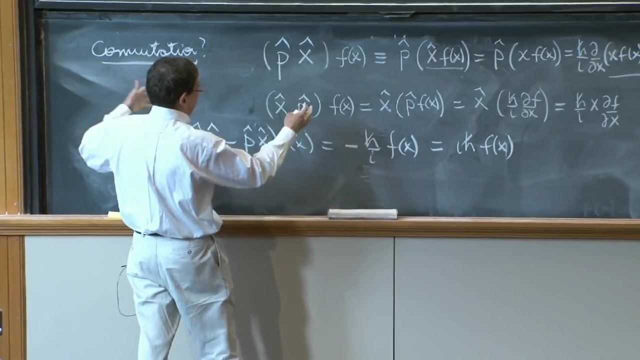 The x is equal to the x. The x times p minus p times x gives you a number, an imaginary number. even worse, times f of x. So from this we write the following. We say: look, operators are defined by the action on functions. 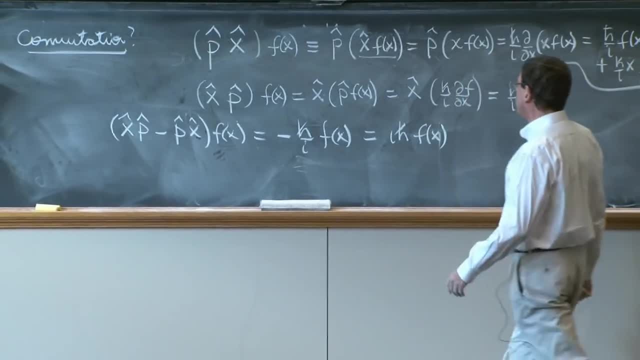 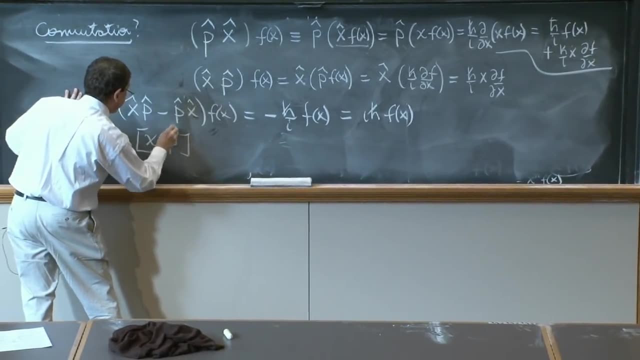 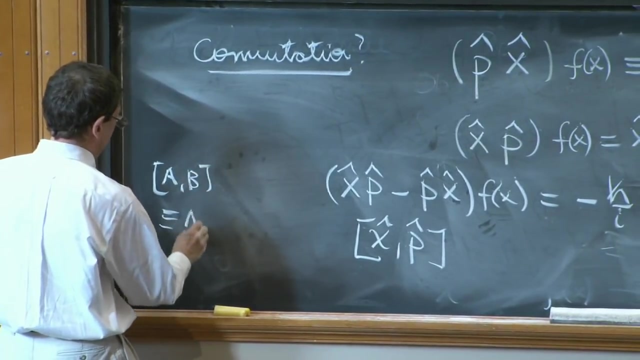 But for any function, the only effect of xp minus px, which we call the commutator of x with p, this definition, the bracket of two things of ab, is defined to be ab minus ba. It's called the commutator. 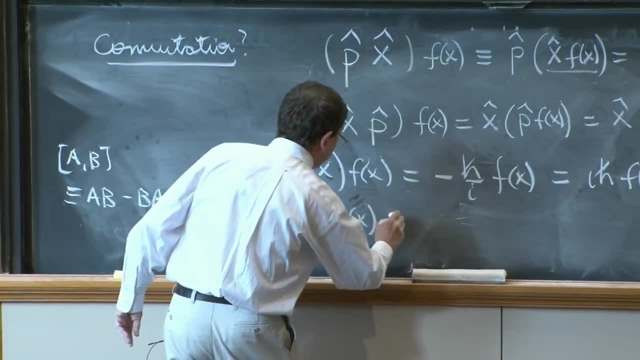 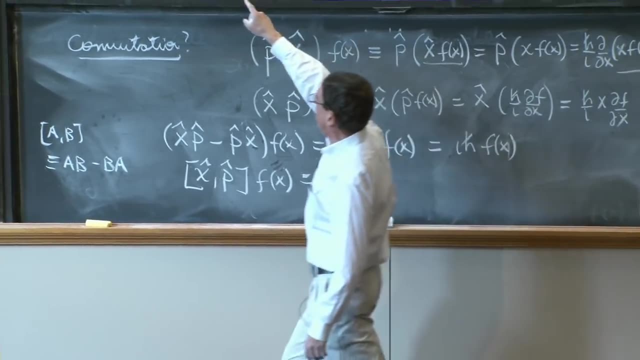 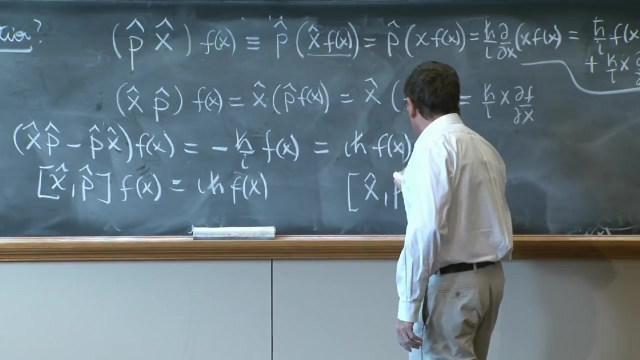 xp is an operator acting on f of x, gives you ih bar times f of x. So our kind of silly operator that does nothing has appeared here because I could now say that x hat with p is equal to i h bar times the unit operator. 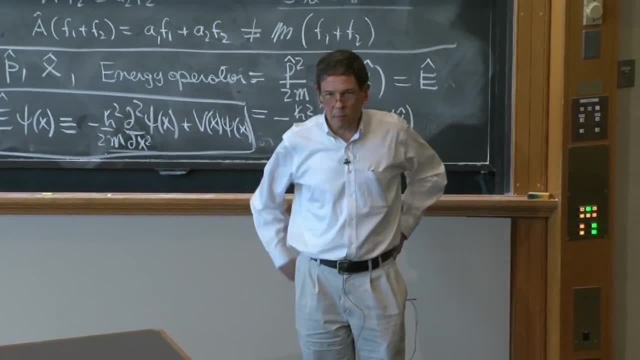 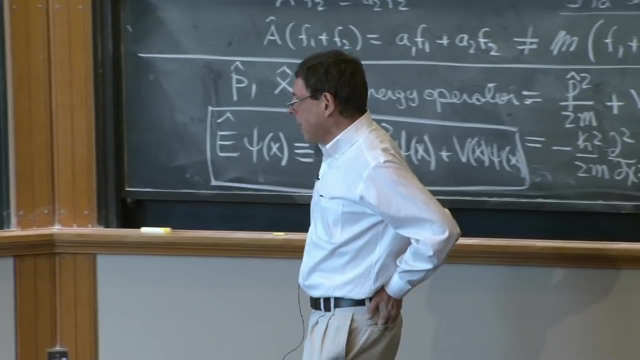 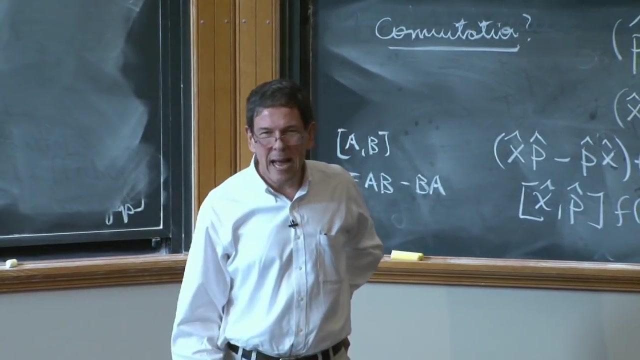 Apart from the Schrodinger equation, this is probably the most important equation in quantum mechanics. It's the fact that x and p are incompatible operators. as you will see later, They don't commute. Their order matters. What's going to mean is that when you measure 1, 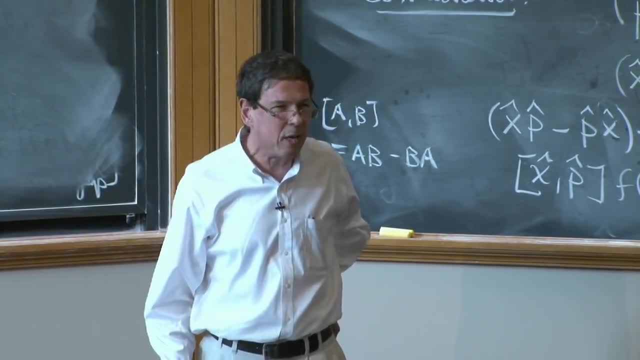 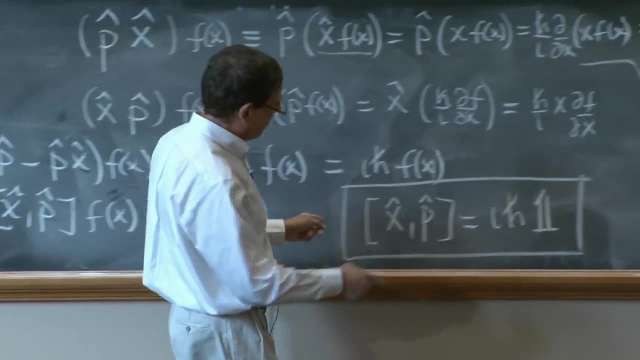 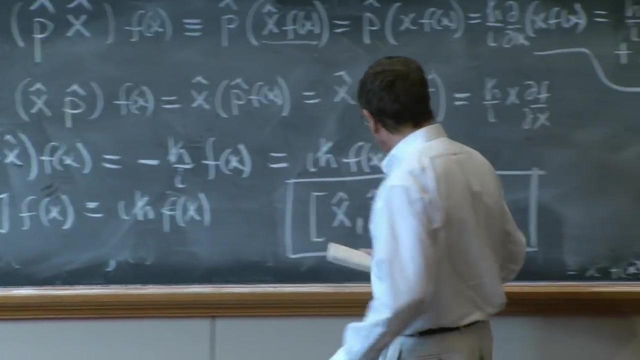 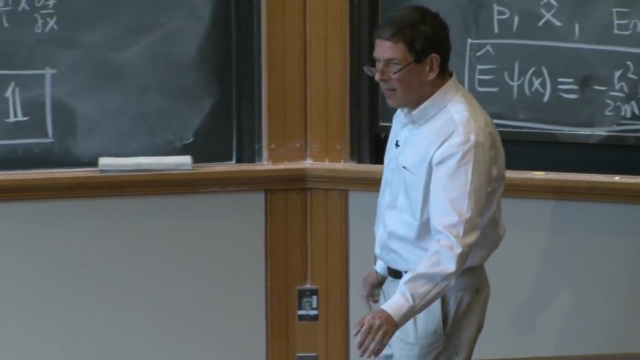 you have difficulties measuring, You have difficulties measuring the other. They interfere, They cannot be measured simultaneously. All those things are encapsulated in a very lovely mathematical formula which says that this is the way these operators work. Any questions? Yes, When x, the commutator of x and p, is itself an operator, right. 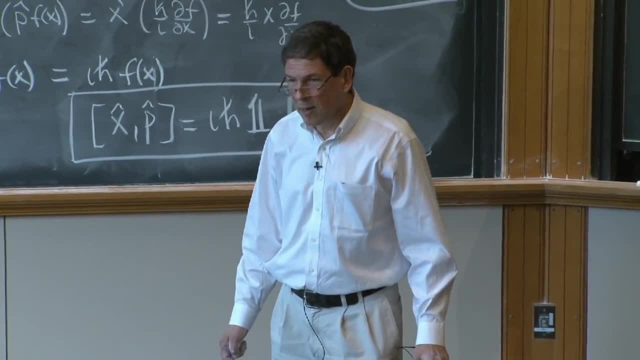 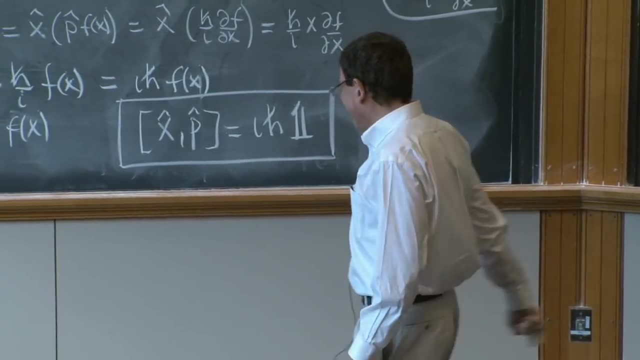 Right. Is that what we're saying When we had operators before? we can't simply just cancel the f of x. I mean, we're not really canceling it, but is it just because ih bar is the only eigenvalue of the operator? 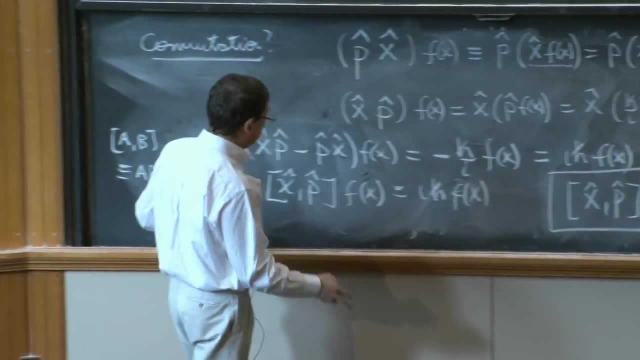 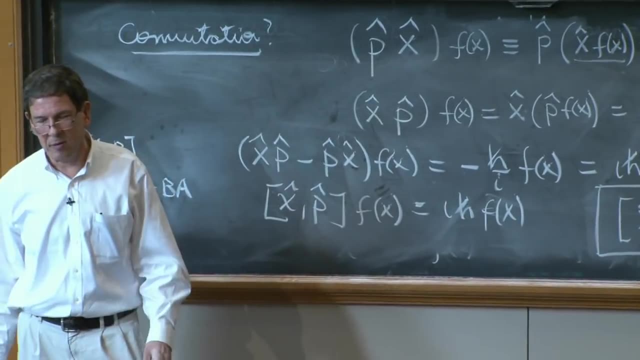 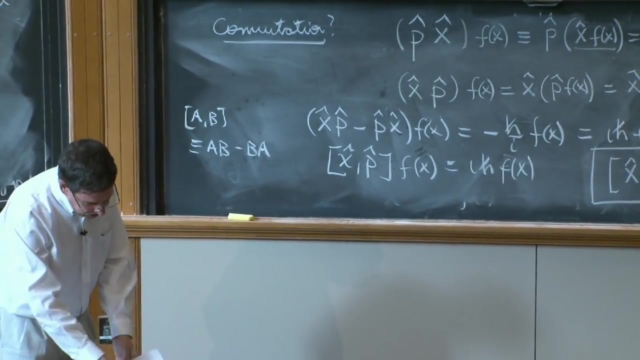 Well, basically, what we've shown by this calculation is that this operator, that this combination, is really the same as the identity operator. That's all. we've shown: that some particular combination is the identity operator. Now, this is very deep, this equation. 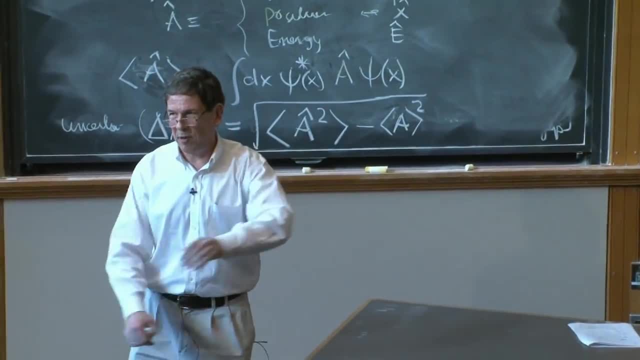 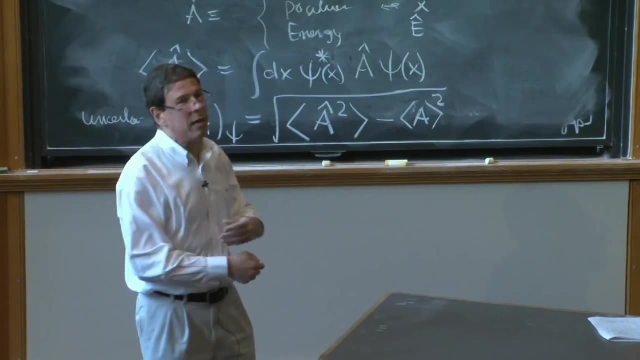 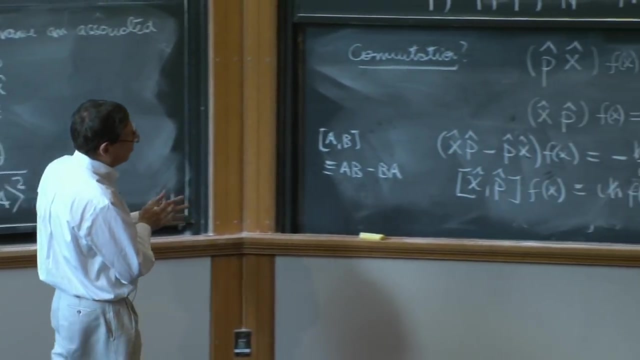 In fact, that's the way Heisenberg invented quantum mechanics. He called it matrix mechanics because he knew that operators were related to matrices. It's a beautiful story how he came up with this idea. It's very different from what we're doing today. 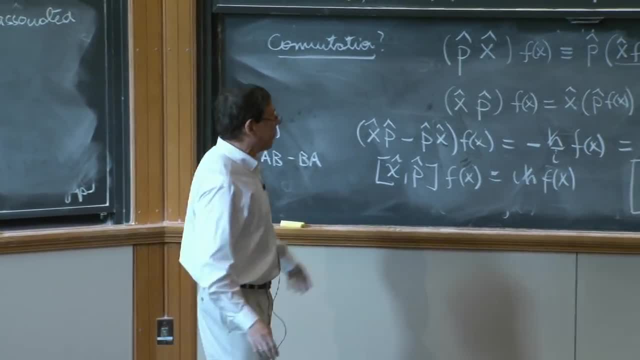 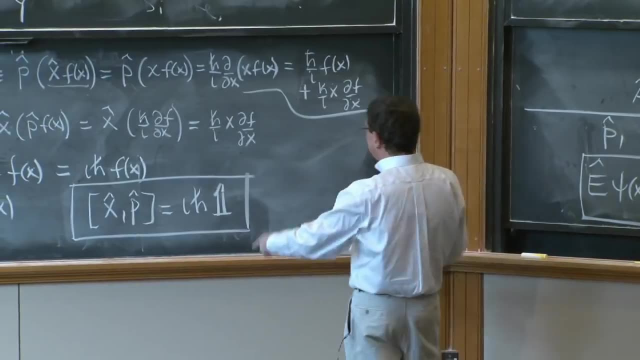 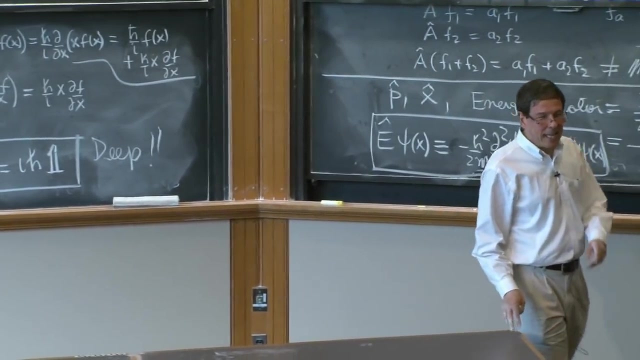 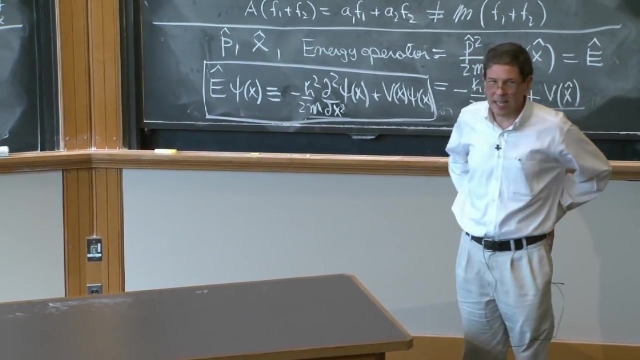 that we're going to follow Schrodinger today, But it's interesting Now. basically, his analysis led very quickly to this idea And this is deep. Why is it deep? Depends who you ask. If you ask a mathematician, they would probably. 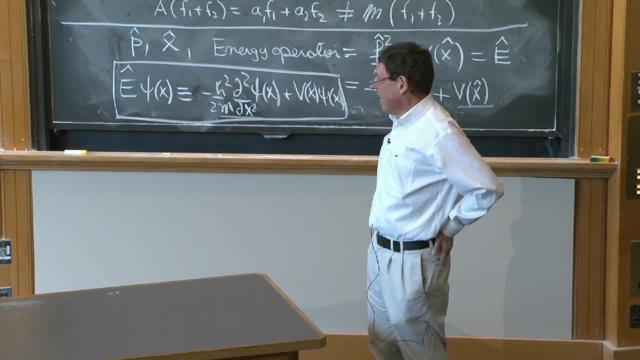 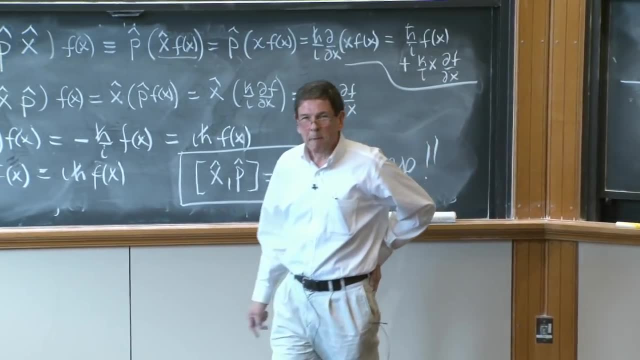 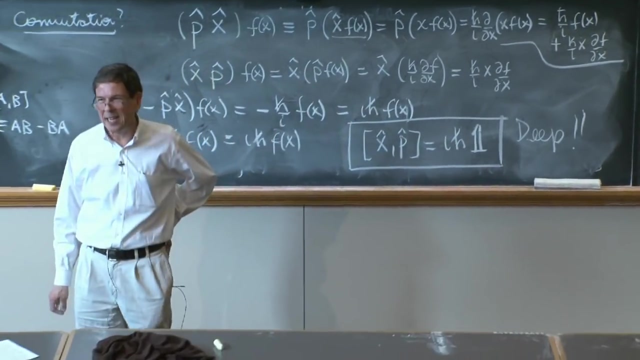 tell you, this equation is not deep. This is a scary equation. And why is it scary? Why? Why? Because whenever mathematicians see operators, they want to write matrices. So the mathematician is showing this equation. We'll say, OK, let me try to figure out. 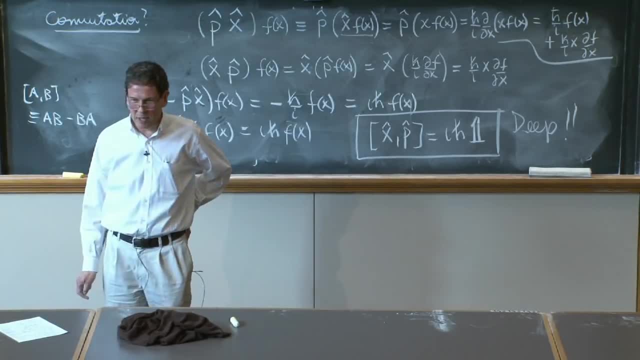 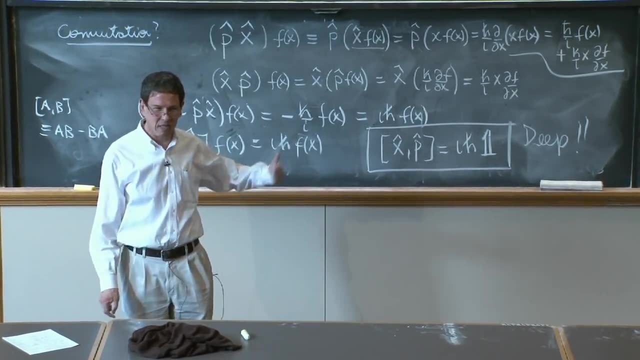 which matrices you're talking about. And this mathematician will start doing calculations with 2 by 2 matrices And we'll say: no, I can't find 2 by 2 matrices that behave like these operators. I can't find 3 by 3 matrices. 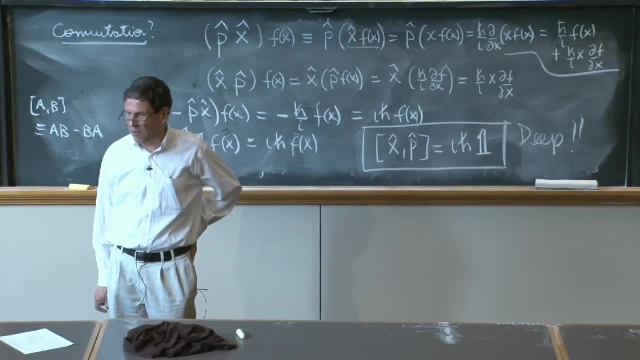 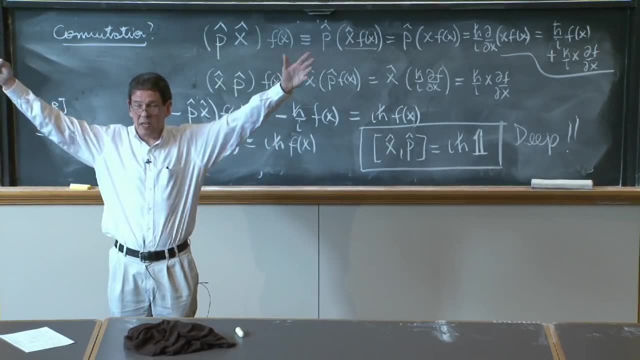 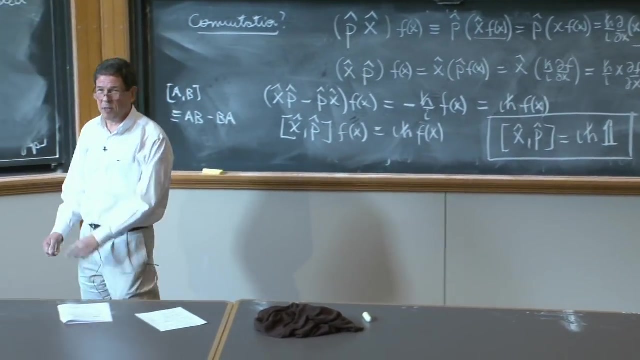 I can't find 3 matrices either, and 4 by 4, and 5 by 5. And in fact no matrix really can do that, except if the matrix is infinite, dimensional, infinite by infinite matrices. So that's why it's very hard for a mathematician. 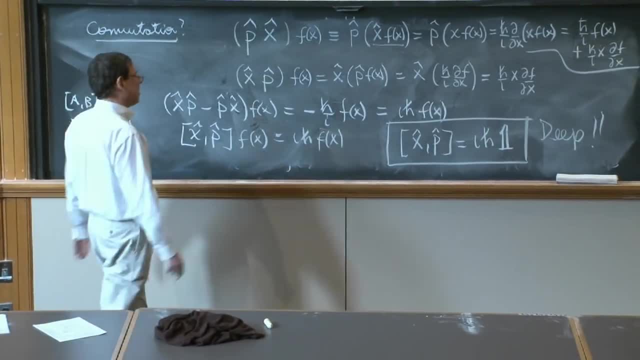 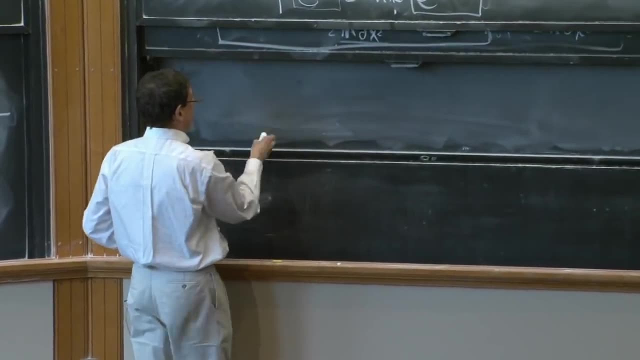 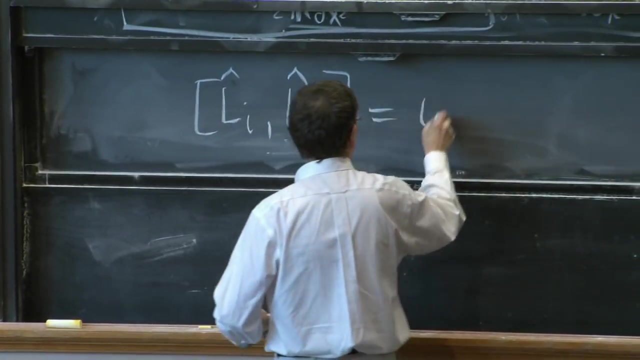 You know this is the beginning of quantum mechanics. This looks like a trivial equation And mathematicians get scared by it. You show them. for physicists they're going to be angular momentum. The operators are like this and they're complicated. 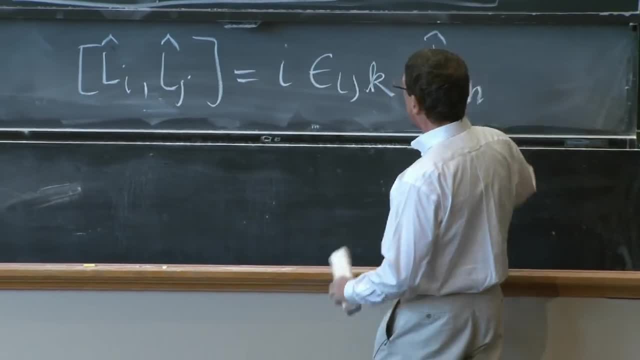 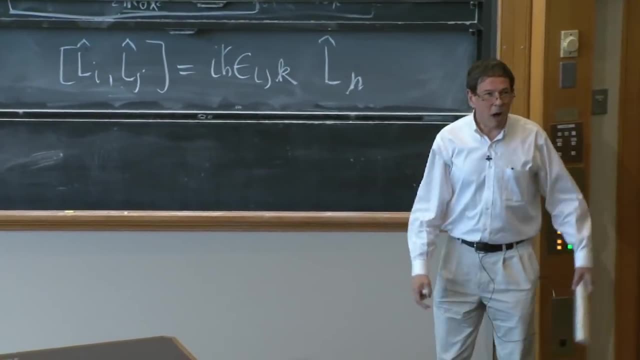 e to the i, j, k, l, k. The three components of angular momentum have this commutation relation and h bar here as well. Complicated Three operators. They mix with each other. Show it to a mathematician and it starts laughing at you. 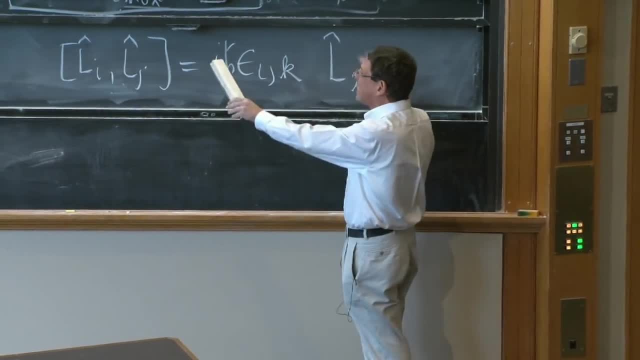 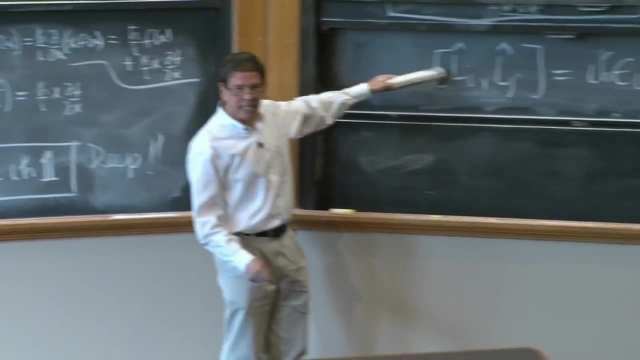 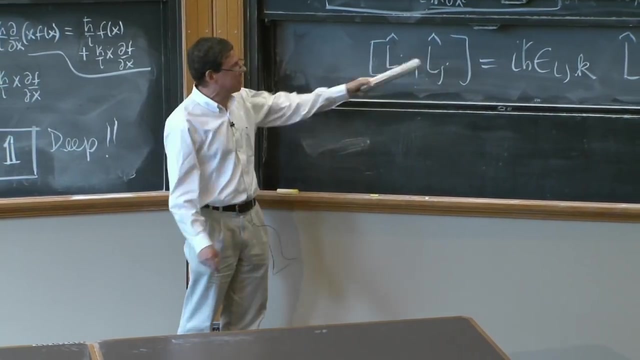 This is the simplest case. This is easy, This is complicated. It's very strange, But the reason this is easy and the mathematician goes and after five minutes comes to you with 3 by 3 matrices. that satisfies this relation. 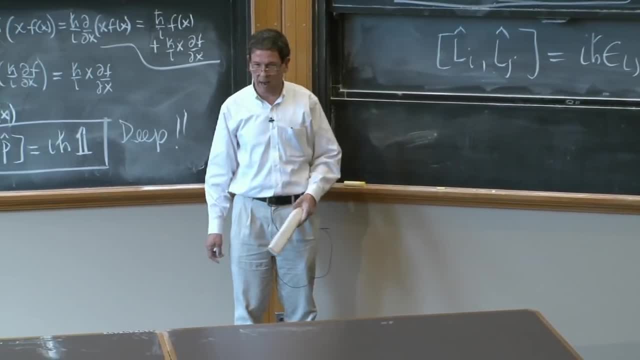 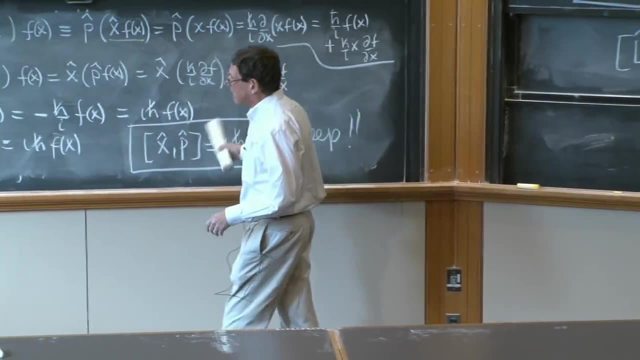 And here there weren't, And 4 by 4 that satisfy, and 5 by 5, and 2 by 2, and all of them. You can calculate all of them for you, But this one needs infinite dimensional matrices. 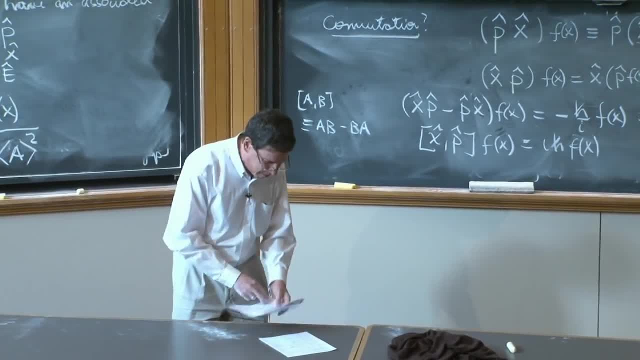 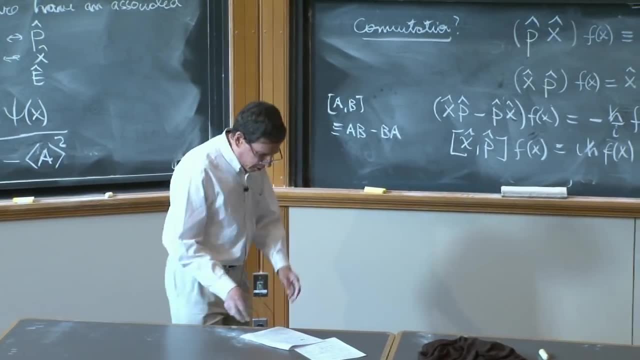 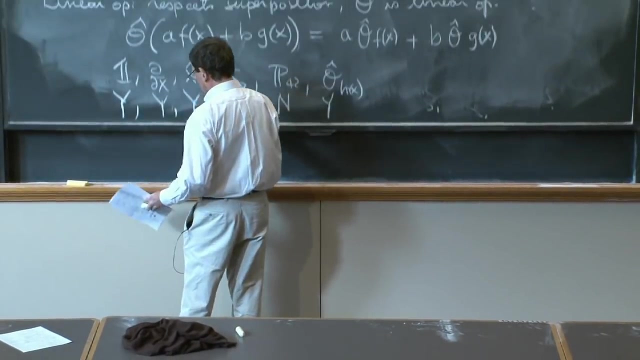 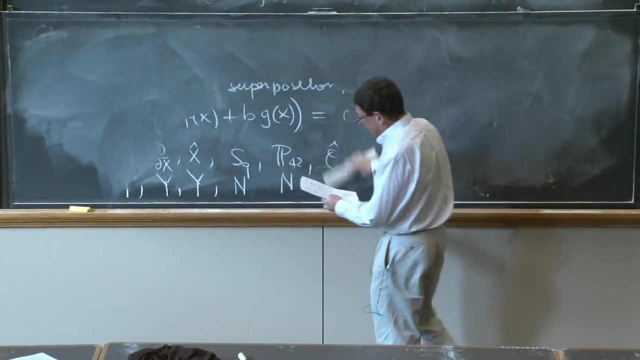 and it's very surprising, very interesting and very deep. All right, So we move on a little bit more to the other observable. So after this we have more general observable, So let's talk a little about them. That's another postulate of quantum mechanics. 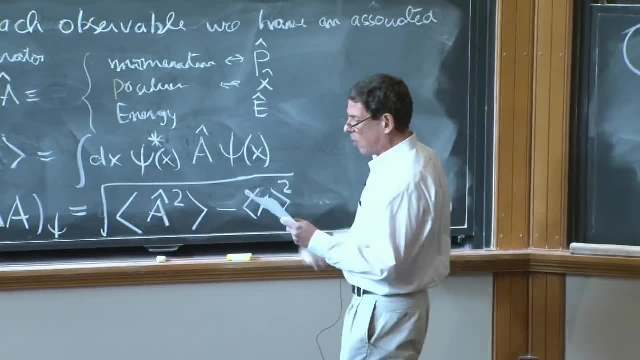 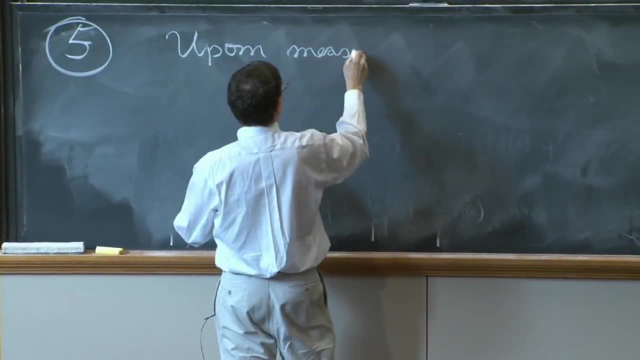 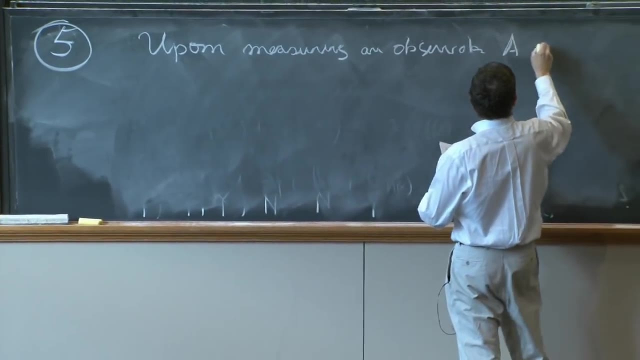 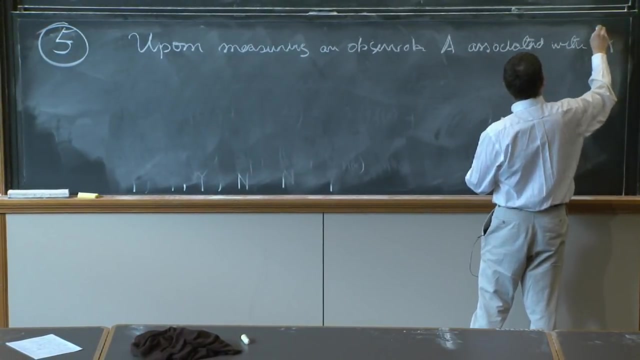 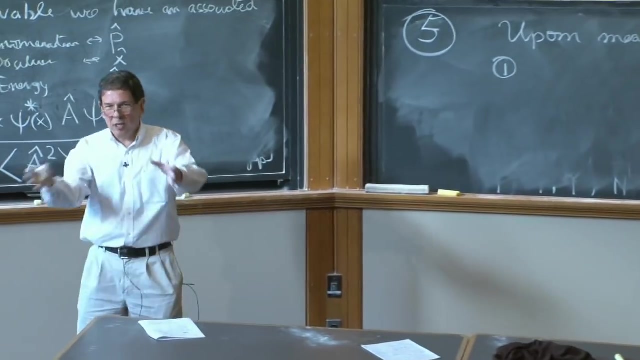 that continues with this one Postulate number five. So what? This is it? Once you measure, upon measuring an observable, A associated with the operator, A hat, two things happen. You measure this quantity, That could be momentum, could be energy, could be position. 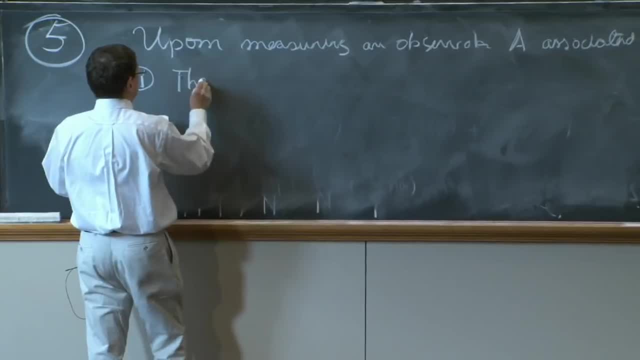 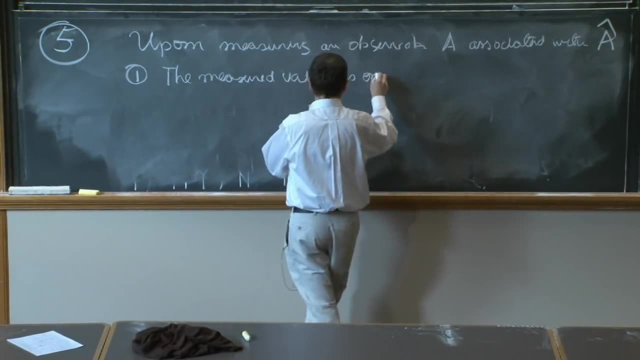 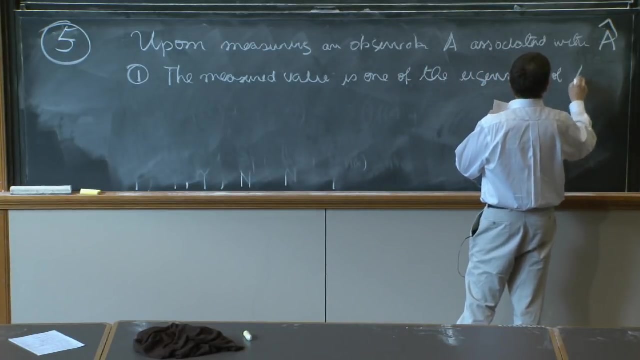 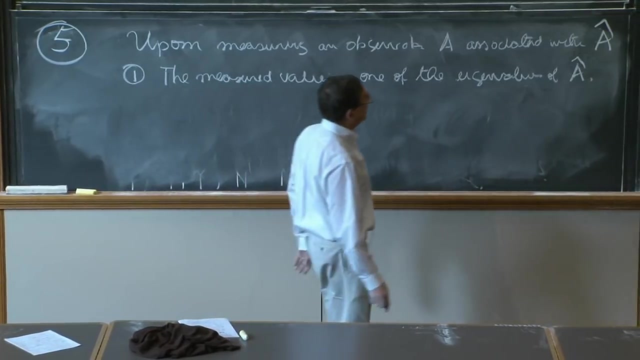 You name it. The measured value must be a number. It's one of the eigenvalues of A hat. So actually those eigenvalues. remember the definition of the eigenvalues. it's there. I said many, but whenever you measure, 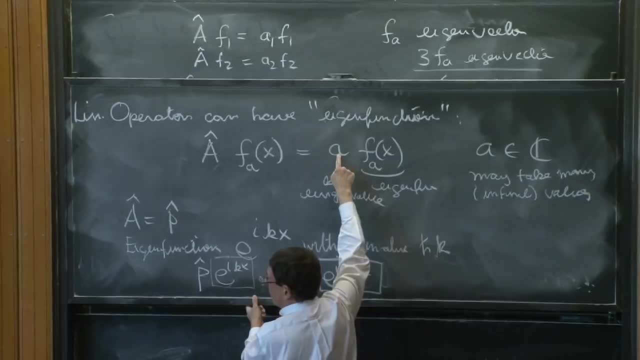 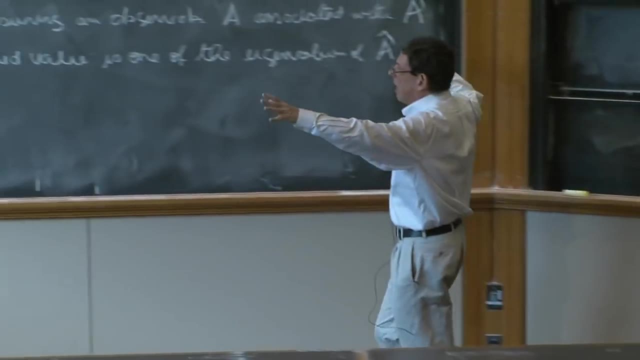 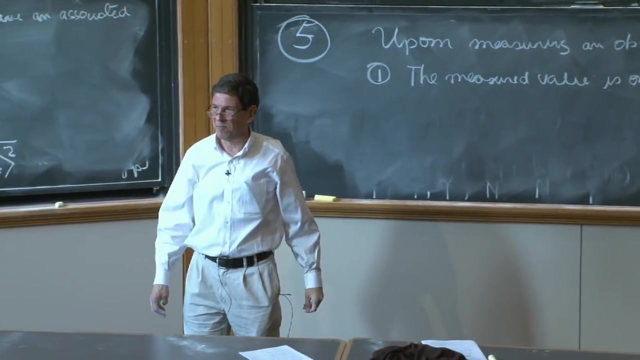 the only possibility is that you get this number, So you measure the momentum. you must get this hk, for example, So observables. we have an associated operator and the measured values are the eigenvalues. Now, these eigenvalues in order to be observable. 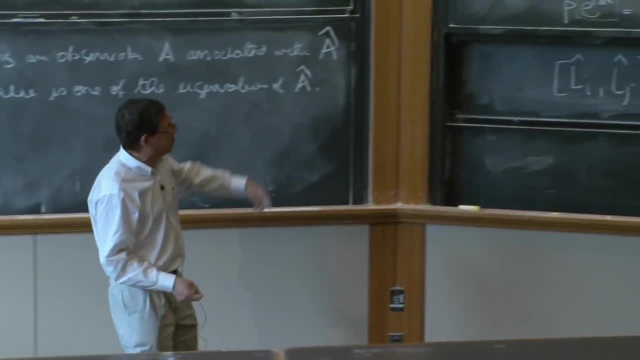 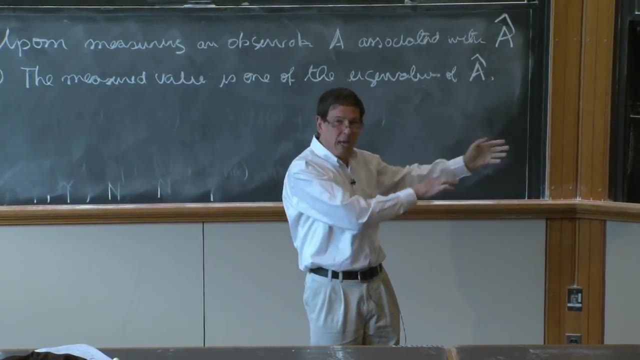 they should be real numbers And we said, oh, they can be complex. Well, we will limit the kind of observables to things that have real eigenvalues, And these are going to be called later on, Hermitian operators. 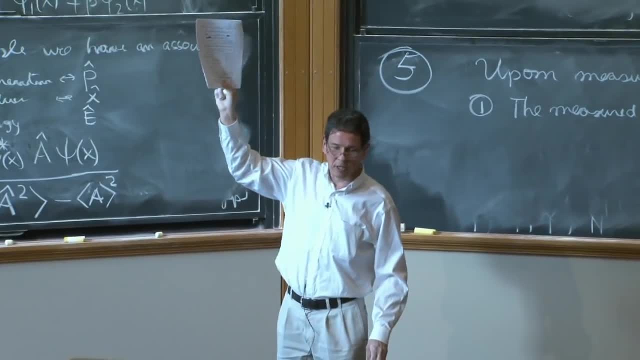 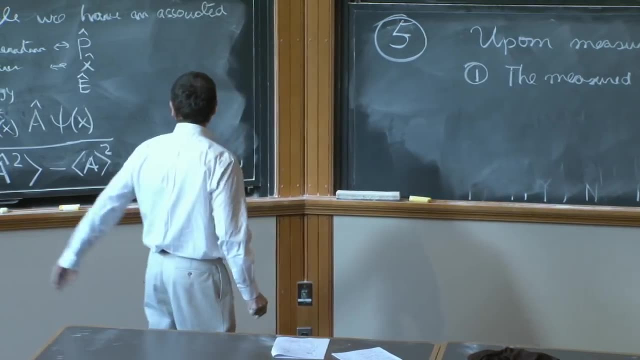 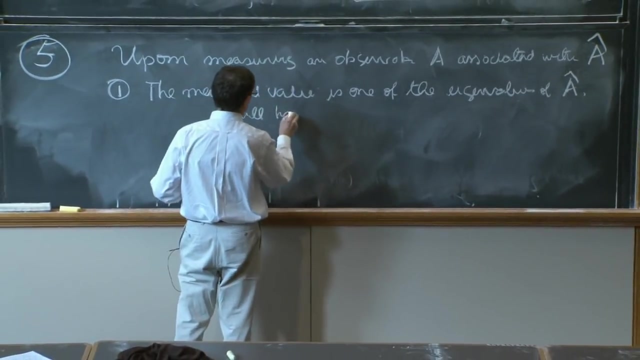 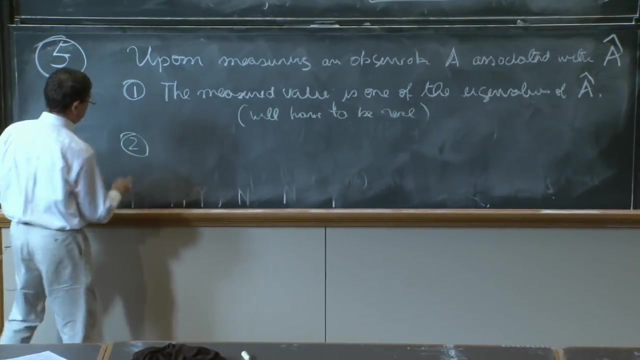 At this moment, the notes say: don't mention them, You're going to get them confused. So, anyway, special operators that have real eigenvalues, And so we'll mention here. they will have to be real, Have to be real. And then the second one, which is an even stranger thing: that 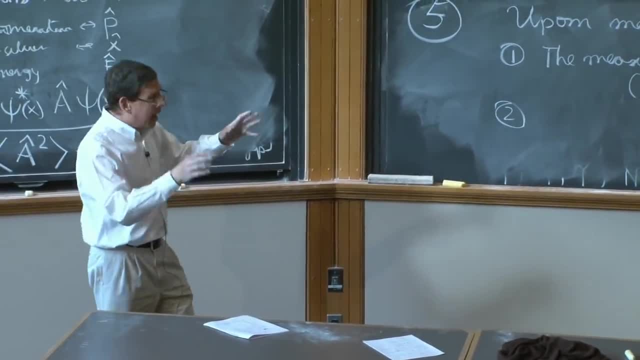 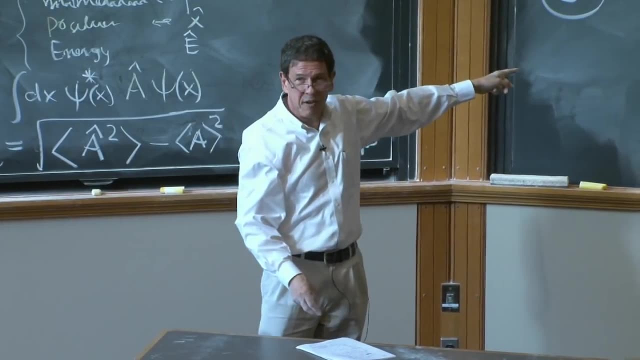 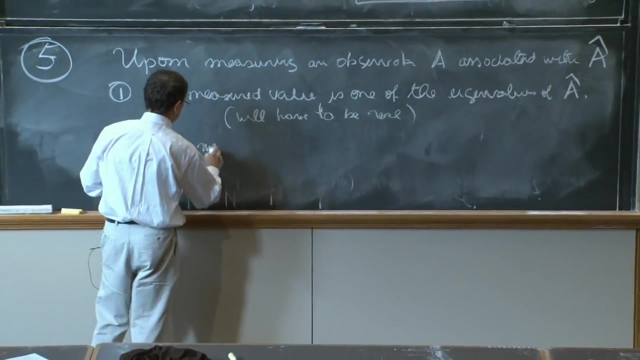 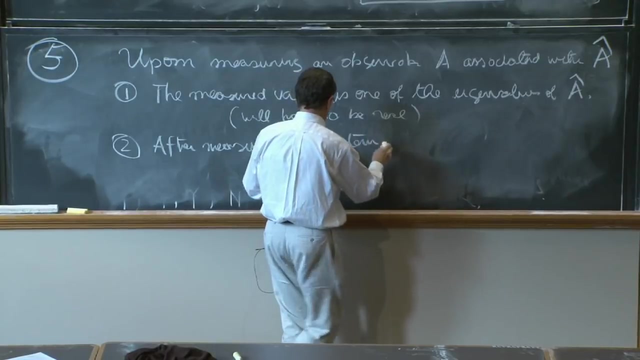 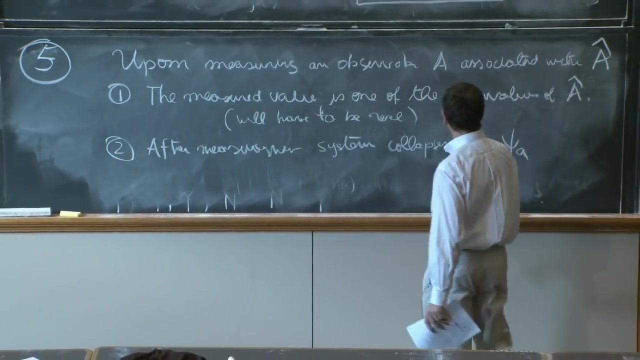 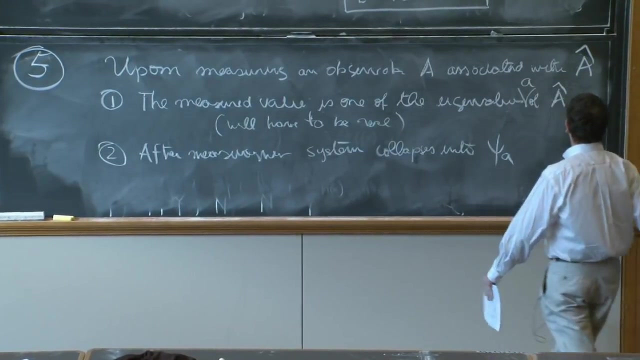 happens is something you've already seen in examples. After you measure, the whole wave function goes into the state, which is the eigenfunction of the operator. So after measurement, Measurement system collapses into psi A, The measured value is one of the eigenvalues A of A. 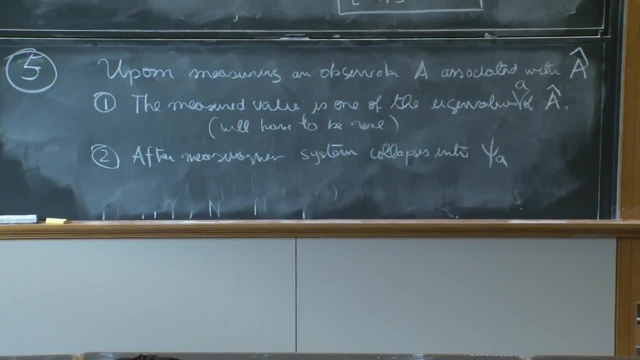 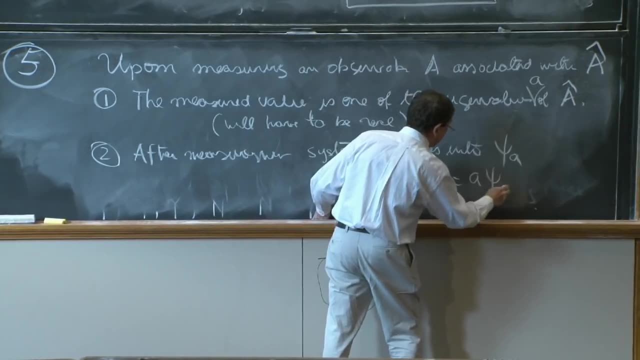 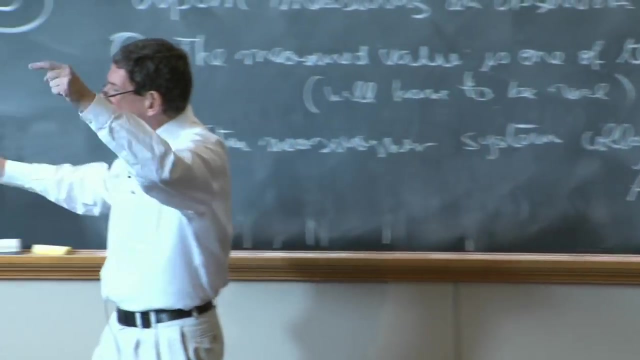 And the system collapses into psi A. So psi A is such that A hat psi A is A psi A. So this is the eigenvector with eigenvalue A that you measured. So after you measure the momentum and you found that it's h bar k the wave function. 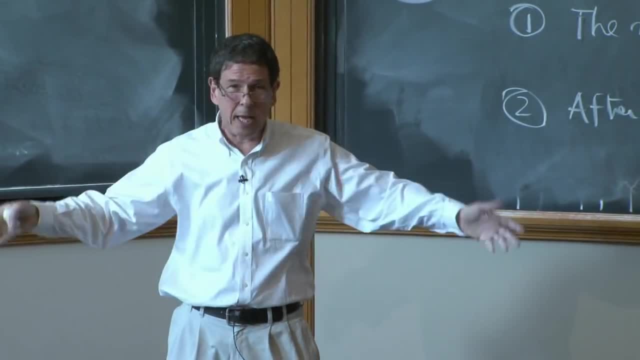 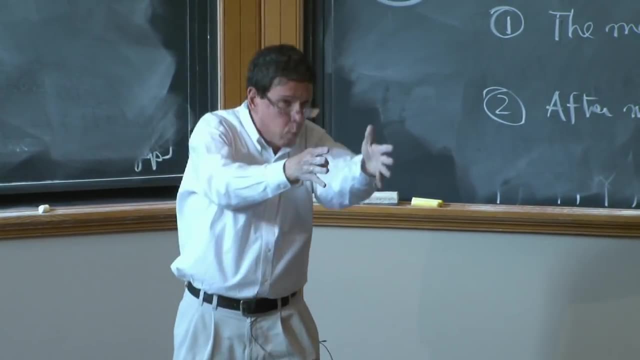 is the wave function of momentum. h bar k. If at the beginning it was a superposition of many, as Fourier told you, then after measuring, if you get one component of momentum, that's all. That's all that is left of the wave function. 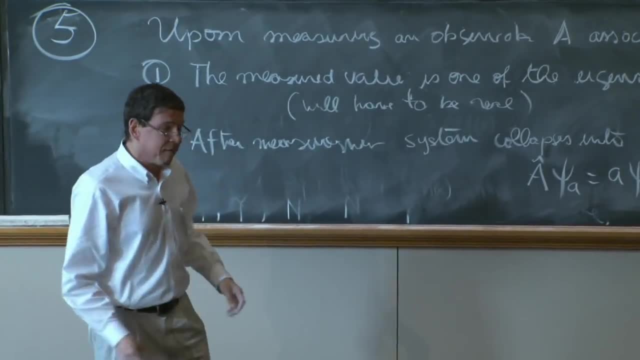 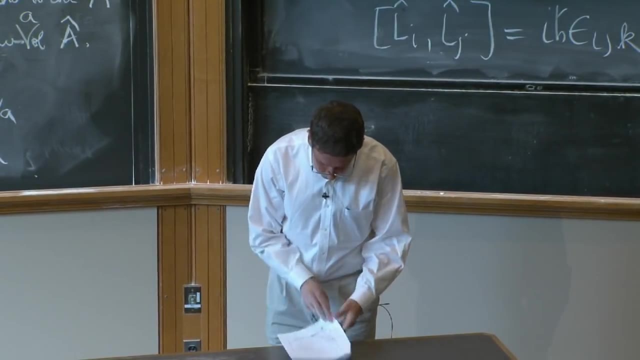 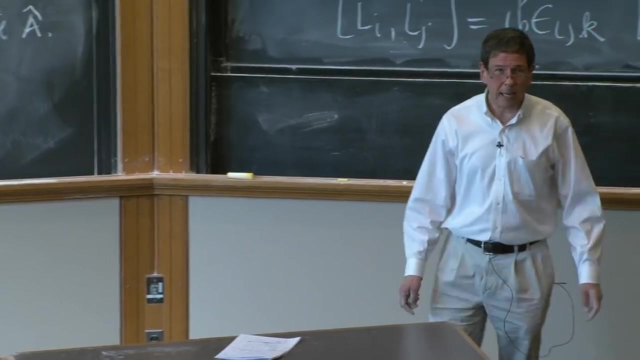 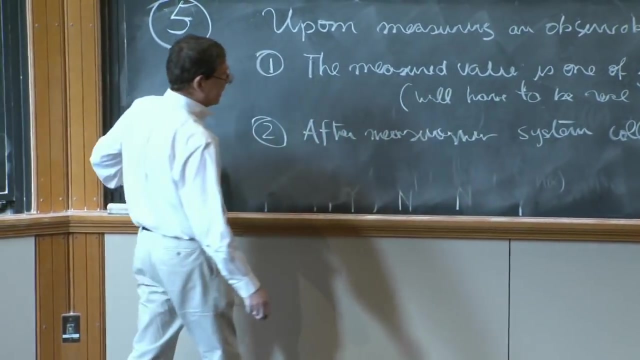 It collapses. This collapse is a very strange thing, And it's something about quantum mechanics that people are a little uncomfortable with And try to understand better, but surprisingly, nobody has understood it better after 60 years of thinking about it, And it works very well. 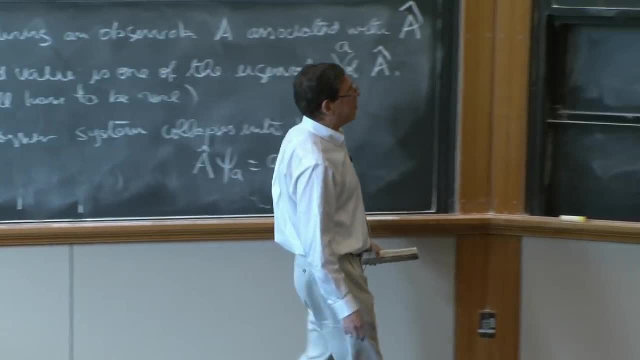 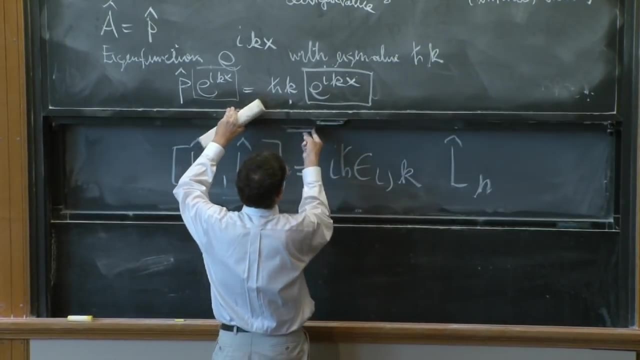 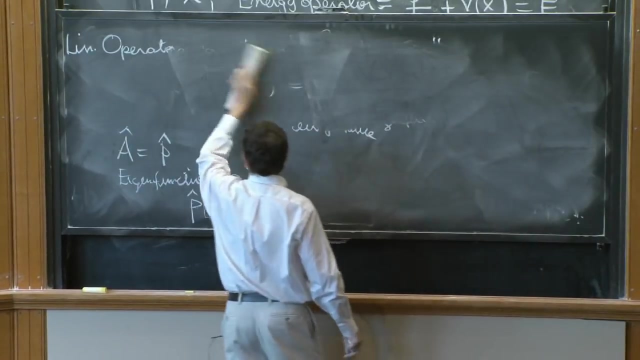 It's a very strange thing Because, for example, if you have a wave function that says your particle can be anywhere, after you measure where it is, the whole wave function becomes a delta function at the position that you measured. So everything on the wave function. 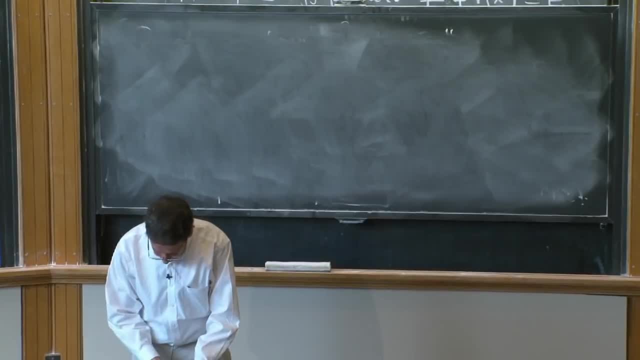 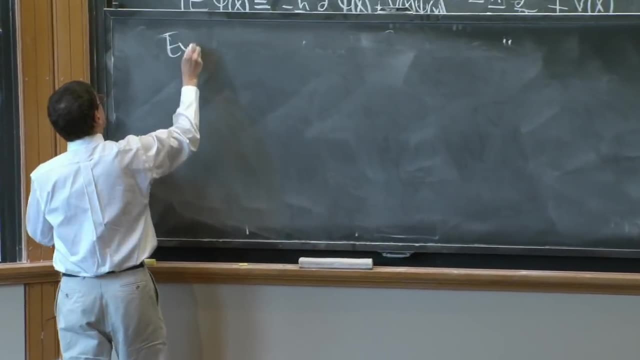 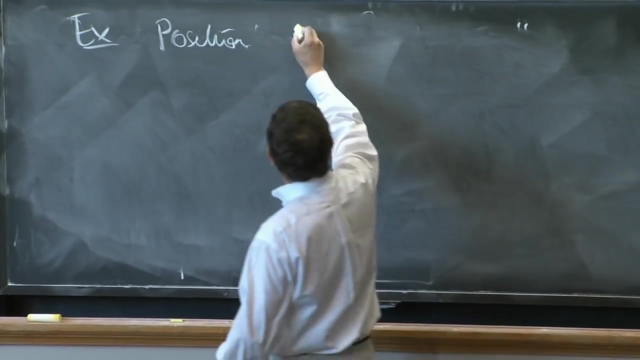 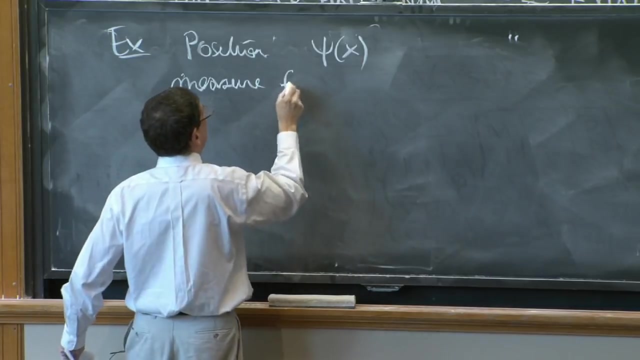 when you do a measurement, basically collapses, as we will say now, For example, Let's do this, Let's do an example Example Position: So you have a wave function, psi of x, You find, measure and find the particle at x0.. 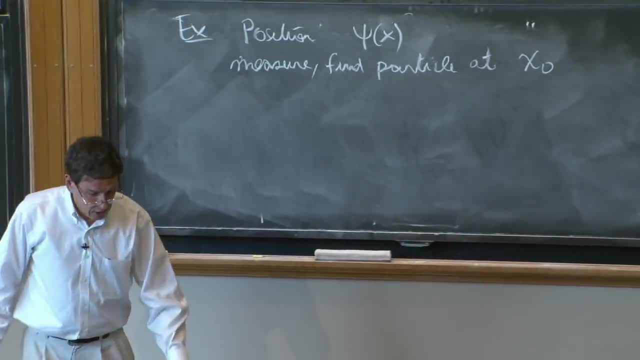 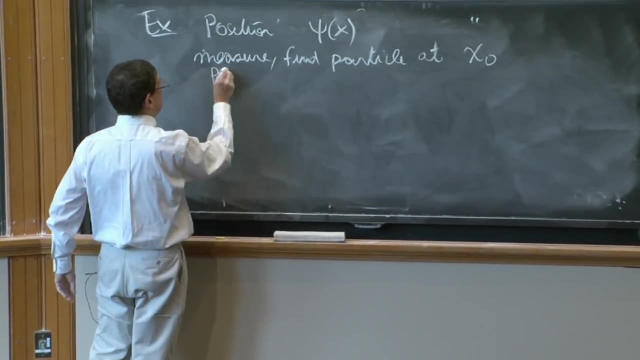 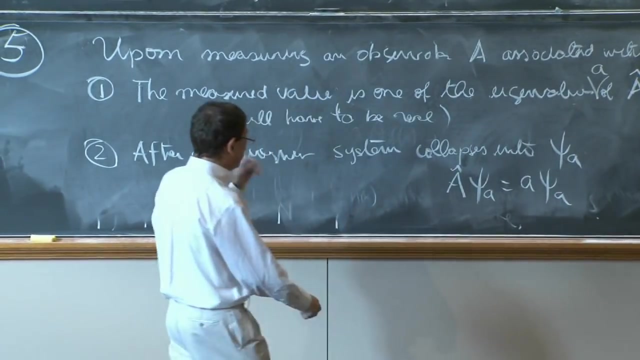 Measure and you find the particle at x0. So measure what I should be clear Measure position. So we said two things: The measured value is one of the eigenvalues of A And after measurement the system collapses to eigenfunctions. 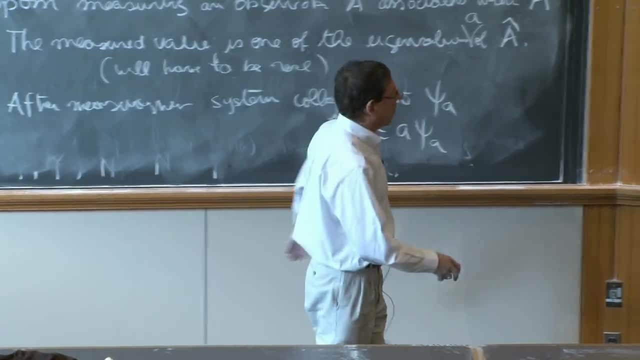 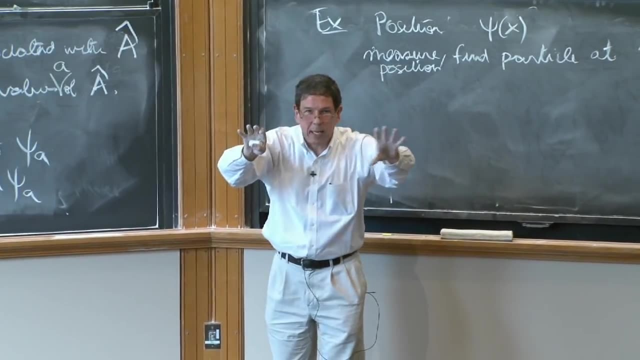 Now, here we really need a little of your intuition. A position eigenstate is a particle localization which is a constant. It's a constant. It's a particle localized at one place. What is the best function associated to a position eigenstate? 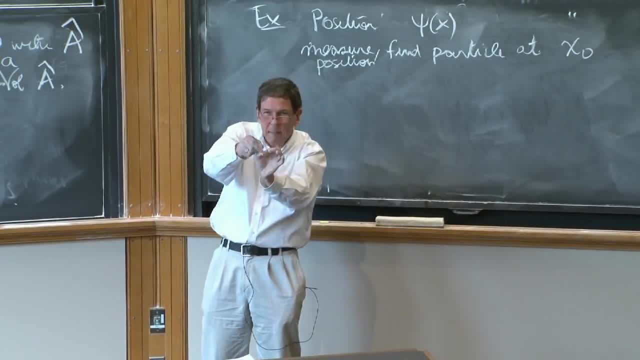 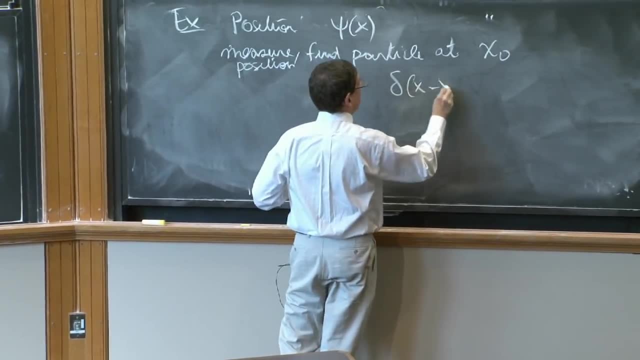 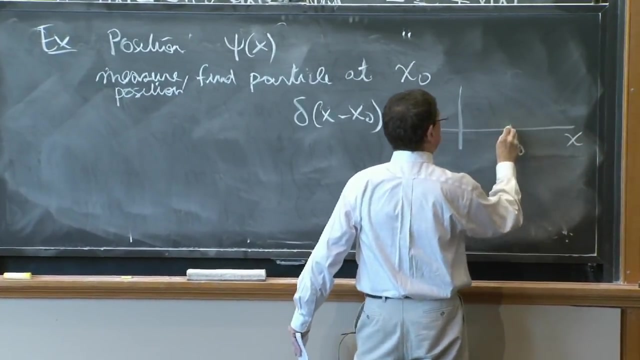 It's a delta function, The function that says it's at some point and nowhere else. So the eigenfunctions delta of x minus x0, it's a function. as a function of x, it peaks at x0. And it's 0 everywhere else. 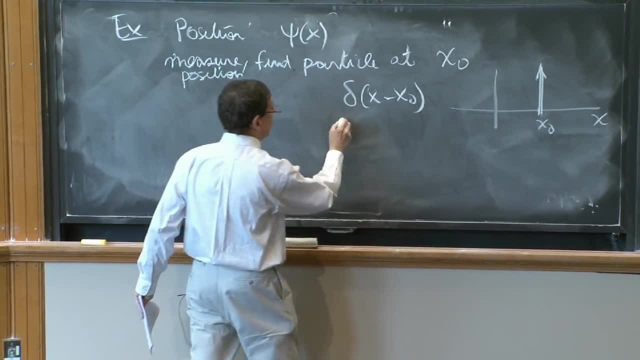 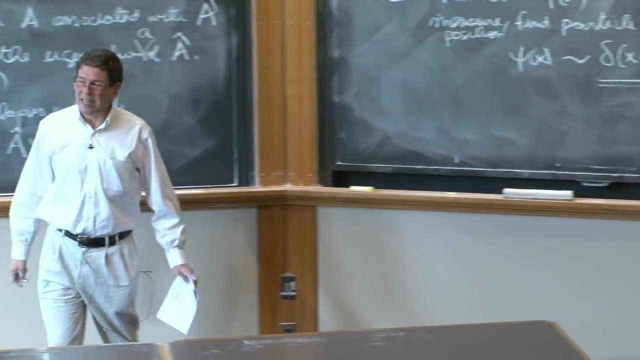 And this is When you find a particle at x0, this is the wave function. The wave function must be proportional to this quantity. Now you can't normalize this wave function. It's a small complication, but we shouldn't worry about it too much. 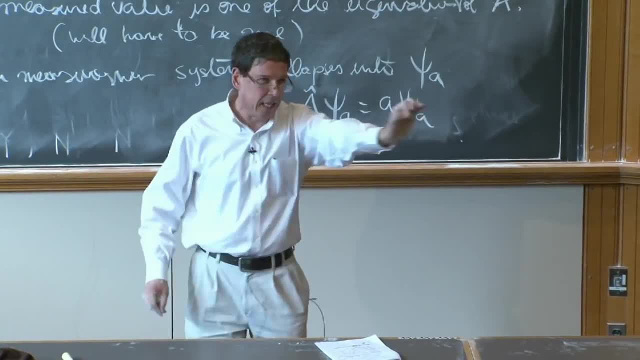 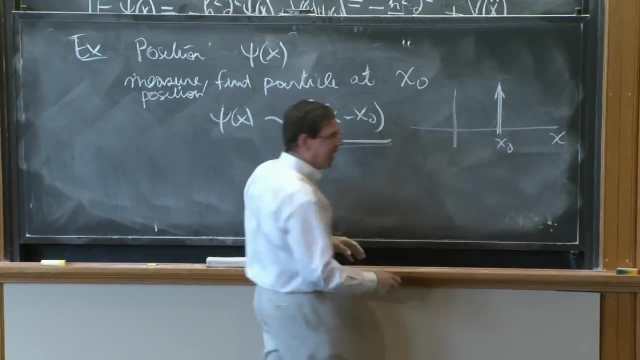 Basically, you really can't localize a particle perfectly, So that's the little problem with this wave function. You've studied how you can represent delta functions as limits And prove it, And probably intuitively, those limits are the best things. 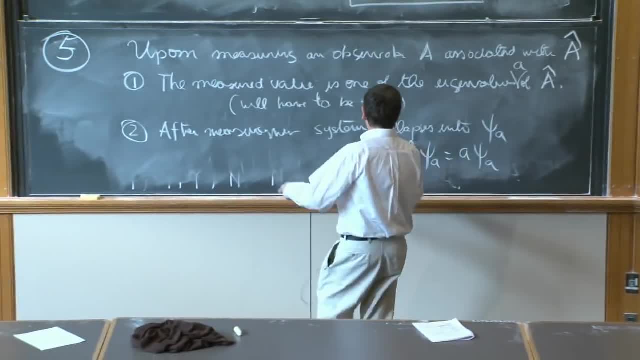 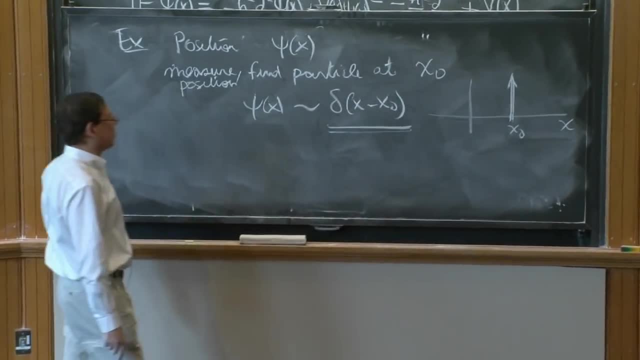 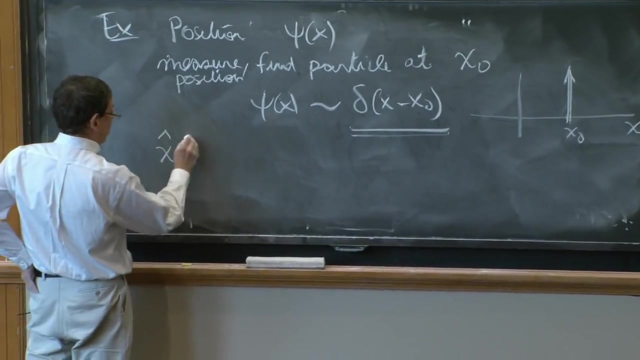 But this is the wave function. So after you measure the system, you go into an eigenstate of the operator. Is this an eigenstate of the x operator? What a strange question, But it is. Look, If you put the x operator on delta of x minus x0,. 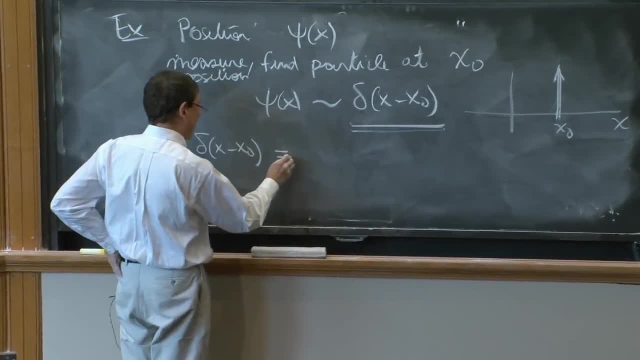 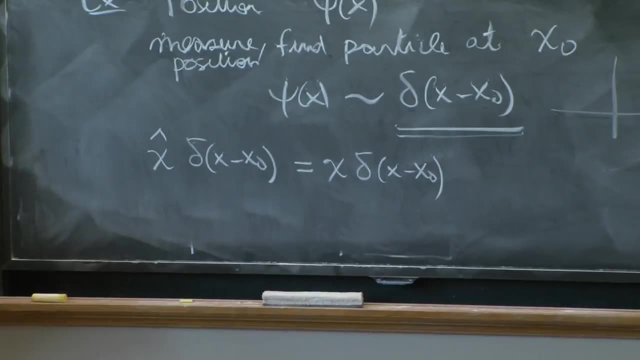 what is it supposed to do? It's supposed to multiply by x. It's supposed to multiply by x, So it's x times delta of x minus x0.. If you had a little experience with delta functions, you know that this function is 0 everywhere. 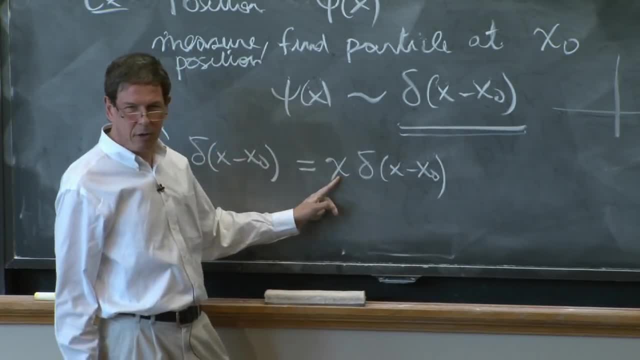 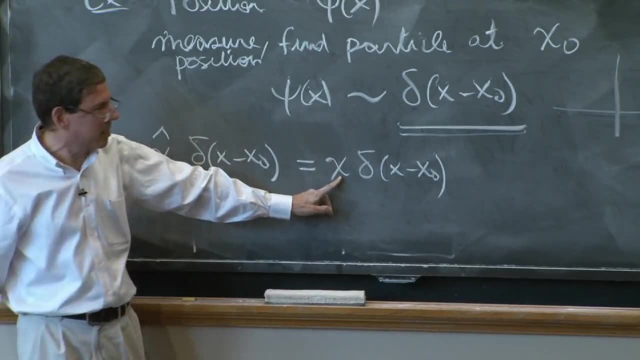 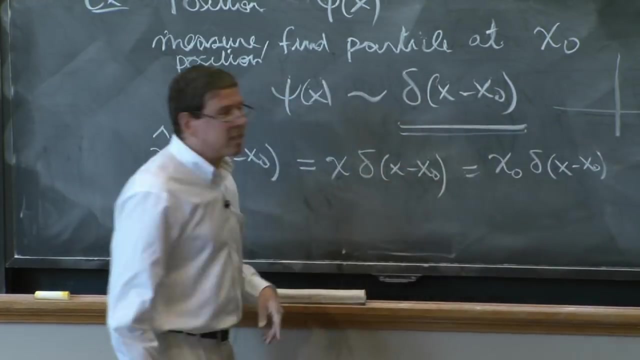 except when x is equal to x0. So this x can be turned into x0. It just never at any other place it contributes. This x really can be turned into x0 times delta of x minus x0. Because delta functions are really used to do integrals. 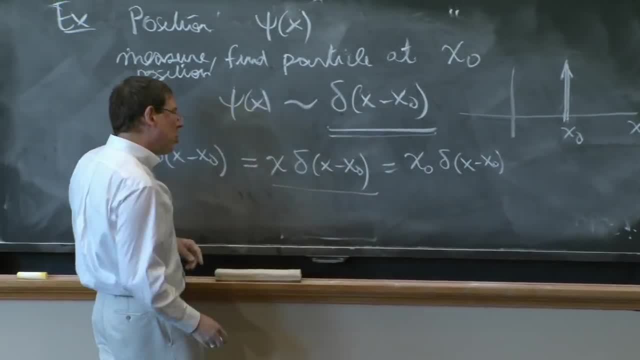 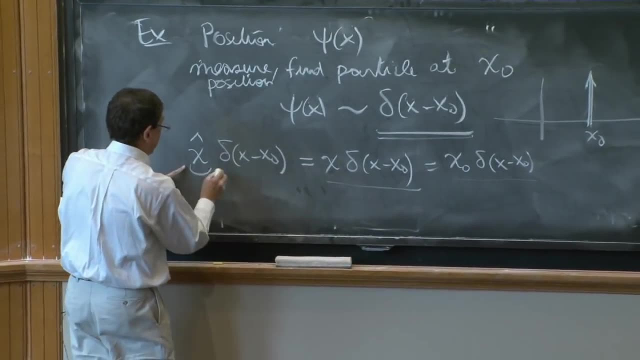 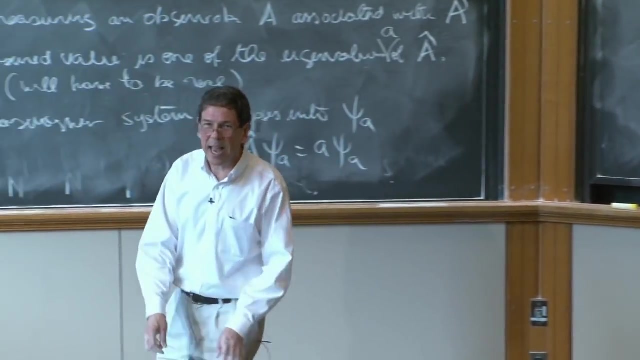 And if you do the integral of this function, you will see that it gives you the same value as the integral of this function. So then you have it. The operator acting on the eigenfunction is a number times this, So these are indeed eigenfunctions of the x operator. 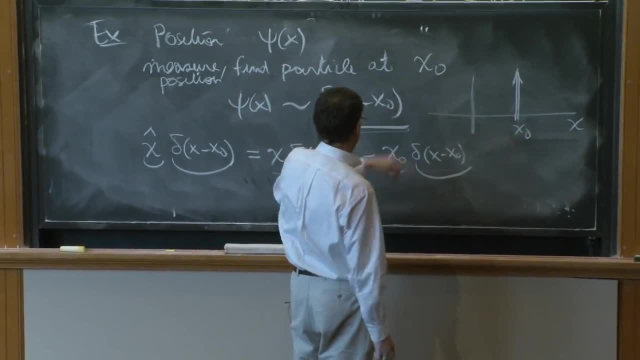 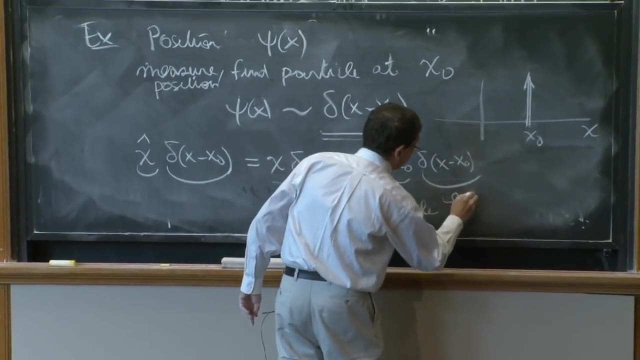 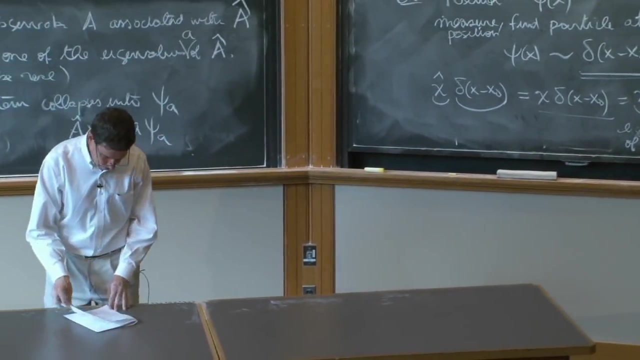 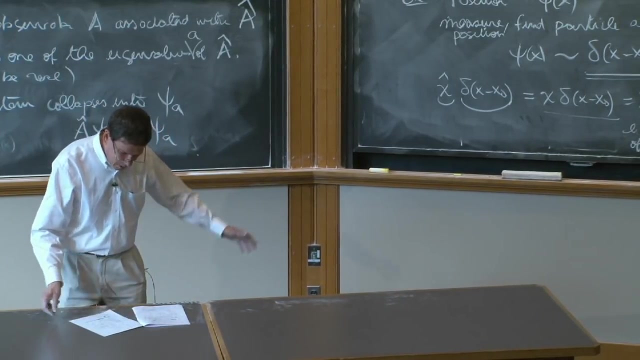 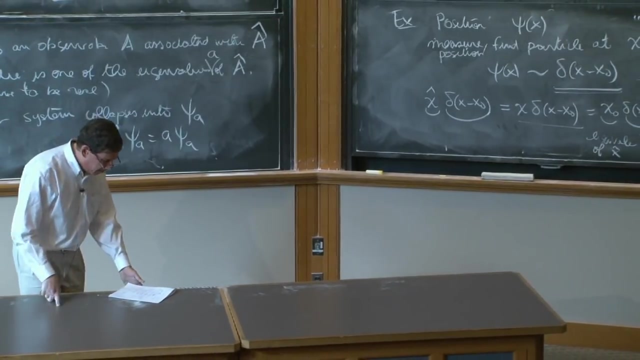 And what you measured was an eigenvalue of the x operator, eigenvalue function of x, and this is an eigenfunction of x. So we can do the same with the momentum Eigenvalues and eigenfunctions. we've seen them more properly. 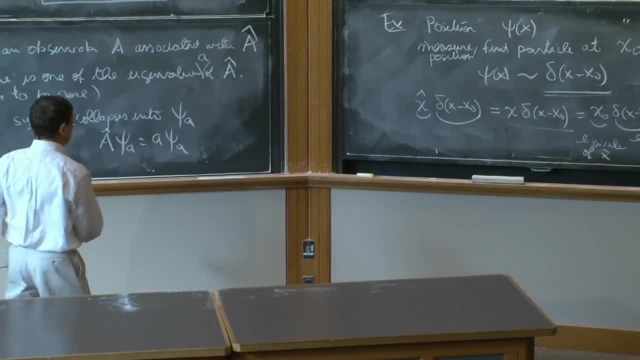 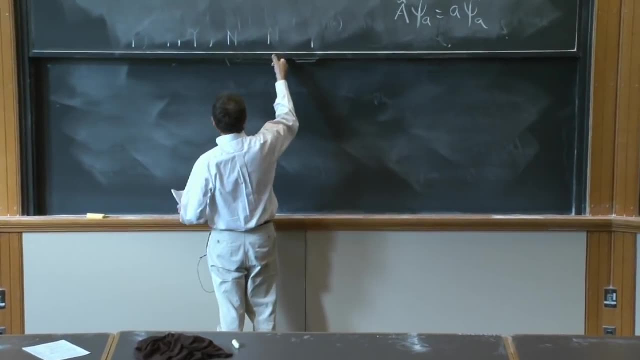 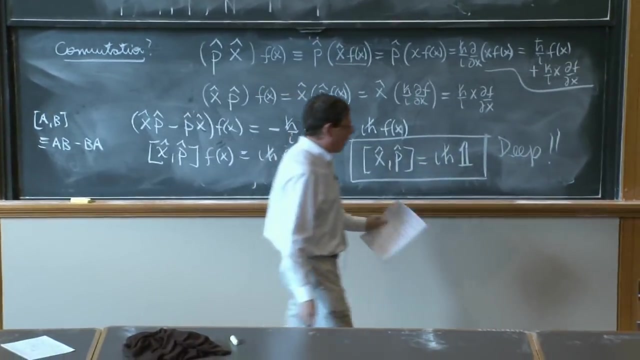 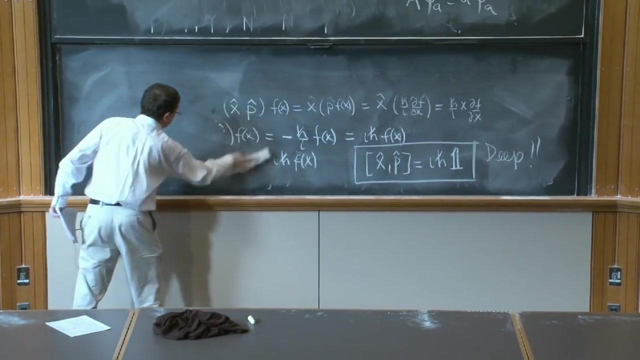 Now we'll go to the sixth postulate. The last postulate that we want to talk about is the one of general operators and general eigenfunctions and what happens with them. So let's take now our operator a and its eigenfunctions. Let's do that. 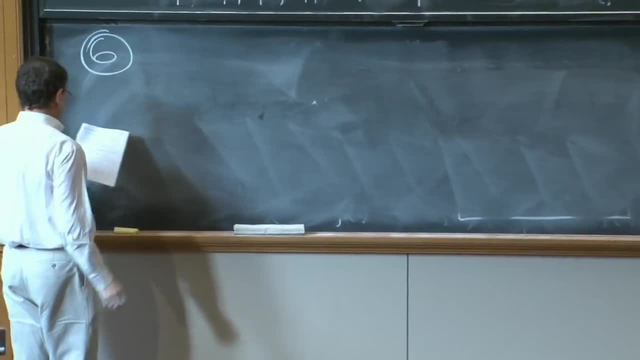 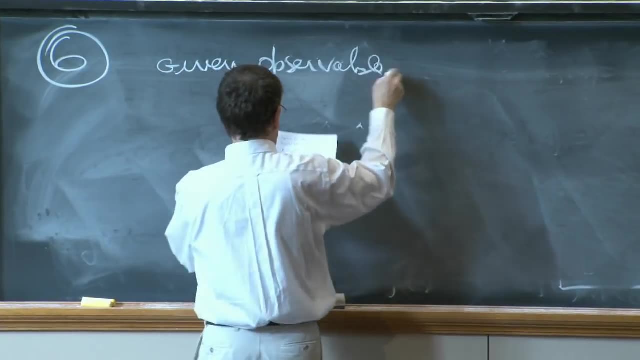 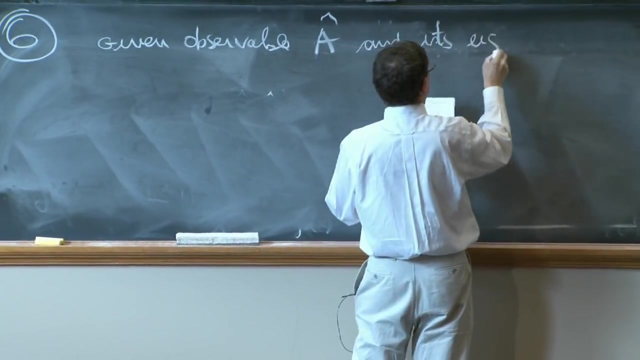 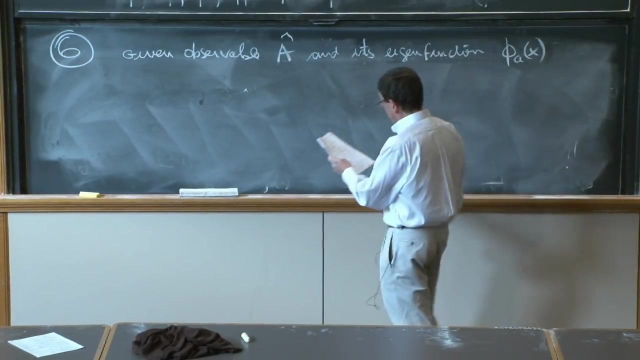 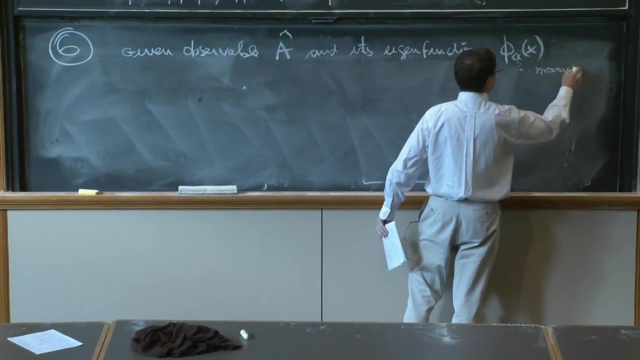 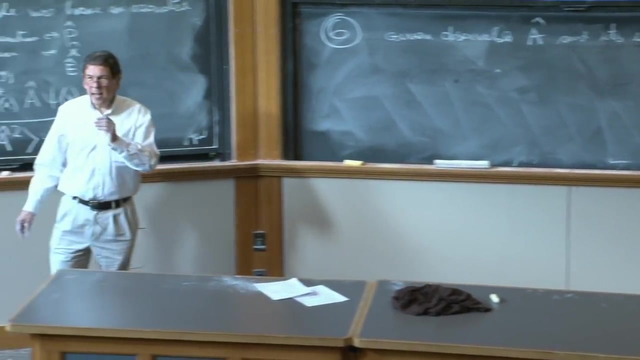 What can be found? So six. Given an observable, a hat, and its eigenfunctions, phi a of x. So an a runs over many values, Many values, OK, So let's consider this case Now. the eigenfunctions of an operator are very interesting objects. 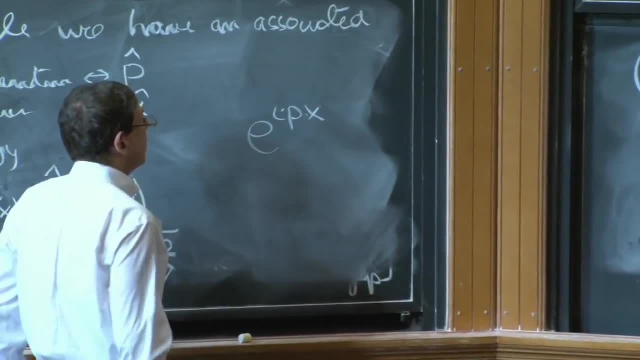 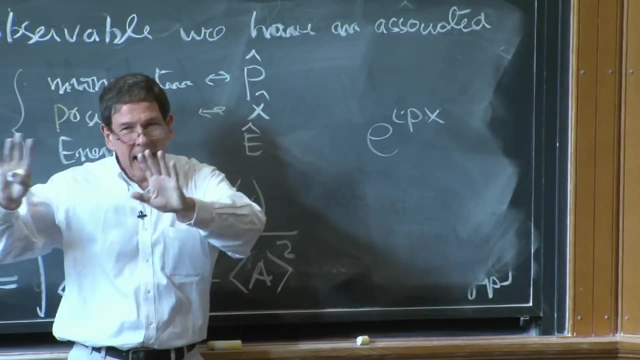 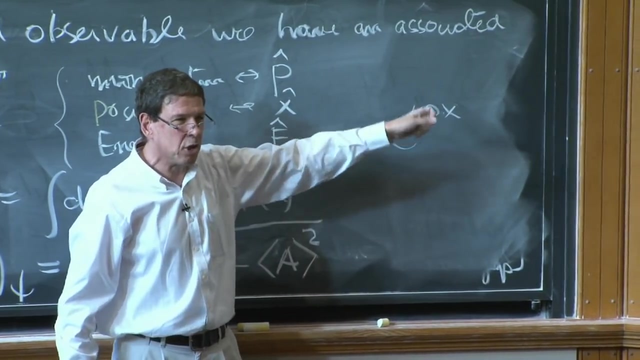 You see, the eigenfunctions of momentum were of this form and they allow you to expand, via the idea of Fourier, any wave function of superpositions of these things. Fourier told you, can I Expand any function in eigenfunctions of the momentum? 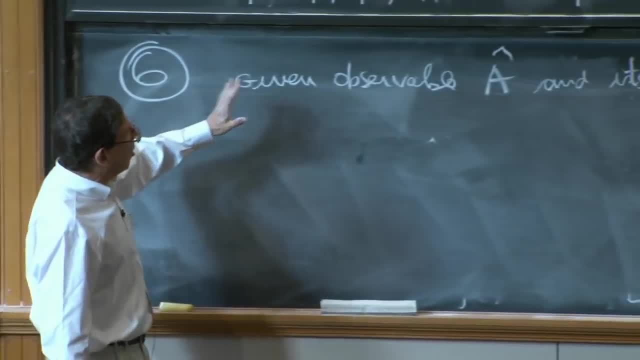 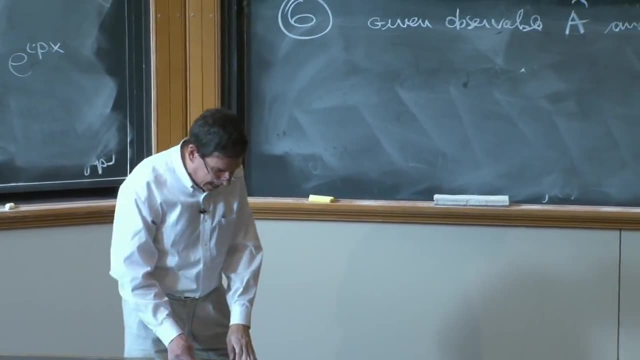 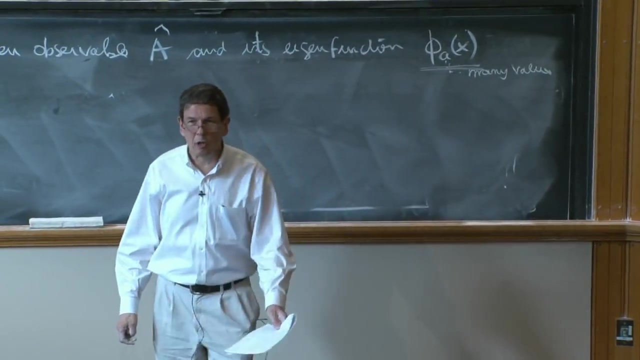 Well, the result is more general, For observables in general, you can expand functions, arbitrary functions, in terms of the eigenfunctions. Now for that, remember, an eigenfunction is not determined up to scale. You change, multiply it by 3, it's an eigenfunction still. 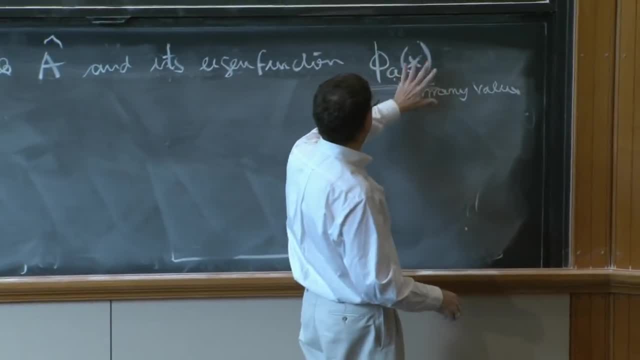 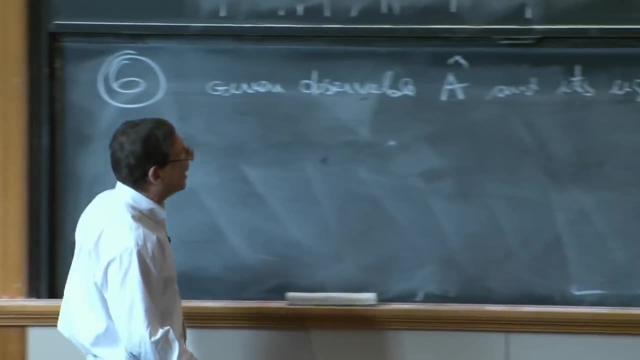 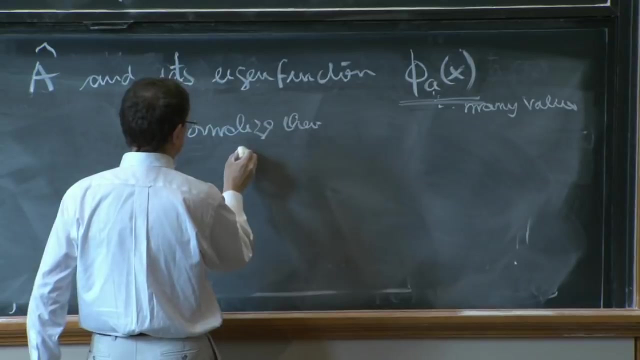 So people like this, They like this, People like to normalize them nicely. the eigenfunctions. You construct them like this and you normalize them nicely. So how do you normalize them? Normalize them by saying that the integral over x of psi a. 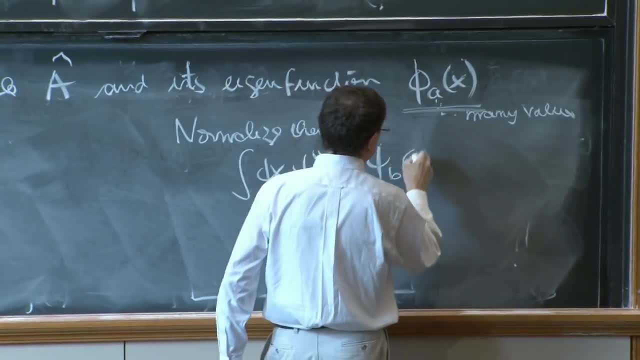 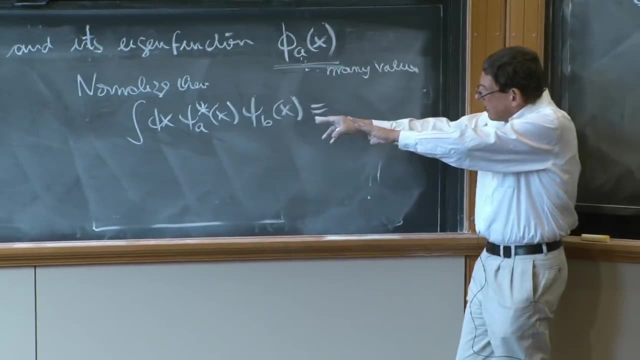 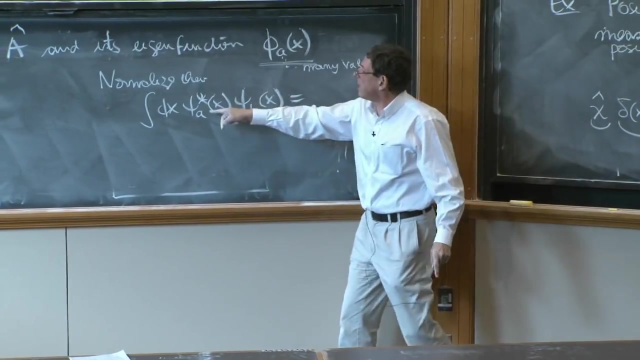 star of x, psi, b of x is going to be what? OK, Ah, Ah, Ah Ah. Basically, what you want is that these eigenfunctions be basically orthogonal, each one orthogonal to the next. So you want this to be 0, unless these two different eigenfunctions. 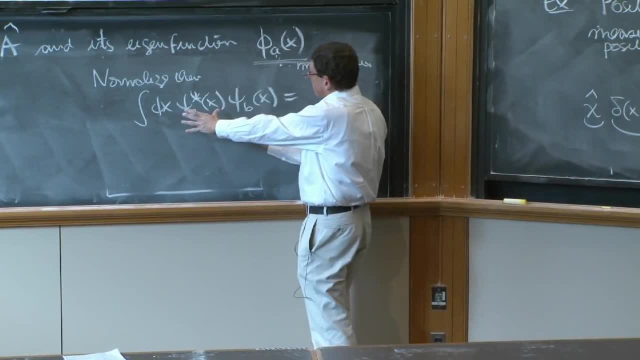 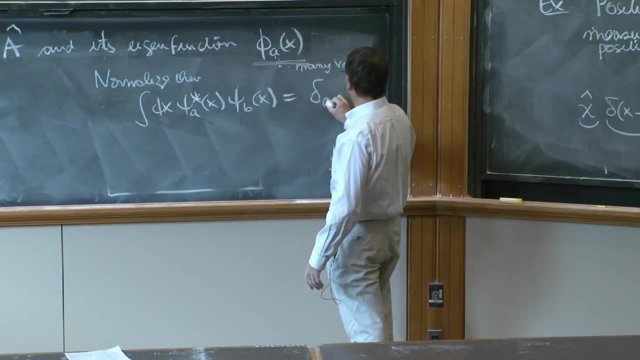 are different, And when they are the same, you want them to be just like wave functions- that their total integral of psi squared is equal to 1.. So what you put here is delta ab. Now, this is something that you can always do with eigenfunctions. 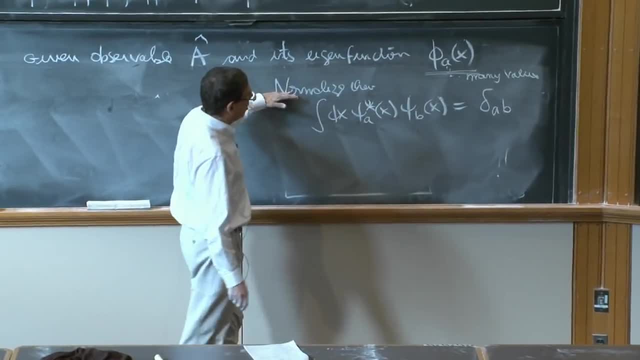 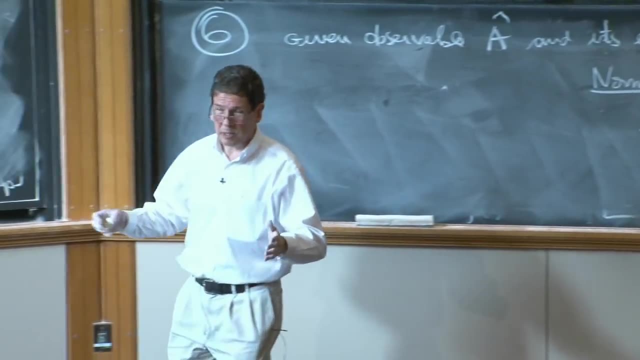 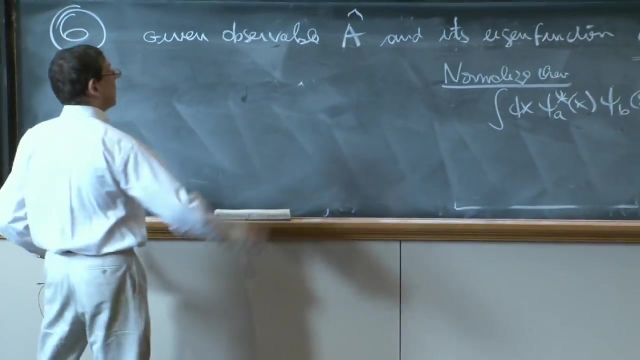 It's proven in mathematics books. It's not all that simple to prove, but this can always be done, And when we need examples, we'll do it ourselves. So, given an operator that you have its eigenfunctions like that, two things happen. 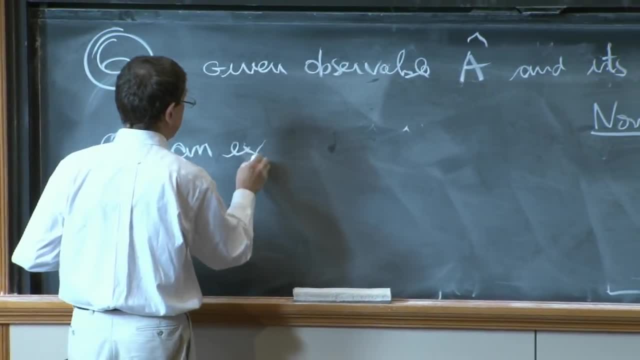 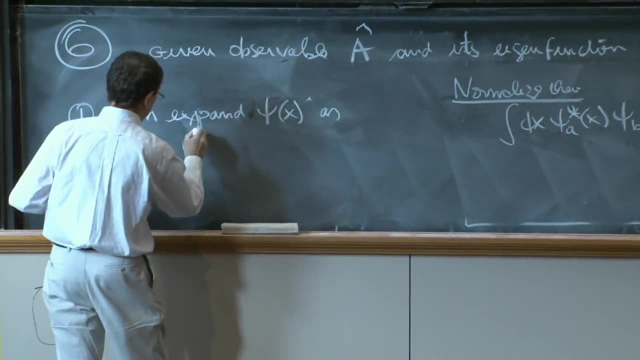 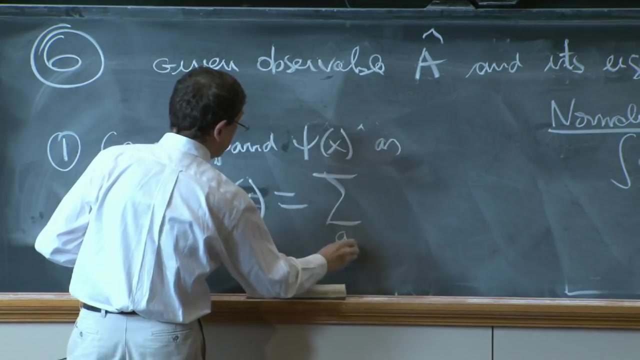 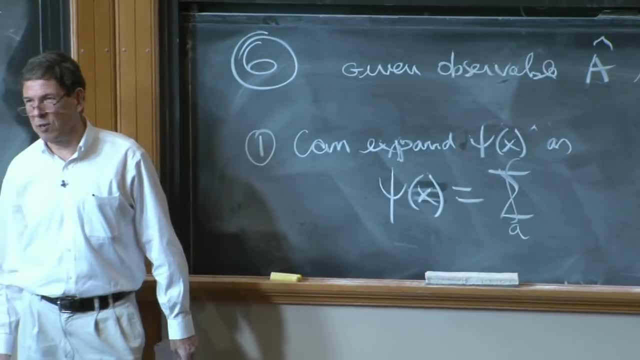 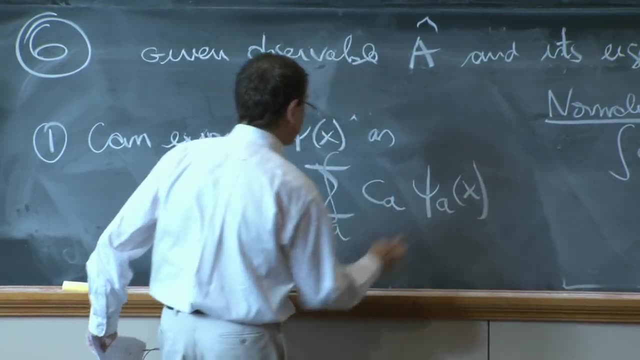 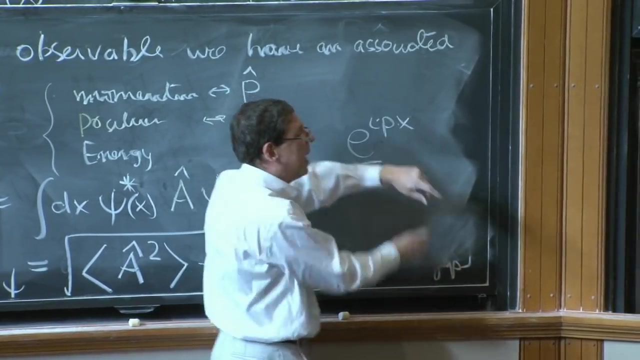 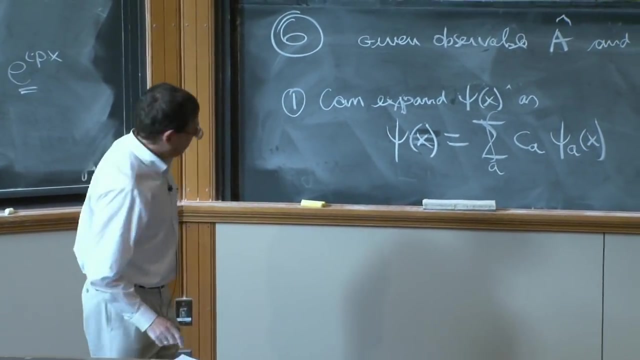 an integral on top of that. You can write it whichever way you want. It doesn't matter Of coefficients times, the eigenfunctions. So just like any wave could be written as Fourier coefficients functions, any state can be written a superposition of these things. 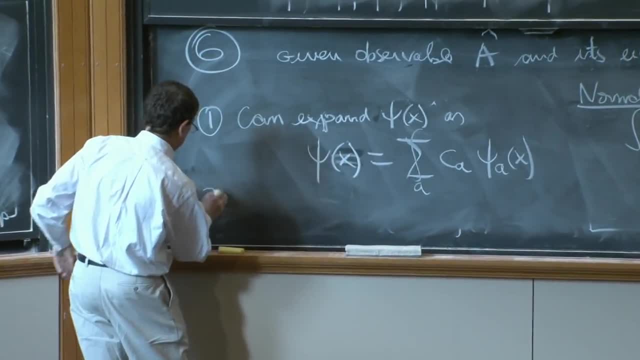 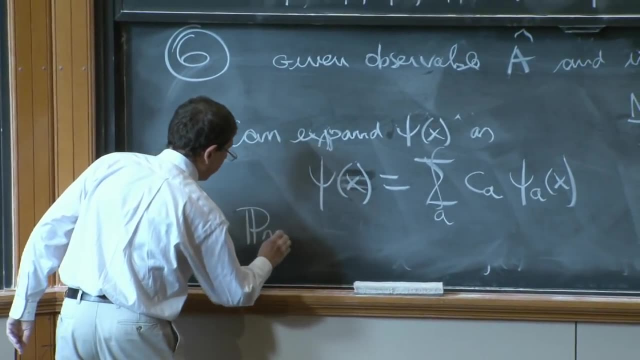 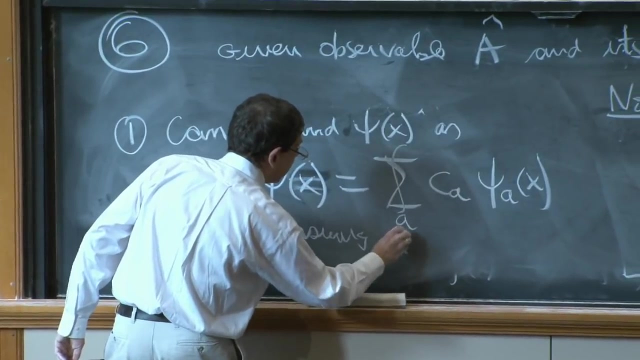 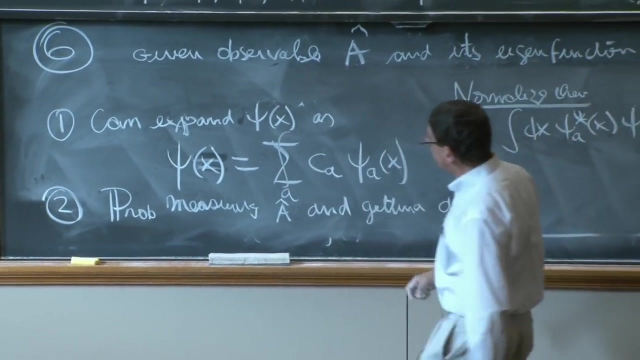 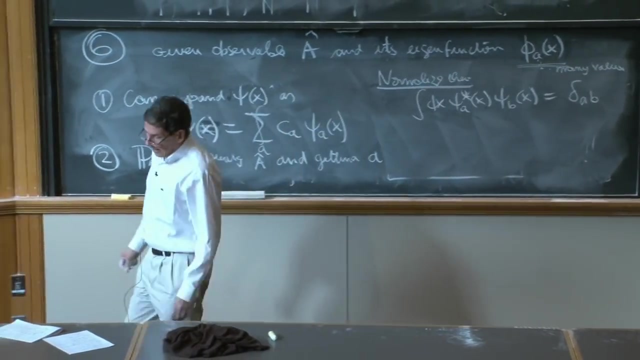 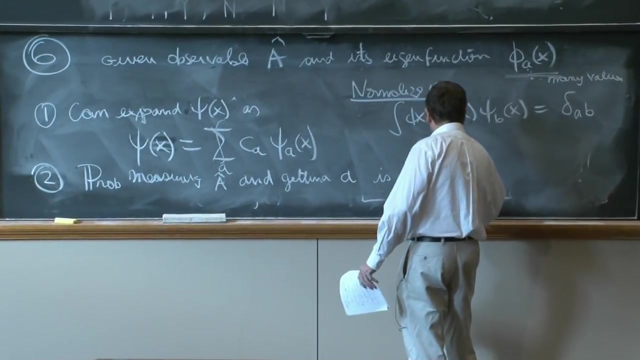 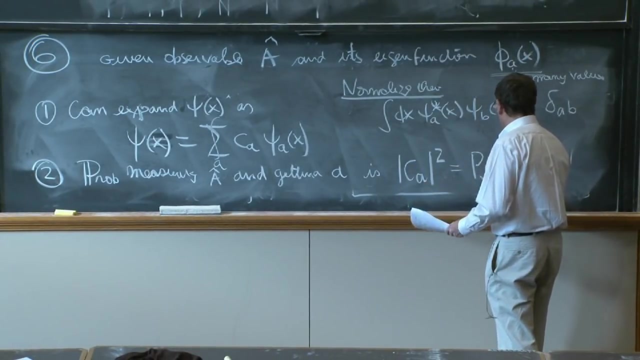 So that's one And two, the probability of measuring A hat and getting A. So A is one of the particular values that you can get. That probability is given by the square of this coefficient, CA squared. So this is P, the probability to measure in psi. 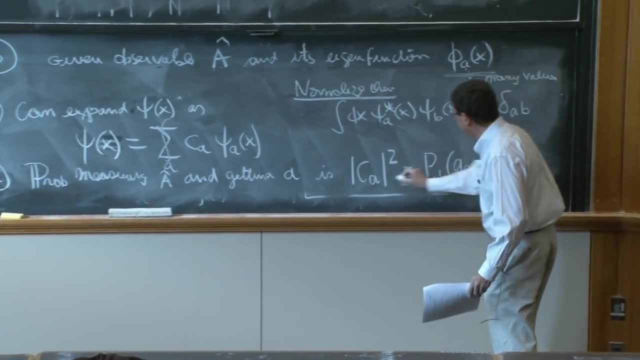 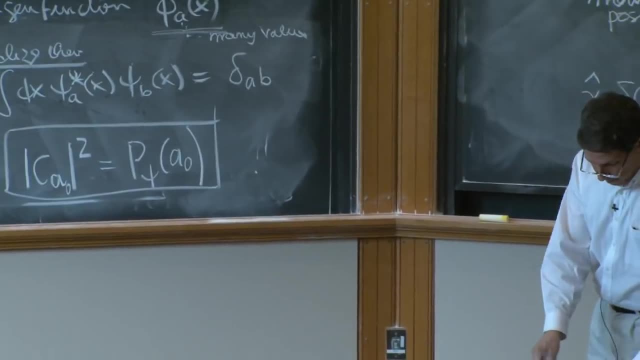 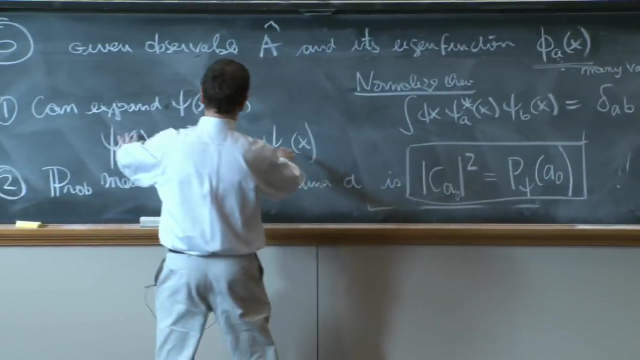 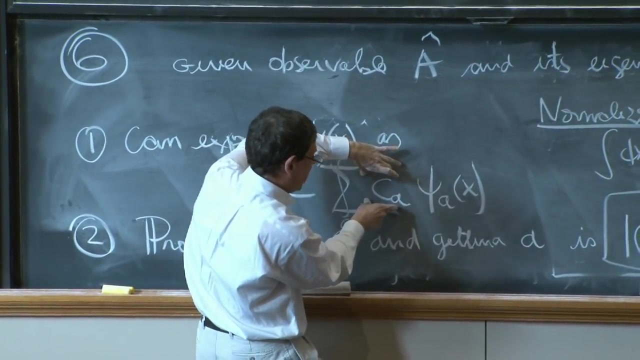 and to get A hat A, And I think actually let's put an A0 there. So here we go. So it's a very interesting thing. Basically, you expand the wave function in terms of these eigenfunctions And these coefficients give you the probabilities. 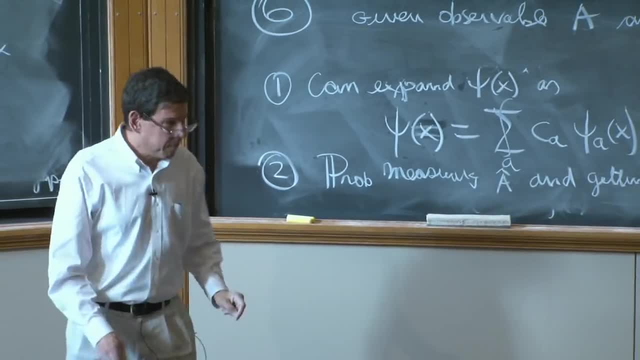 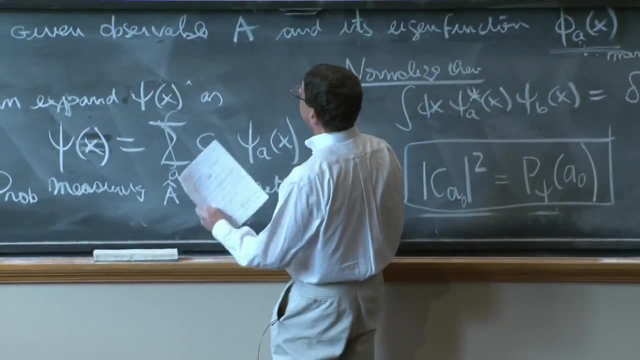 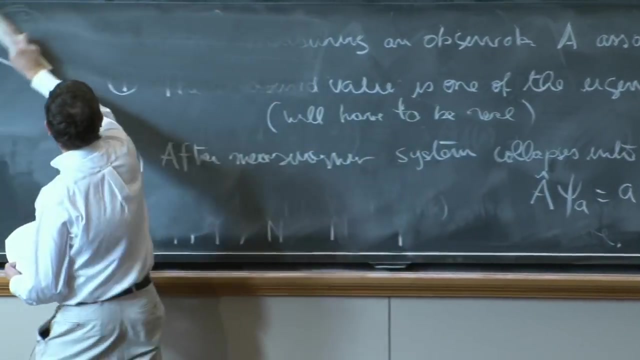 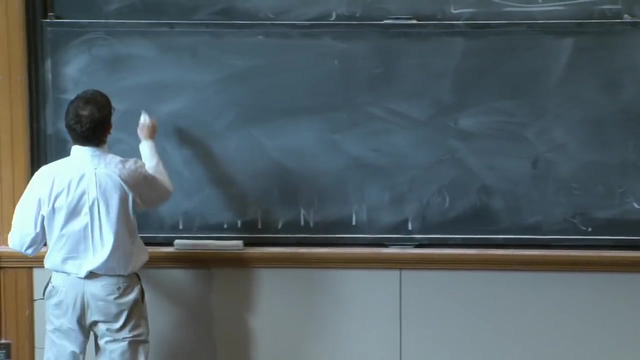 of measuring these numbers. So So we can illustrate that again with the delta functions, And we'll do it quick because we get to the punchline of this lecture with the Schrodinger equation. So what do we have? Well, let me think of the operator x, example. 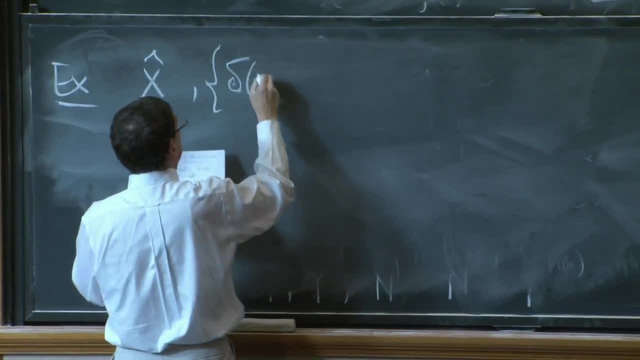 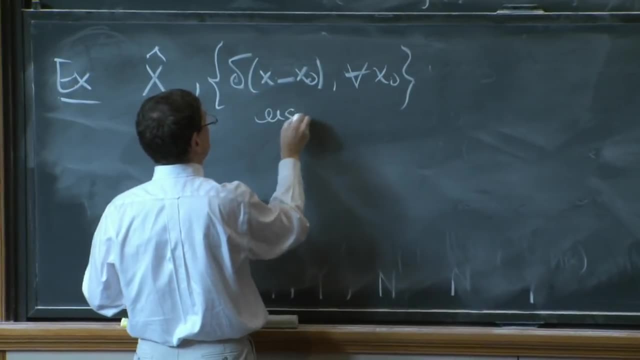 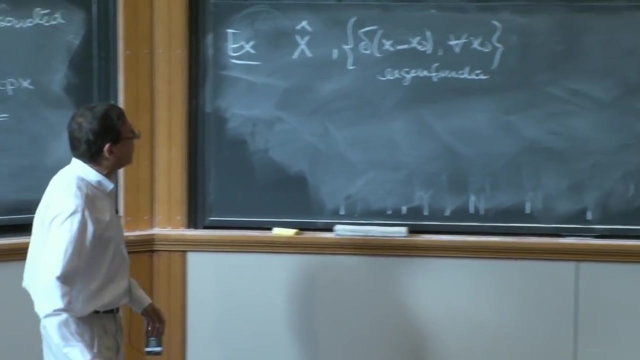 Operator x. the eigenfunctions are delta of x minus x0.. OK, So we have delta of x minus x0 for all x0.. These are the eigenfunctions And we'll write a sort of a trivial equation, but it sort of illustrates what's going on. 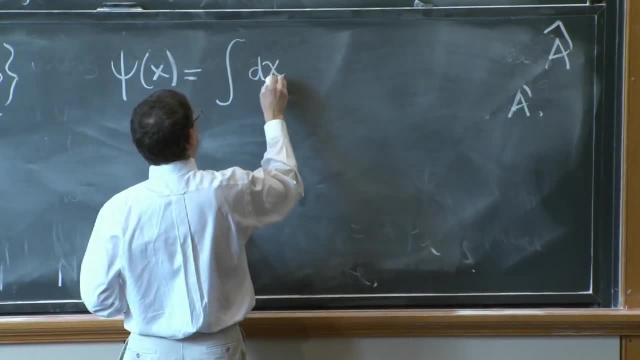 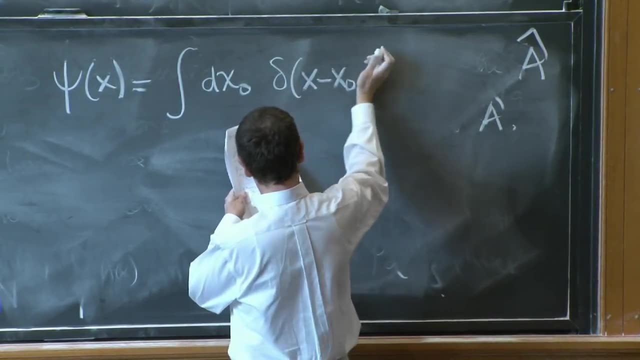 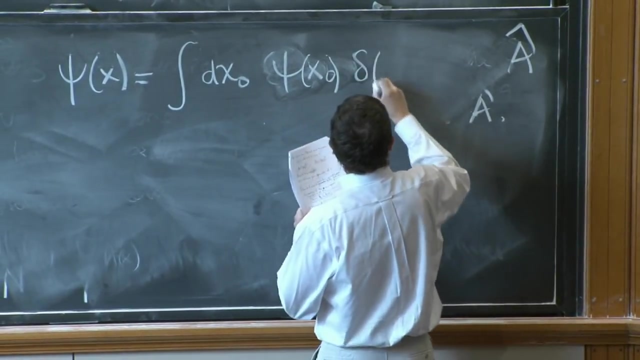 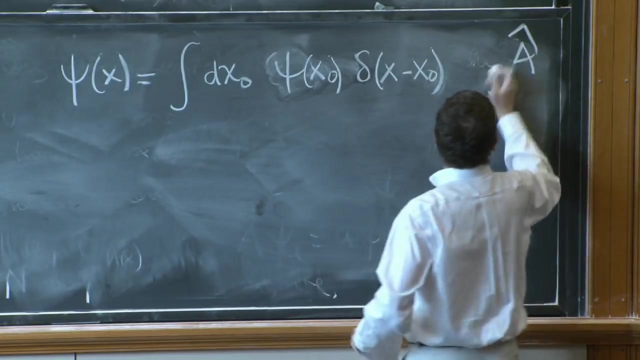 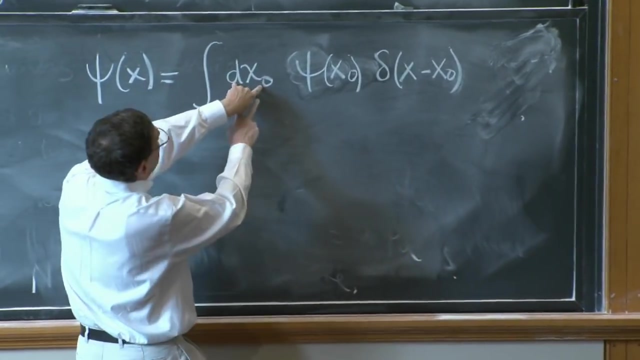 Psi of x as a superposition over an integral over x0, of delta of x minus x0.. Psi of x0- delta of x minus x0, or like this. OK, First let's check that this makes sense. Here we're integrating over x0. 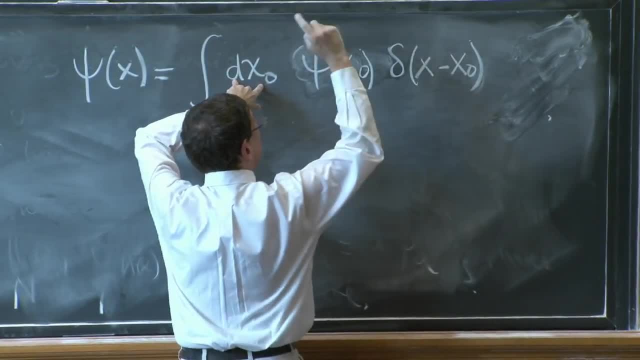 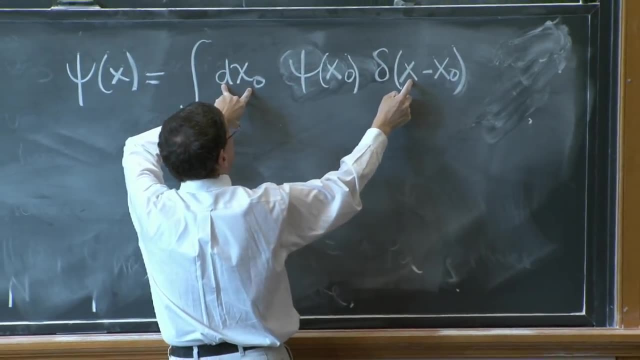 x0 is the variable. This thing shoots and fires whenever x is equal to x, Whenever x0 is equal to x0.. Whenever x0 is equal to x0.. When x0 is equal to x, When x0 is equal to x0. 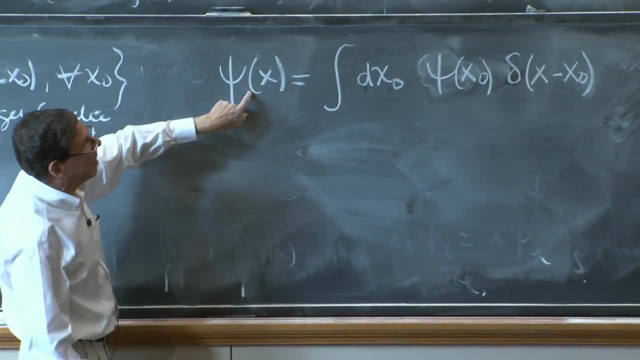 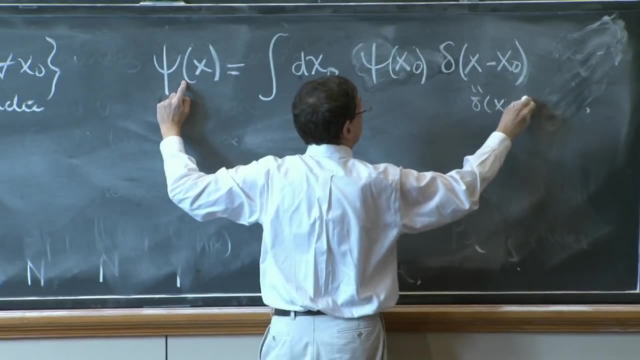 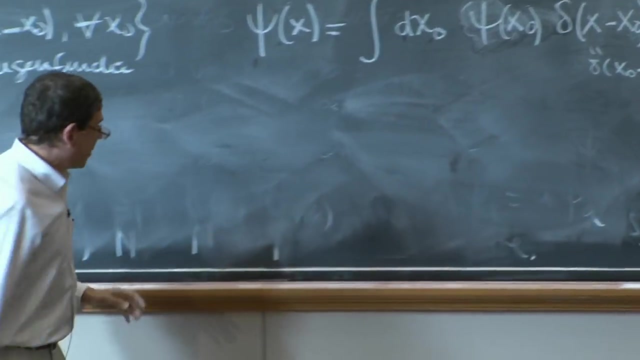 Therefore, the whole result of that integral is psi of x. It's a little funny how it's written, because you have x minus x0, which is the same as delta of x0 minus x. It's just the same thing. And you integrate over x0, and you get just psi of x. 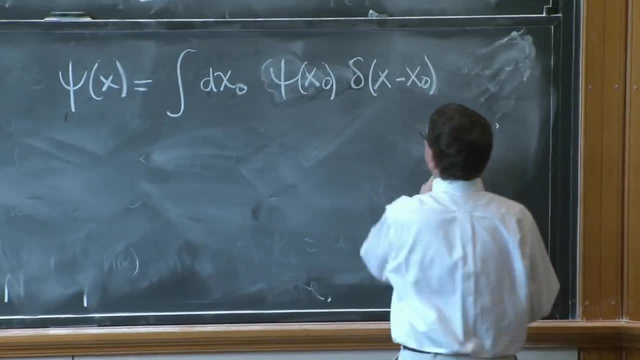 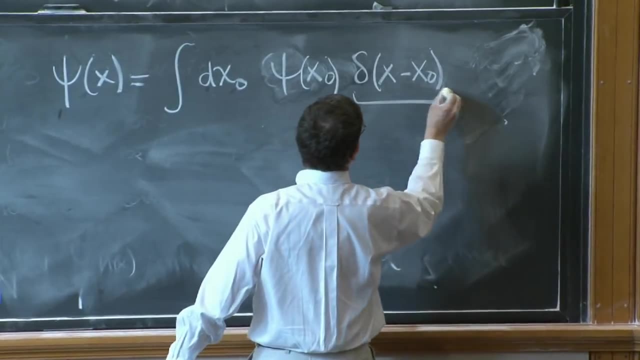 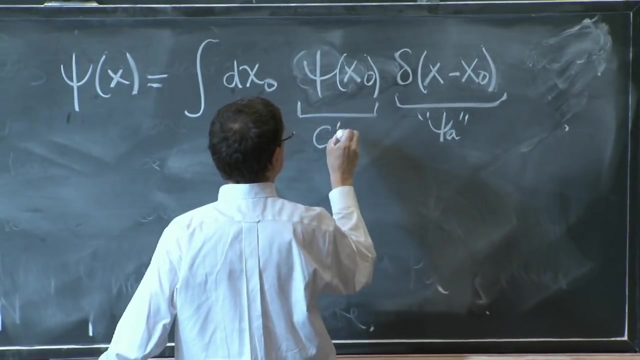 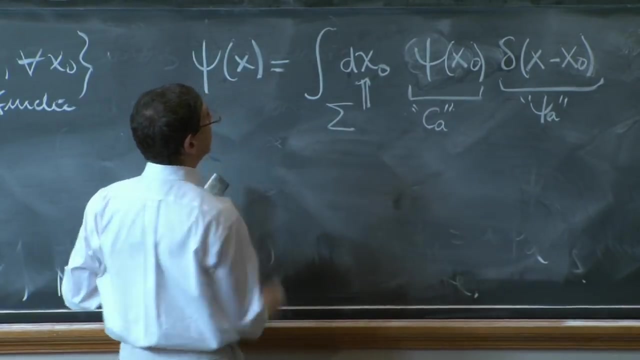 But what have you achieved here? You've achieved the analog of this equation, in which these are the eigenfunctions, These are the psi a's, These are the coefficients c? a's, And this is the sum, this integral. So there you go. 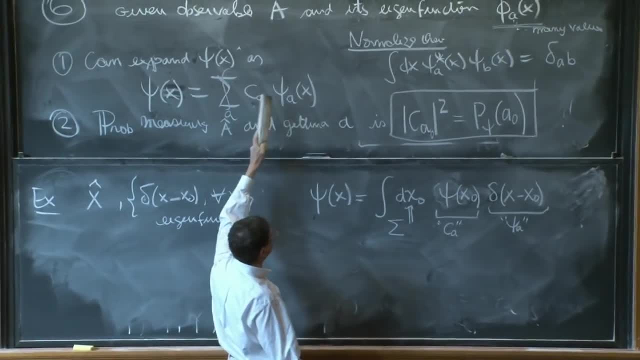 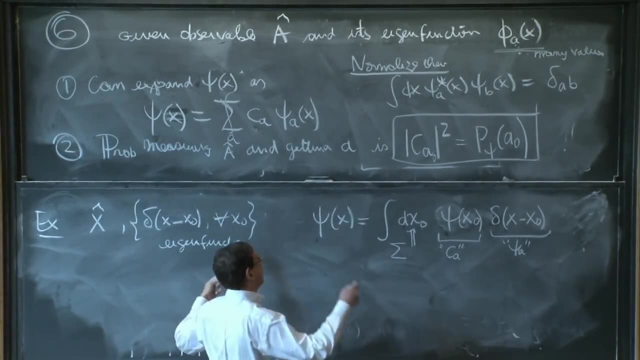 Any wave function can be written as the sum of coefficients times the eigenfunctions of the operator. And what is the probability to find the particle at x0?? Well, it's from here. the coefficient c a squared. That's exactly what we had before. 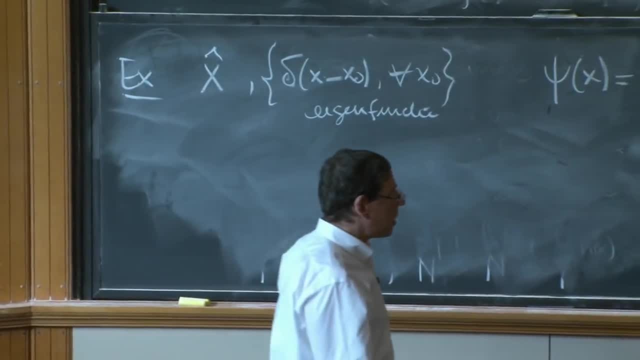 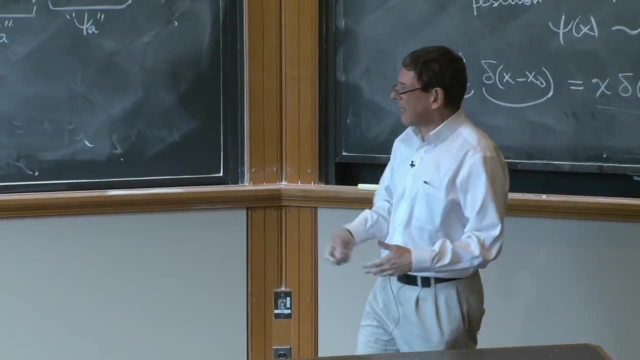 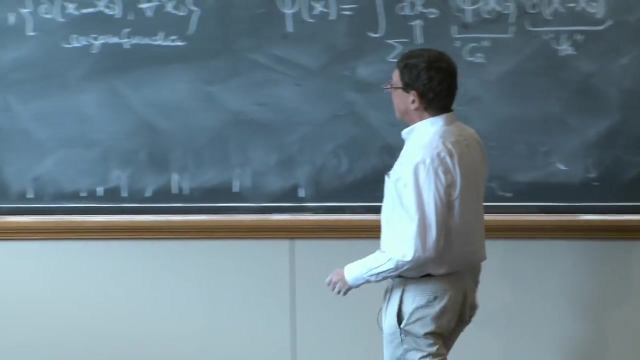 So this is getting basically what we want. So this brings us to the final stage of this lecture, in which we have to get the time evolution finally. So how does it happen? Well, it happens in a very interesting way, So maybe I'll call it Seven-Schrodinger equation. 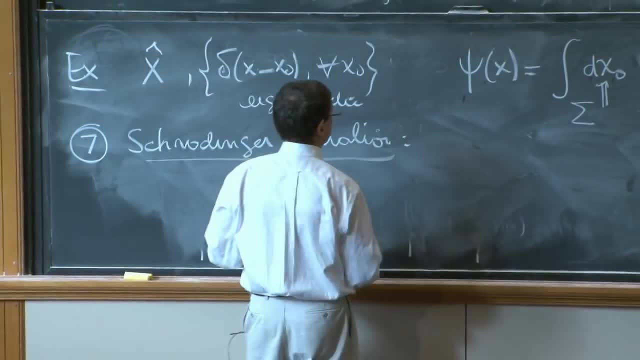 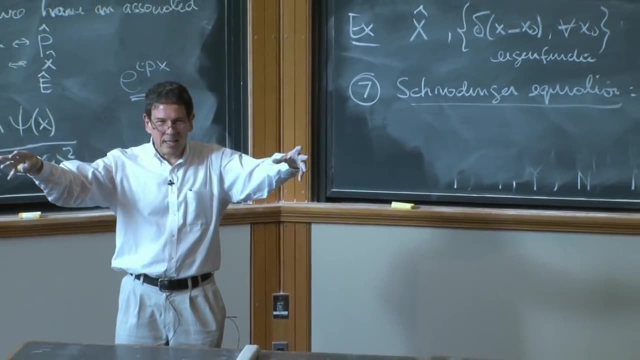 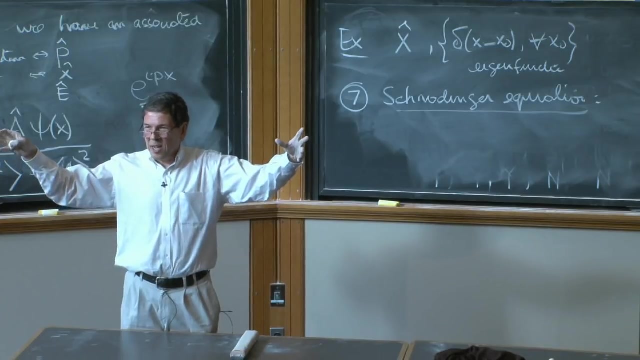 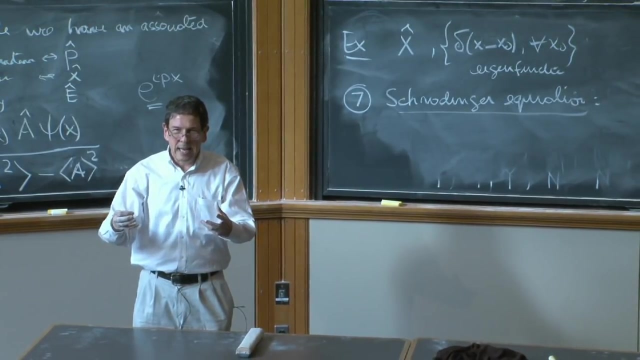 So, as with any fundamental equation in physics, there's experimental evidence And suddenly, however, you have to do a conceptual leap. Experimental evidence doesn't tell you this. Experimental evidence doesn't tell you the equation, It suggests the equation And it tells you, probably, what you're doing is right. 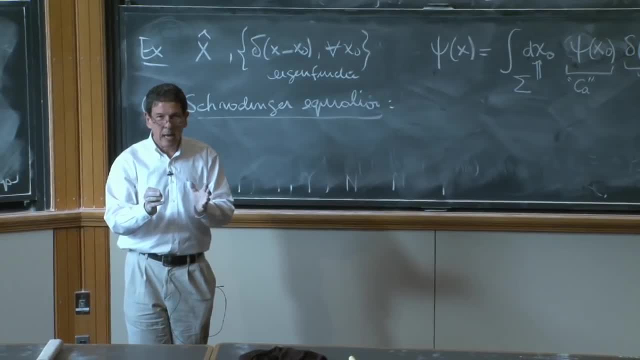 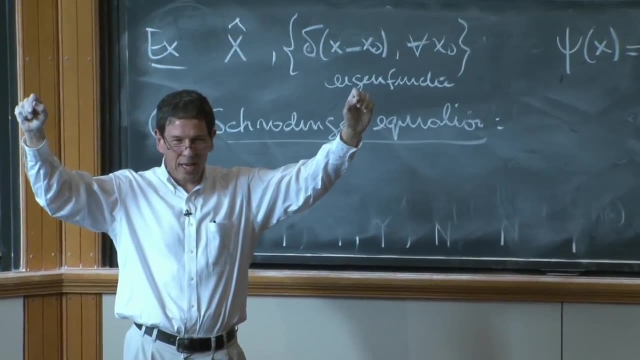 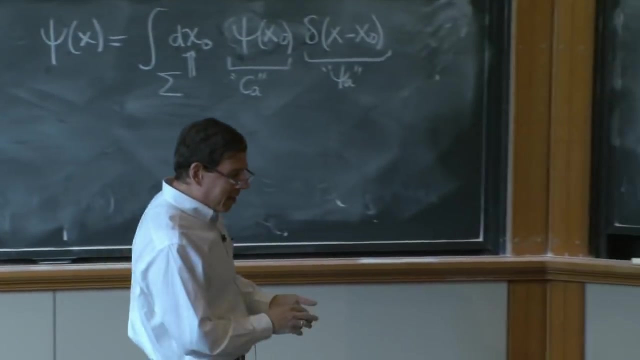 So what we're going to do now is collect some of the evidence we had and look at an equation and then just have a flash of inspiration, change something very little, And suddenly that's the Schrodinger equation. Alan told me that in fact, students sometimes say: 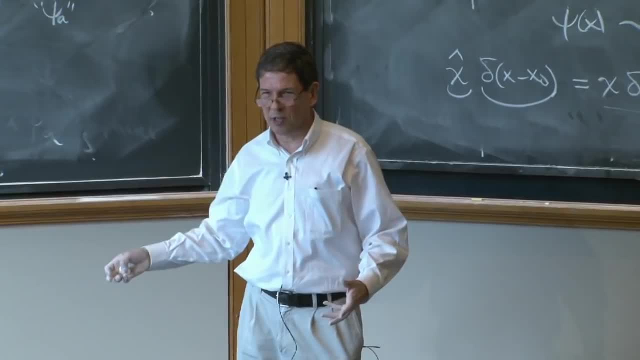 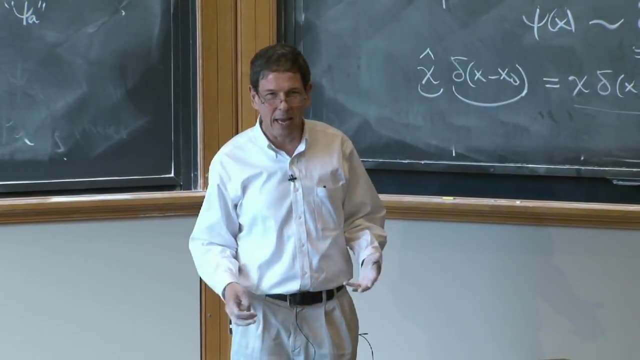 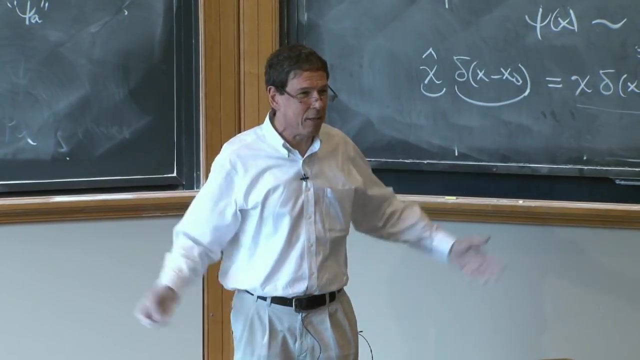 I'm disappointed that we don't derive the Schrodinger equation. Now let's derive it mathematically. But you also don't derive Newton's equations F equal ma. You have an inspiration, You get it, Newton got it, And then you use it and you see it makes sense. 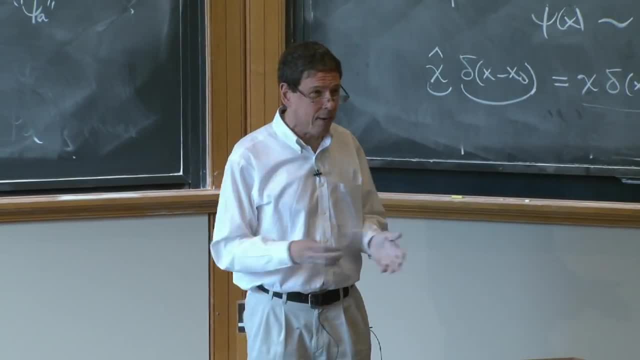 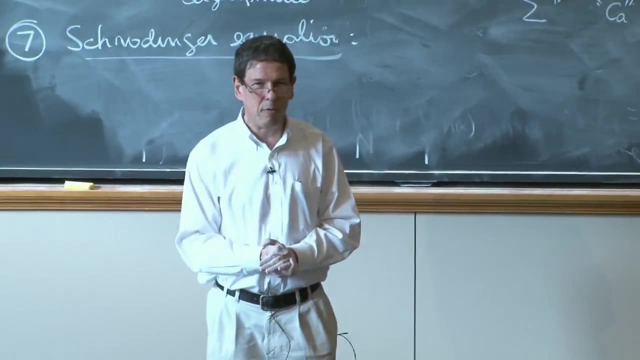 It has to be a sensible equation. And you can test very quickly whether your equation is sensible. But you can't quite derive it. So I'm a little closer to deriving the Schrodinger equation, which we say unitary time evolution. 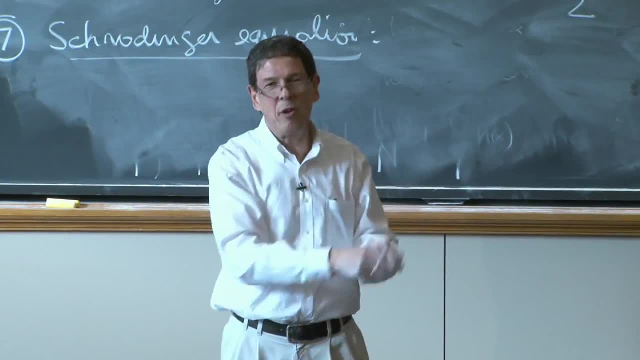 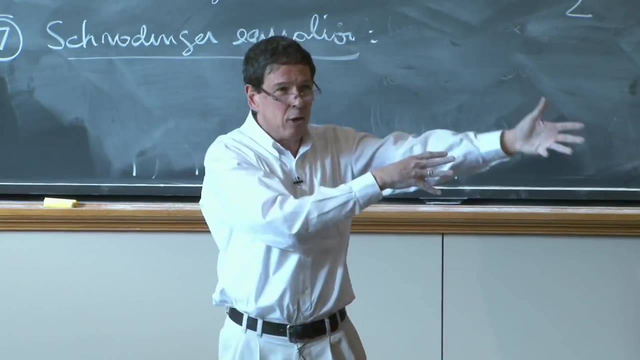 something that I haven't explained. what it is implies the Schrodinger equation And that's a mathematical fact. And you can begin Unitary time evolution, define it and you derive the Schrodinger equation, But that's just saying that you've 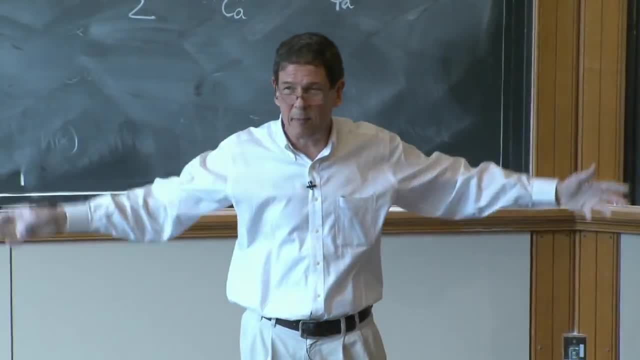 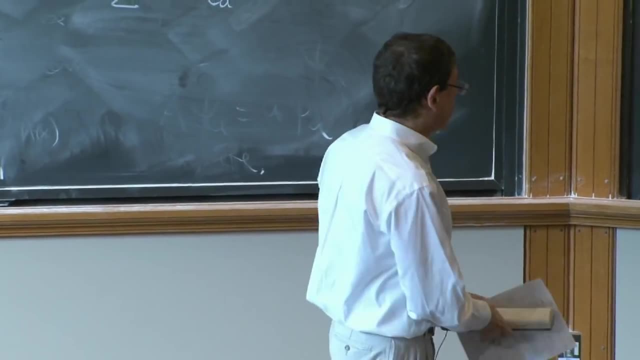 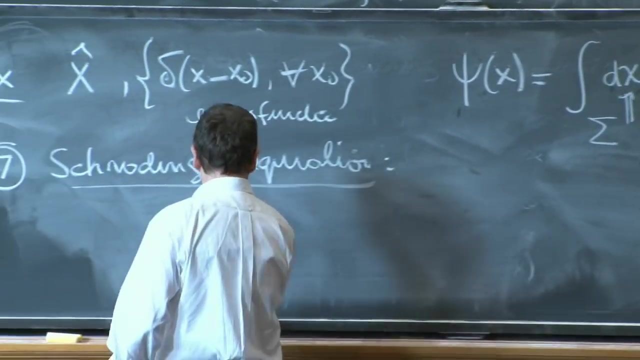 substituted the Schrodinger equation by saying there is unitary time evolution. The Schrodinger equation really comes from something a little deeper than that. Experimentally, it comes from something else. So how does it come? Well, you've studied some of the history of this subject. 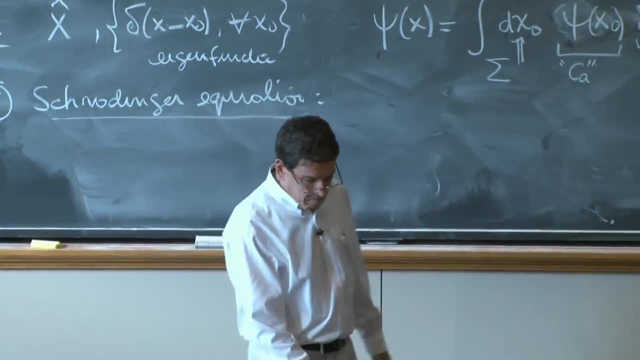 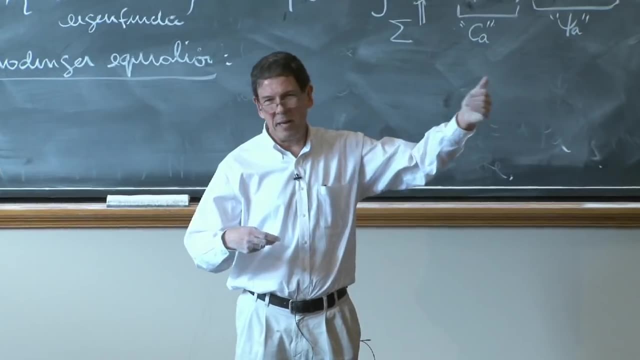 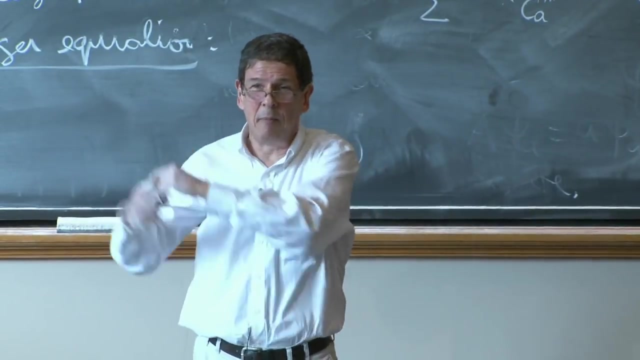 And you've seen that Planck postulated quantized energies in multiples of h bar omega. And then came Einstein and said: look, in fact the energy of a photon is h bar omega And the momentum of the photon was h bar k. 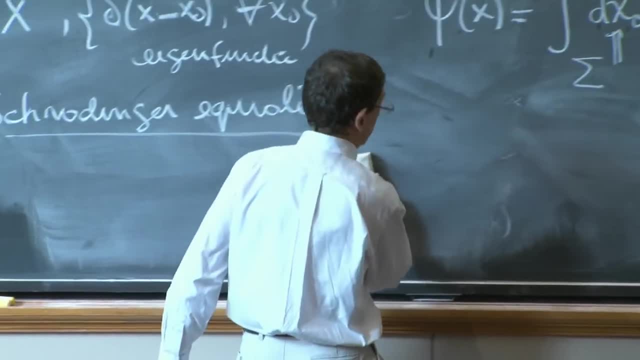 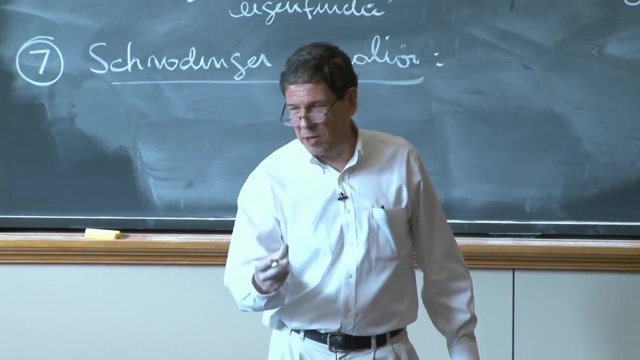 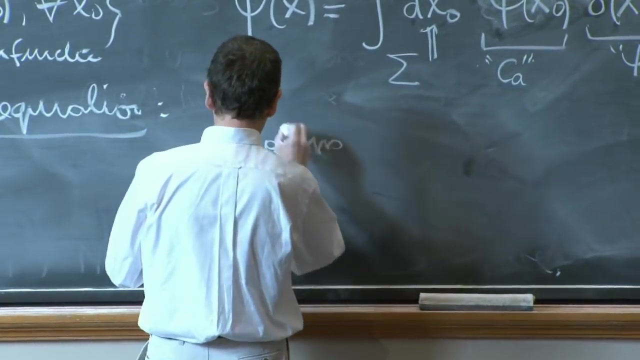 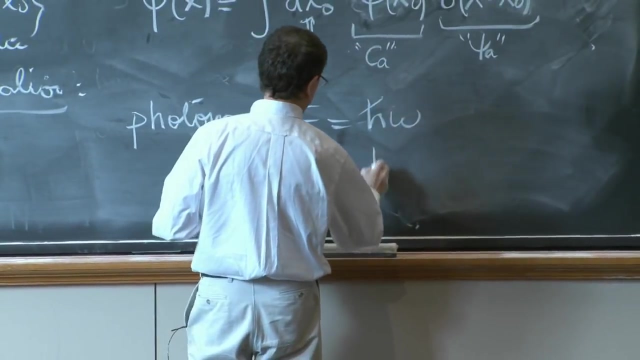 So all these people, starting with Planck and then Einstein, understood what the photon is, The quantum of photons. for photons you have, E is equal h bar omega And the momentum is equal to h bar omega, h bar k. I write them as a vector because the momentum is a vector. 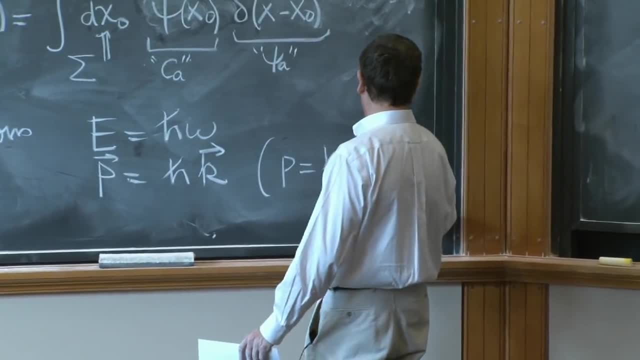 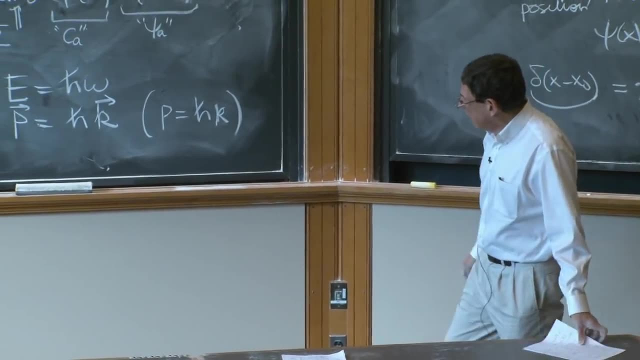 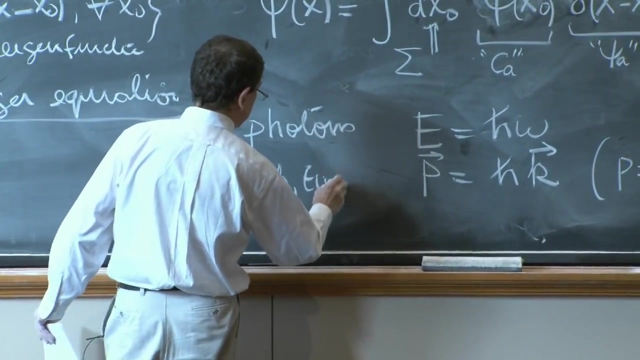 But we also write them in this course: p equal h, bar k, assuming you move just in one direction, And that's the way it's been written. So this is the result of much work, beginning by Planck, Einstein and Compton. 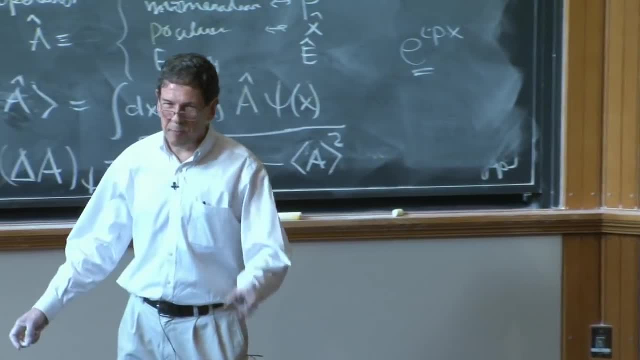 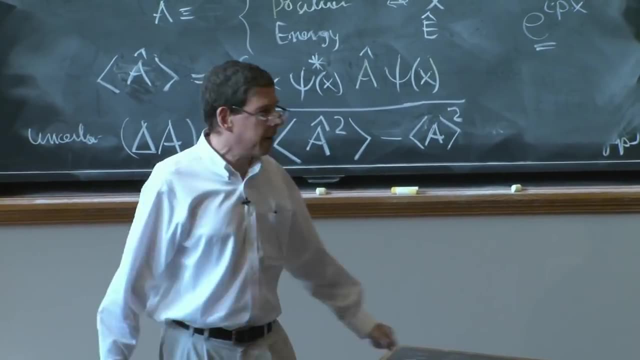 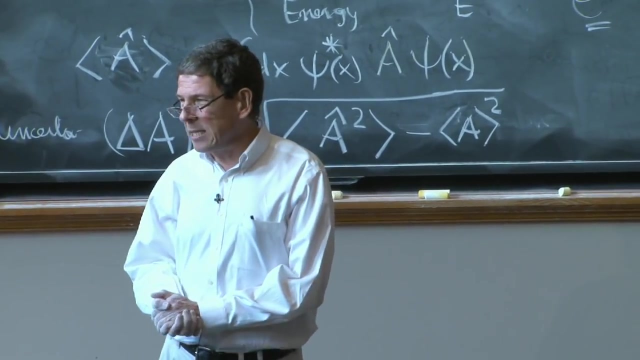 Einstein said in 1905 that there seemed to be this quantum of light that carry energy, h, omega. Planck didn't quite like that And people were not all that convinced. Experiments were done by Millikan in 1915. And people were still not quite convinced. 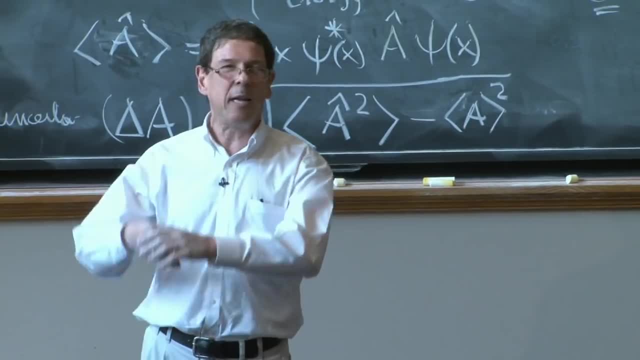 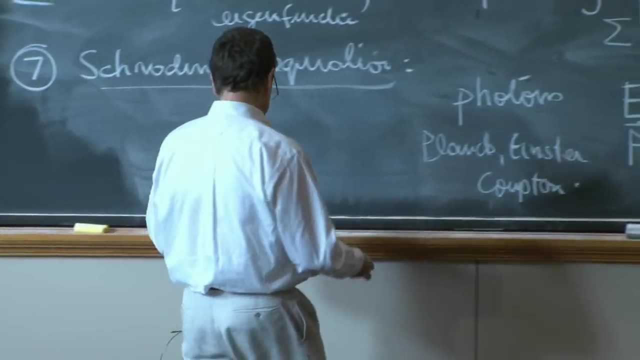 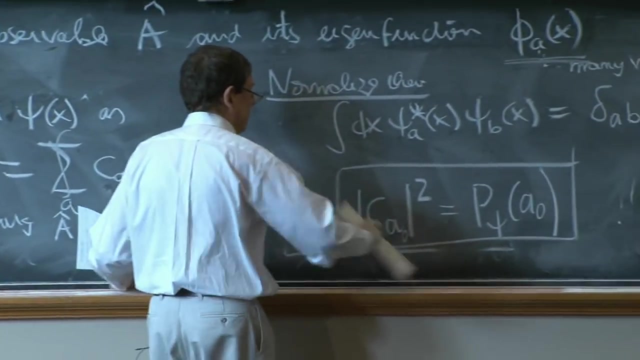 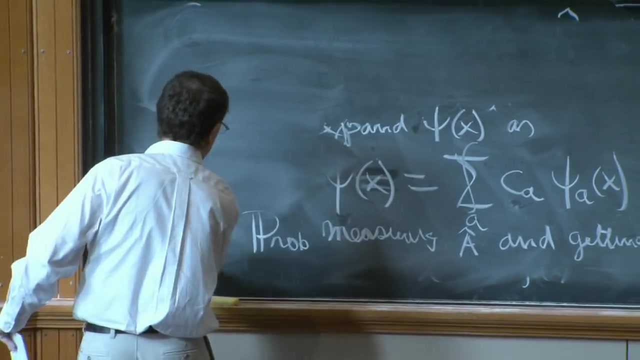 And then came Compton and did Compton scattering, And then people said, yeah, these seem to be particles. No way out of that. And they satisfied Such a relation. Now, there was something about this that was quite nice, That these photons are associated with waves. 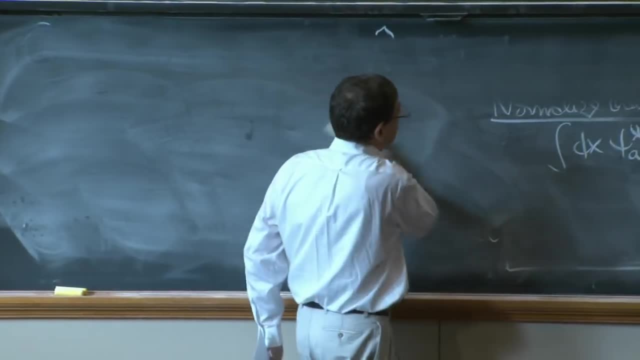 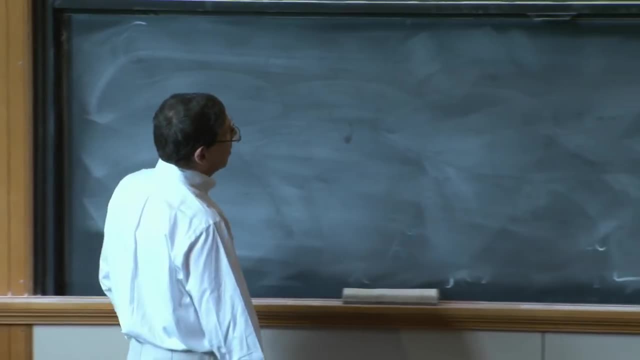 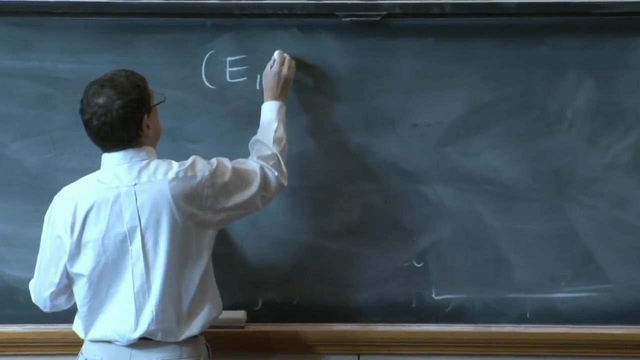 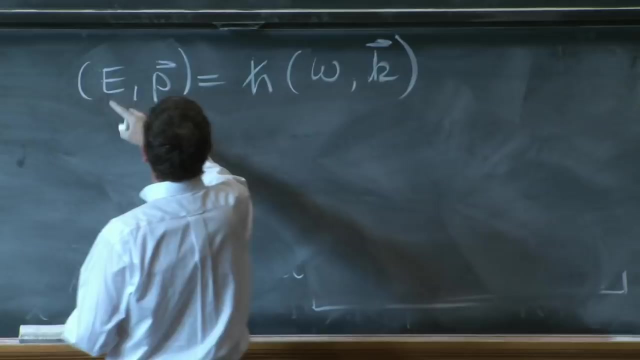 And that was not too surprising Because people understood that electromagnetic waves are waves that correspond to photons. So you can also see that this says that ep is equal to h bar omega k as an equation between vectors. You see, the e is the first and the p is the second equation. 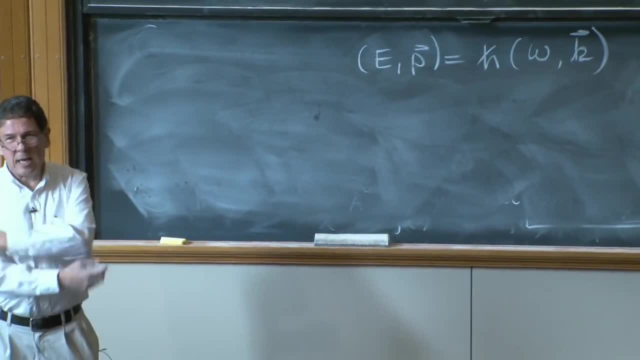 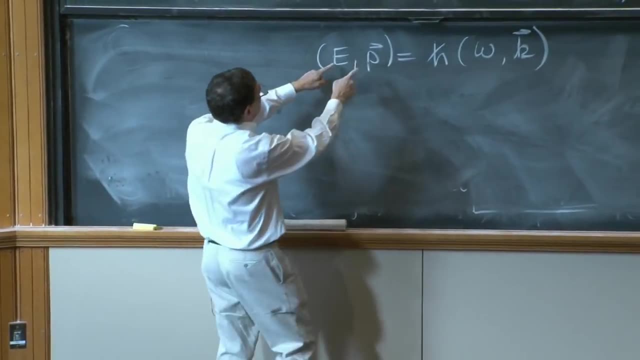 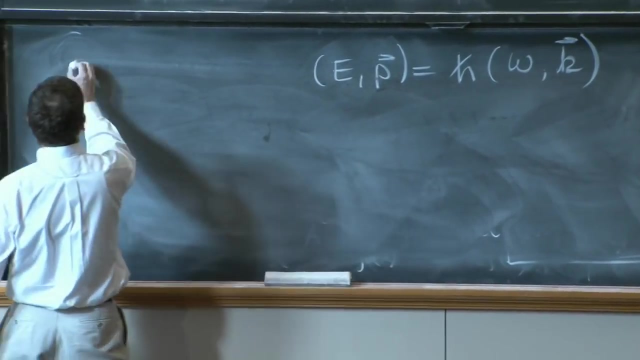 And this is actually a relativistic equation. It's a wonderful relativistic equation because energy and momentum form what is called a relativistic a four-vector. It's the four-vector. This is a little aside of relativity: Ep Four-vector. 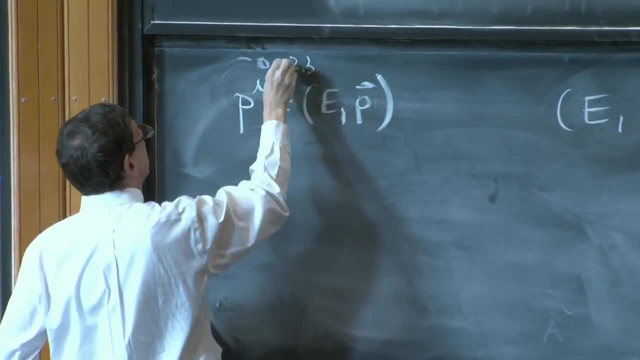 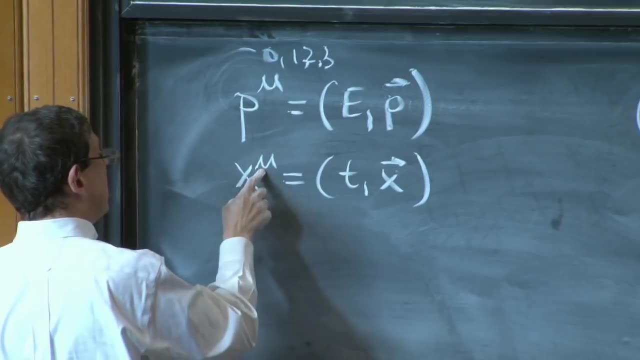 The index mu runs from 0,, 1,, 2,, 3.. Just like the x mus, which are t, and x run from x0, which is t, x1, which is x, x2, which is y, 3.. 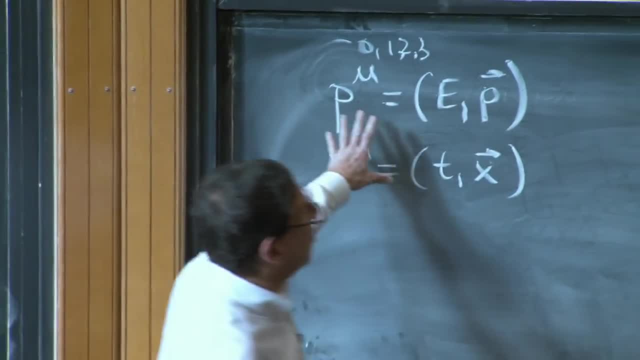 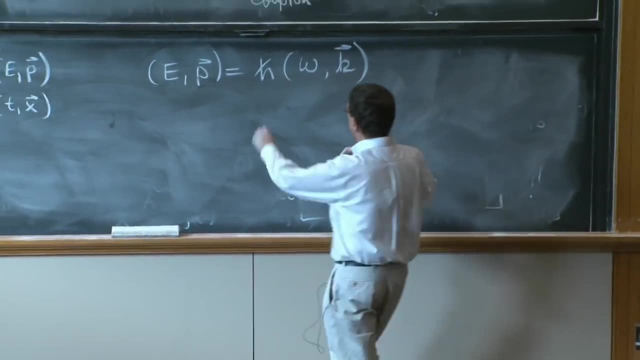 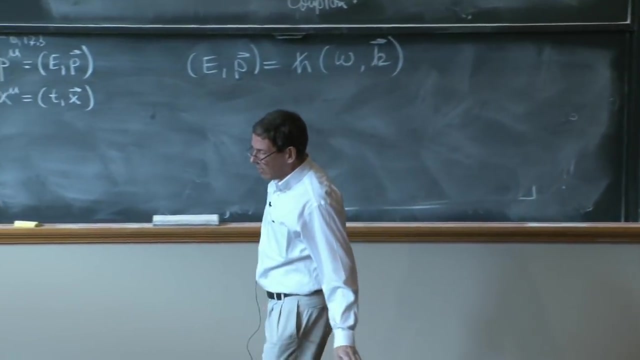 These are four vectors. And this is a four-vector, This is a four-vector. This all seemed quite pretty And this was associated to photons. But then came de Broglie, And de Broglie had a very daring idea that even though this was written for photons- 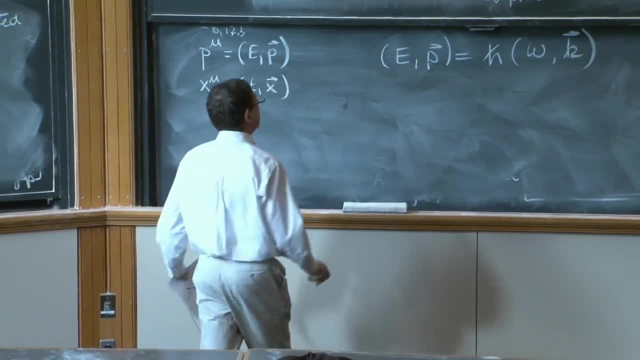 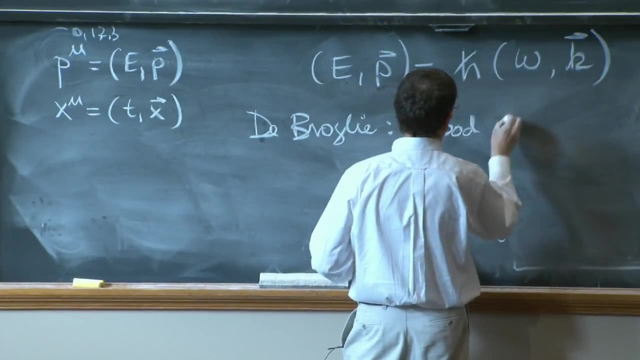 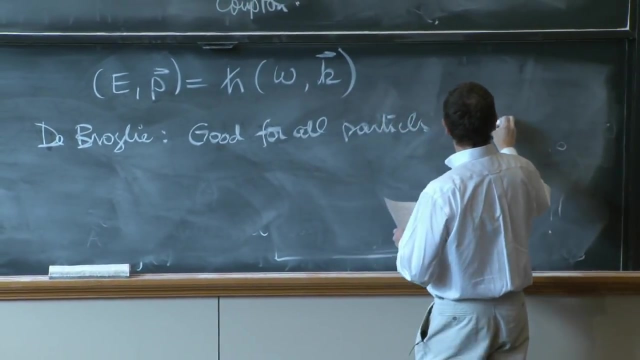 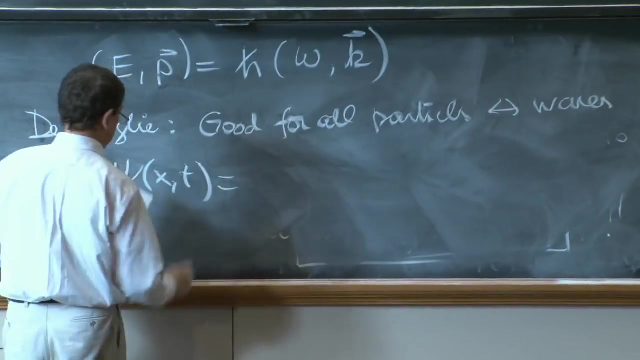 it was true for particles as well, For any particle. de Broglie says good for particles, All particles, And these particles are really waves. So what did he write? He wrote: psi of x and t is equal. a wave associated to a matter, particle. 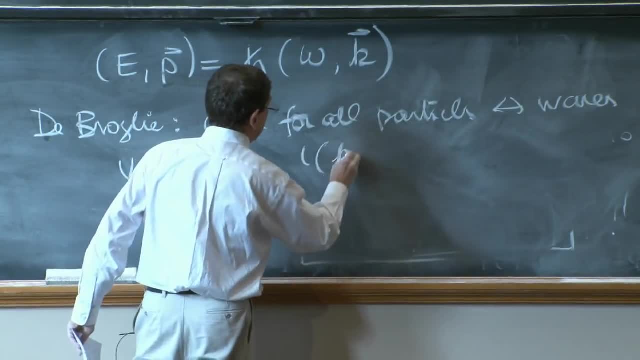 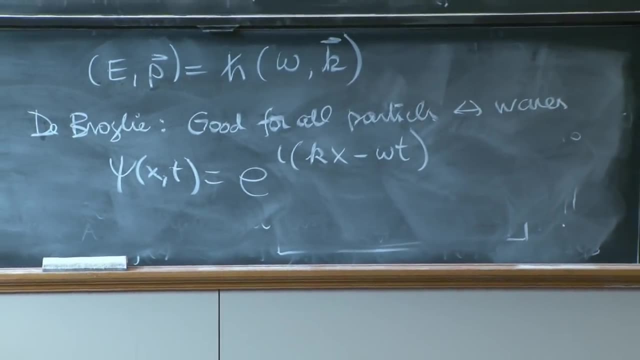 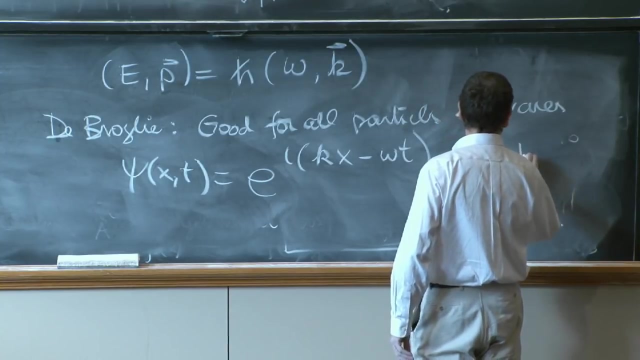 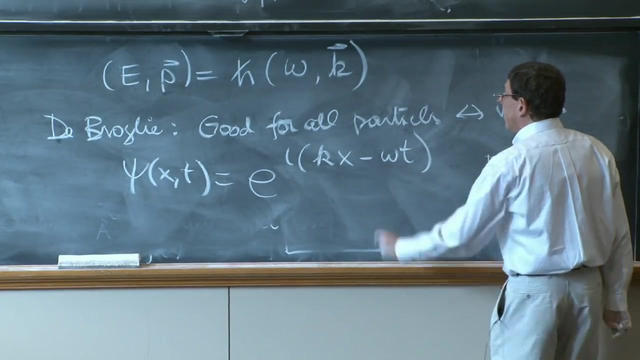 And it would be an e to the i kx minus omega t. That's a wave And you know that this wave has momentum p equal h bar k. If k is positive, look at this sign. If this sign is like that and k is positive, 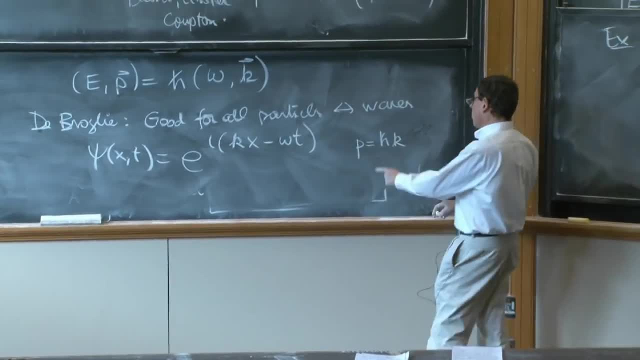 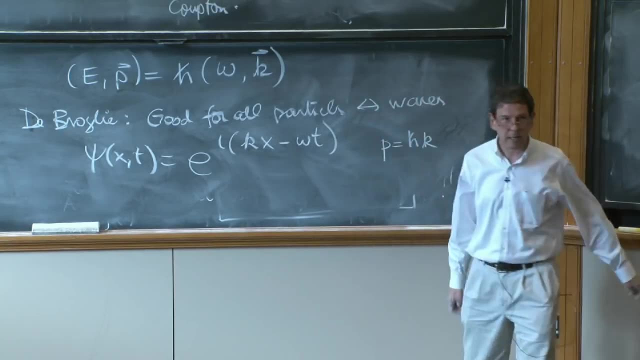 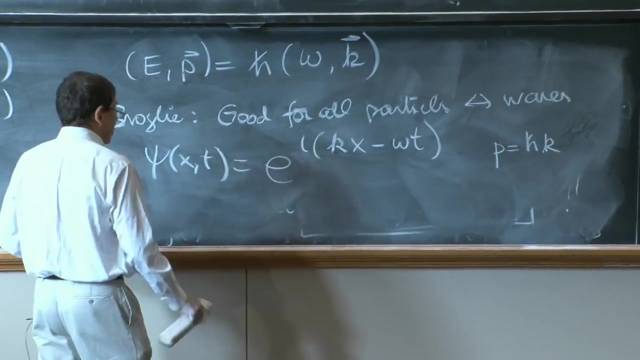 this is a wave that is moving to the right, So p being hk- if k is positive, p is positive- is moving to the right. This is a wave moving to the right And has this momentum, So it should also have an energy. 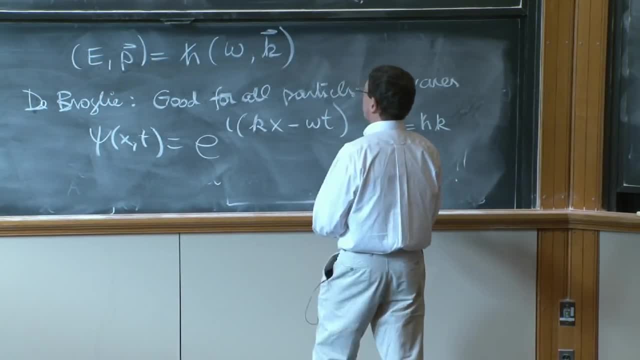 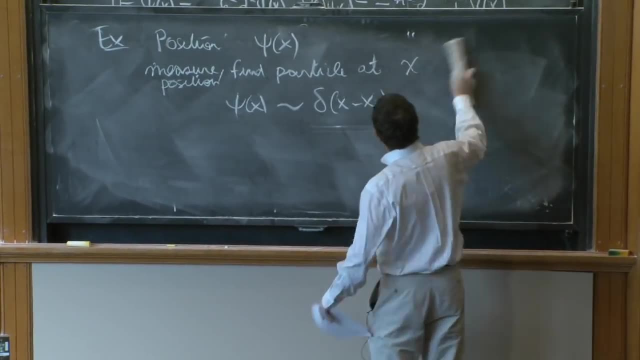 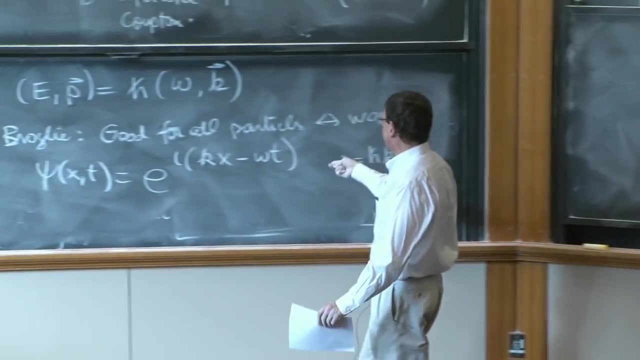 Compton said that this is relativistic because this all comes from photons. So if the momentum is given by that and the energy? the energy must also be given by a similar relation. In fact, he mostly said: look, you must have the energy being equal to h bar omega. 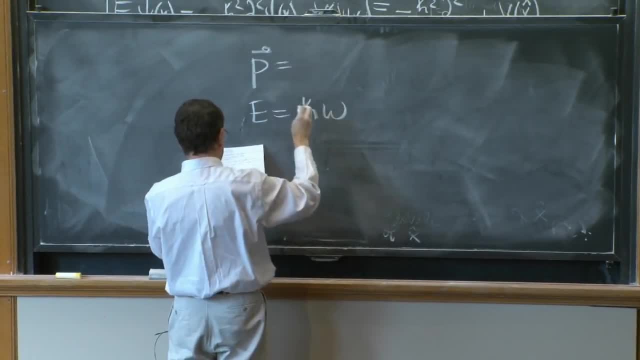 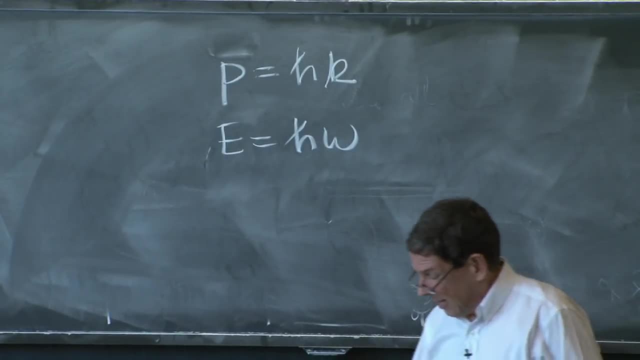 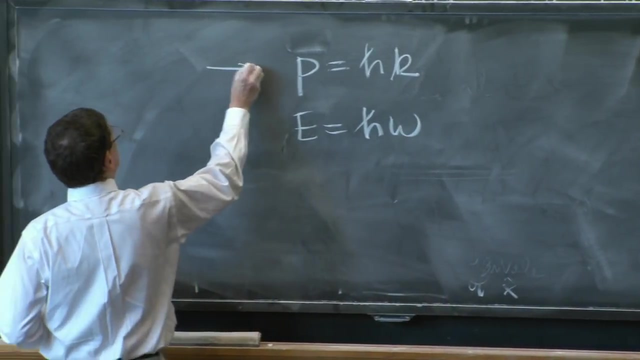 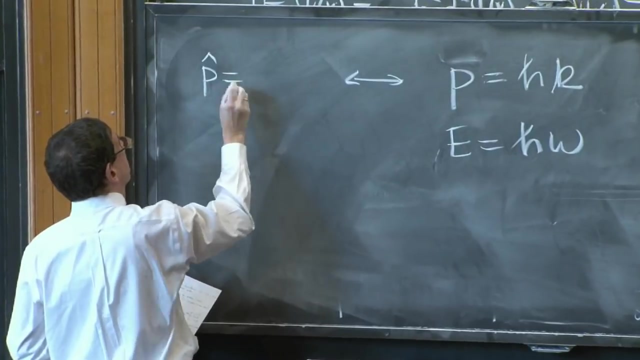 The momentum, therefore, would be equal to h bar k, And I will sometimes erase these things. So what happens with this thing? Well, momentum equal to hk. we've already understood this as momentum operator being h bar over i, d, dx. 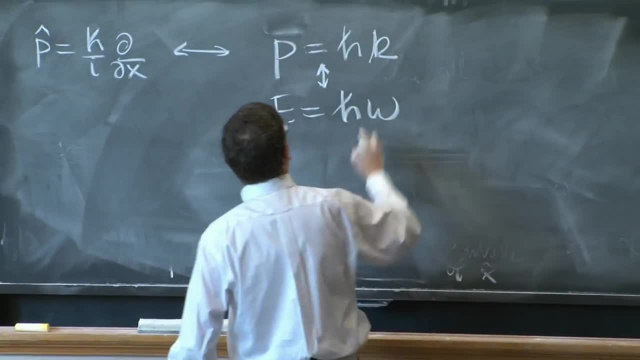 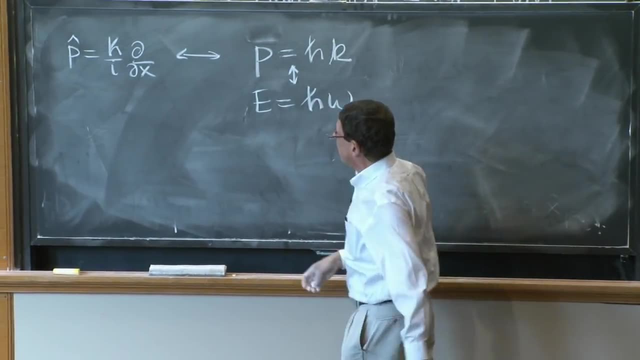 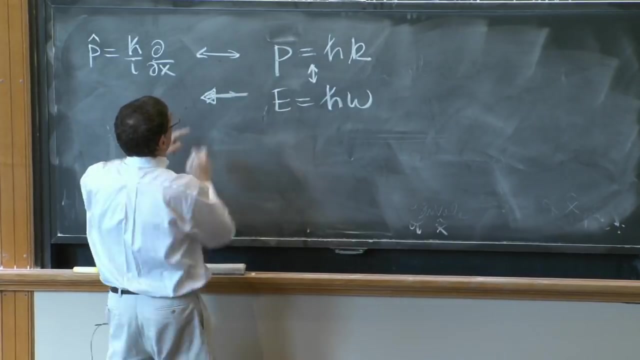 So this fact that these two must go together and be true for particles, was the Broglie's insight and the connection to relativity. Now, here we have this. So now we just have to try to figure out what could we do for the energy. 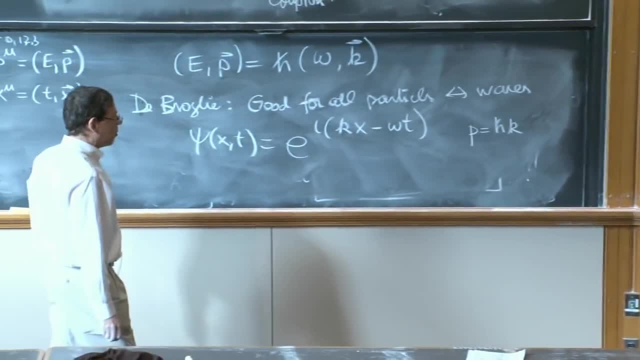 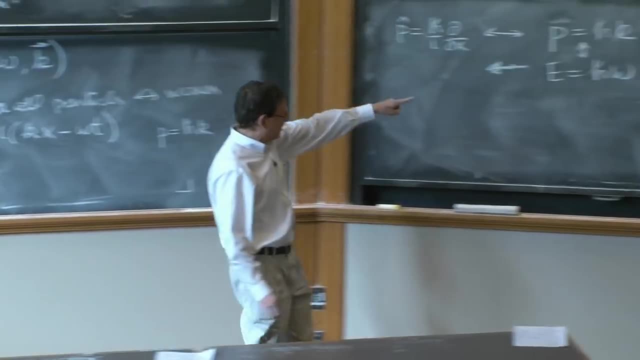 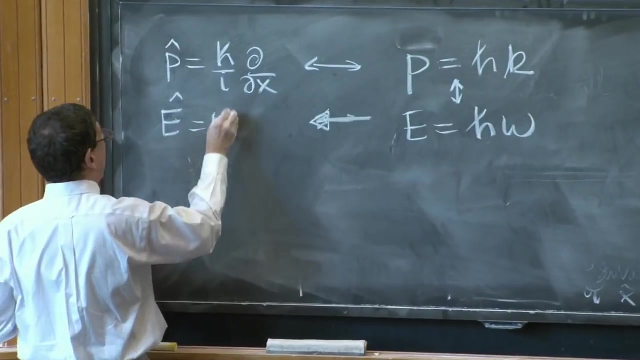 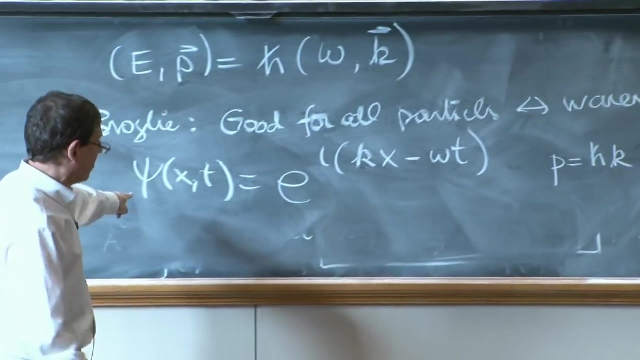 Could we have an energy operator? What would the energy operator have to do? Well, if the energy operator is supposed to give us h bar omega, the only thing it can be is that the energy is ih bar d, dt. Why? Because you go again at the wave function. 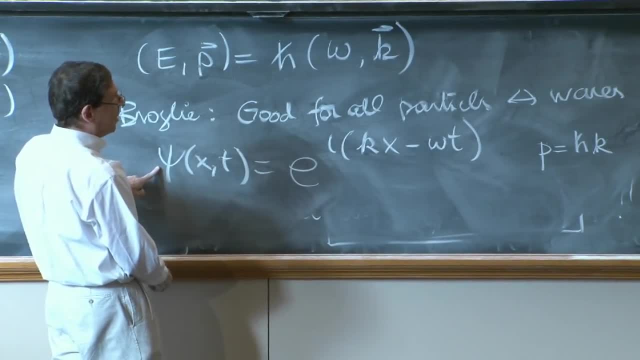 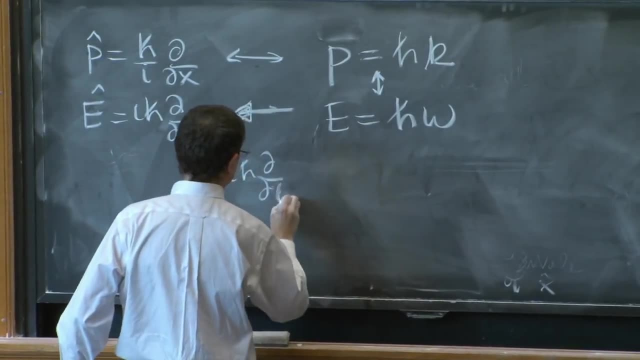 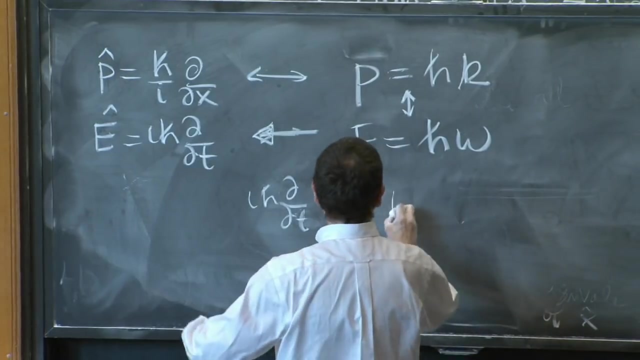 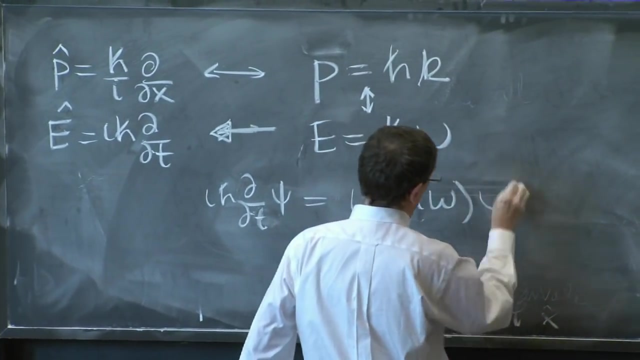 And you take ih bar d dt And what do you get? ih bar d dt on the wave function is equal to ih bar. You take the d dt, You get minus i omega times the whole wave function. So this is equal h bar omega times the wave function. 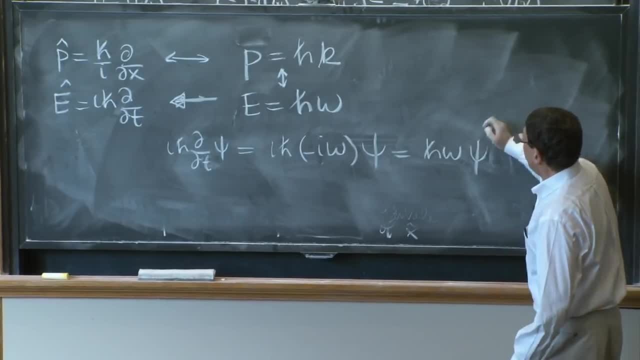 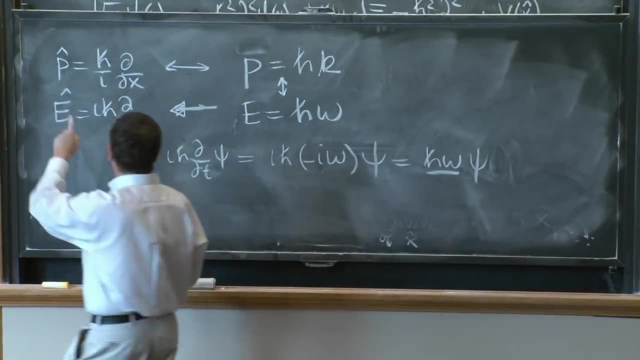 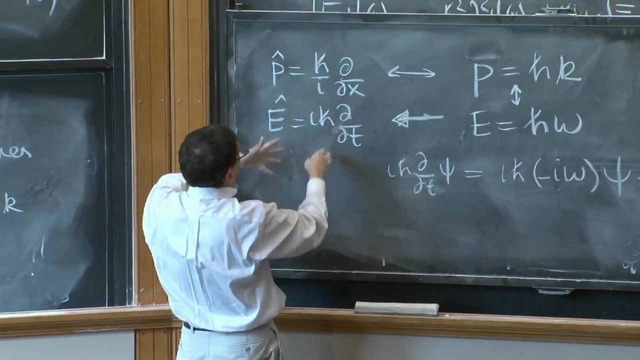 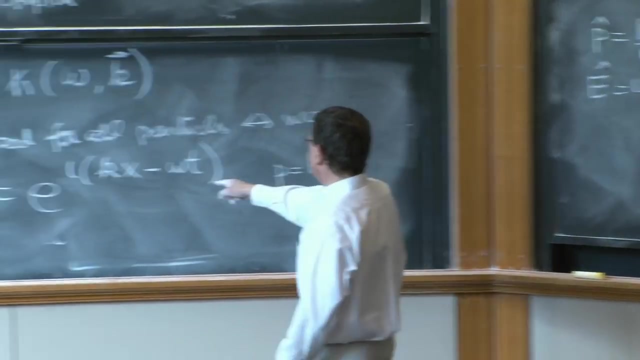 Times the wave function like that. So here it is: This is the operator that realizes the energy, just like this is the operator that realizes the momentum. You could say these are the main relations that we have. So if you have this wave function, 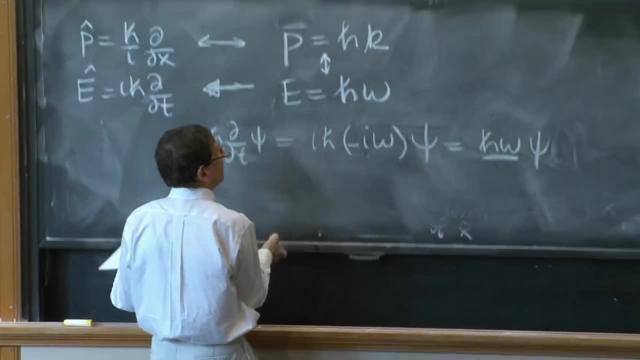 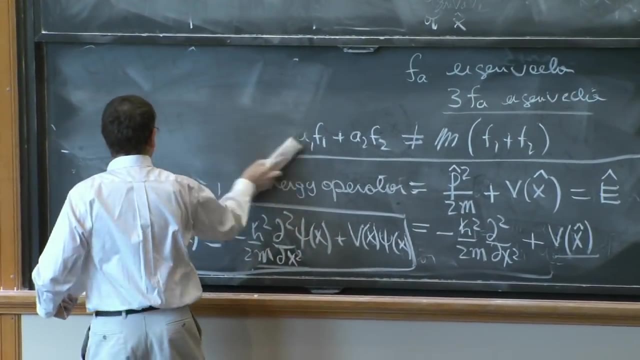 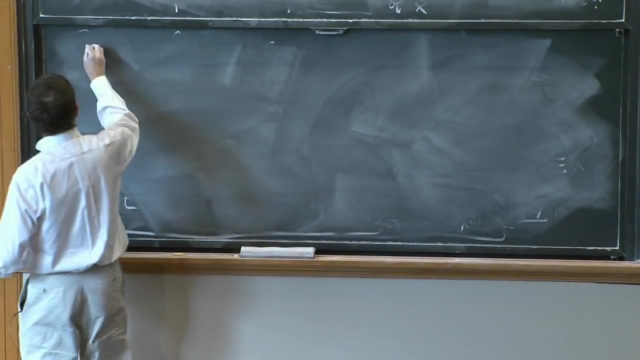 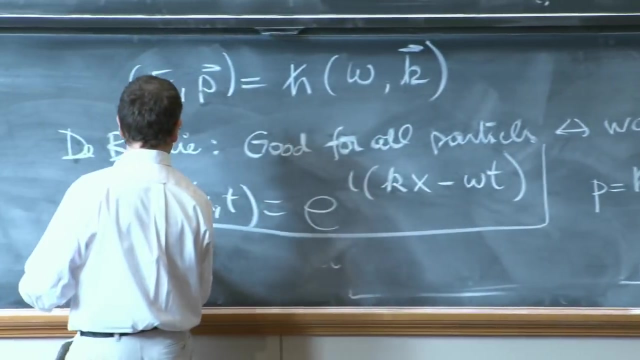 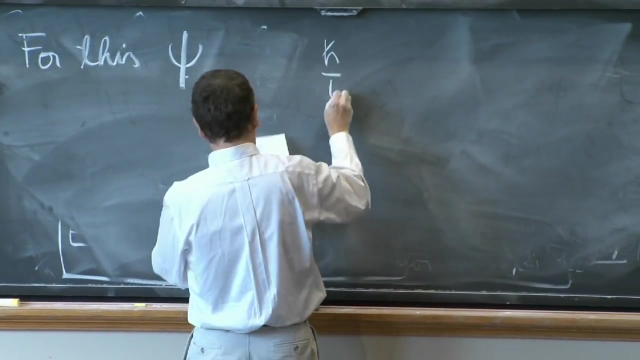 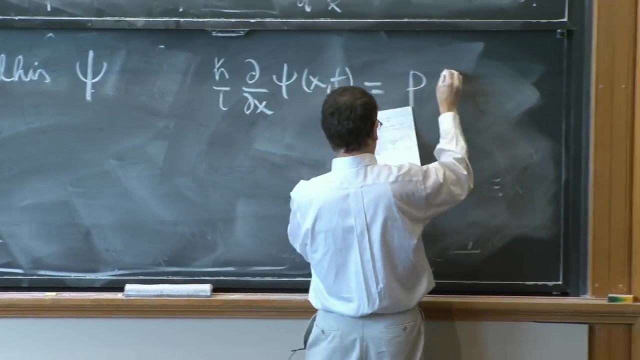 it corresponds to a particle with momentum h bar, Momentum h k and energy h omega. So now we write this. So for this psi, this psi that we have here, h bar over i d, dx of psi of x Times, psi of x and t is equal to the value of the momentum. 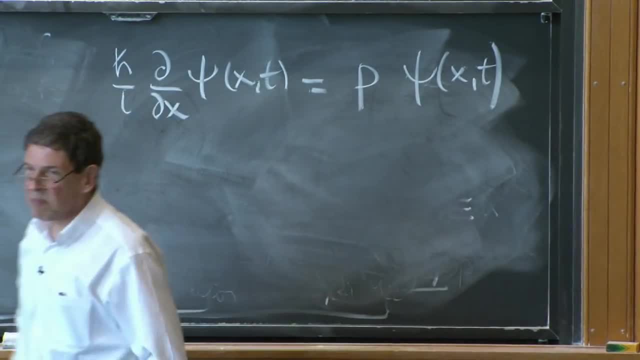 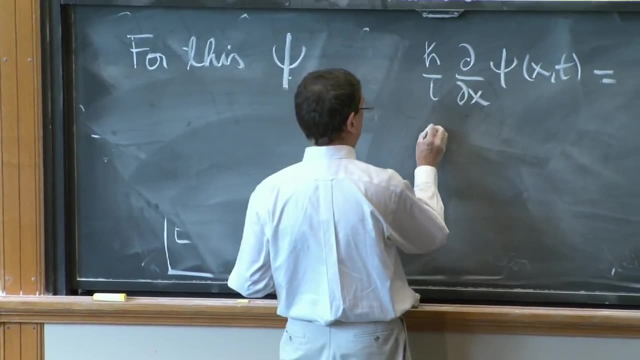 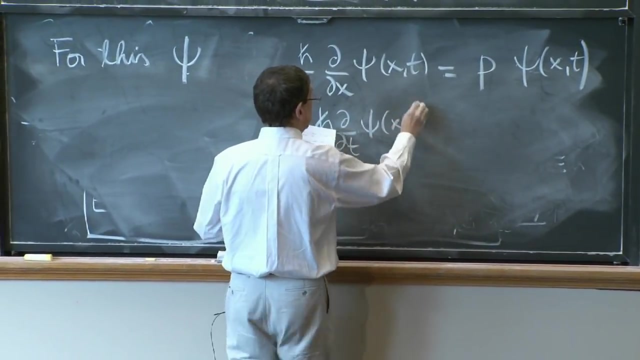 times psi of x and t. That is something we've seen. But then there's a second one For this psi. we also have that ih bar d dt of psi of x and t is equal to the energy of that particle times x and t. 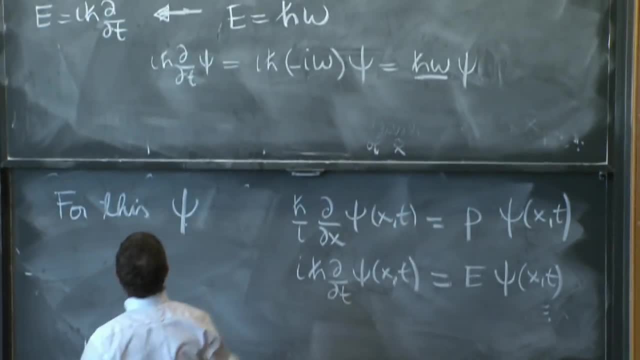 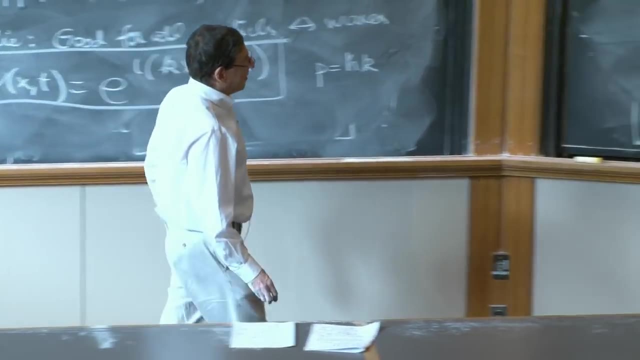 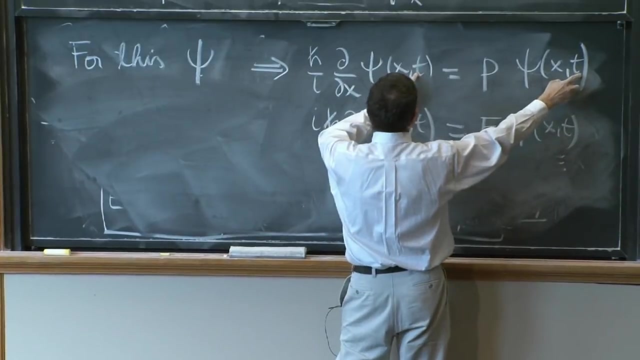 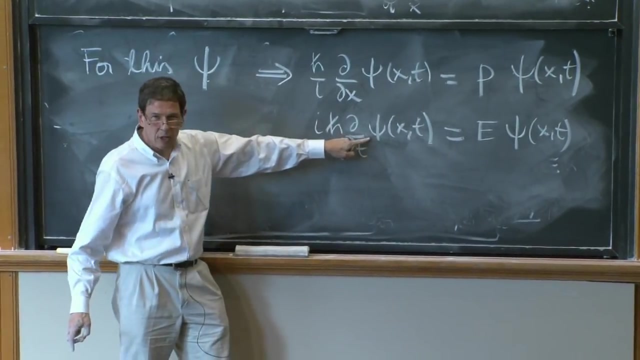 Because the energy of that particle is h bar omega, And look, This is familiar. And here the t plays no role. But here the t plays a role And this is prescribing you how a wave function of energy, e, evolves in time. So you're almost there. 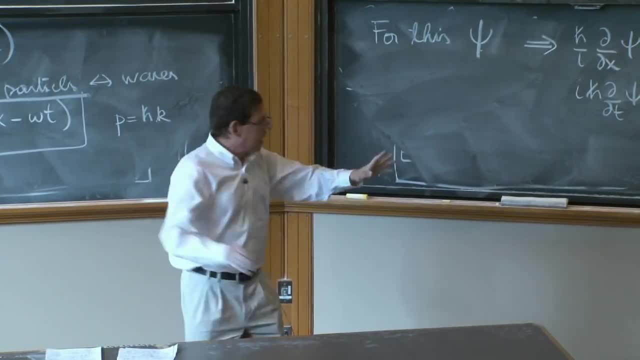 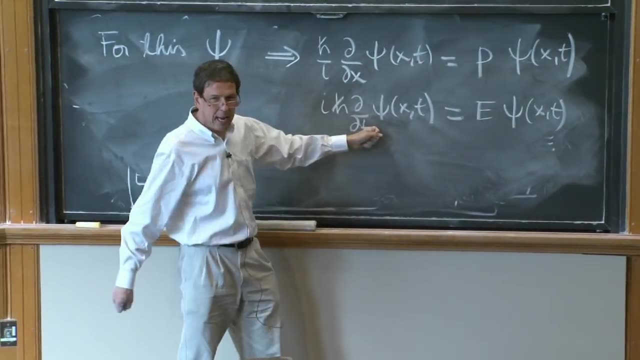 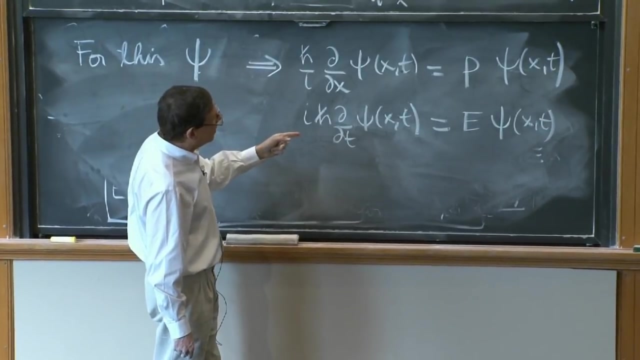 You have something very deep in here. It's telling you if you know the wave function and it has energy e. this is how it looks. later You can take this derivative and solve this differential equation. Now this differential equation is kind of trivial because e is a number here. 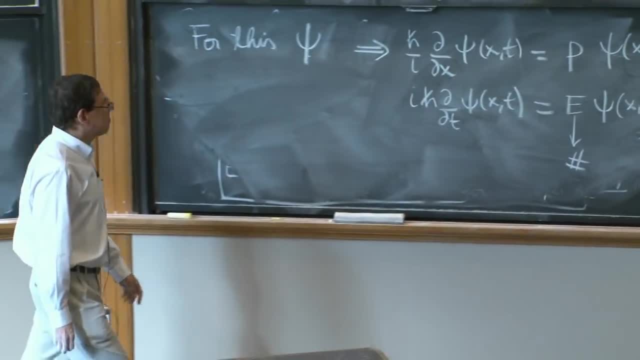 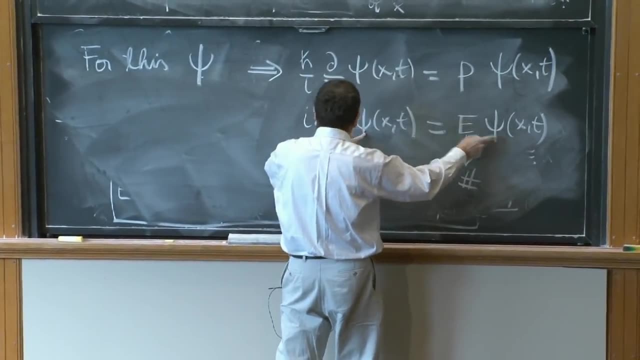 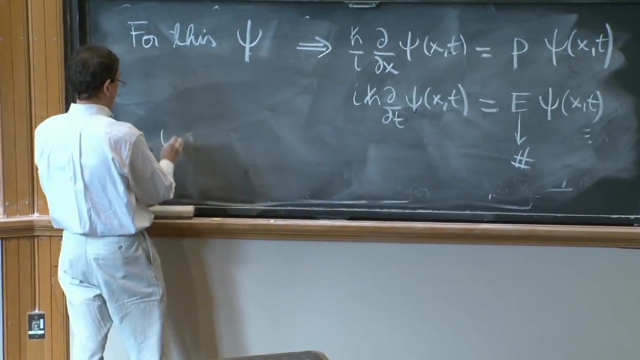 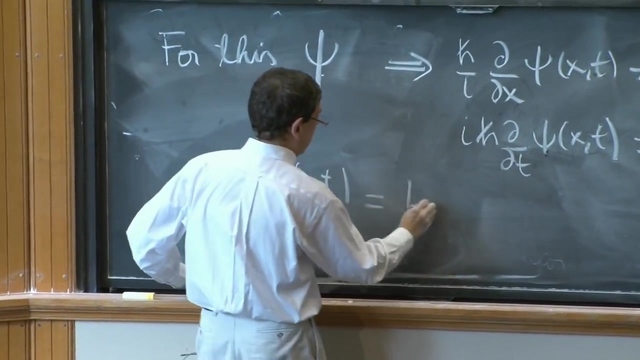 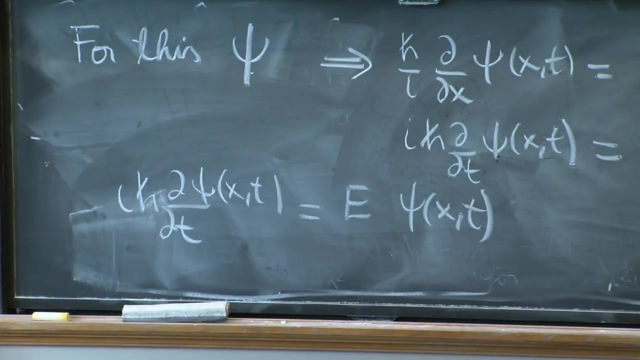 But if you know that you have a particle with energy e, that's how it evolves in time. So came Schrodinger and looked at this equation: Psi of x and t equal e. psi of x and t. This is the equation. This is true for any particle that has energy e. 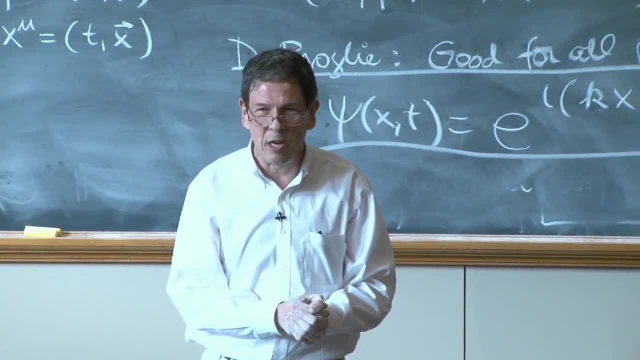 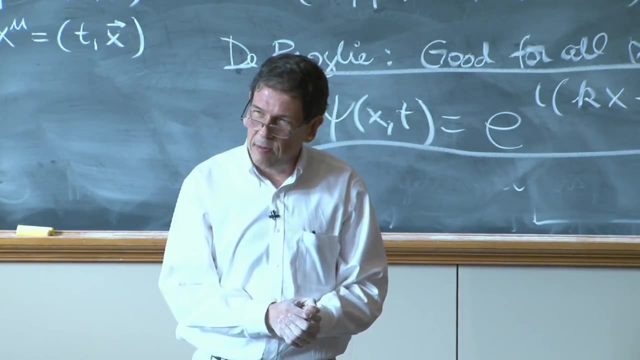 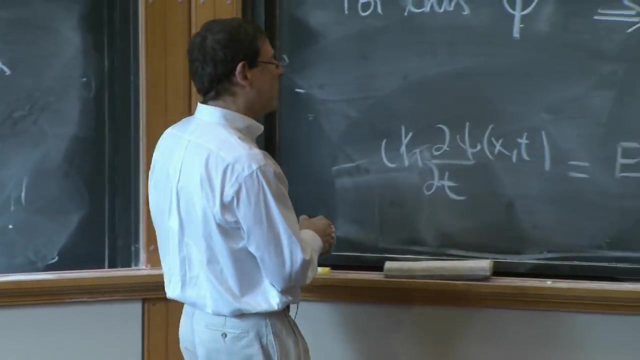 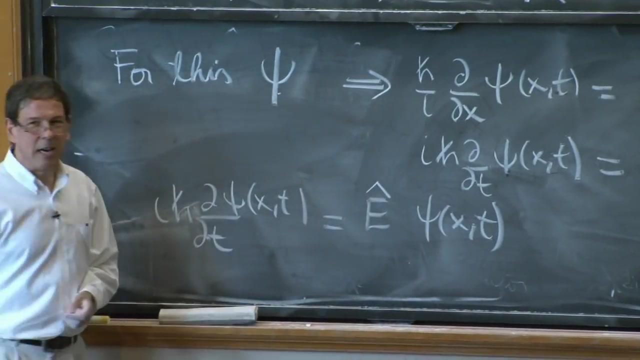 How can I make out of this a full equation? Because maybe I don't know what is the energy e? The energy e might be anything in general. What can I do? Very simple, One single replacement on that equation. Done It's over. 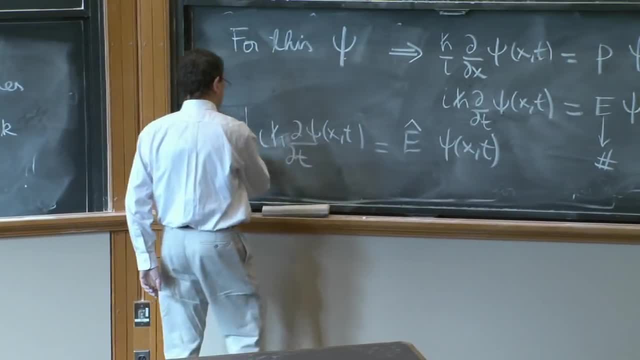 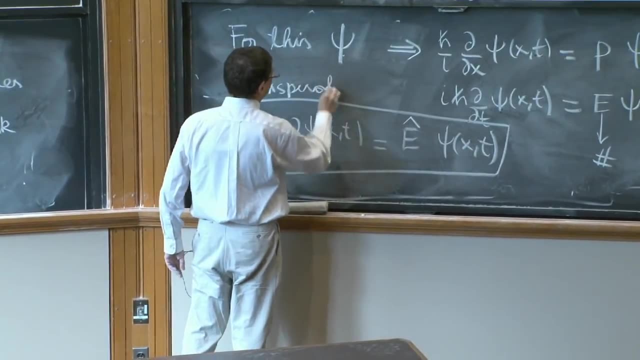 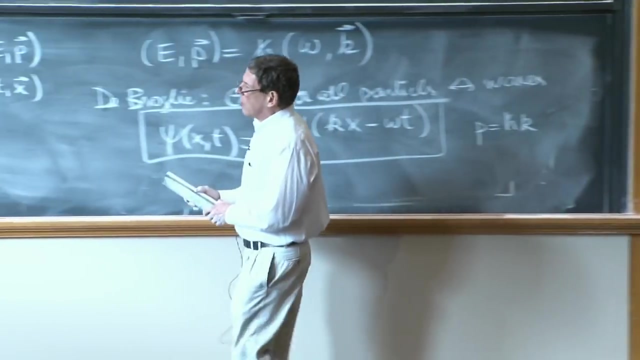 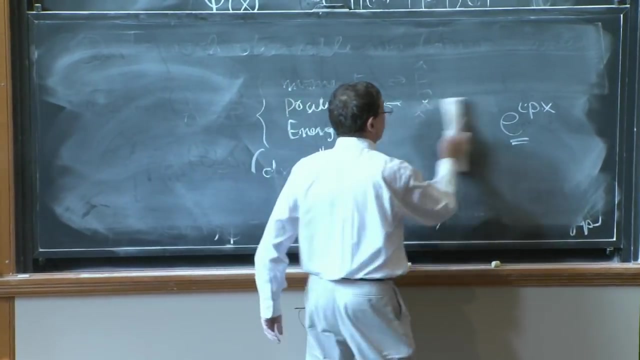 That's the Schrodinger equation. It's the energy operator that we introduced before Inspiration. Change e to e hat. This is the Schrodinger equation. Now, what has really happened here? this equation that was trivial for a wave function that 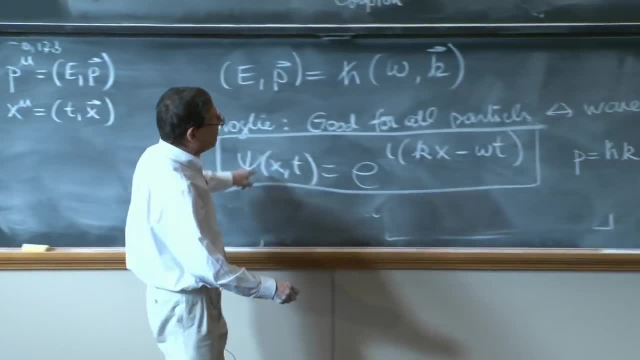 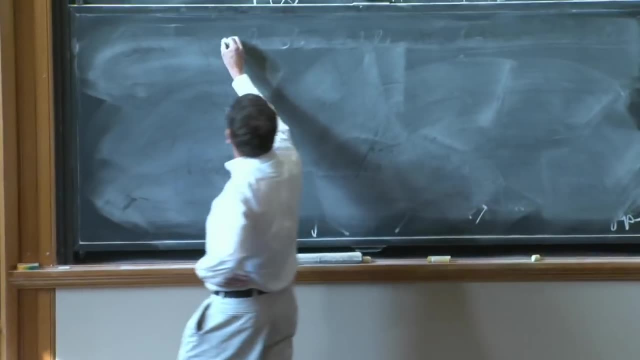 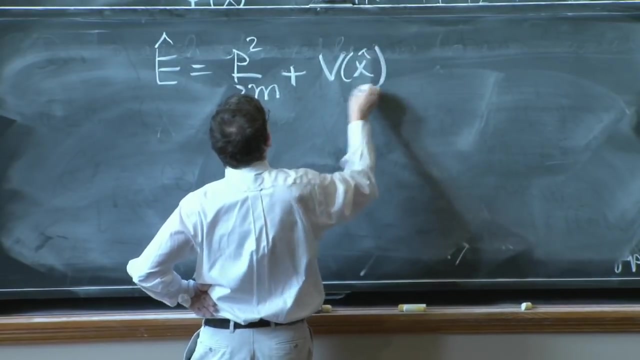 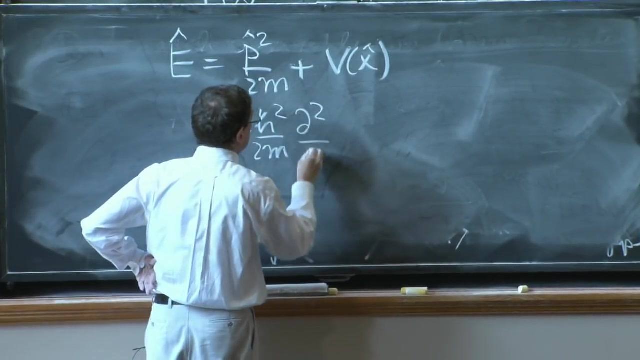 represented a particle with energy e. if this is the energy operator, this is not so easy anymore Because, remember, the energy operator, for example, was p squared over 2m plus v of x, And this was minus h squared over 2m d, second dx squared. 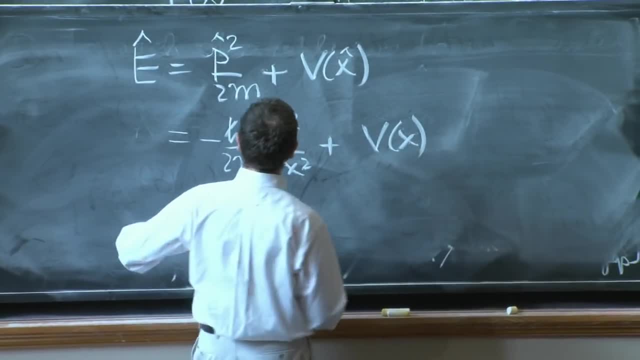 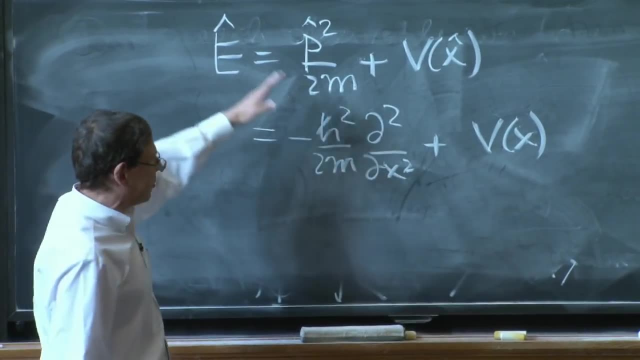 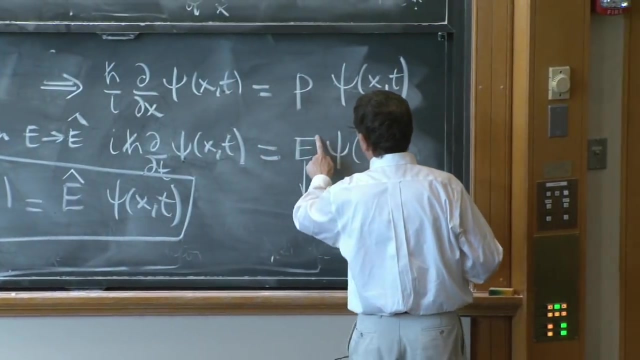 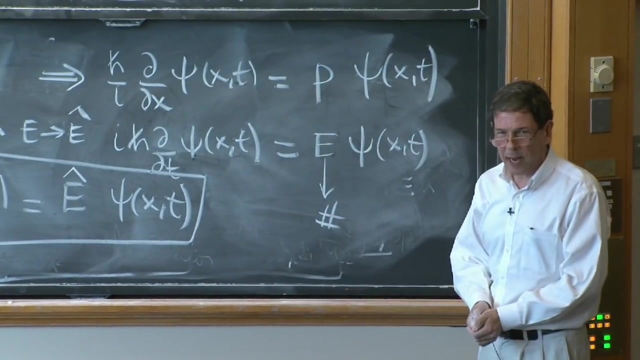 plus v of x acting on wave functions. So now you've got a really interesting equation, Because you don't assume that the energy is a number, because you don't know it In general, if the particle is moving in a complicated potential, you don't know what are the possible energies. 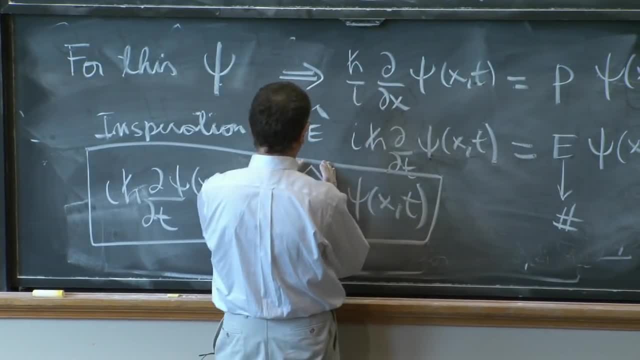 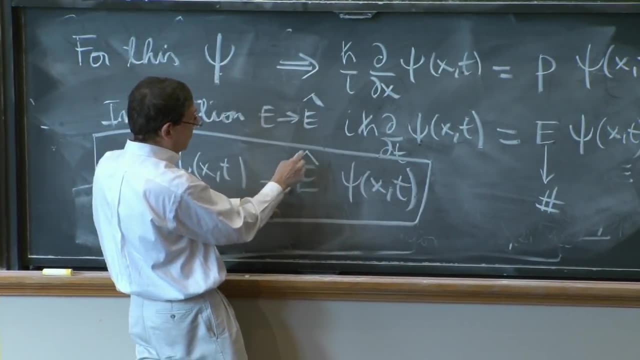 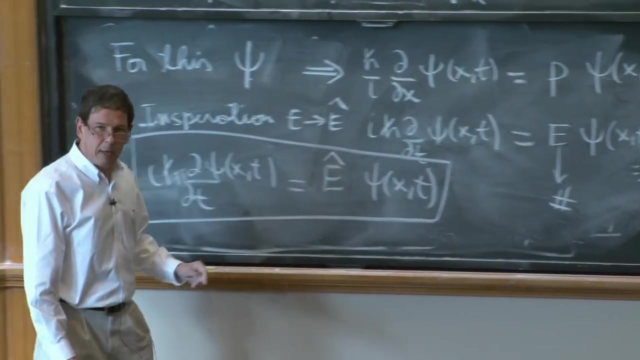 But this is symbolically what must be happening, because if this particle has a definite energy, then this energy operator gives you the energy acting on the function, And then you recover what you know is true for a particle of a given energy. So in general, the Schrodinger equation. 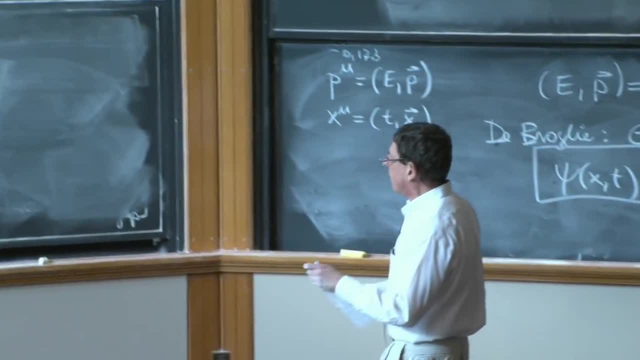 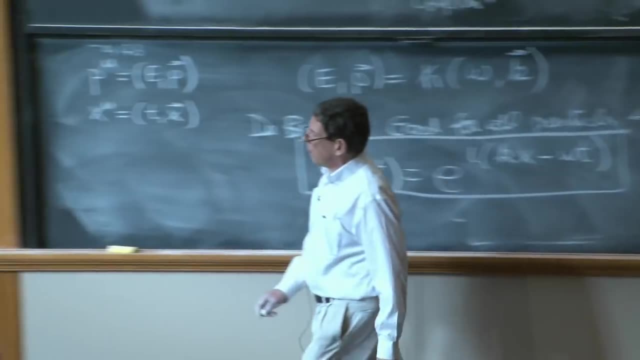 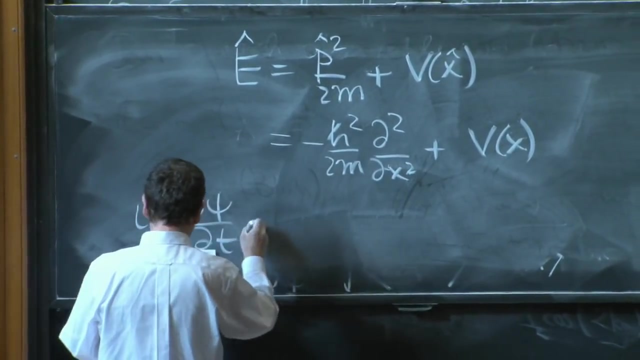 is a complicated equation. Let's write it now completely. So this is the Schrodinger equation, And if we write it completely, it will read: ih bar d, psi d. psi dt is equal to minus h. bar squared over 2m d second dx.